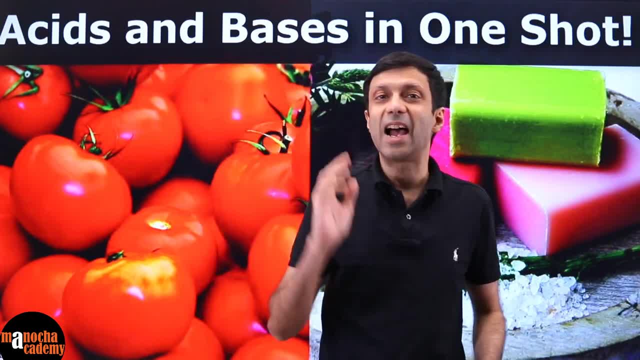 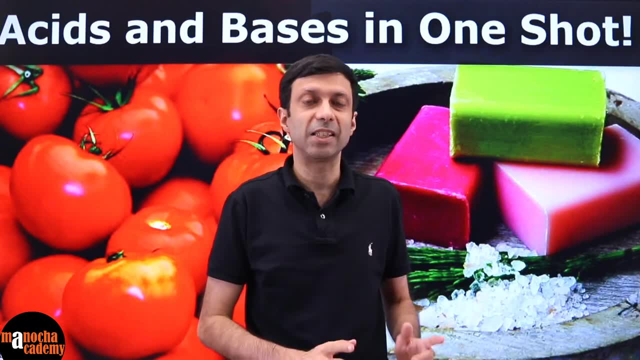 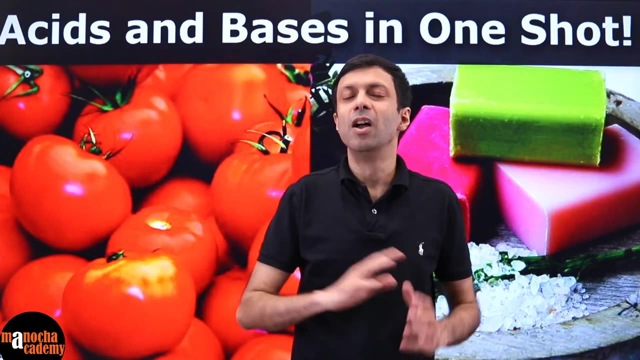 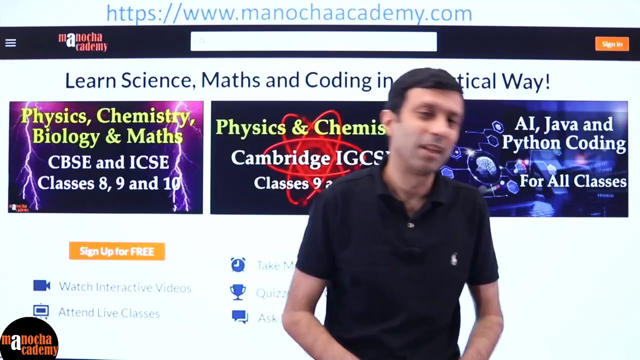 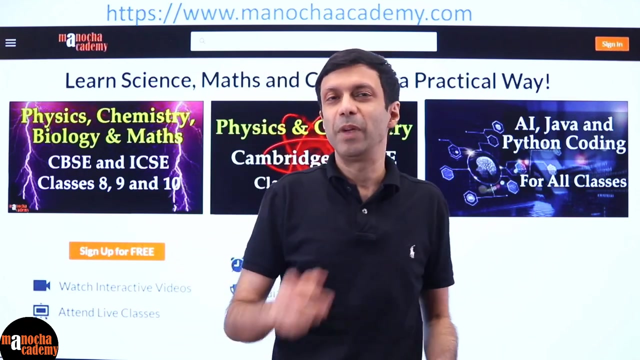 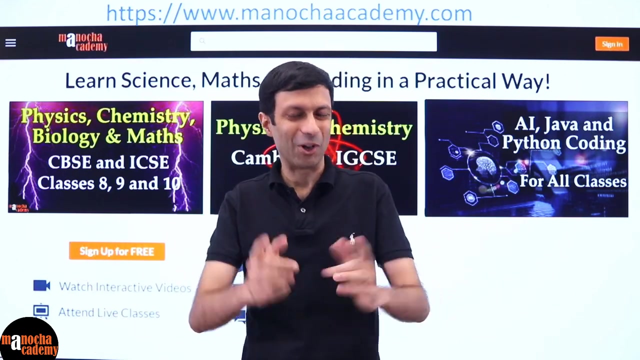 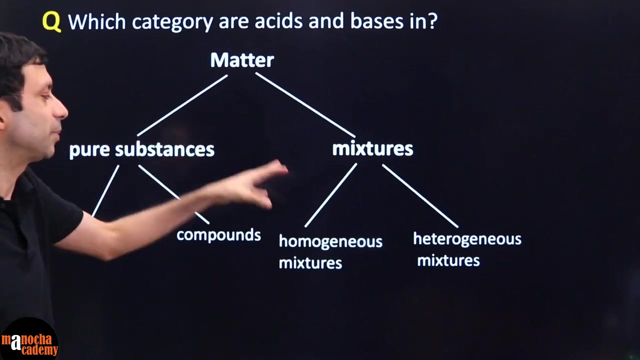 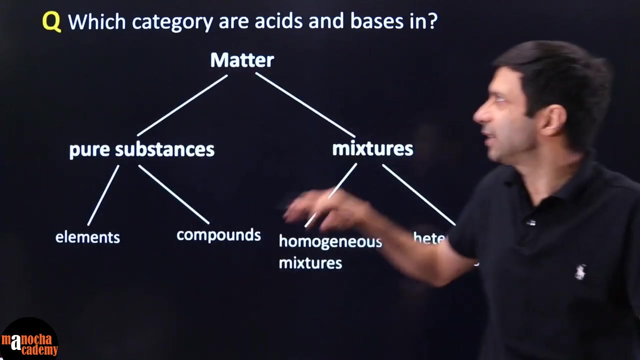 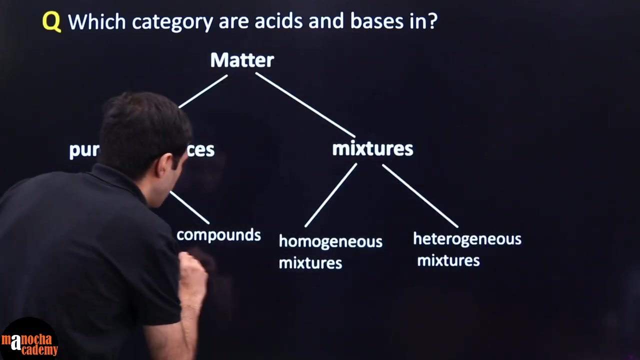 Hi everyone, welcome to this class where we'll be looking at acids and bases in one shot. So this will be a great revision for you on the topic of acids and bases. Please make sure you guys watch the earlier videos on what is an acid, what is a base and in this class we are going to cover both acids and bases in the acid-base salt chapter. So keep your pen and paper ready and let's dive into it. Before we begin, I just want to quickly say do check out the other courses on our website and our Android app. Do share it out with your friends. Make sure you have subscribed to our YouTube channel and follow us on Facebook and Instagram. So stay connected with Manocha Academy and keep on learning. So can you guys tell me which category do acids and bases come under? You know matter can be divided into pure substance mixtures, pure substance can be divided into elements and compounds, mixtures as homogeneous or heterogeneous mixture. Where does acid, bases or even salts come in? So please understand they all acids, bases, salts, bases come in. So please understand they all acids, bases, salts, bases come in. So please understand they all acids, bases, salts, bases, salts, bases come in. So please understand they all acids, bases, salts, bases come in. So please understand they all acids, bases, salts, bases, salts, bases come in. So please understand they all acids, bases, salts, bases, salts, bases come in. So please understand they all acids, bases, salts, bases come in. So please 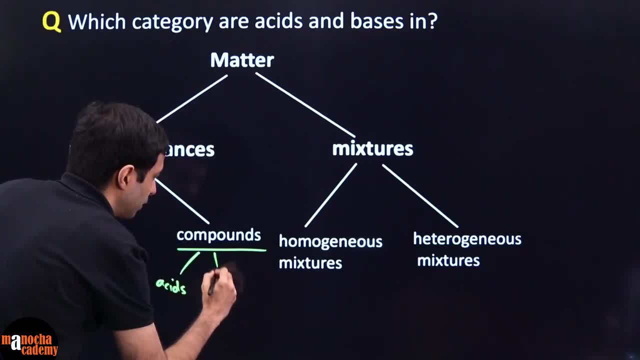 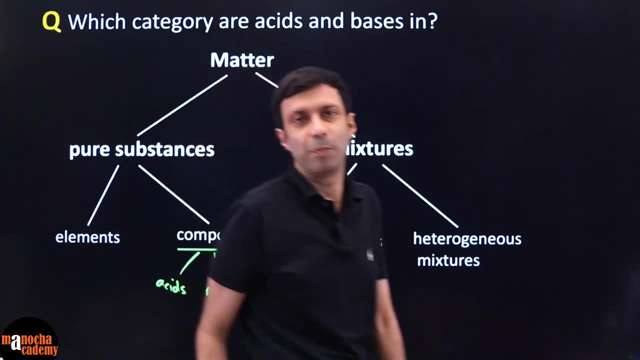 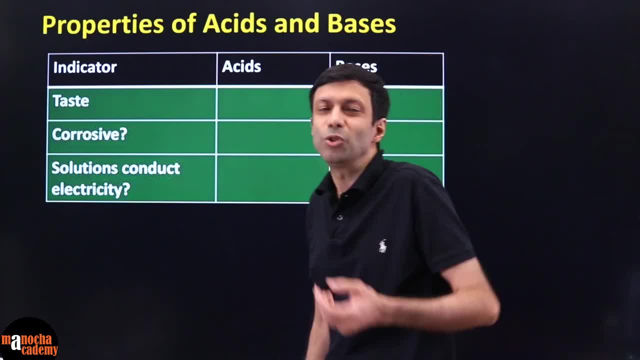 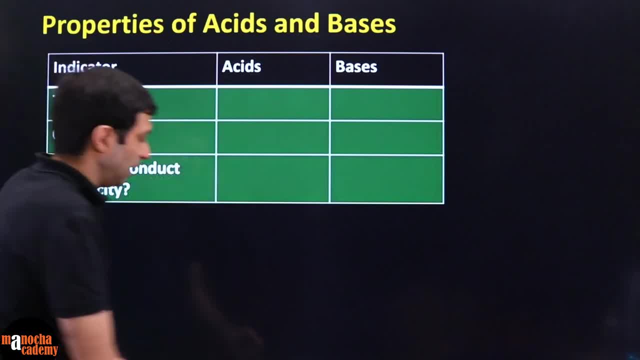 vinegar or you have tasted lemon juice it clearly has a sour taste now don't go around tasting 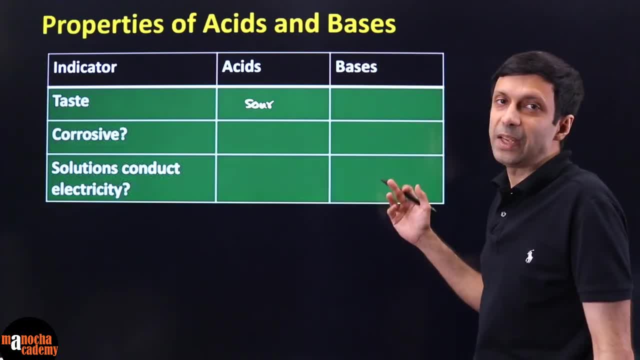 acids right so acid as a sour taste what about bases bases typically tend to have a bitter taste 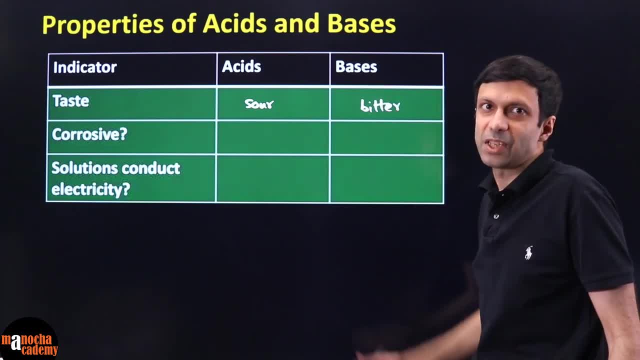 it is easy to remember B for base B for bitter sour you know acid rate you have tasted corrosive 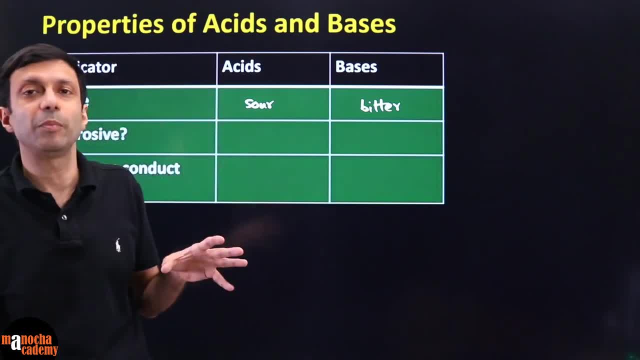 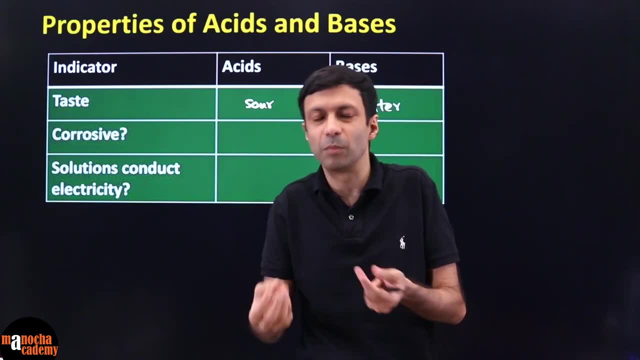 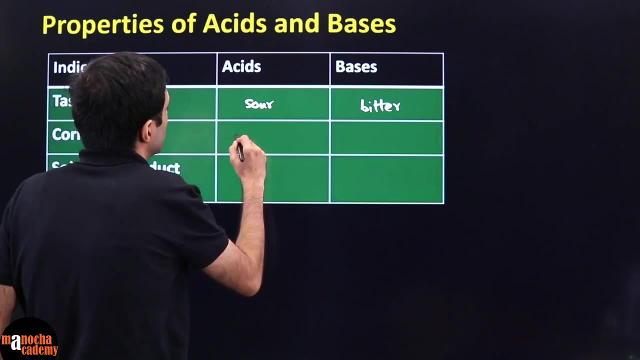 are they corrosive yes what is first of all what is the meaning of corrosion corrosion means it eats up the substance for example if you take acid and you put it on sponge or you know some rubber material it will eat up through it highly dangerous okay so acids are definitely corrosive 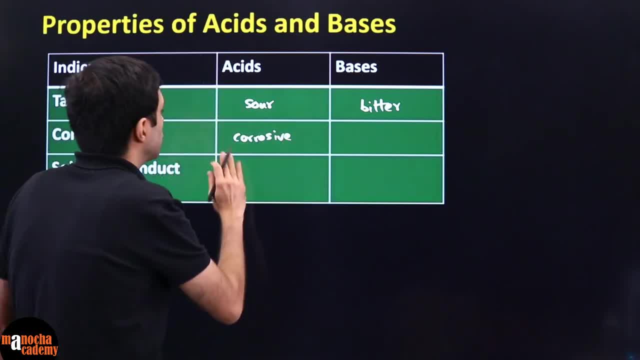 in nature what do you think about bases so if you ask this question are they corrosive the answer 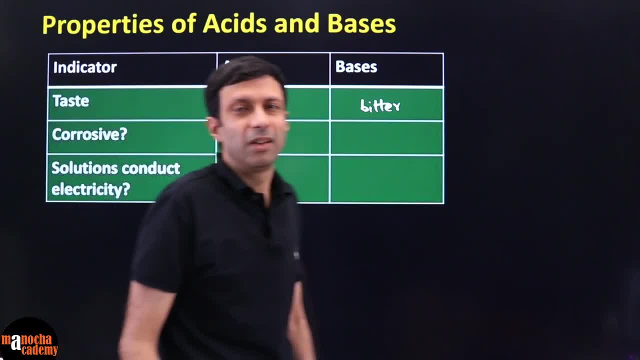 is yes what do you guys think about bases are they corrosive it seems like you know acids seem 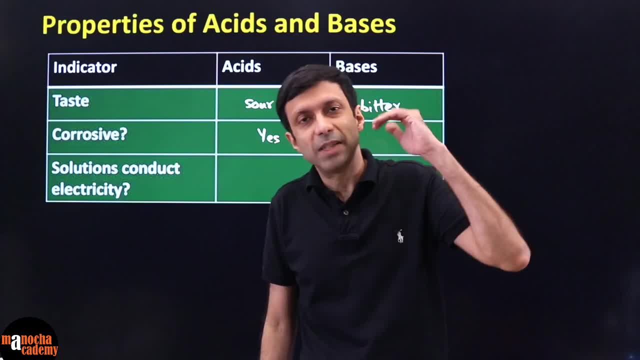 dangerous bases seem bases are mild no bases also like sodium hydroxide potassium hydroxide they can also be dangerous 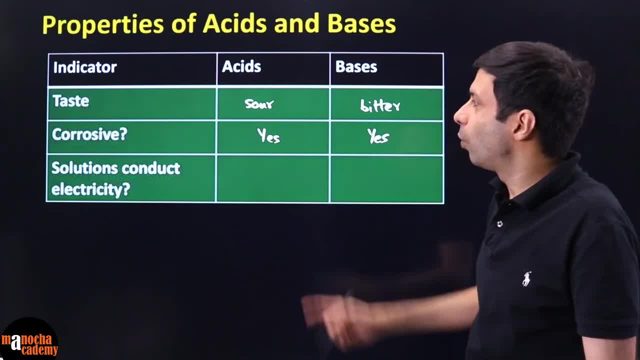 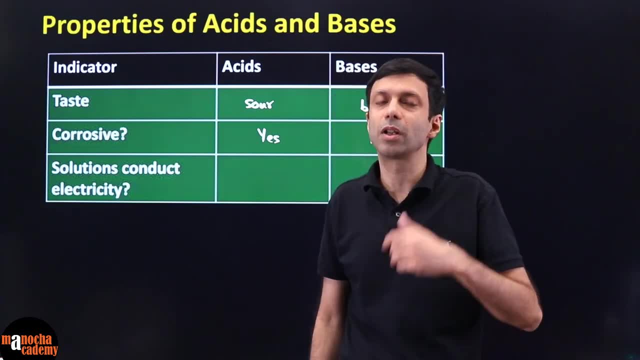 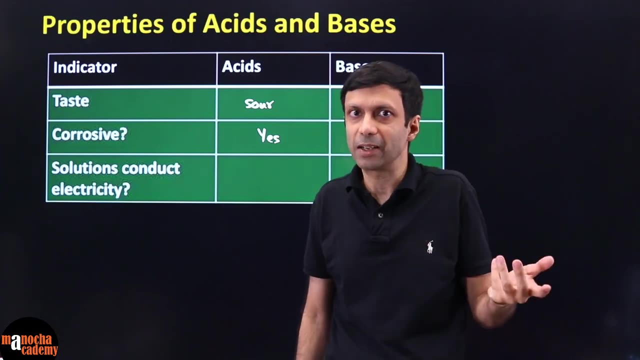 they are also highly corrosive in nature what about do acid and base solution conduct electricity you can do a simple experiment dissolve an acid in what in water or a base in water you know have this conductors use a battery and see if the bulb is glowing is it conducting electricity the answer is yes they are good conductors of electricity in solution 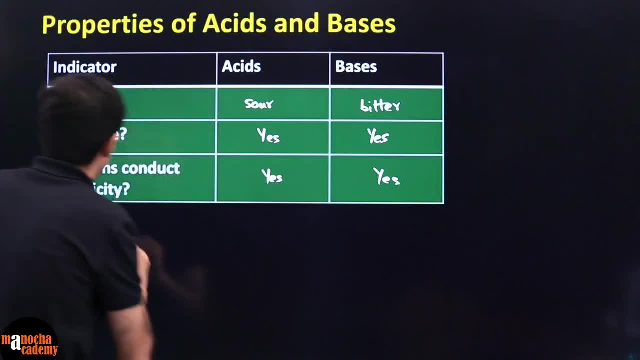 form and as a result they are known as because they are good conductors of electricity that is why we use acid and base solutes to conduct electricity. 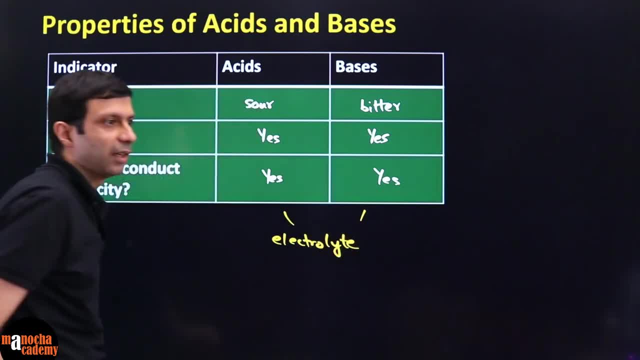 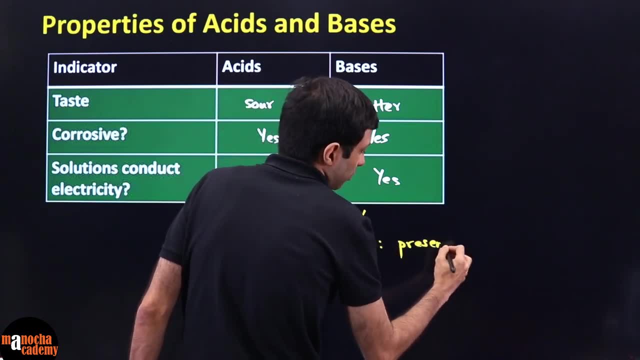 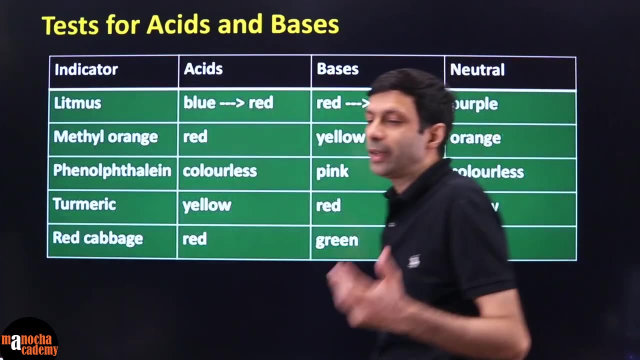 use the term electrolyte they conduct electricity why do they conduct electricity they are good electrolytes due to the presence of ions as we'll see because you need charged particles and what are the charged particles here not electrons they are basically ions in the solution now how do you test acid and 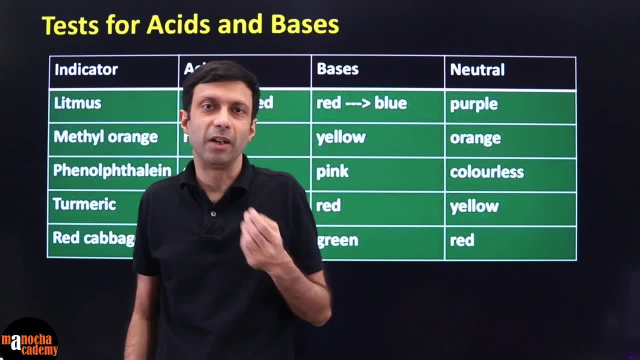 base you shouldn't always taste it because it is highly corrosive you know it can burn your tongue or very bad for your stomach right so the strong acid 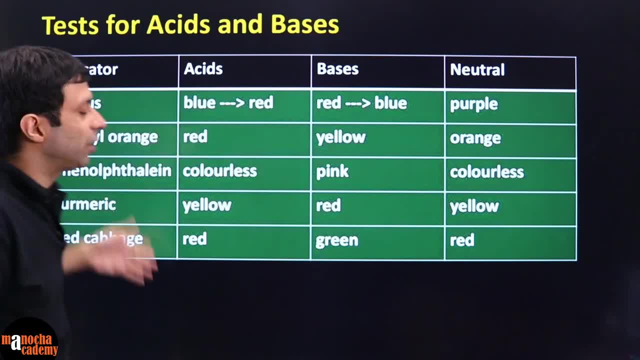 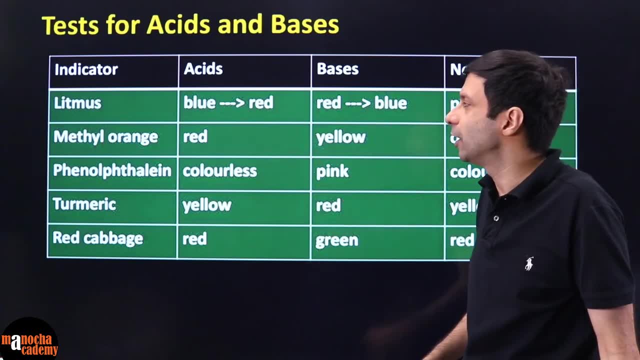 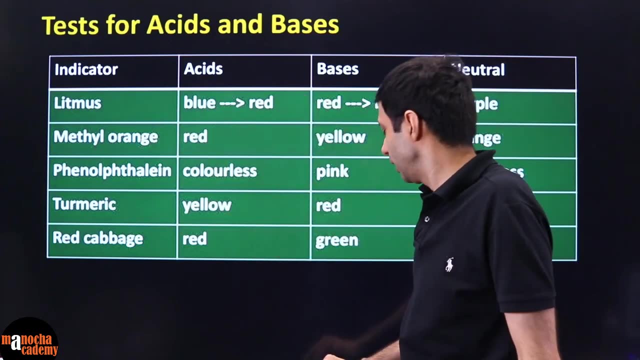 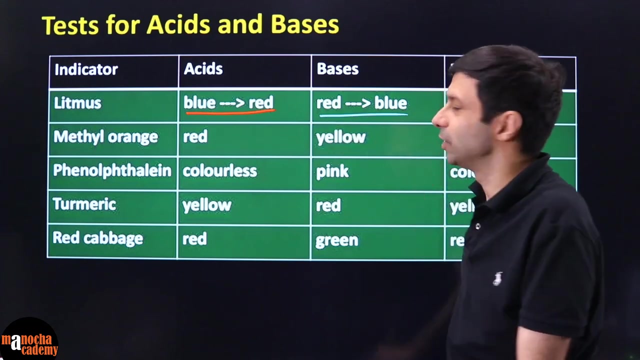 right mild are fine so how do you test them basically we use what is known as indicator test we use these materials we use these chemicals such as litmus methyl orange phenolphthalein turmeric and see what is the color change like for example litmus you should remember blue litmus turns red for acids right blue turns into red for bases red turns into blue it is exactly the opposite methyl orange methyl orange the neutral color and neutral color of litmus is purple okay 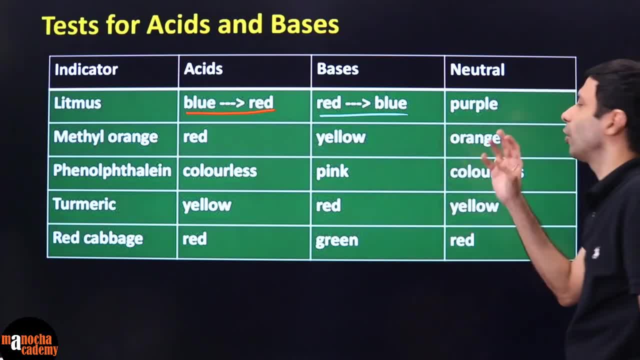 , but it turns red for acids blue for bases methyl orange as the name suggests 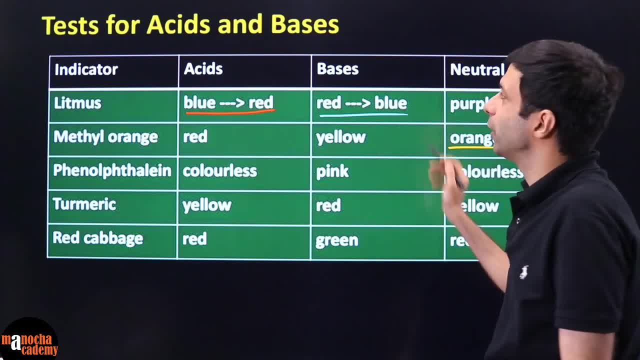 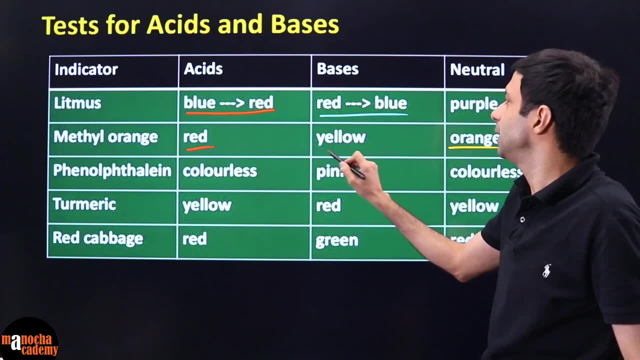 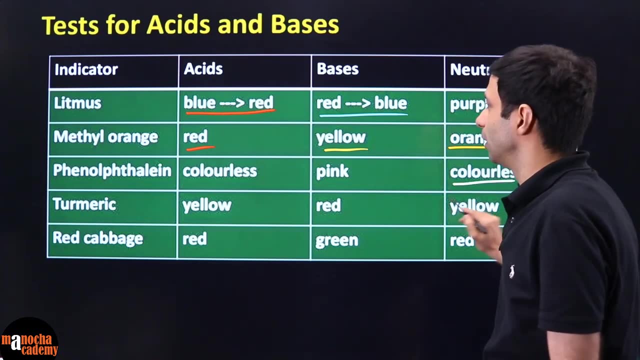 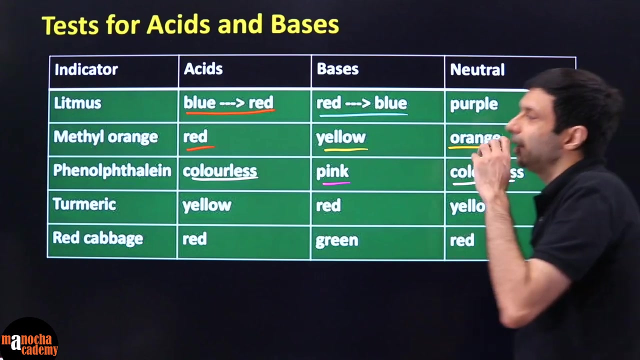 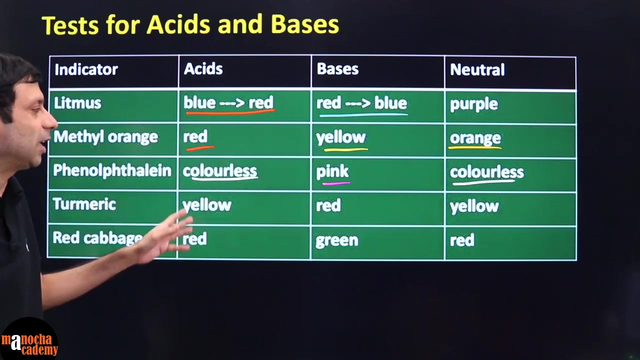 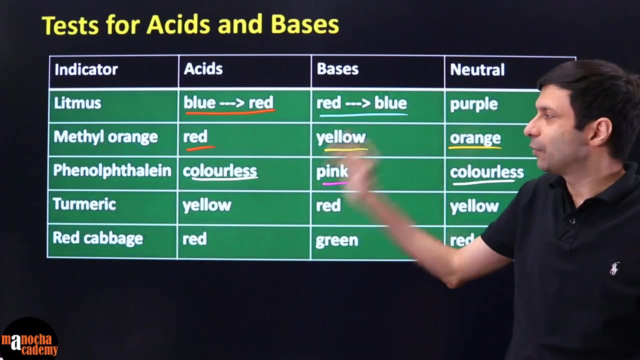 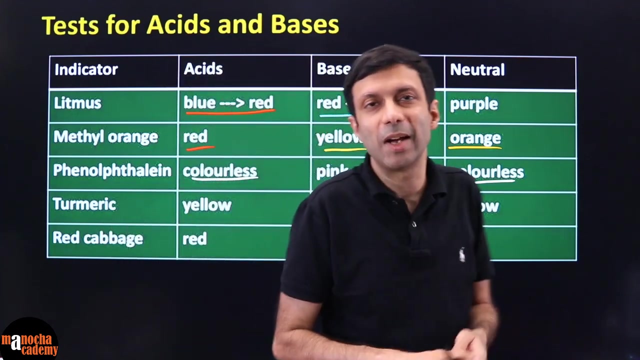 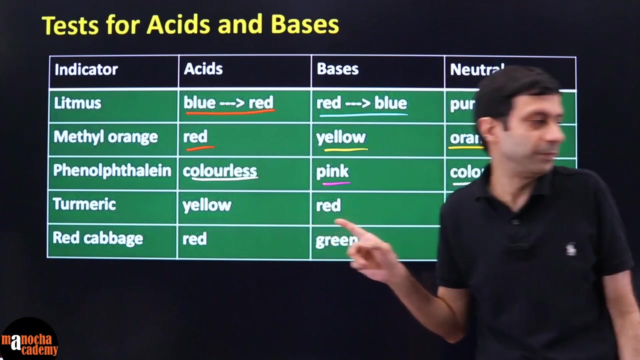 it is orange in color the neutral color is orange but when you add a acid to it acid turns red it makes it turn red just like litmus for the bases it turns yellow phenolphthalein phenolphthalein when it is neutral it is a colorless liquid in acid it remains colorless but when you add bases it becomes a nice pretty colored pink here so these are all indicators you know just like turmeric turmeric is called haldi in India right so haldi is the neutral colors yellow it remains yellow in acid but bases turn it red okay red cabbage red cabbage as the name suggests it will neutral color will be red it remains red in acid but turns to green for bases so these are this is a very important chart these are given in your books or I've given it here please do not take this lightly make sure you learn these colors because they ask very basic questions you know they may ask a certain substance you know changes terma to red what is it an acid base or neutral you should know from the color so those are color indicators you can also have olfactory indicator what is 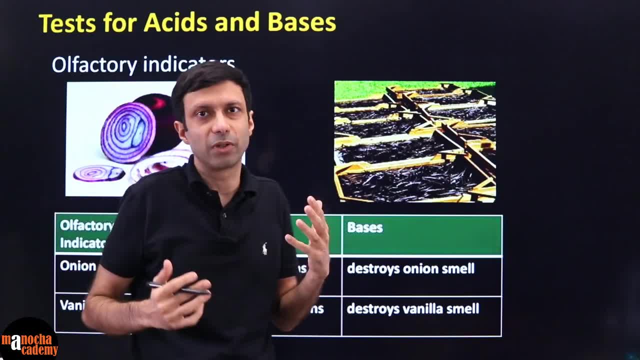 the meaning of the word olfactory we use olfactory senses for basically our nose 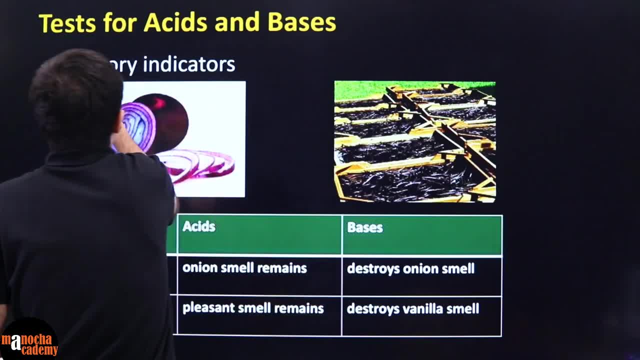 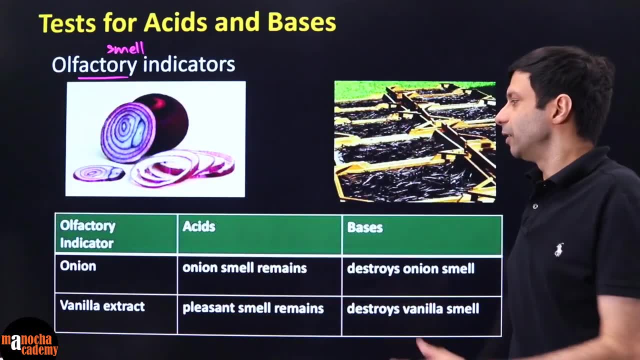 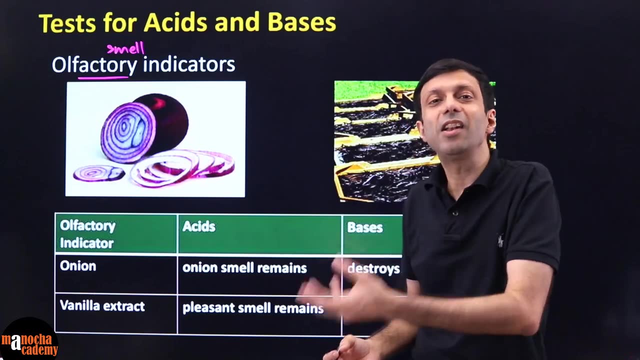 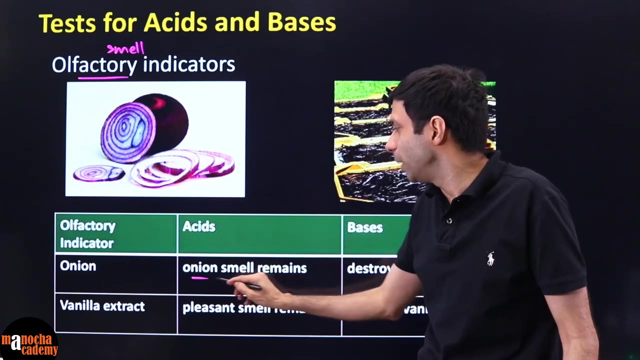 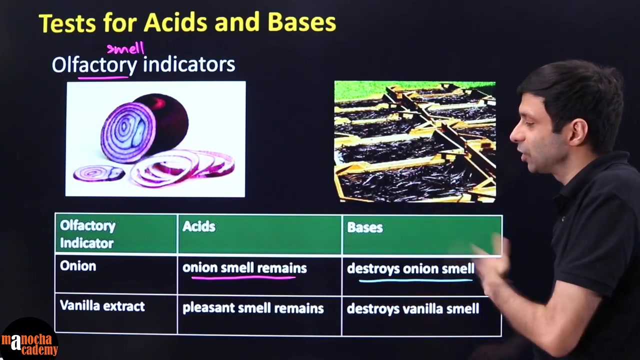 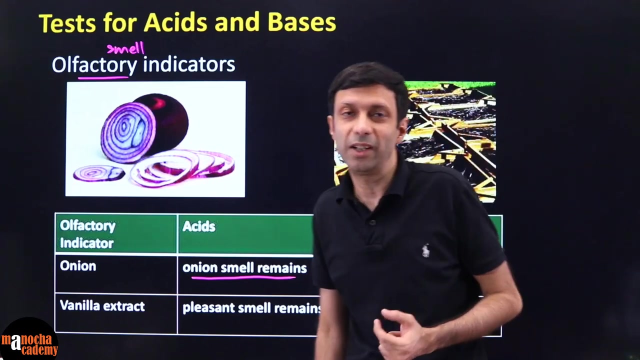 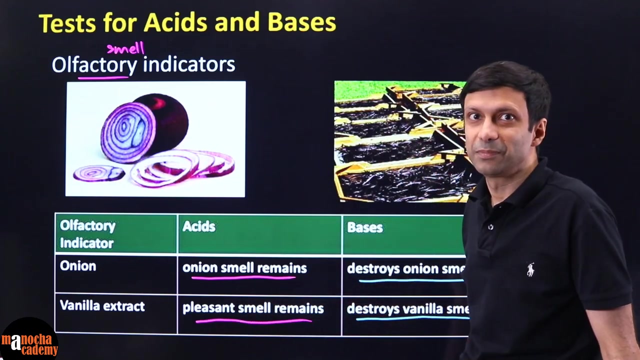 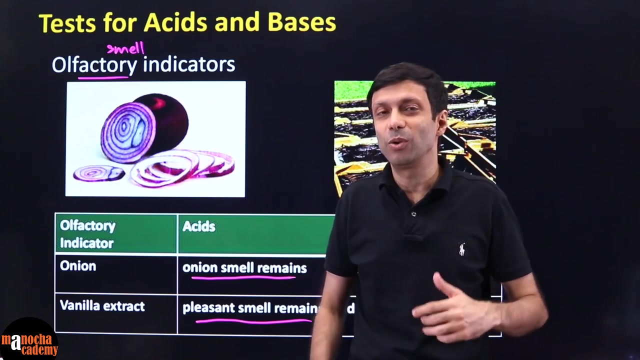 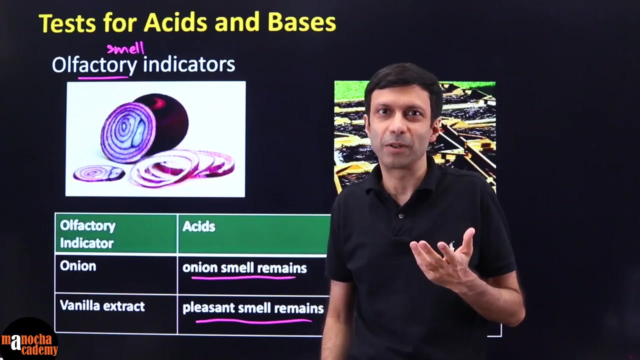 right so these are basically the smell indicators olfactory means the sense of we are using our nose smell for example if you take onion in acids the onion smell remains and this you can remain you can remember because you know in restaurants you have seen they put onion and vinegar you like that taste of onion dipped in vinegar because vinegar gives it a sour taste and here the onion smell remains it's there but what happens for bases bases basically destroy the onion smell so the smell of onion it just disappears goes away right similarly bases destroy the vanilla smell vanilla essence smell is very good right it has a very good smell but the for acid the pleasant smell remains in fact you know that vanilla essence reminds me of the vanilla essence that's how I detected I had kovat so during kovat time you know I I found that I'm not able to smell things even though my I'm able to I mean my nose is not blocked okay so for example I was not getting the smell of soap I thought that something's going wrong so I went to the refrigerator and took out that vanilla essence which they put in the cakes and you know I opened it and I 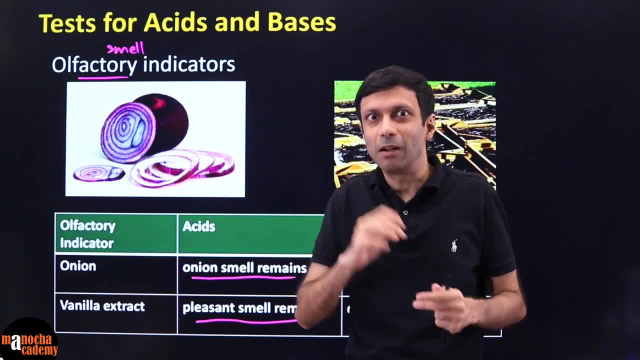 brought it near my nose so I'm using my olfactory senses there was no smell I was 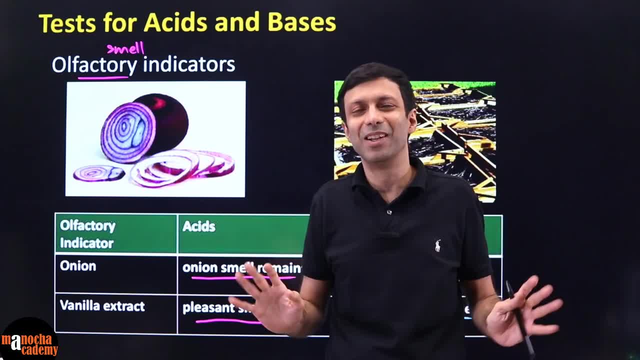 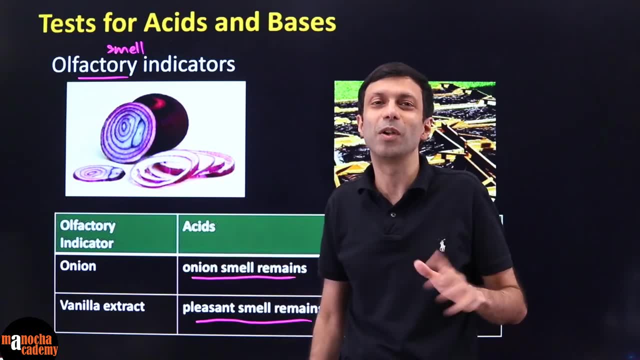 100% sure I had kovat and then with the kovat test you know it came out as kovat positive I knew the simple vanilla essence gave me that test that I had kovat because my nose was not blocked so this is what you know the pleasant smell 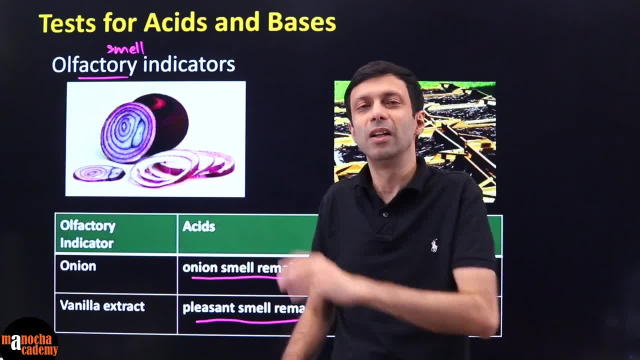 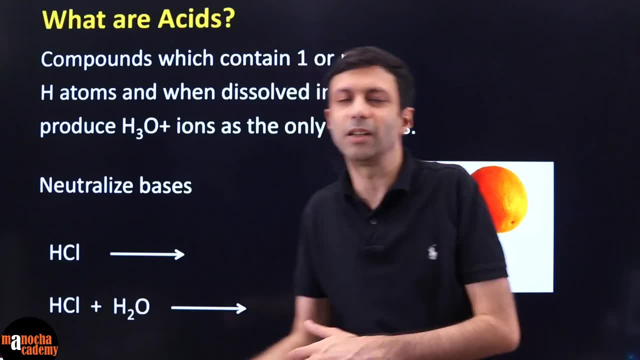 remains for acid but bases will destroy the vanilla if you add a base to it the vanilla smell will go away so now let's answer this question what are acids we know that acids are sour they're very corrosive you know they turn blue litmus 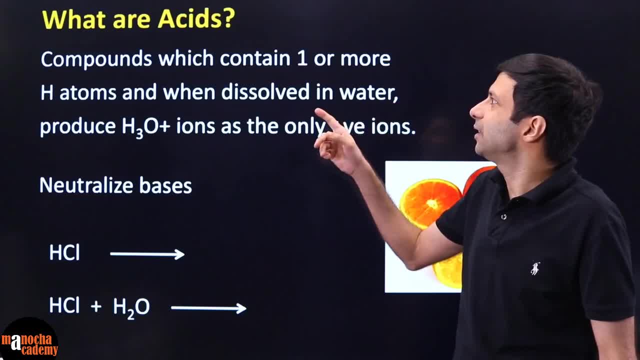 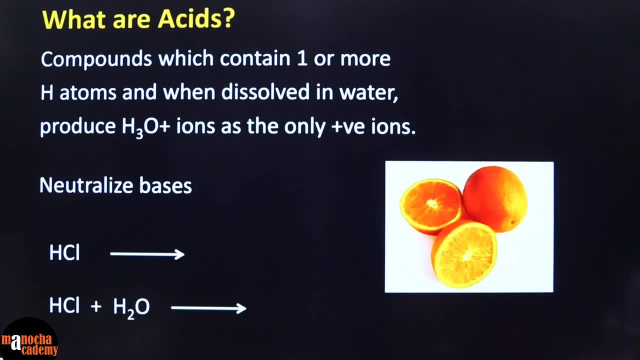 to red and all of that but basically how do we define acids acids are compounds which basically contain one or more hydrogen atoms okay so what are acids acids are basically they are compounds that contain one or more than 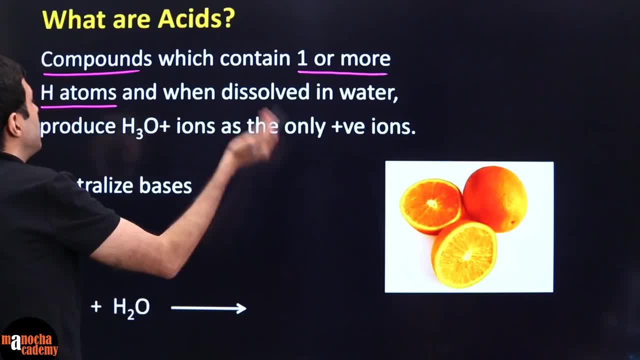 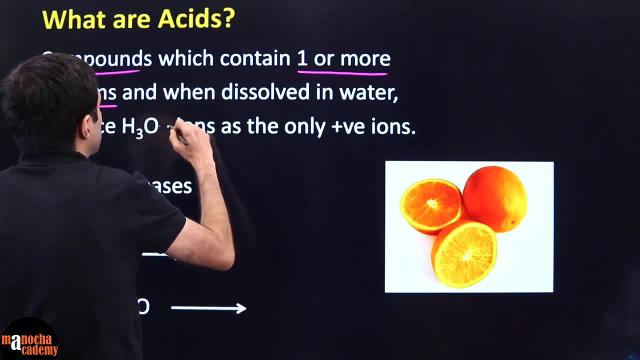 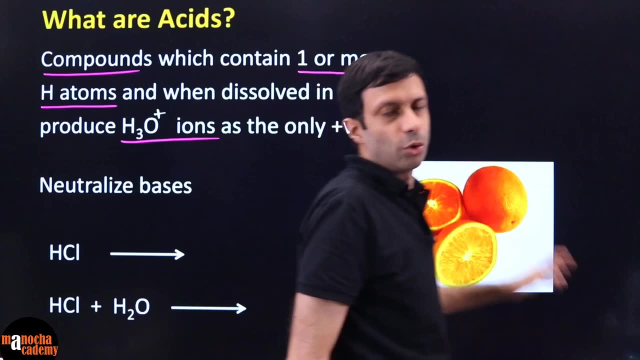 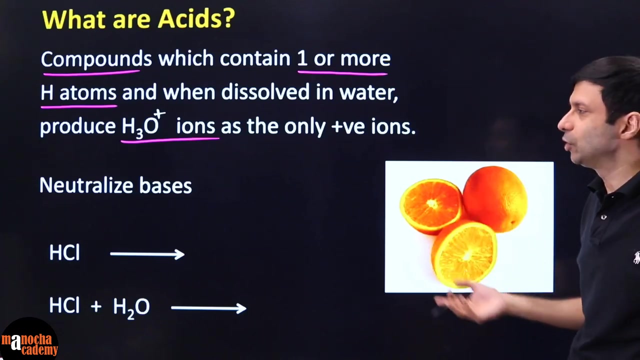 one hydrogen atom and when they are dissolved in water they end up producing this we should write it like this here h3o plus ions they end up producing this h3o plus ions as the only positive ions so it looks like a very fancy definition right so let's try to understand this for example if you dissolve lemon orange juice or lemon juice in water it's going to produce 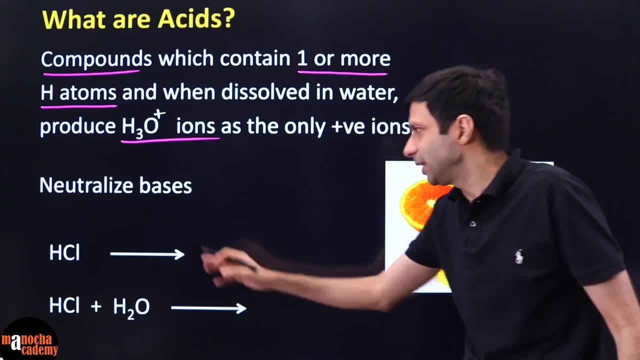 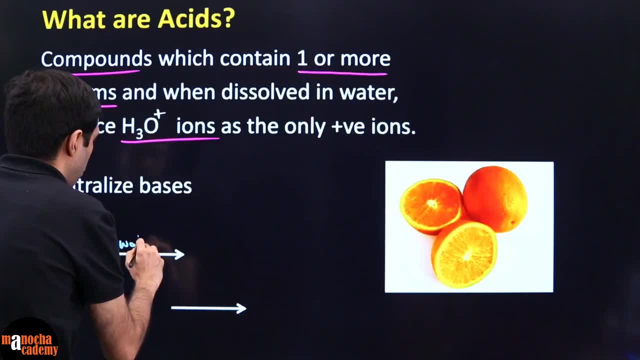 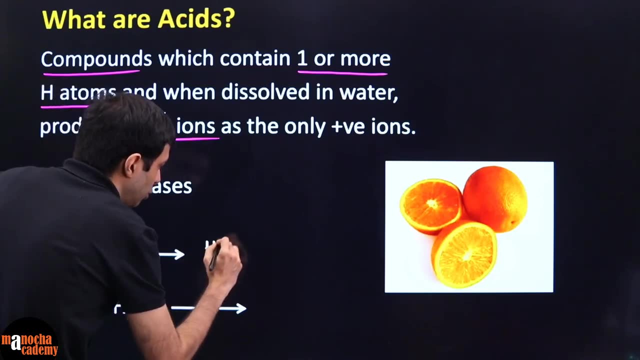 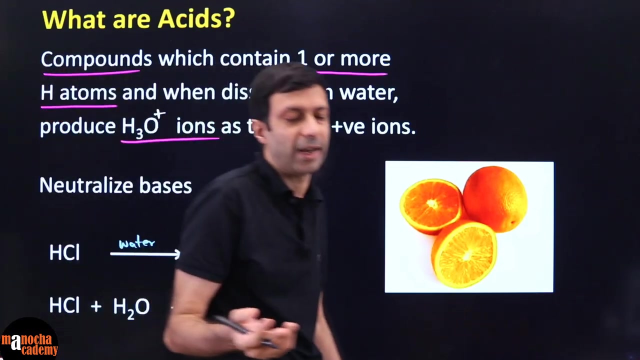 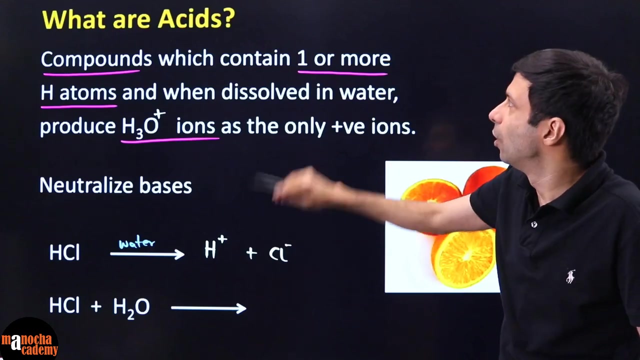 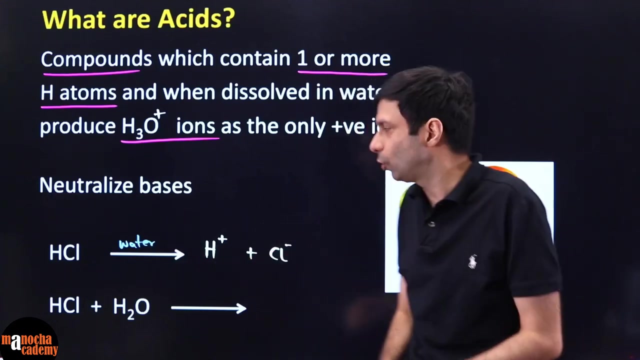 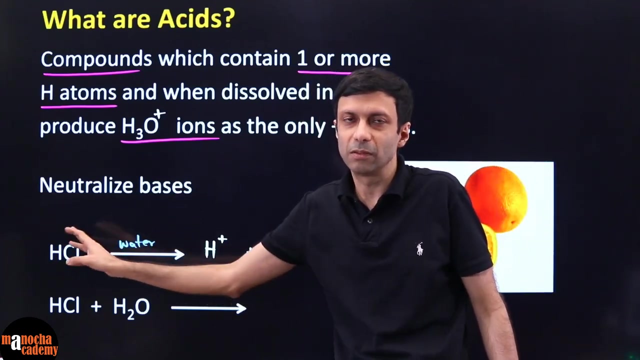 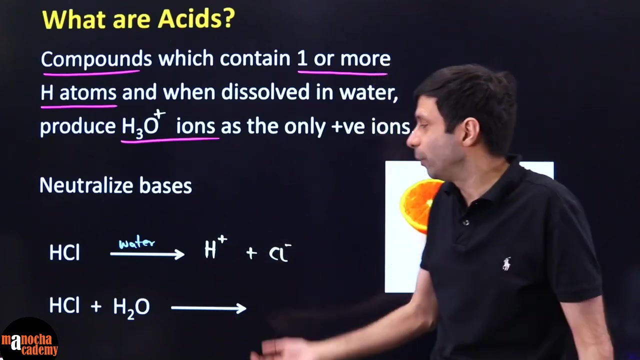 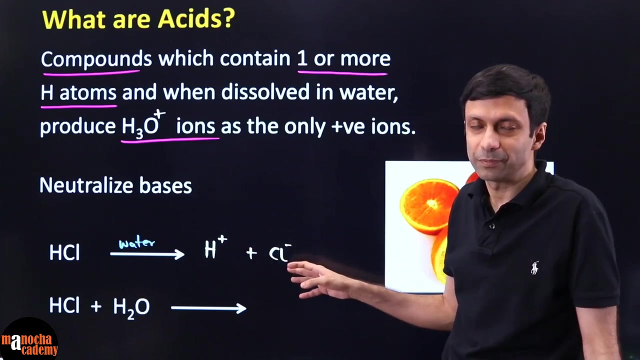 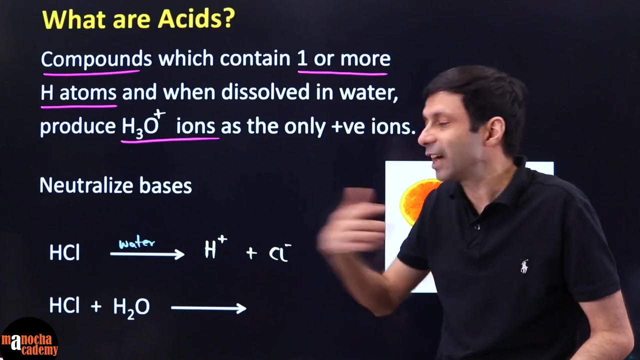 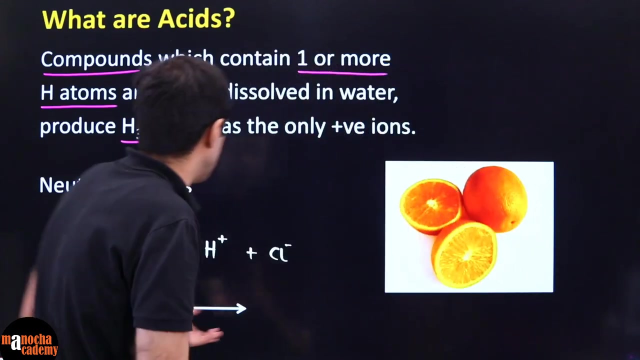 high this h3o plus ions or let's take the simple example of HCl so when I take you know water so when I take HCl with water what happens is HCl is hydrochloric acid water is going to break it down into a H plus and Cl minus ions. What is H plus? Hydrogen ions and Cl minus is called chloride ions. So, as you can see, based on the definition, hydrogen is a, acid is a compound which contains one or more hydrogen atom. Is that true? HCl is having one hydrogen atom. Now, when you dissolve it in water, it breaks down into H plus and Cl minus. Note the difference here. On the left hand side, it is a compound. Compounds are neutral like atoms, right? There is no plus minus I have written. But water is breaking it into charged particles, which are called ions. So, it breaks it into a positively charged particle H plus and Cl minus. Can you see that split is happening? H plus and Cl minus. Okay. Now, the interesting thing is that this H plus which is produced in water reacts with the water. So, H plus reacts with the water to produce hydronium ion, the H3O plus ion. So, what happens is that this H plus . 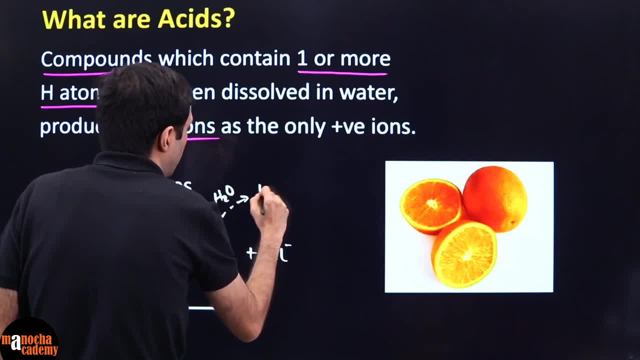 HCl goes and reacts with water to produce your H3O plus. So, this is the simplified equation. We can 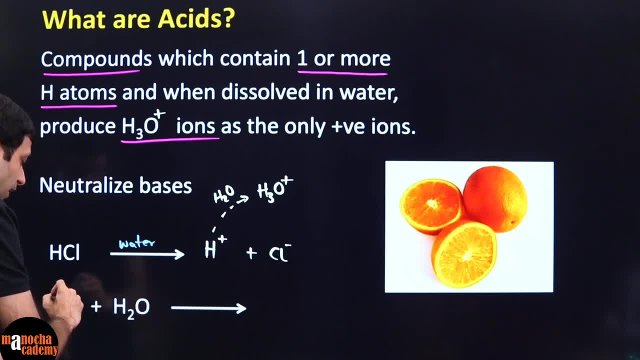 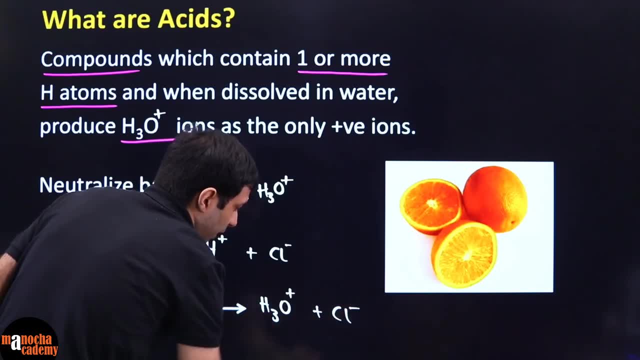 write it this way. HCl is reacting with water where it takes away the H plus ion. So, it is going to basically give me an, the reality is H3O plus plus Cl minus. Please note that this is the simplified 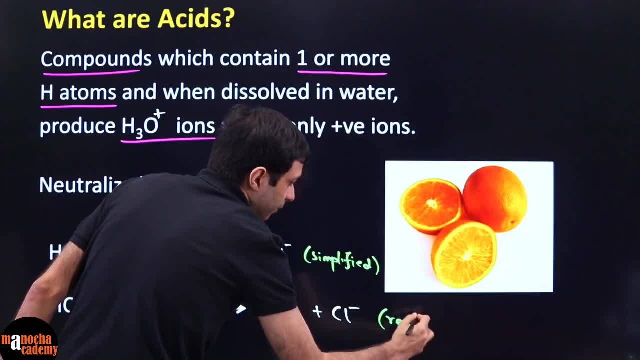 equation and this is what is really happening. This is the real correct equation. HCl reacts with water to produce H3O plus. 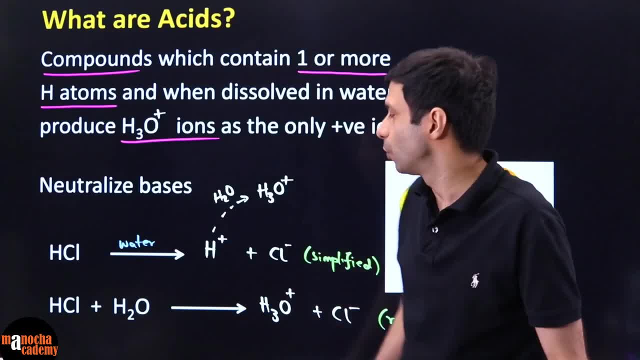 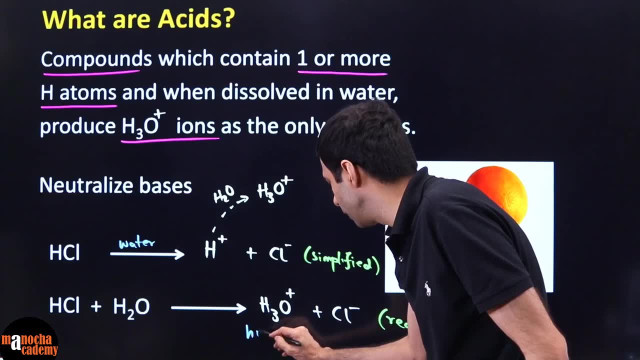 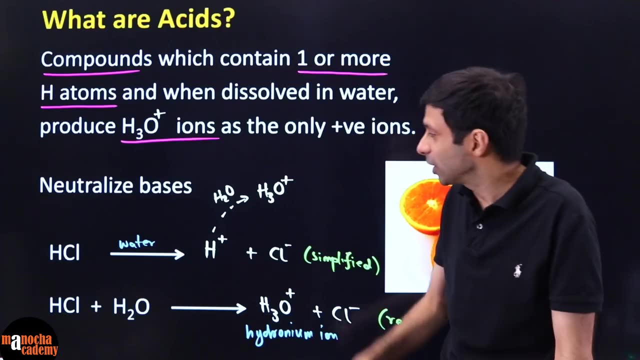 Hydronium ion and chloride ion. So, note the difference in words here. H plus is called hydrogen ion. This H3O plus, this is known as hydronium ion. And this is the indication that yes, this is an acid because the acid's property is it must produce hydrogen ions or what we, 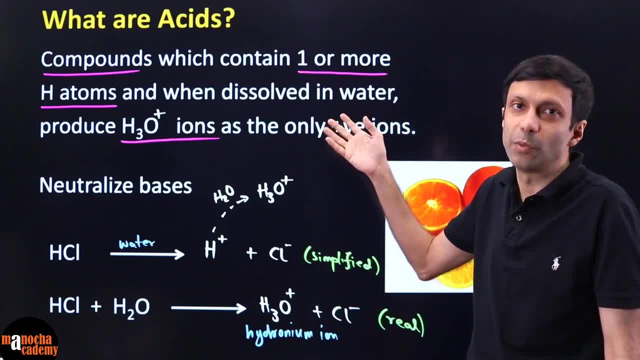 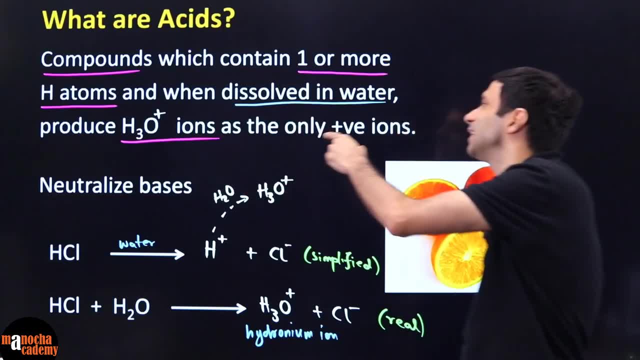 or more correctly, hydronium ions when they are dissolved in water. Because the best part is all acids are soluble in water. So, when you dissolve it in water, it produces hydronium, hydronium ions as the only positive ions. No other positive ion should be produced by the acid. 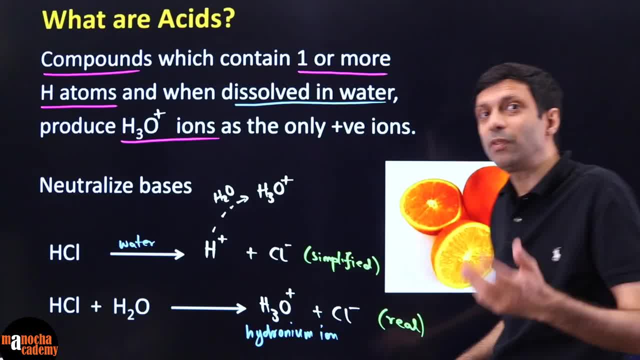 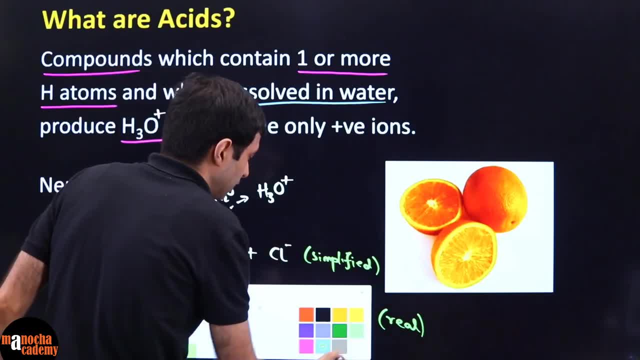 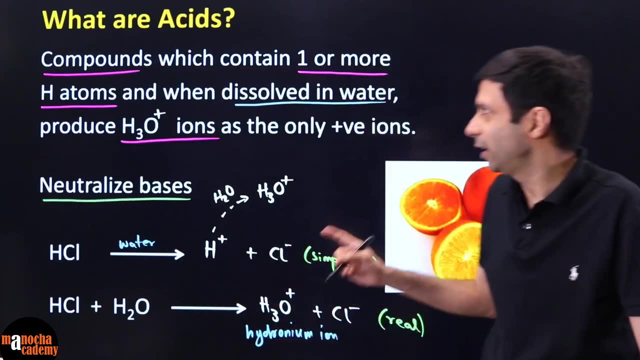 It only produces hydronium ions. And another way we know, acids basically neutralize bases. You might have heard of the famous reaction, acid plus base is salt and water. That is a neutralization reaction. So, another way to define acid is those guys who neutralize bases. Clear? How is the hydronium ion produced? Again, I am reminding you here, H plus, 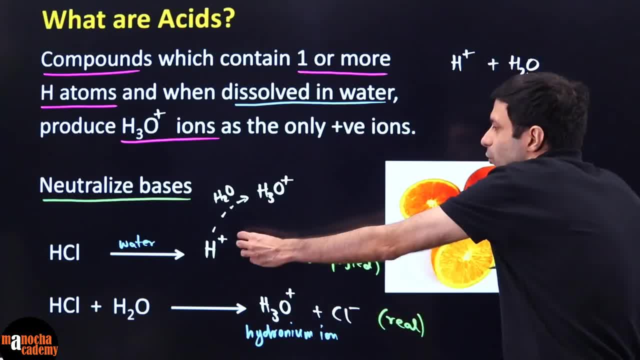 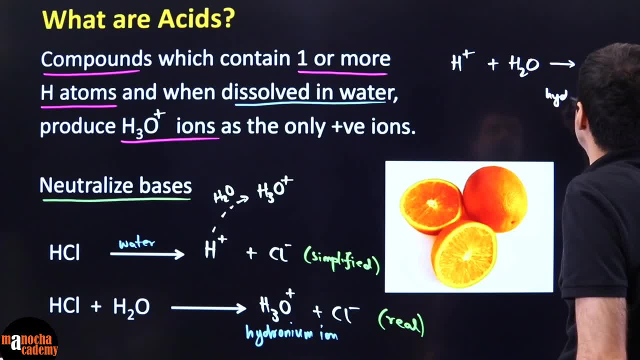 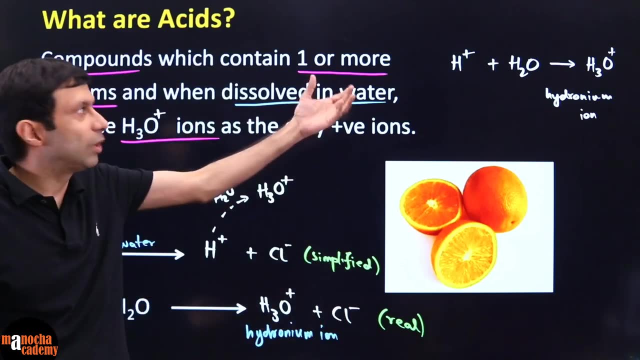 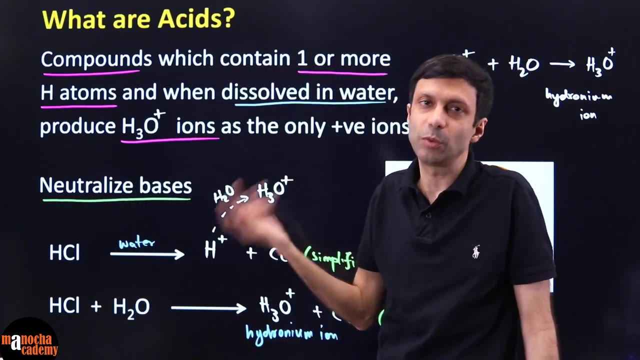 combines with H2O. So this H plus which was produced quickly combines with the water to give you your H3O plus. This is the important guy for the acid, hydronium. So basically when you're feeling that sour taste, right, or the corrosive nature, it is due to the presence of hydronium ions. That is what makes the acid. And where does the hydronium ion come from? Because acid must have atoms of hydrogen. So if you show me a compound like carbon dioxide, which is not having 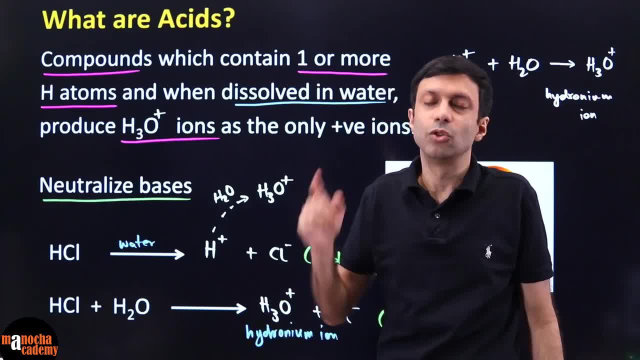 any hydrogen in it, is it an acid? No, right. So every compound, every acid must have hydrogen. 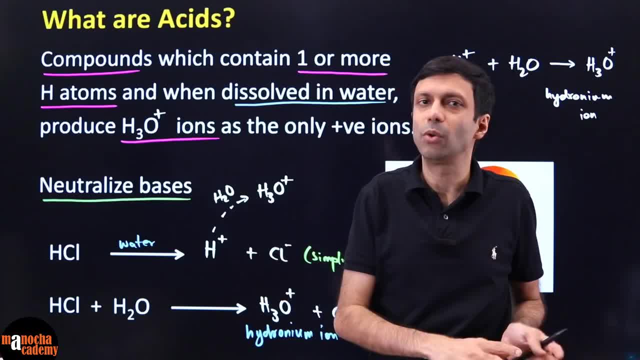 But water is not an acid. It is H2O. So it's not necessary. If you have hydrogen, it will be an acid. But acid must have hydrogen. Clear? So we discussed the basic thing about what are acids. 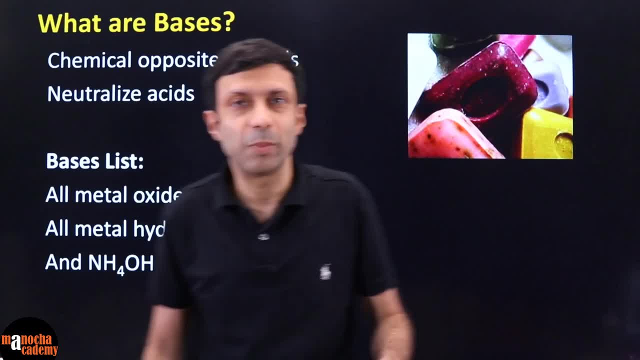 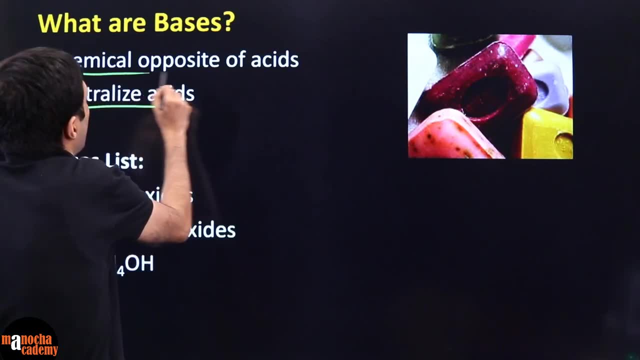 Now let's talk about what are bases. Just like we said, acid neutralized bases. Similarly, bases neutralize acid. Or one very easy way to define them is they neutralize acid. So they are the chemical opposite of acid. 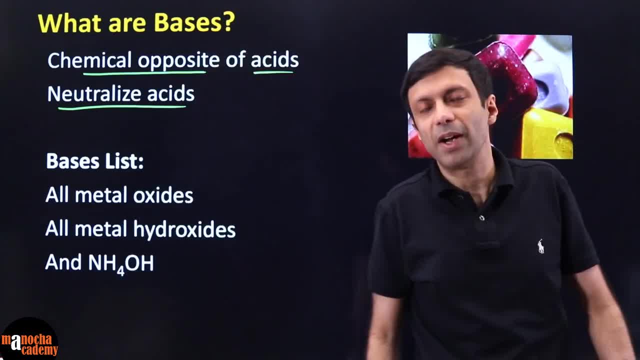 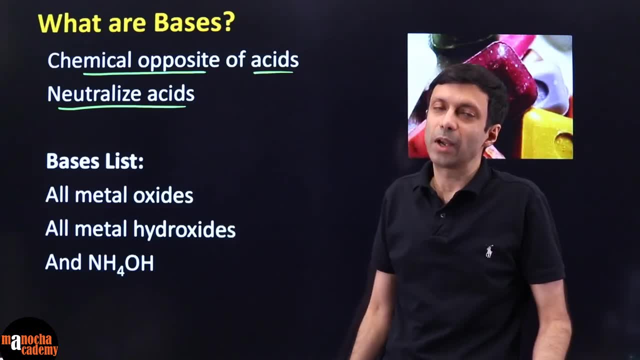 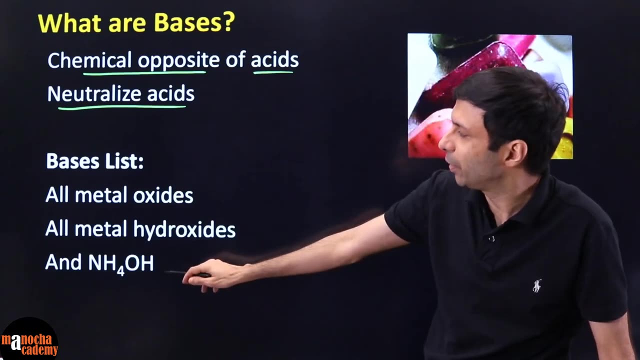 OK. Because bases are not that easy to define. We can't say, oh, it produces hydroxide ion only. No. Because bases, the list is a little more. What are bases? They are basically metal oxides, metal hydroxides, and ammonium hydroxide. Can you tell me why I've written this separately? Why I'm not just simply saying metal oxide, metal hydroxide? Why have I written NH4OH, which is ammonium 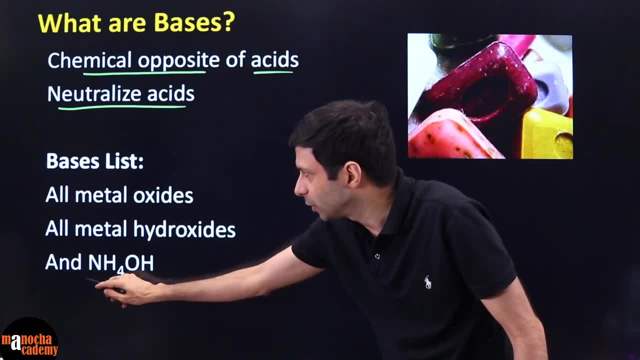 hydroxide, separately? Because NH4 is a special ion. It is an exception. 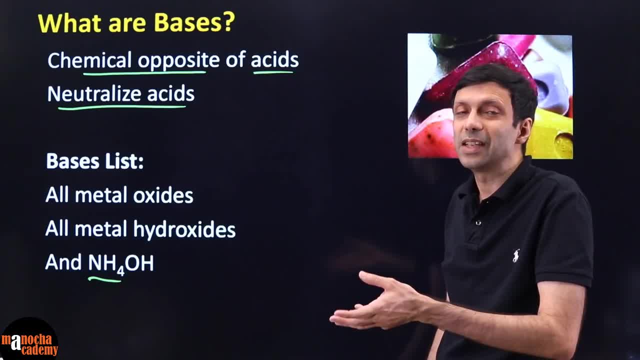 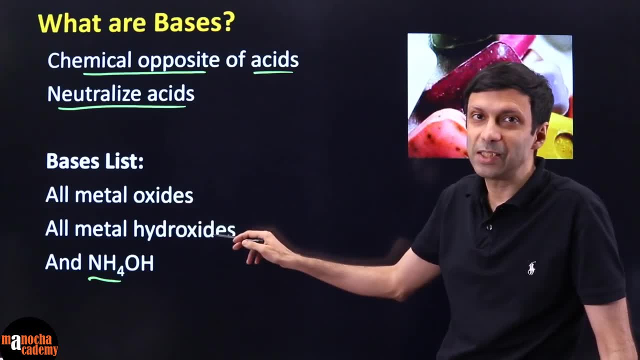 It is made of non-metals. But this ammonium hydroxide behaves as a base. So that is why we always have to remind that all metal hydroxides are bases. But ammonium hydroxide also is a base. So these are the three 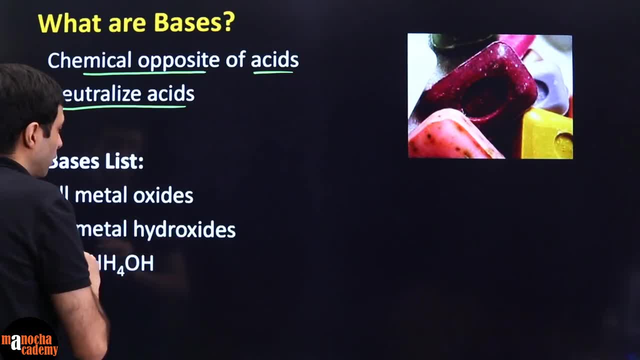 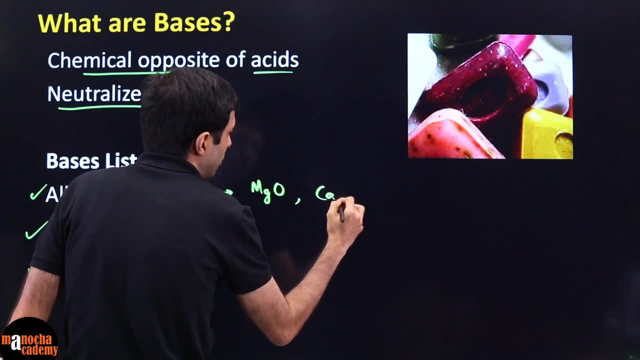 important bases you can remember. Metal oxides, metal hydroxides, ammonium hydroxide. What are some examples? So metal oxide, you can take an example. Magnesium oxide, that's going to be a base. Calcium oxide, copper oxide. Right? 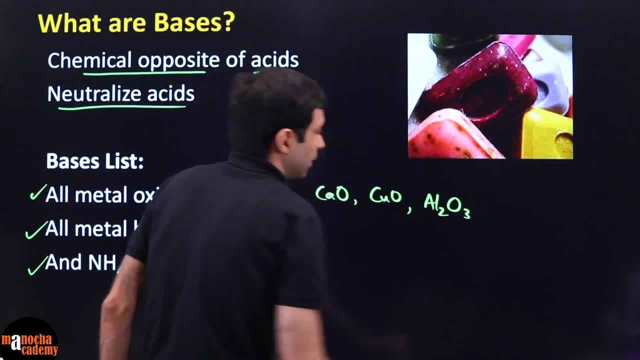 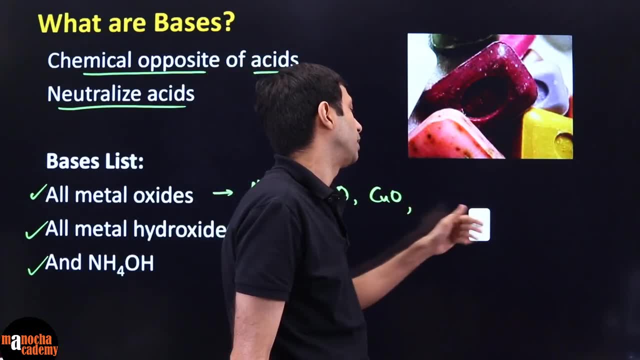 All these guys are bases. Aluminium oxide. These can all act as bases, right? What about metal hydroxide? Aluminium maybe because it comes under amphoteric, so for now I'll remove it, right? But iron 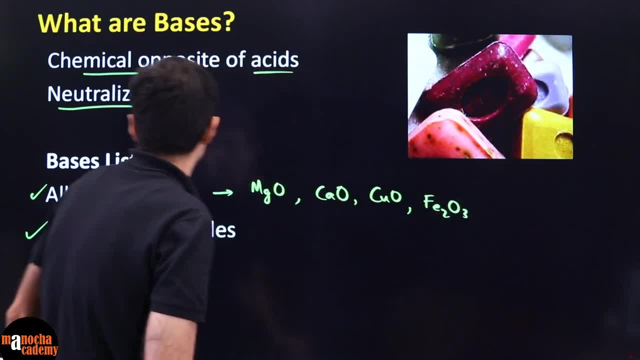 oxide, ferric oxide, this is a base. What about metal hydroxides? Sodium hydroxide, potassium 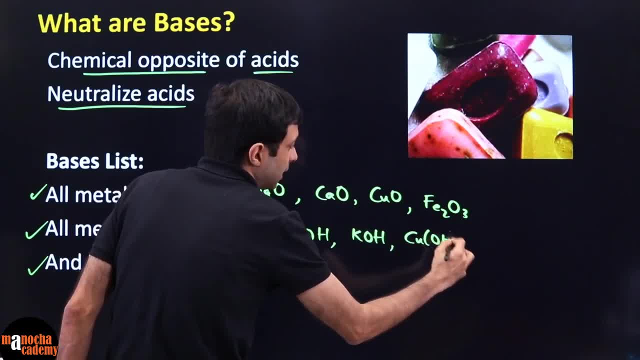 hydroxide, copper hydroxide. All these guys are bases. All metal hydroxides, of course in chemistry there are some, one or two 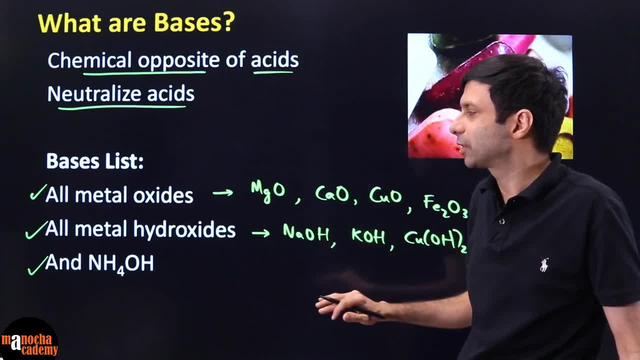 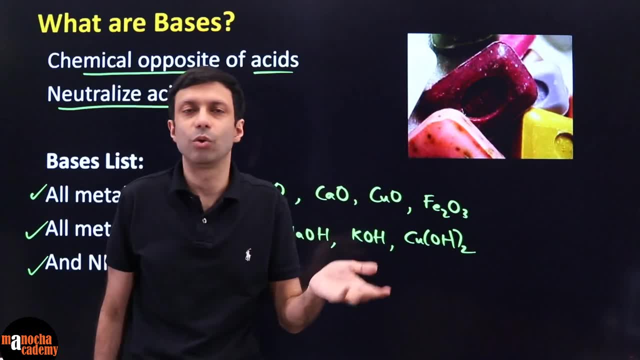 different trap reader have exceptions here and there. But them general rule all metal oxides, all metal hydroxides and ammonium hydroxide these are all bases. Where are bases used? Acid you know, it's there 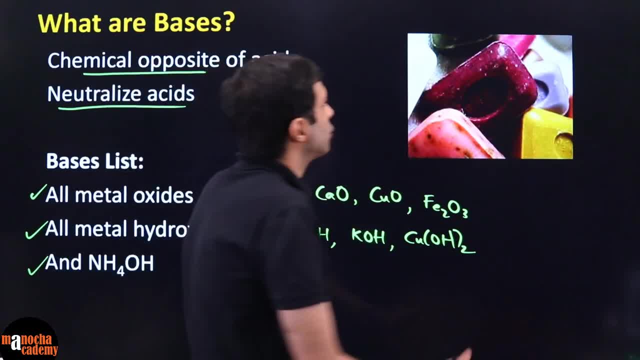 in the juice, it's used in tomato sauce and all. In this picture you can see these are soap bars. 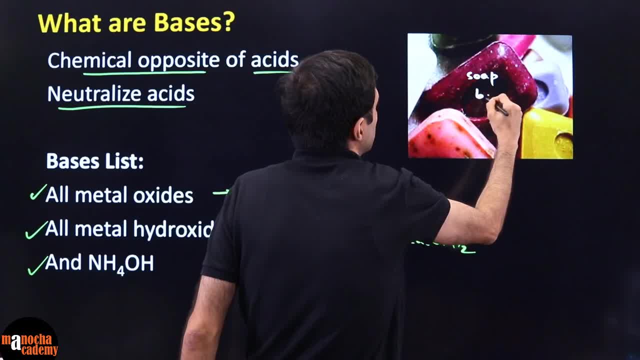 These are basically soap bars, bars of soap. So bases are used in soaps. So tomorrow when you're taking bath, remind me? These are only base you see, these areду Ji YHa of soap, okay?空気. So baseball, rubbish. So are does.wolves, snacks if you feel. They're nécessaire. So tomato sauce. 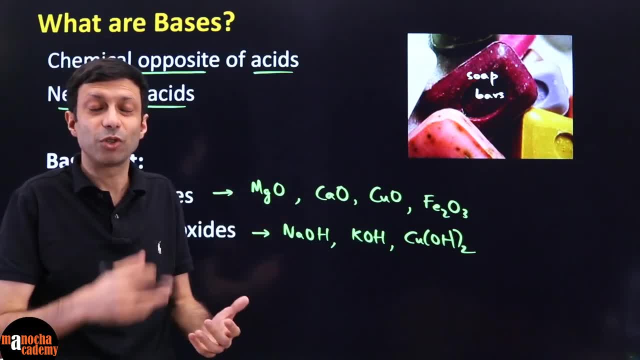 so tomorrow when you're taking bath remind you yourself you're using a base so they basically 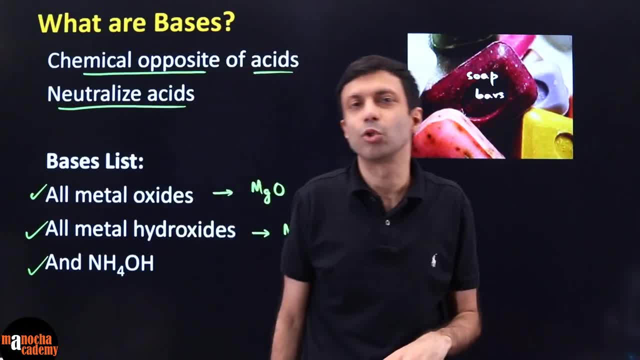 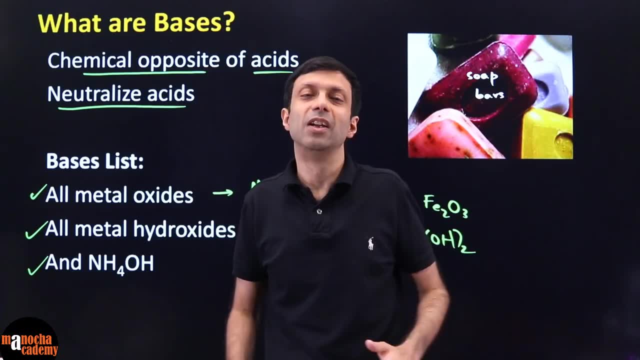 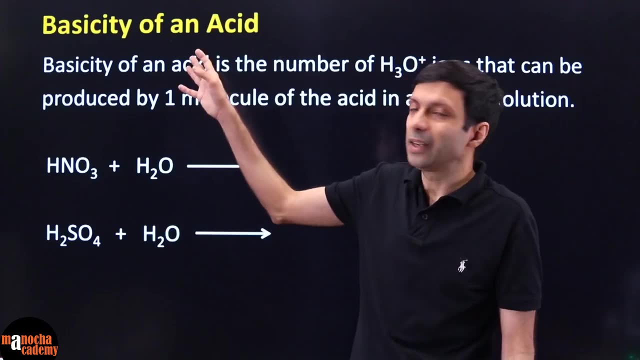 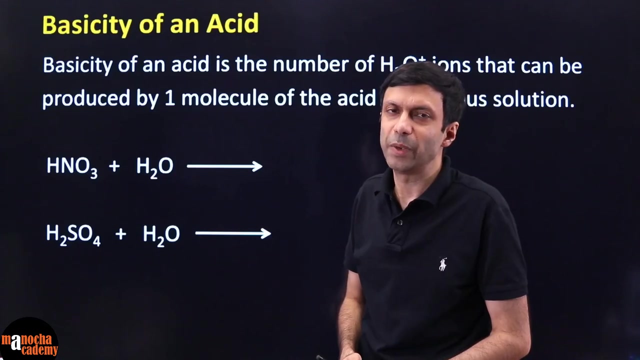 contain soap bars typically contains uh they are made from sodium hydroxide so they contain sodium stearate uh your liquid soap typically contains potassium hydroxide okay so soaps are made from bases so this is one very interesting thing uh sometimes you'll see this is not given clearly in your book in some of the books they have this thing so i'm going to teach this concept basicity of an acid what does this mean it sounds very funny right normally we should say acidity of an acid what is basicity of an acid look at the definition carefully 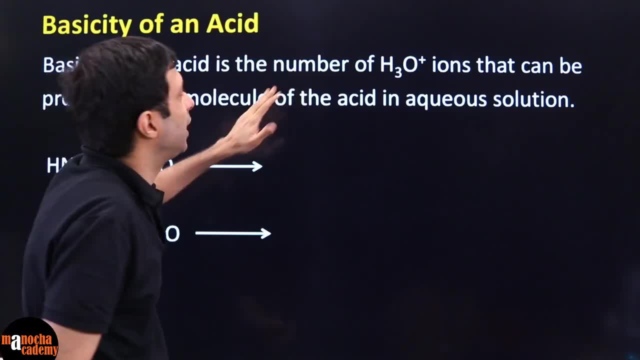 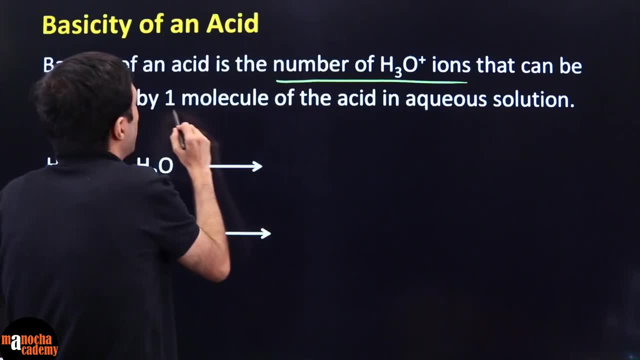 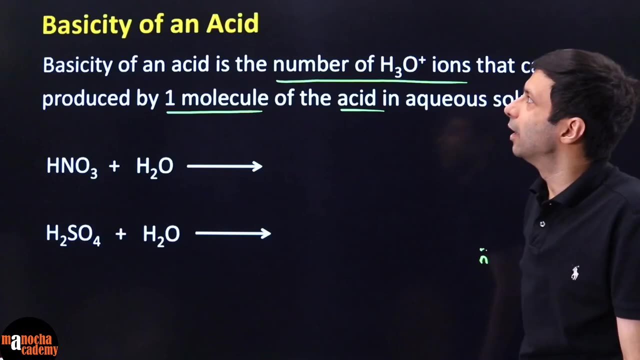 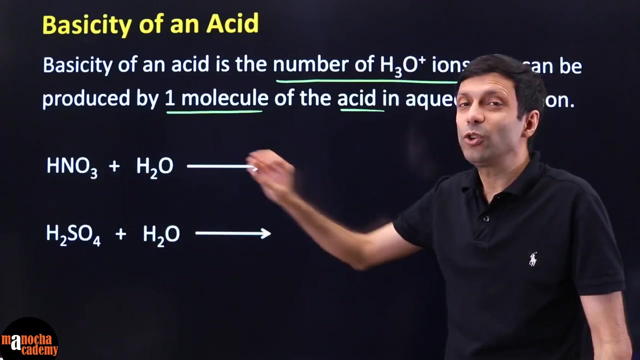 basicity of an acid is it's a very simple definition it is the number of hydronium ions the number of hydronium ions that can be produced by one molecule of the acid of course in aqua solution you'll dissolve it in water okay so the number of hydronium ions that can be produced by one molecule of the acid when dissolved in water so let's understand this uh with an example who is this guy hno3 you might have heard of him he is basically nitric acid when you take nitric acid and you dissolve it in water can you guys predict what's going to happen here so very similar 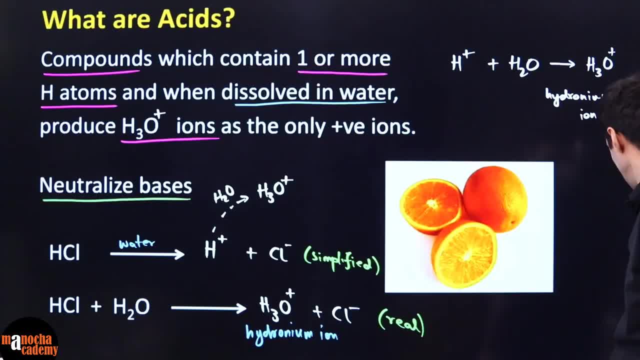 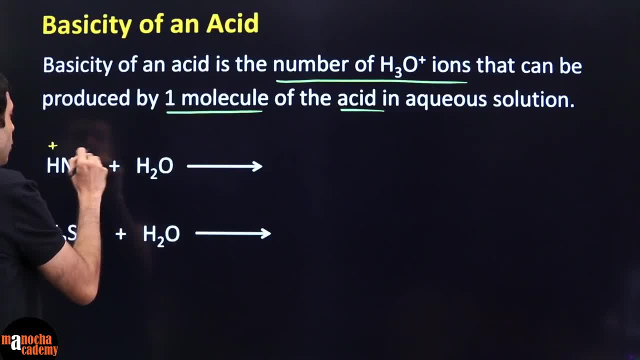 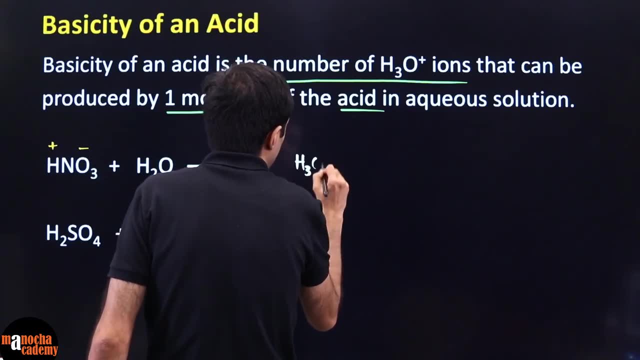 to the equation we did earlier hcl plus water you know it breaks down so how will nitric acid break down you can divide it like this this is basically nitric acid is h plus and no3 minus so this h plus and combined with it so it's going to form very simple you can predict this reaction h3o plus 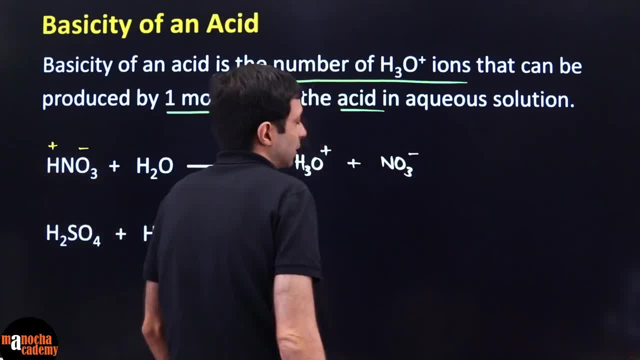 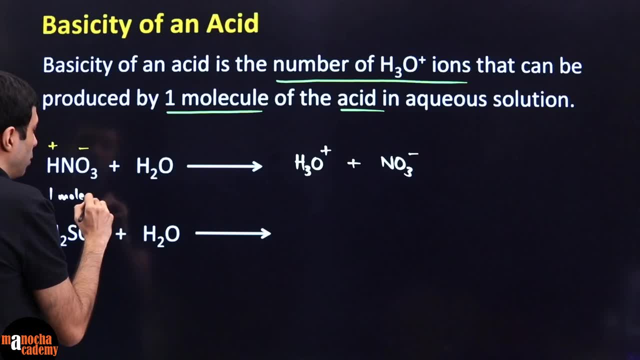 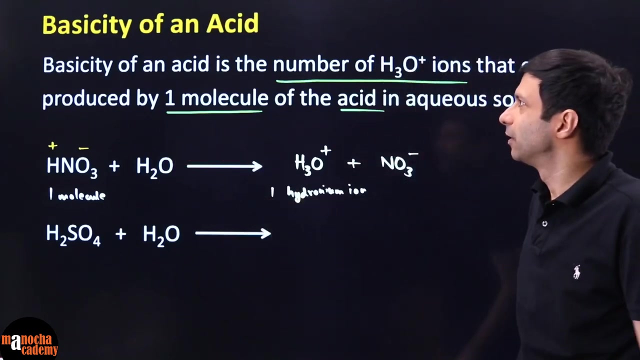 plus no3 minus right all you need to do is break those guys so if you look here carefully one molecule of nitric acid hno3 the name is nitric acid one molecule of nitric acid is producing how many hydronium ions and see equation is balanced you guys can check the number of atoms see it is producing one hydronium ion so what is the basicity of nitric acid according to the definition if one molecule produces one hydronium ion we can say basicity of nitric acid is basically one base it has basicity of one it's like a 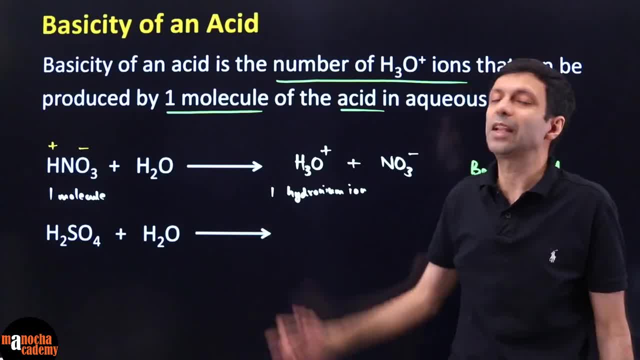 it's like this valency number right it has a power of one what about sulfuric acid 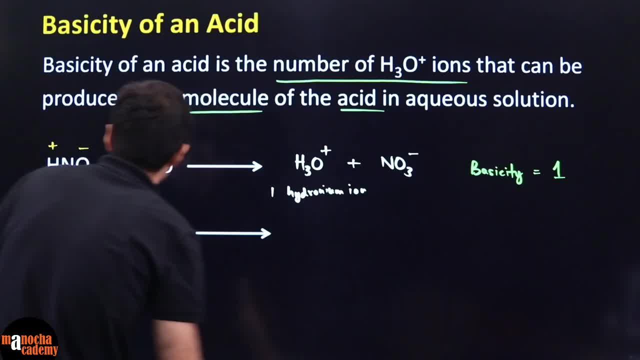 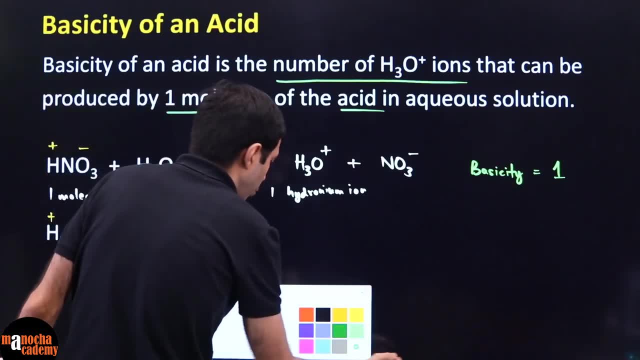 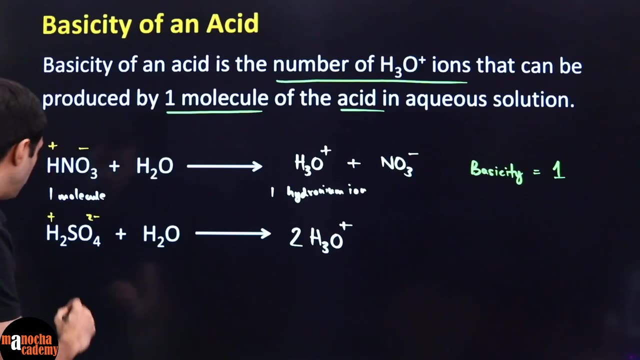 if you take one molecule of sulfuric acid what will happen again you break down sulfuric acid there are two h plus over here and there is sulfate is two minus two h pluses will combine there is lots of water so what will happen is they will form two hydronium ions why because this is getting split up like this it is producing two h pluses and a sulfate ion these two h pluses go to water and produce two hydronium molecule uh ions and 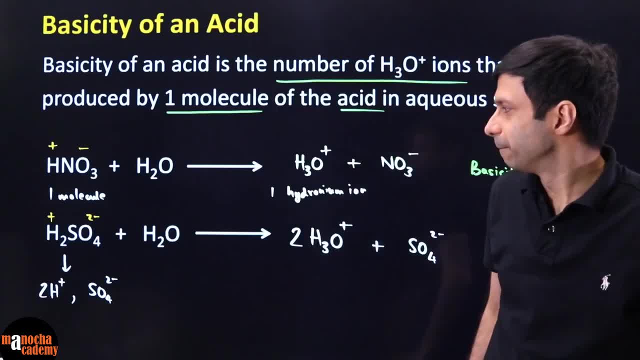 the sulfate ion this is all happening in water do you agree so what can you see here one molecule one molecule of sulfuric acid 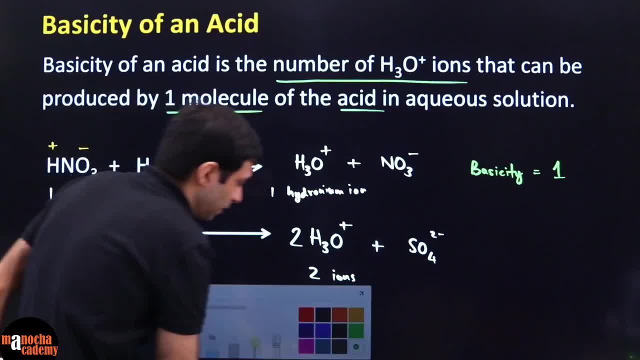 is producing two ions of hydronium so what is its basicity the basicity should be two 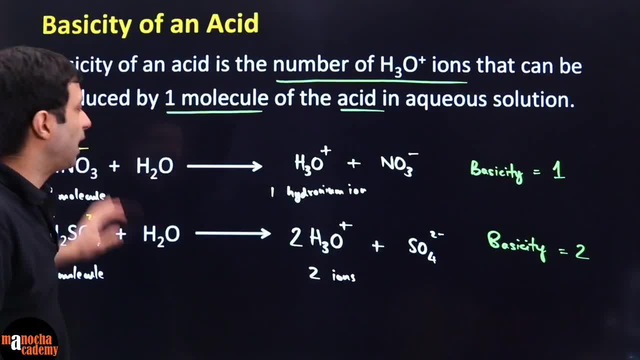 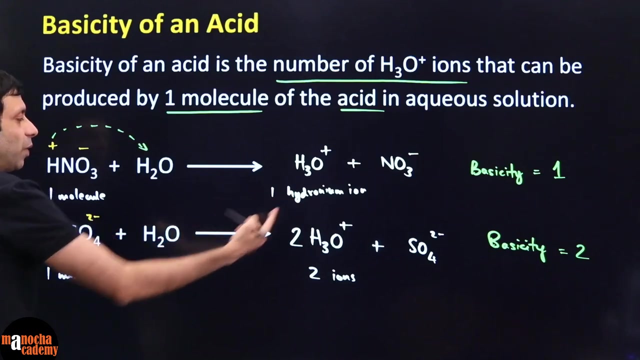 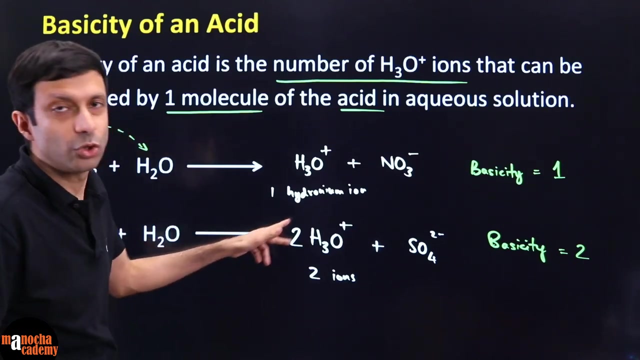 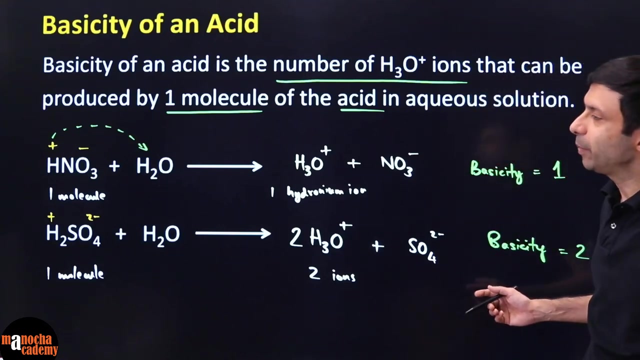 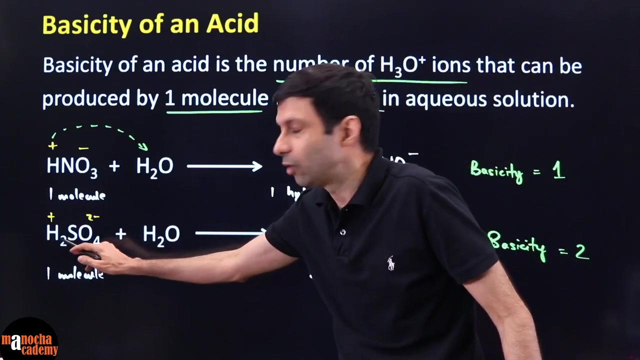 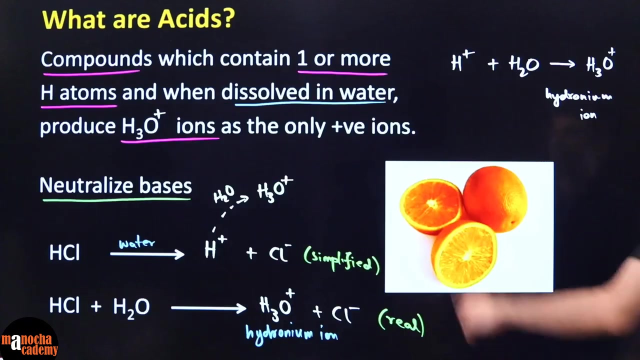 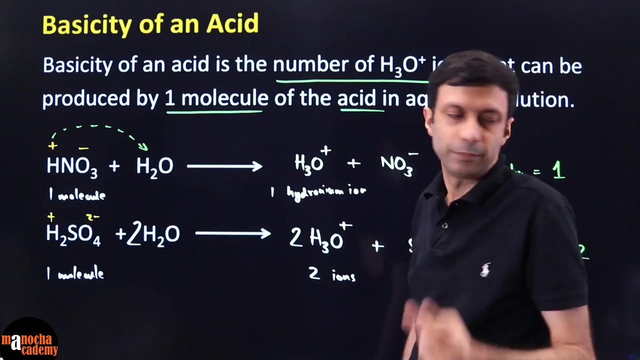 basically what we are trying to show in this equation is that when you take the acid and you dissolve it in water how many hydronium ions is it producing one simple technique here is you break it down into its ions so nitric acid produces one h plus ion and a nitrate ion that h plus ion goes and combines with the water to produce one hydronium ion so see one molecule of nitric acid produces one hydronium so we say its basicity or its power is one in sulfuric acid it does not produce an h2 it produces two h plus ions there are two h pluses produced those two h pluses go to water and produce two hydronium ions right plus a sulfate ion so do you guys agree that the basicity here is going to be two and please check is your equation balanced so you should make sure your equation is balanced it is actually not balanced because if you need two hydrogen ions you need two water molecules to produce those two hydroniums because remember we saw how is hydronium produced by combination of h plus and water that's it so basicity of sulfuric acid is two so in the second equation what is happening is 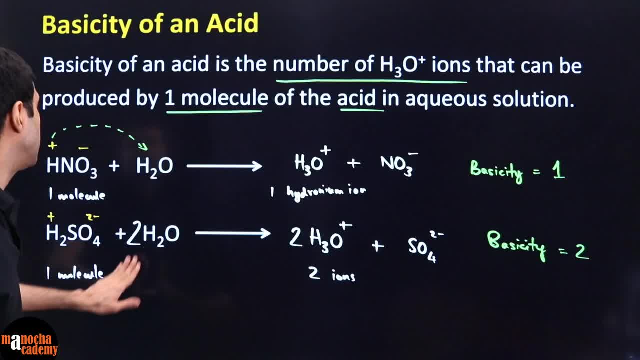 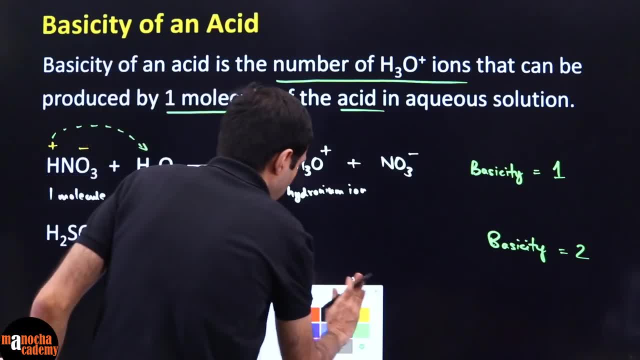 that these two h pluses are going so if you didn't understand it this way another way is you can break it down you can go step by step so you can say that hey one of the h 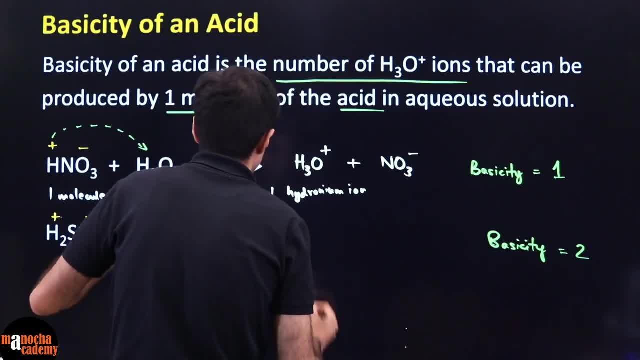 plus so you can break it down into two steps you can say first the h plus combined with the water 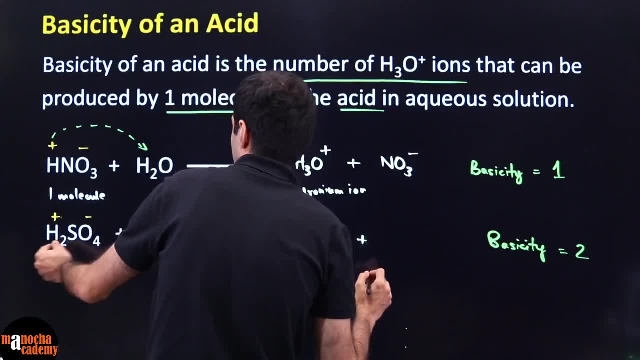 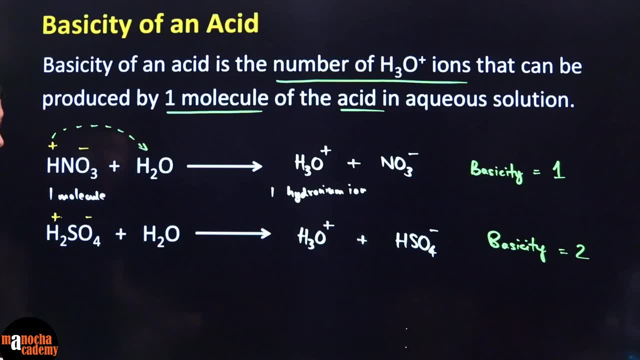 to produce an h3o plus and what is the remaining part hso4 bisulfate is a negative ion hso4 minus okay this is the first step then what happens in the second step hso4 is still there 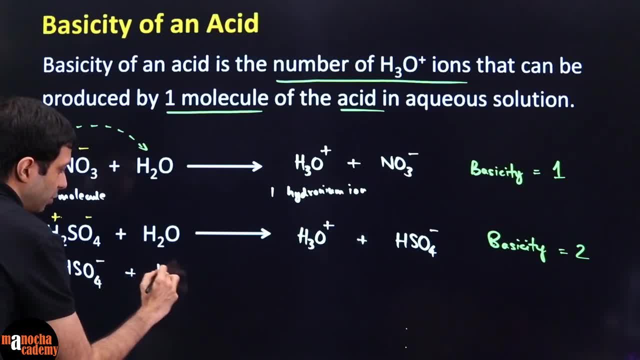 there is still some hydrogen there in the bisulfate or hydrogen sulfate it will combine with water again you split this up this the plus here 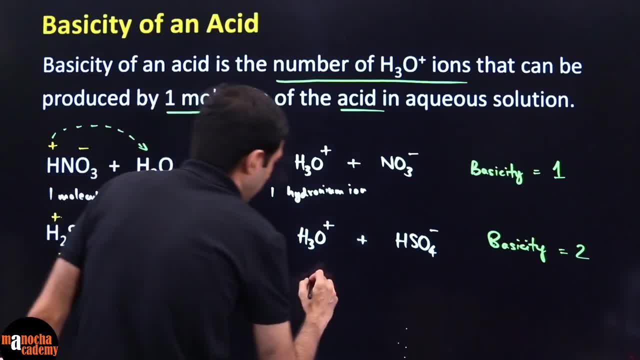 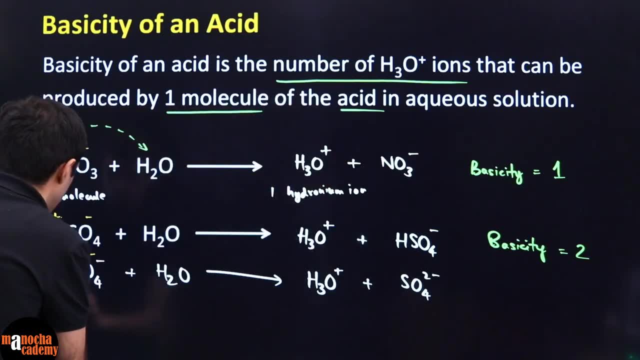 and this is 2 minus so what will we get as a result of that h plus will combine with water to give h3o plus and sulfate two minus so overall what happened is what the equation i showed you 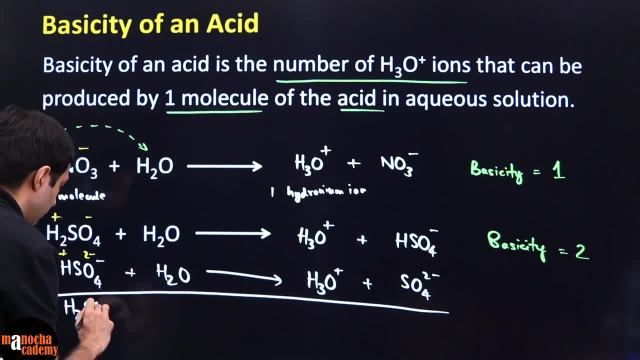 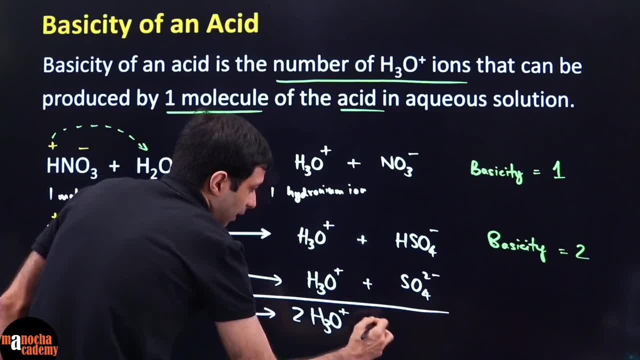 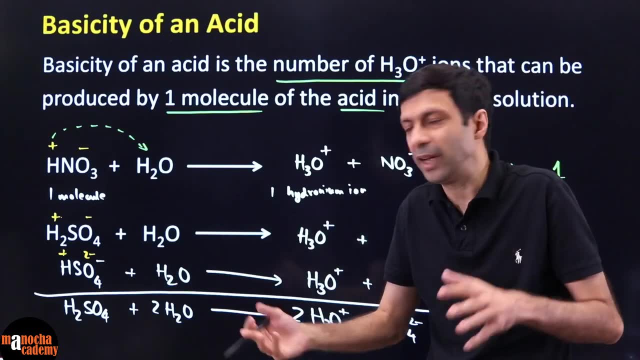 that basically what is happening h2so4 is reacting with two water molecules to produce two hydronium ions and a sulfate molecule so basically those two hydrogen atoms in H2SO4 are breaking away combining with two molecules of water to produce two hydronium 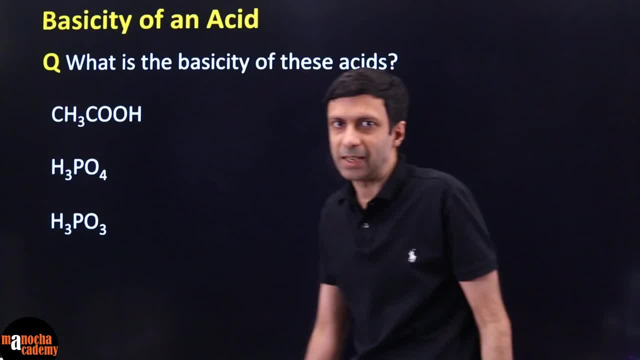 ions. So now can you guys tell me what is the basicity of these acids? One of course we can do you know we can sit and write those equations and try to predict but is there a easier way? 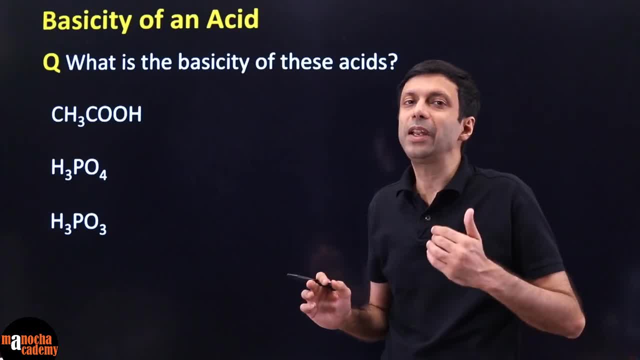 The main trick is you need to see how many replaceable hydrogens are there or basically 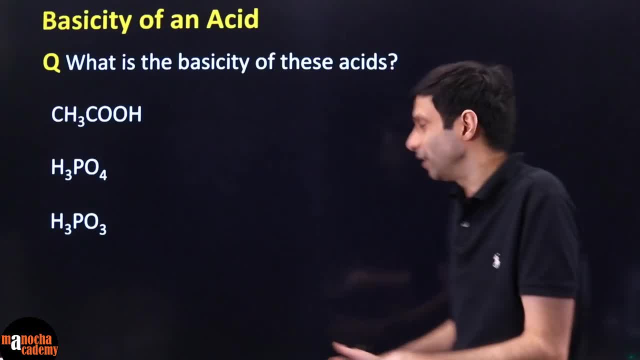 how many hydrogens are ready to leave the acid that is the basicity because if you look here in nitric acid one hydrogen was ready to leave the acid combined with water to produce hydronium 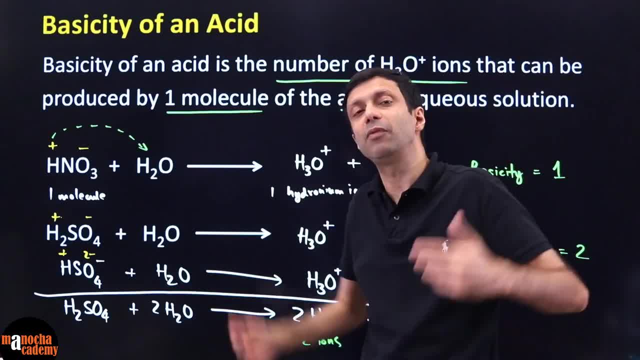 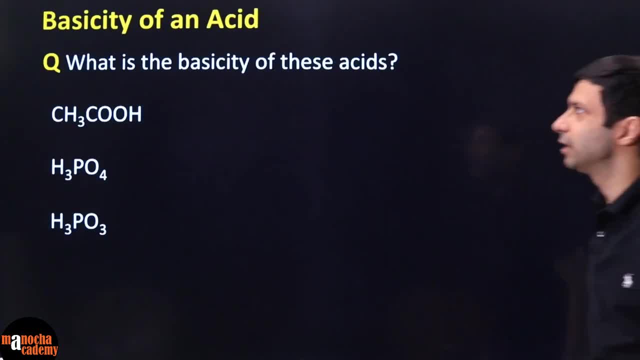 so its basicity was one. In sulfuric acid both the hydrogens say we are ready to leave you right and combined with water so they produce two hydronium basicity is two. Now the question is 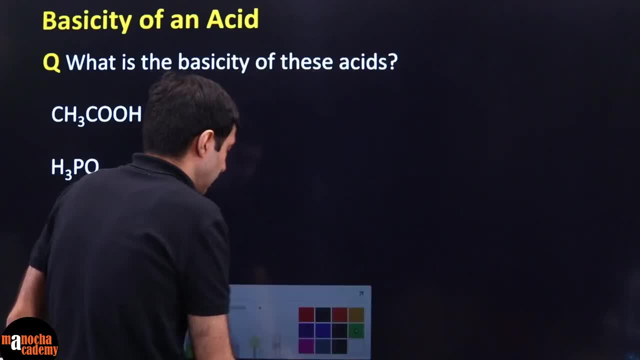 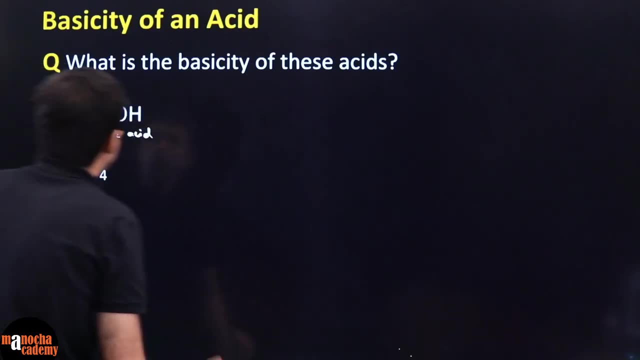 who is this guy CH3COH? This guy is basically acetic acid the one found in vinegar. In acetic acid one thing is very interesting only one hydrogen is replaceable. 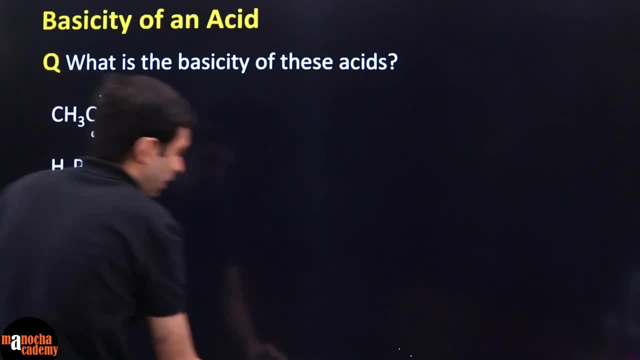 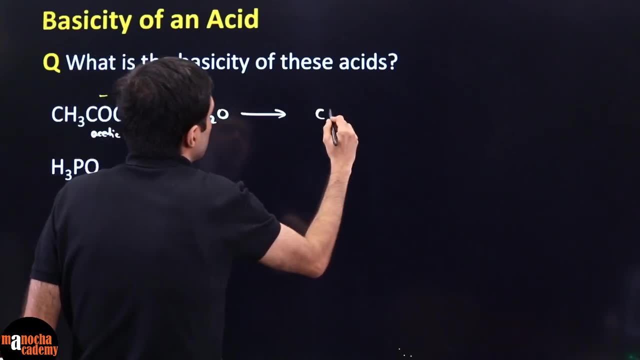 one hydrogen only this outside they're not these guys they are tightly bound to carbon so what happens is when this reacts with water it produces ch3 COO 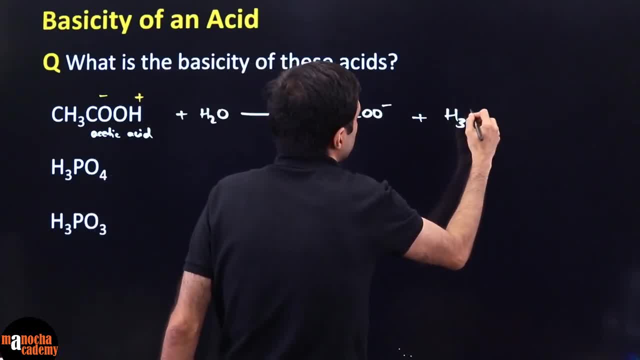 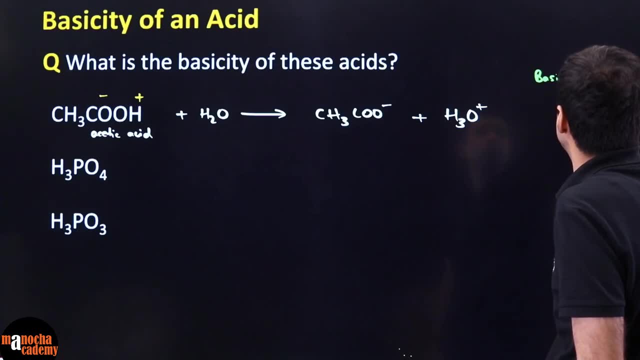 minus and only one hydronium so that is why we say basicity is how much one because one molecule is producing only one hydronium ion in spite of it having 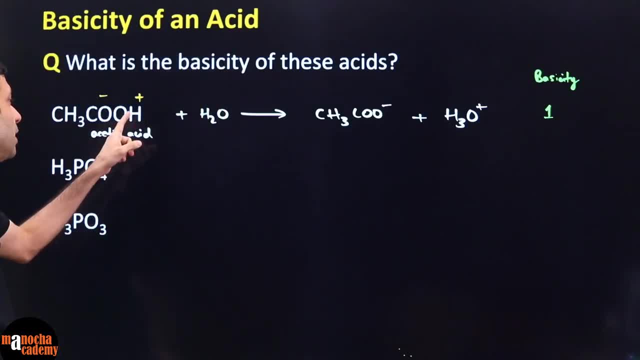 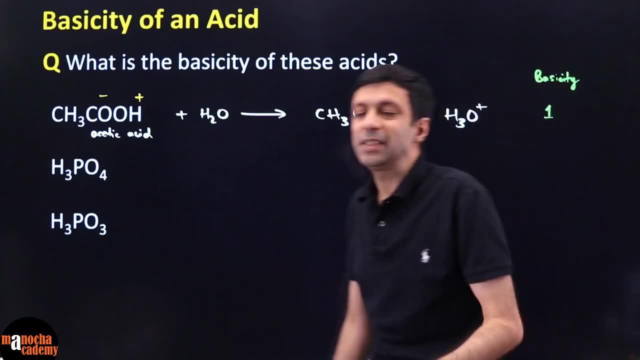 four hydrogen atom so don't be fooled by counting hydrogen atom so 1 2 3 4 basicities for no it is only one when basicity is one we say it is mono basic 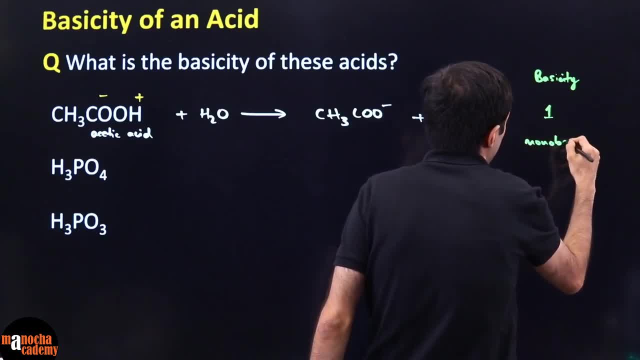 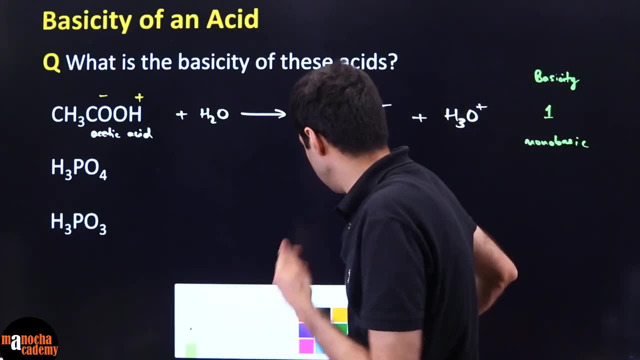 this is called mono basic mono means one what about the next one h3po4 that is called phosphoric acid so you need to learn these names guys h3o4 po4 is called phosphoric acid 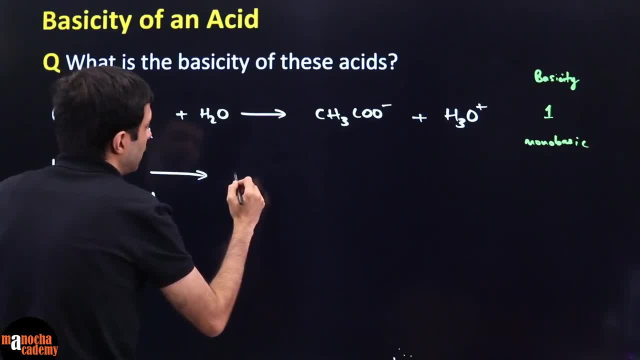 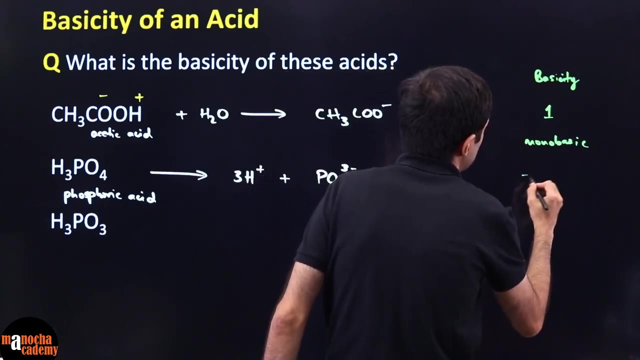 this when combined with water or if you break it down it basically ends up producing 3h plus ions and phosphate ions and these will of course combined with water to form hydronium so here basicity I just written it in the simplified form basicity is three this is dry basic what about the last one 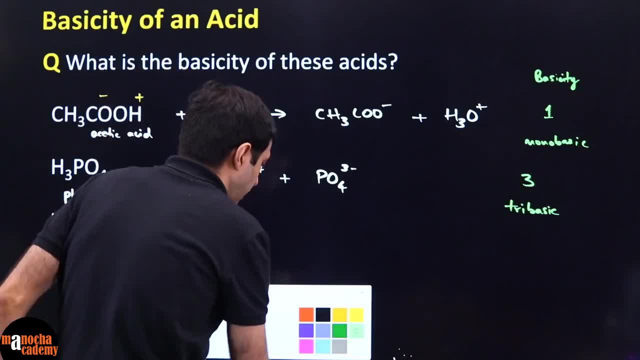 h3po3 this one is called phosphoric acid this one is called phosphorous acid 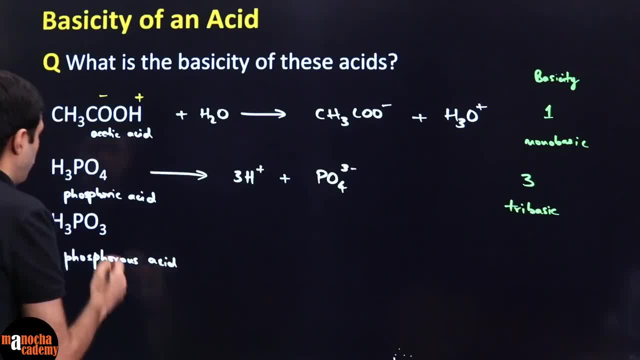 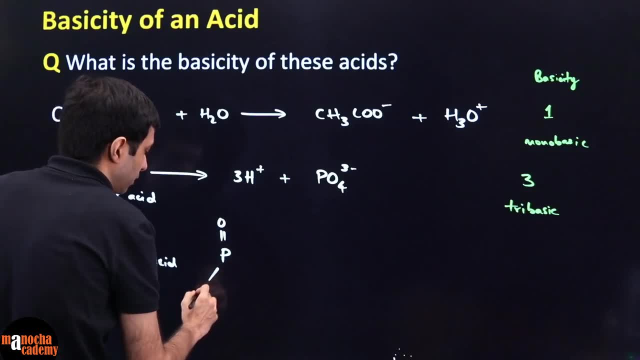 here it is very interesting phosphorous acid has a different type of structure its structure is phosphorus combined with there to OH over here and so see three oxygens and there's one hydrogen in phosphorus as valency of five and this 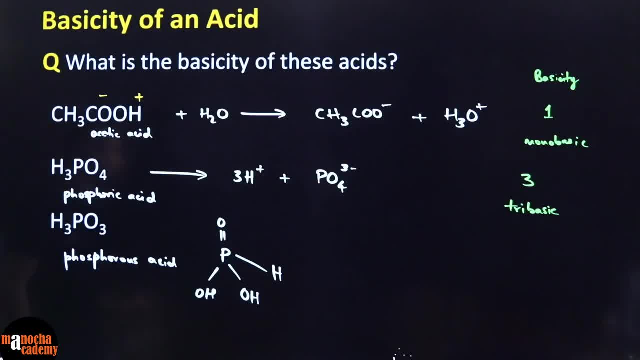 is how the structure looks like in this the interesting thing is only these two hydrogens are replaceable only to replaceable hydrogens so here I want to calculate only the two changeable hydrogens 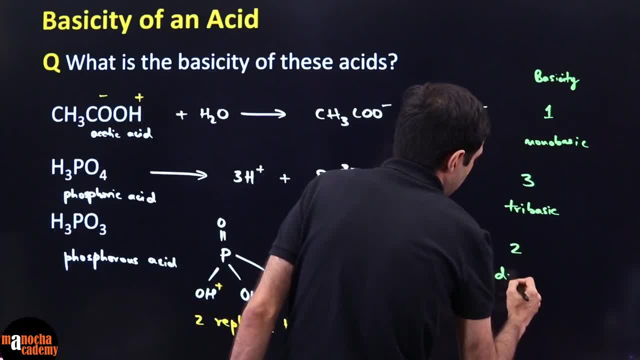 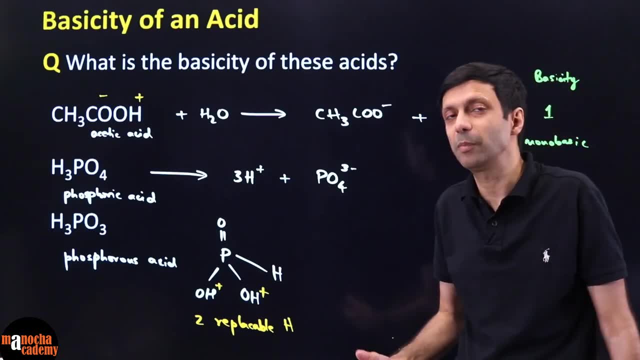 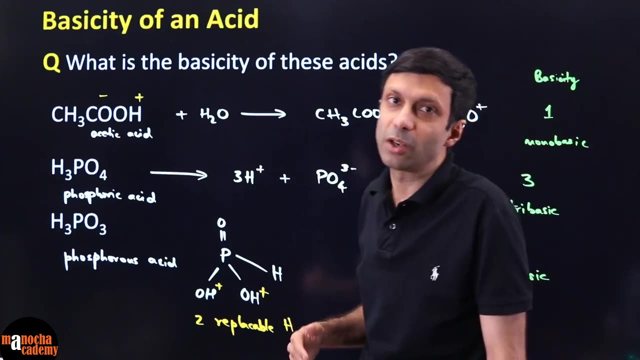 the basicity is going to be 2. It is dibasic. So please do not be fooled by the number of hydrogens. It depends on how many hydrogens are actually replaceable. So these are famous questions that acetic acid, what is its basicity? Even though it has four hydrogens, why is it not tetrabasic? Because only one replaceable. Same way, phosphorus acid, only dibasic. So 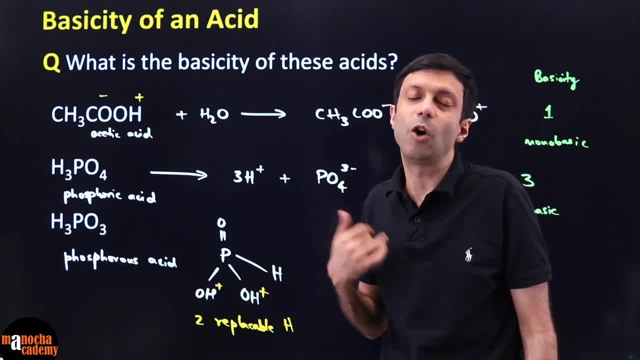 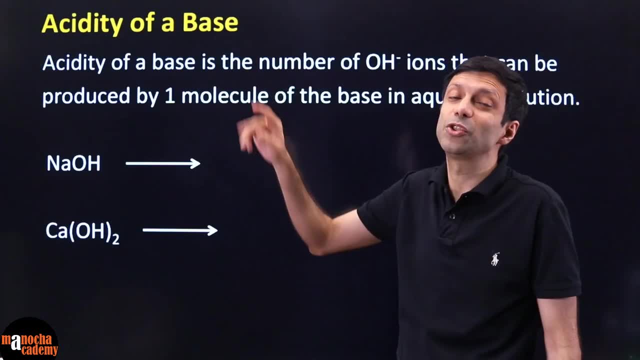 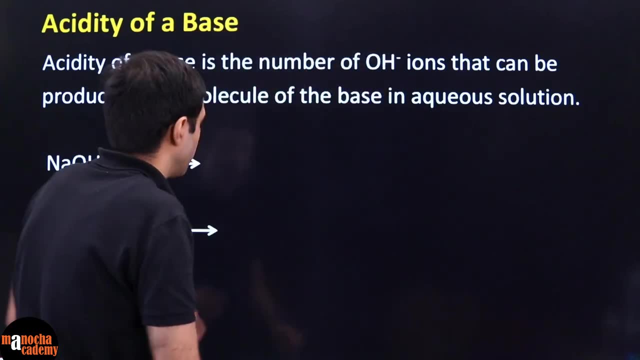 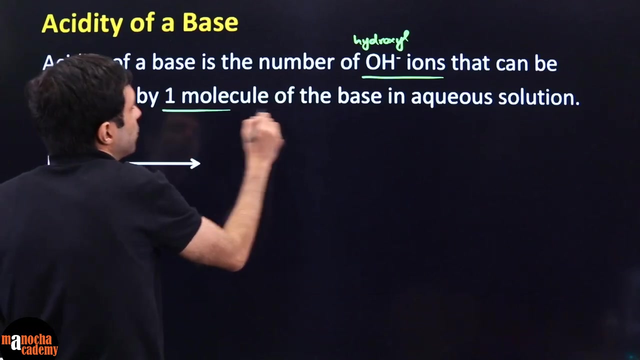 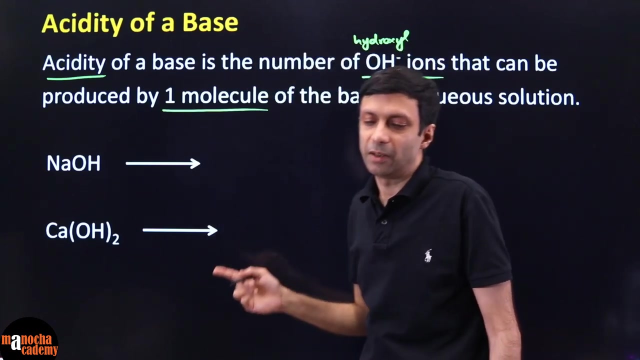 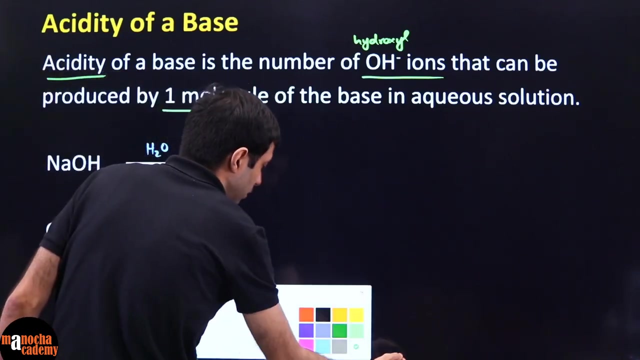 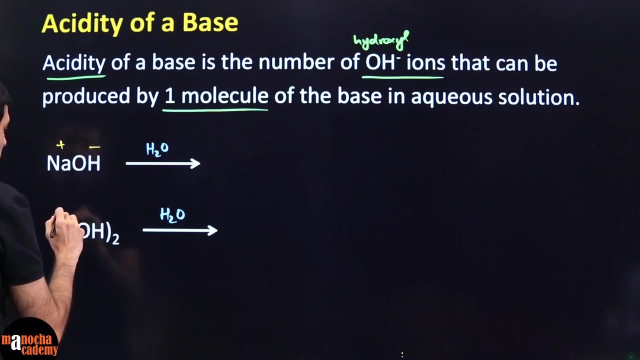 the difficult thing is you can't predict it, you have to learn it up, right? You need to know how many hydrogen atoms will come out. Just like you have basicity of an acid, it's funny, you don't have basicity of base, it is called acidity of base. So why these funny names? Because base neutralizes acid, right? So that is why we use the term acidity of the base. And here it is exactly the opposite of basicity. It is basically how many hydroxyl ions, OH minus, OH minus is called hydroxyl. So how many OH minus ions one molecule of the base is producing, that is called the hydroxyl. So this is the acidity of the base, okay? So for example, here, if you take sodium hydroxide and you put it in water, similarly, you take calcium hydroxide and put it in water, how will it break down? So this one is actually simpler, because you know, sodium hydroxide breaks down as Na plus and OH minus. Similarly, for calcium hydroxide, Ca2 plus and OH minus. 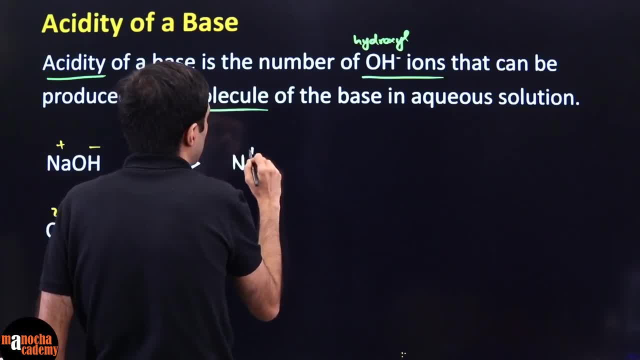 So what's going to happen here? Sodium hydroxide is going to produce sodium ions and hydroxyl ions. 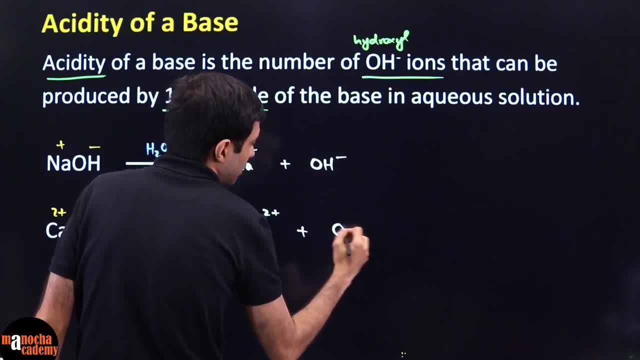 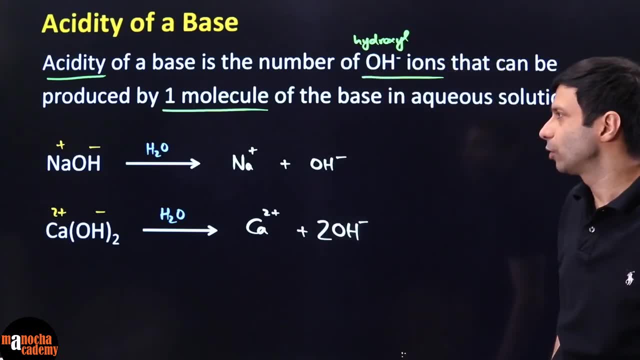 Calcium hydroxide is going to produce calcium and hydroxyl, but because there is two hydroxyl, it is going to produce two OH minus ions, both the hydroxyls will come out. So can you 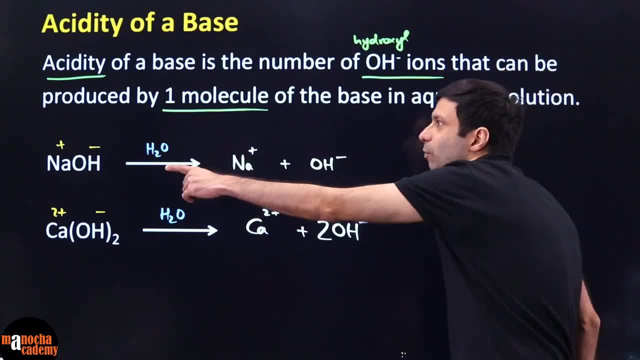 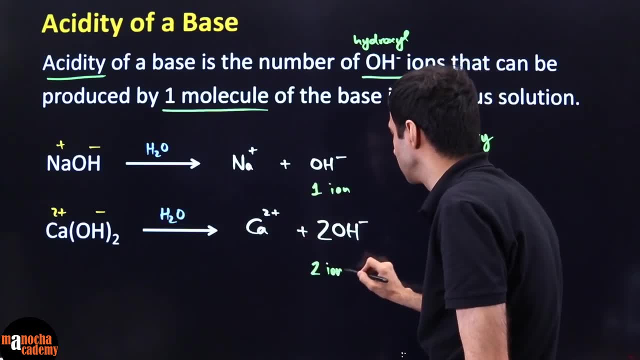 guys tell me what are the acidity of these bases? One molecule producing one ion. They are one molecule producing two ions. So here we can say acidity is one. This is monoacidic base. 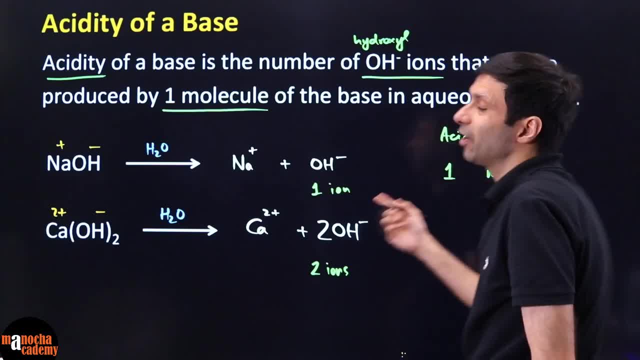 We say this is a monoacidic base, because it is having a power of one, it produces one 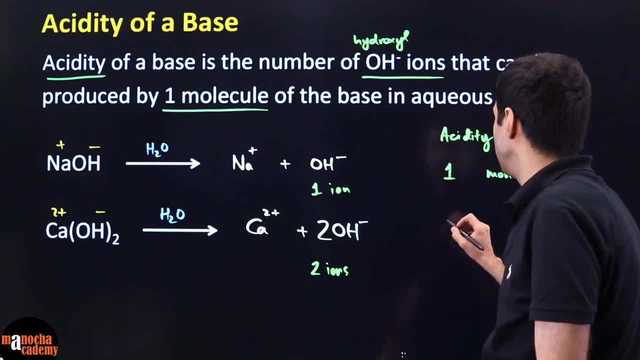 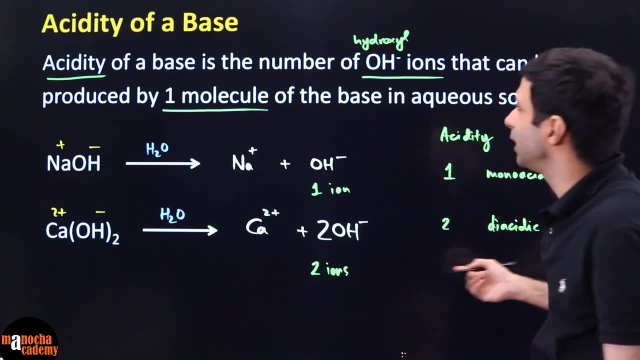 OH minus to neutralize the acid. Similarly, here, acidity is two. This is basically diacidic base. Only the names are a little confusing. It is not mono basic. It is called monoacidic 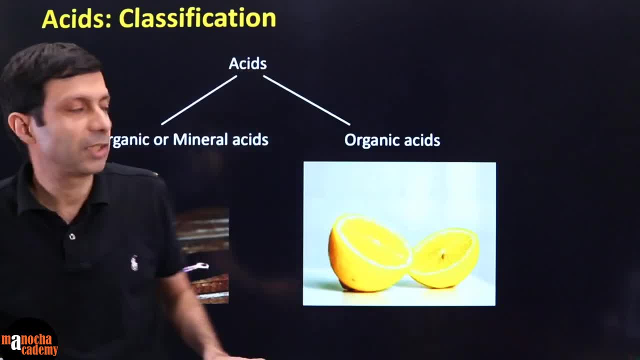 base. How can we classify acids? You might have heard of this classification. Acids can be classified as organic and inorganic. Organic means these are coming from nature. So these are organic and inorganic. So these are coming from nature. So these are coming from nature. 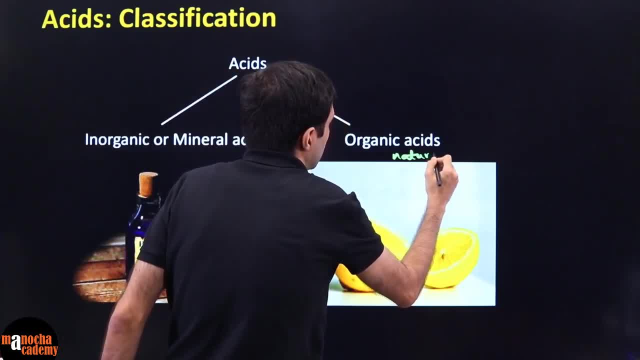 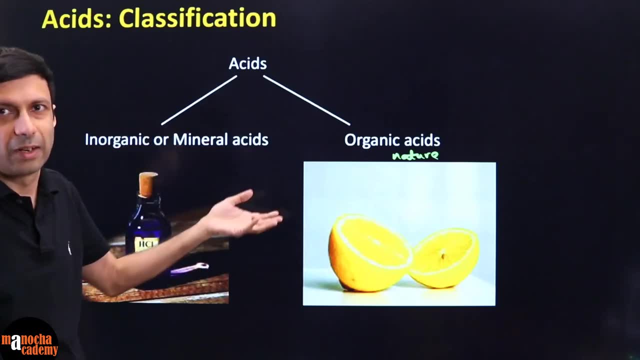 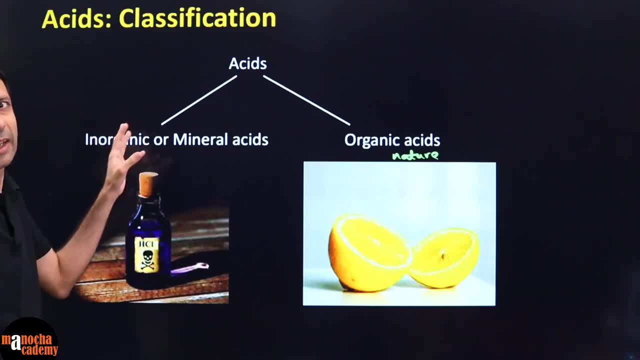 These are all your organic acids. And opposite is called inorganic or mineral. So what are some examples here? So you need to learn some examples. So mineral acid, the examples of which are found in rocks and minerals like hydrochloric acid, sulfuric acid, nitric acid. 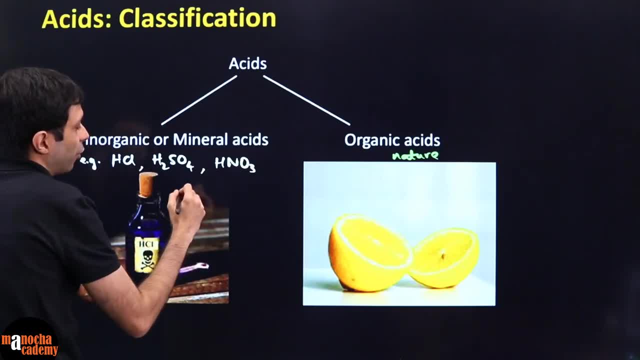 And usually these are the strong acids. Typically. Often we find organic-derived acid. So we put right except for carbonic acid which is the weak acid rest are all typically the strong ones 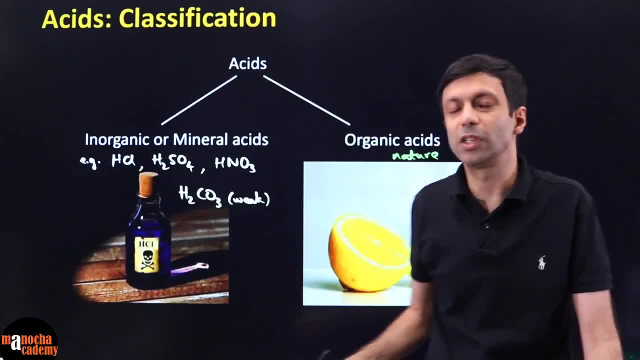 hydrochloric acid is very interesting it is considered mineral acid because it is found in rocks and minerals plus it is found in our stomach so don't say it is organic because it 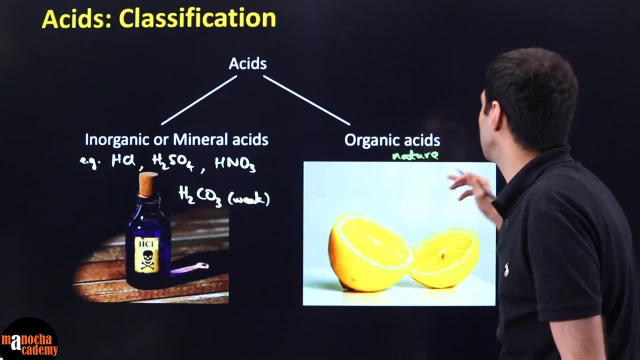 is also found in the rocks and minerals it is in the inorganic and here organic examples are basically your citric acid acetic acid all these acids found in fruits you know and we usually 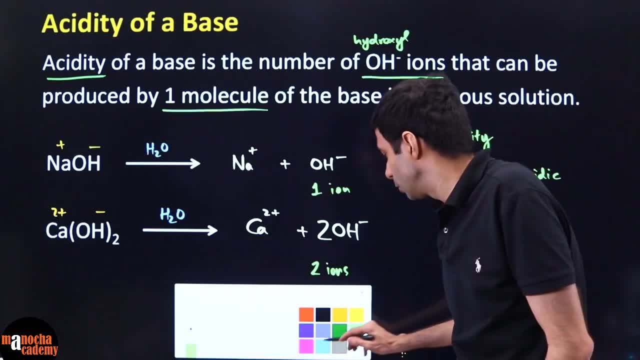 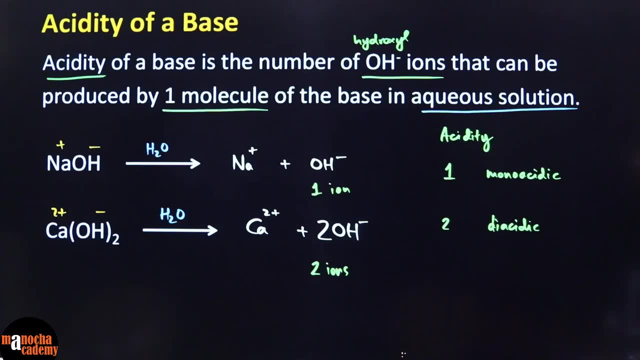 eat these acids they are weaker acids so that is why we will be coming to that it is for the alkalis the bases which are soluble in water that's why i want you guys to watch the basic videos today i'm doing the more difficult concepts which a lot of students don't understand clearly 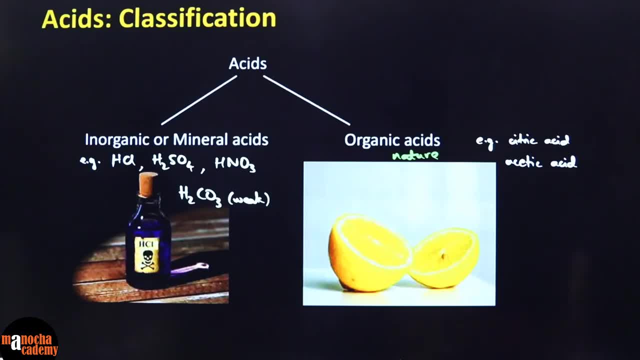 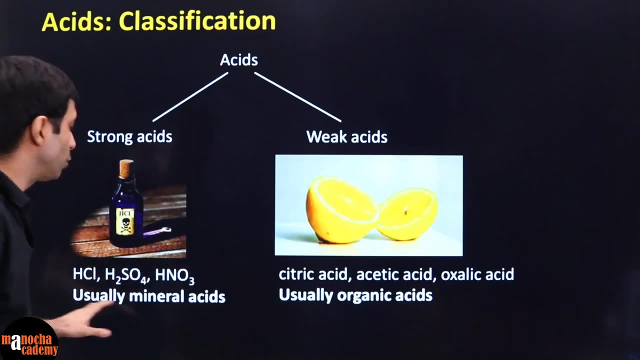 for these basic kind of things you can watch the videos on that so just like we can say organic inorganic we can also classify acids as strong and weak acids so weak acids is usually all the mineral acids right like hcl h2so4 hnothorax 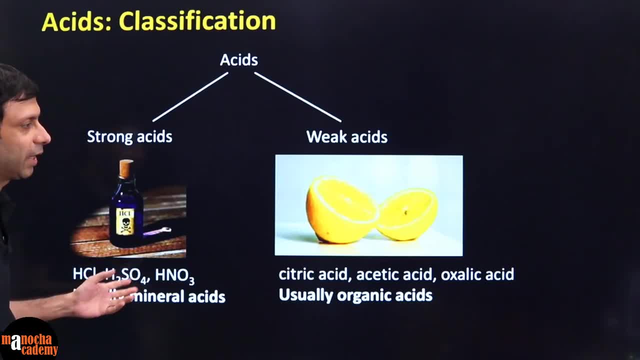 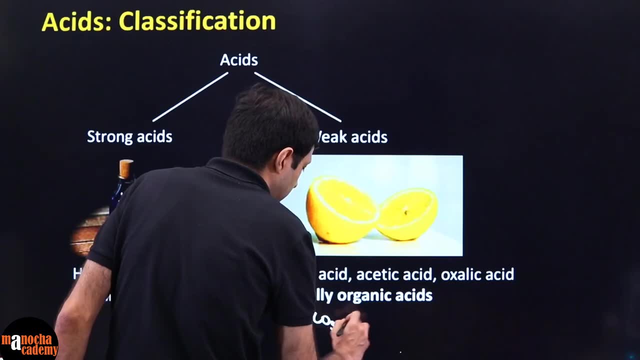 3 exception is carbonic acid right carbonic acid comes under weak acid even though it is mineral so even here you have carbonic acid is a weak acid which is a mineral acid usually the weak 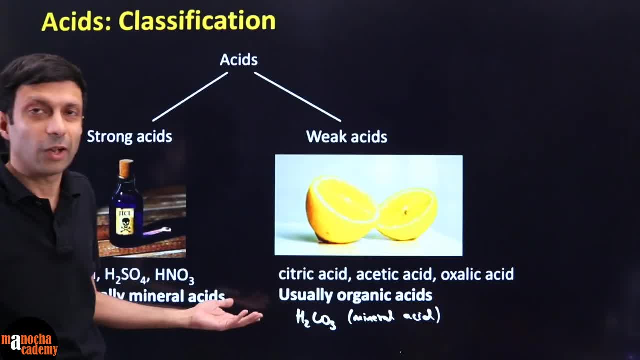 acids you have eat you have had you have eaten it have do you know where carbonic acid you have 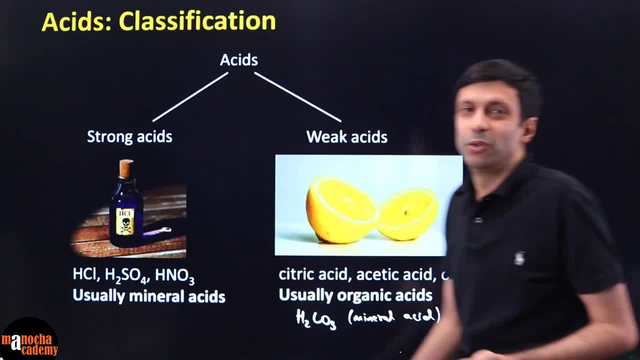 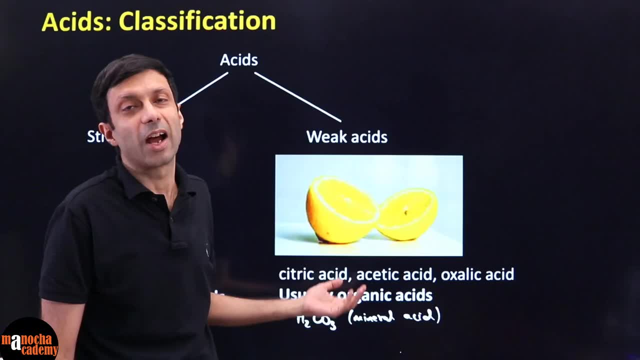 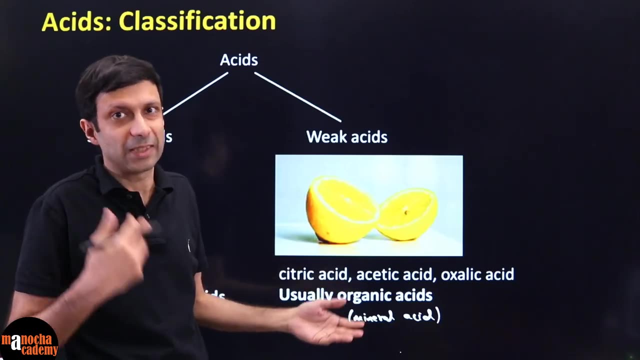 you've had or you've drunk carbonic acid can you guys tell me so in the the carbonic acid is what you drink in the aerated drinks the soda drinks right they basically contain your carbonic acid that is why you see that phase because carbonic acid is made by carbon dioxide and water and it's obviously a weak acid since you are having it right these are strong acids 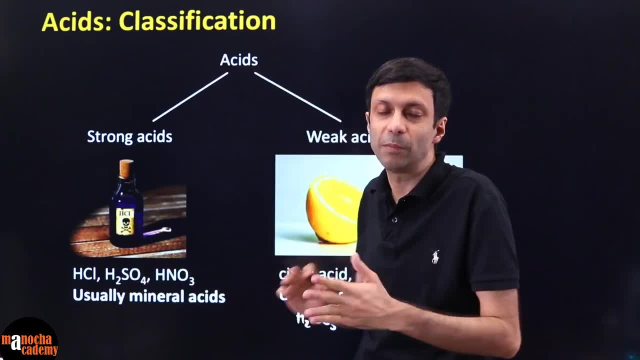 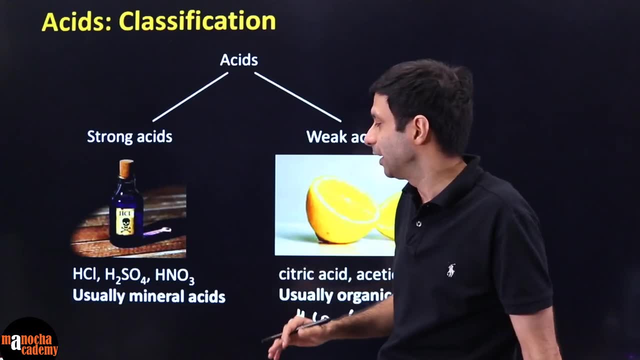 are very dangerous hcl h2so4 hno3 we should not even touch them they can corrode our skin right make the skin black and cause this kind of you know corrosion in the skin so they are highly 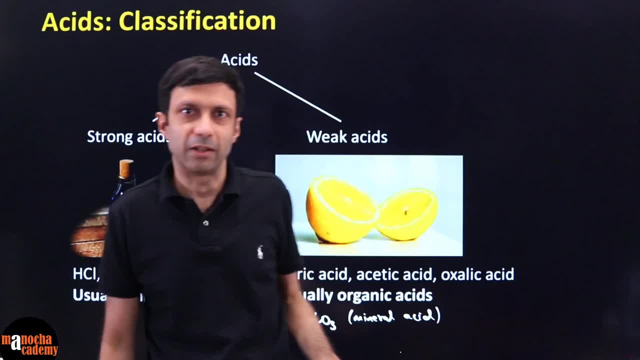 dangerous now what makes an acid strong or weak it's not like did it come from nature or not right what makes it strong 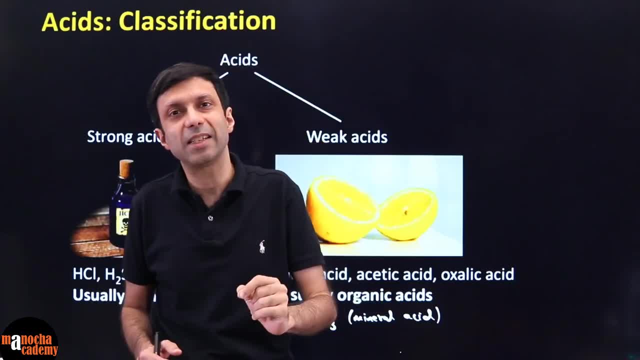 or weak again reminding you that how what makes something an acid it is not just the hydrogen 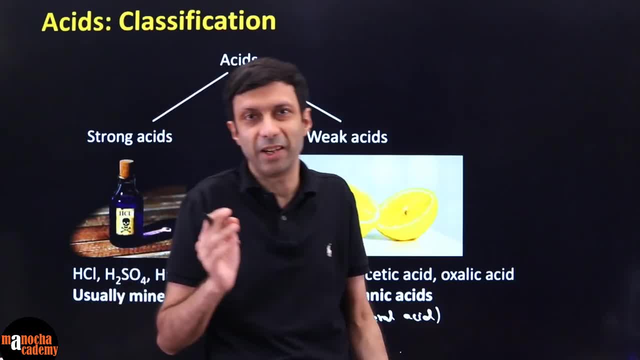 present in it otherwise water would also be a would also be an acid right water is not an acid 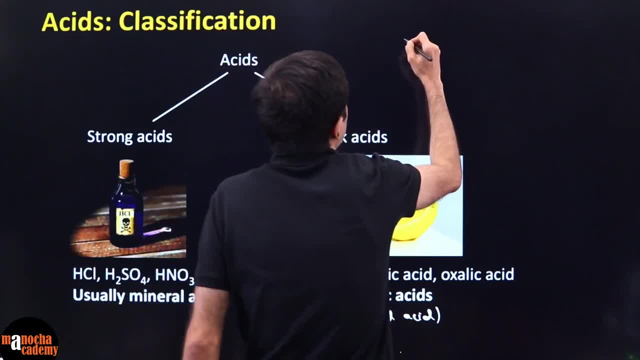 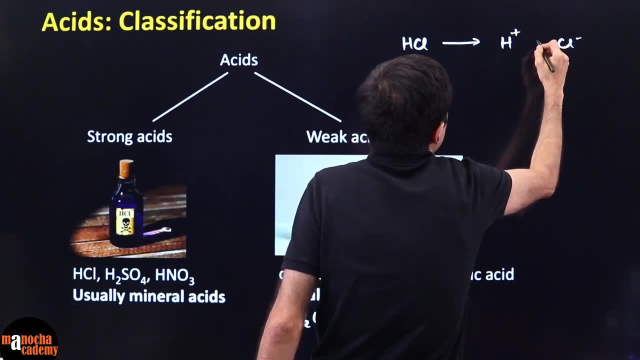 it is basically that if you take any acid like hcl it breaks down in water to produce h plus and cl minus ion see i'm writing this simple equation i i can also write it as plus 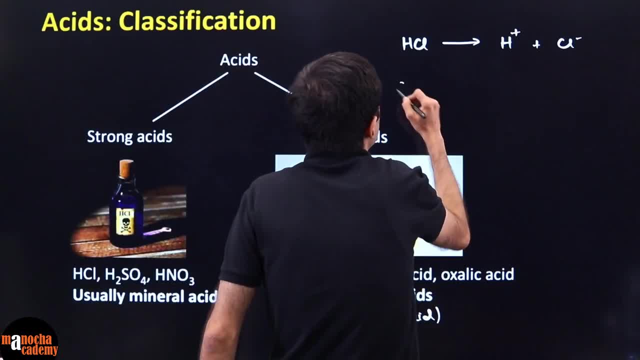 water and show hydronium i'm just showing the simplified equation similarly if you take acetic 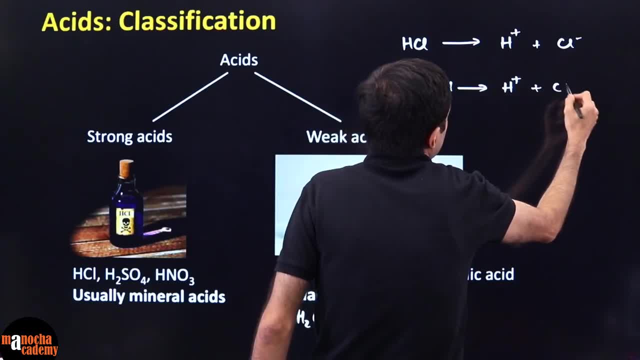 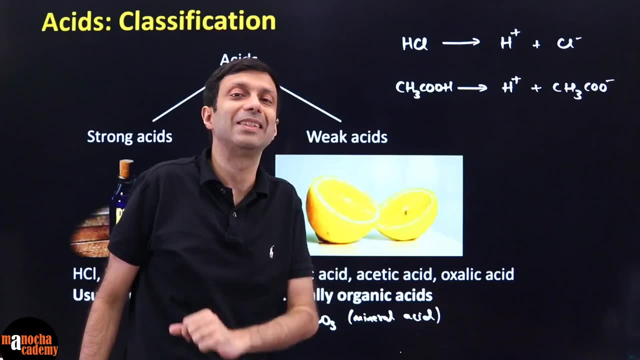 acid it breaks down in water to produce h plus and acetate ions right so what makes an acid strong or weak again it will break down to give h plus and acetate ions right who is strong or weak it 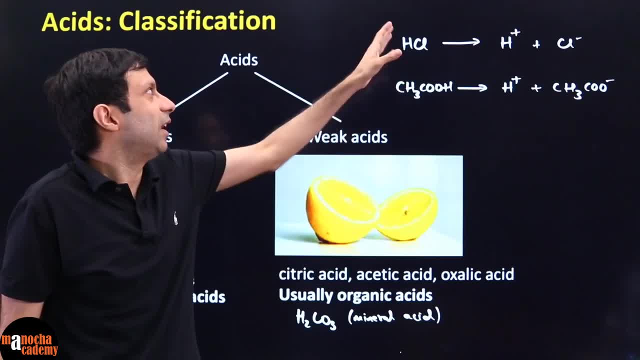 depends on how much it breaks down or what we call as degree of dissociation so basically think about 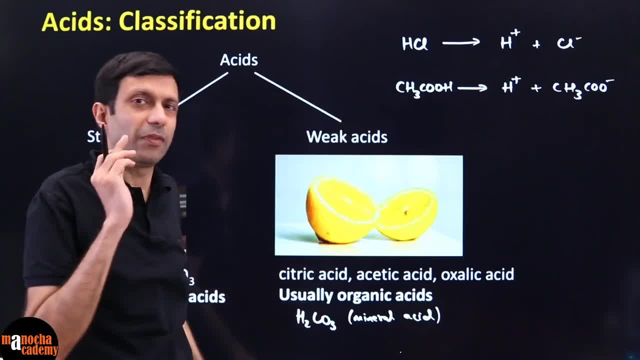 this let's say in a solution you have 100 molecules of hcl and 100 molecules of acetic acid in two separate glasses okay so you have taken 100 molecules of hcl imagine you have 100 molecules of 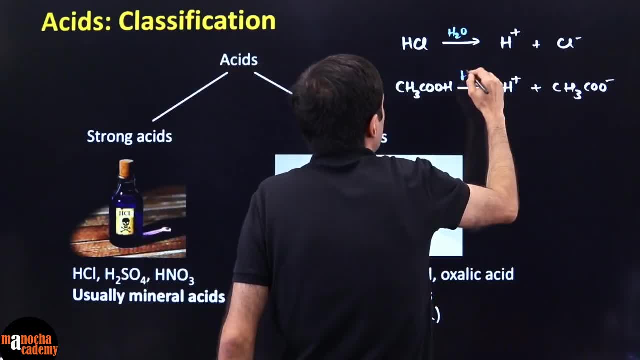 acetic acid and you dissolve it in water so when these guys are put in water what the scientists 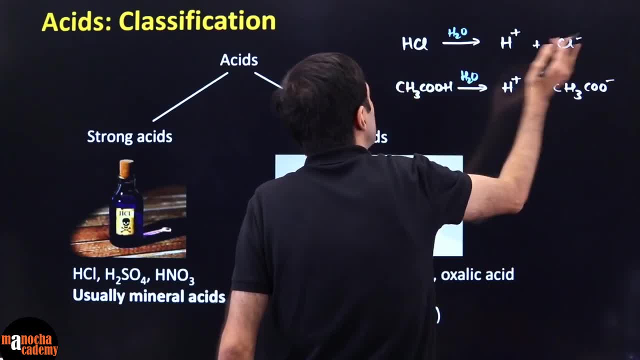 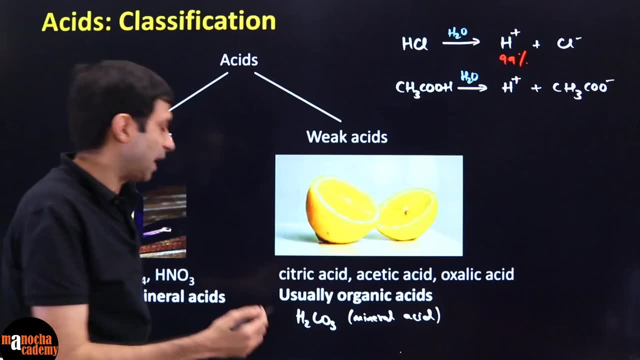 have observed is that hcl almost 100 percent breaks down or 99 percent it breaks down and produces a lot of h plus ions but acetic acid on the other hand they found it is only producing 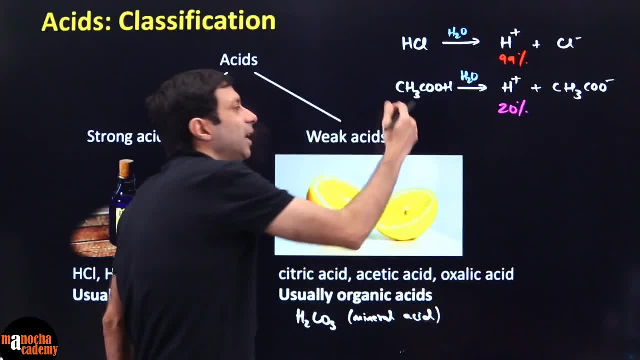 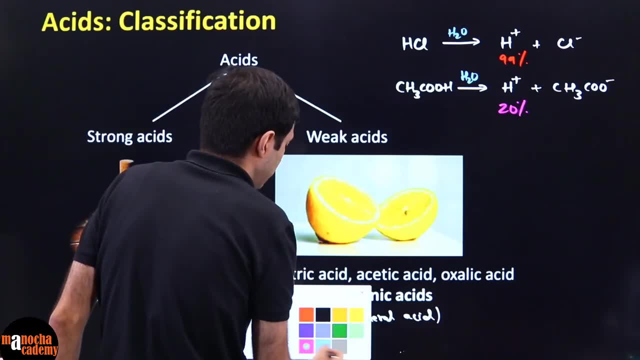 let's say 20 percent it breaks down remaining is not broken down or we say undissociated so what does the strength depend on it basically depends on the 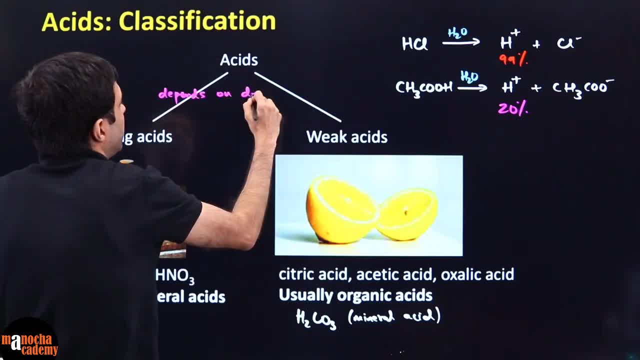 this classification depends on degree of dissociation how much the acid breaks in water 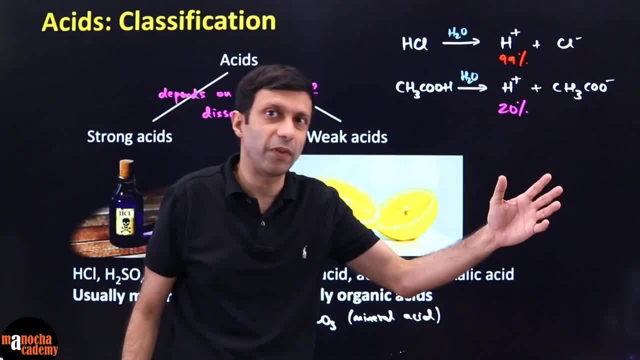 that means if it breaks a lot in water it will produce a high concentration of h plus or a high concentration of hydronium ions right h plus and water then it will become a strong acid but if an 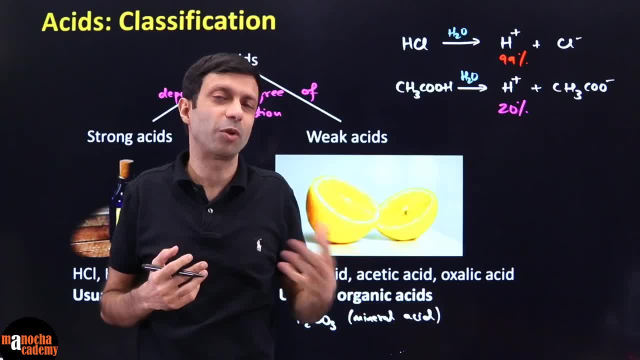 acid produces very less h plus even though it has lots of hydrogen it's not producing h plus it will be having a low concentration is that clear and this degree of dissociation is typically denoted by the symbol of dissociation or it is denoted by the symbol of dissociation or in the 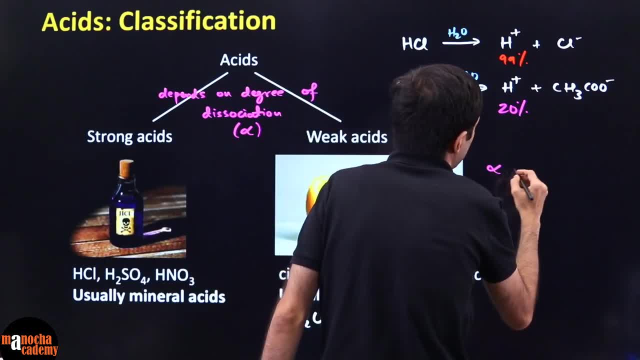 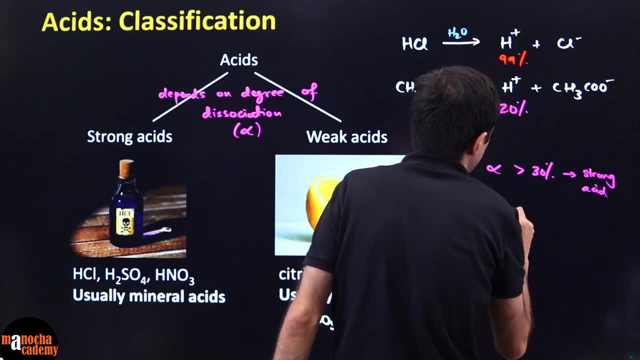 alpha so what is the general rule that a degree of dissociation is greater than 30% then it is a strong acid if degree of dissociation is less than 30% it is a 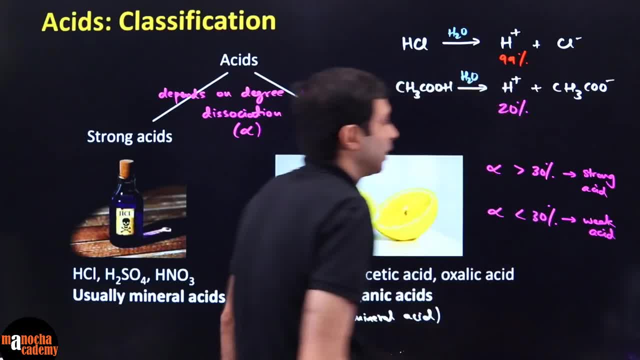 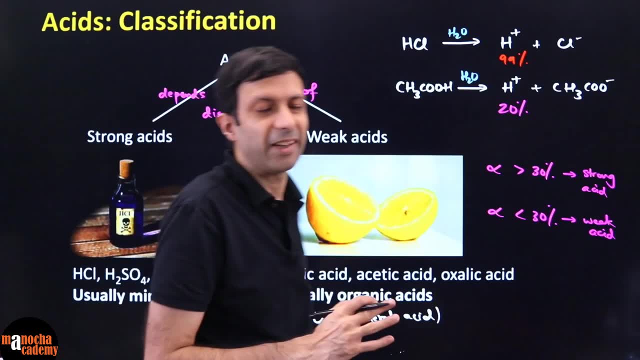 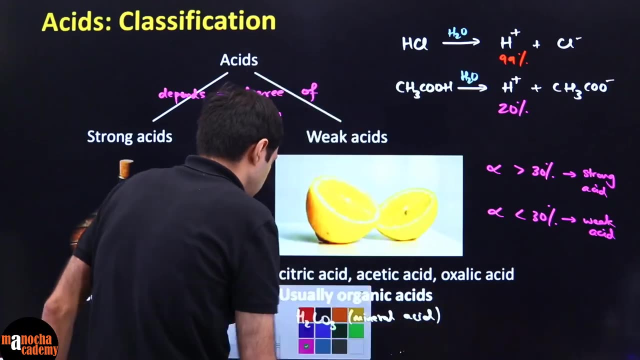 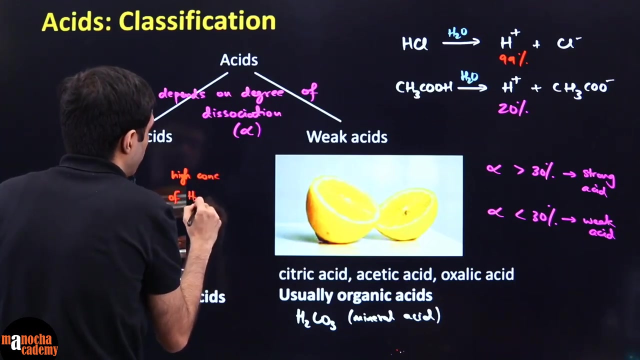 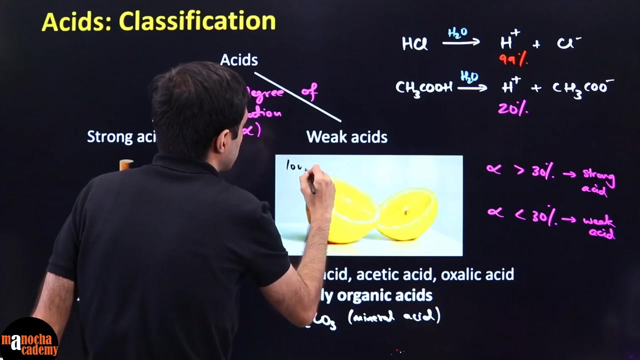 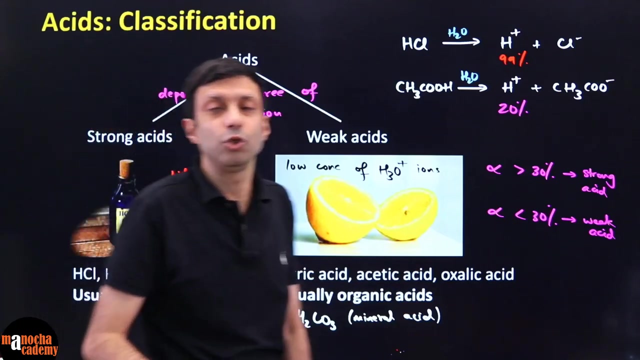 weak acid so usually you'll see in the books 30% 20% this kind of number is given so basically if it almost fully dissociates like strong acid they almost break down completely right 9900 percent so that is when they are strong acids so strong acid is a strong acid because it is having a high concentration high concentration of h3o plus scenes ok and this one is having a weak acids ever low concentration of hydronium ions since you guys angplastin typically you should use the word hydronium avoid the word H plus ion because you guys in class 10 that is the simplified form 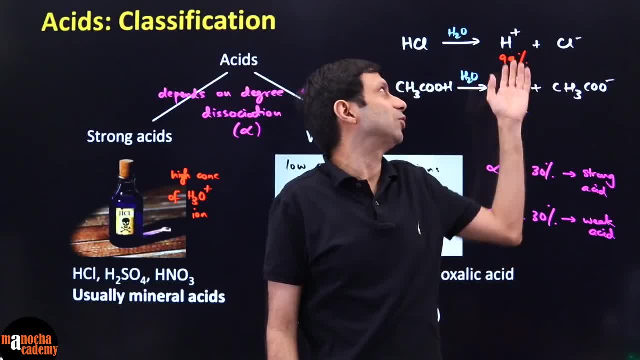 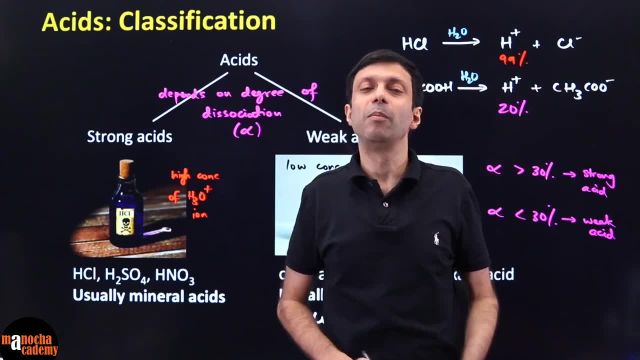 the real form is H plus combines with water but just to explain it simply many times you'll see in the books it is also written in terms of H plus but when you are writing your answers this is an important tip please write hydronium H3O 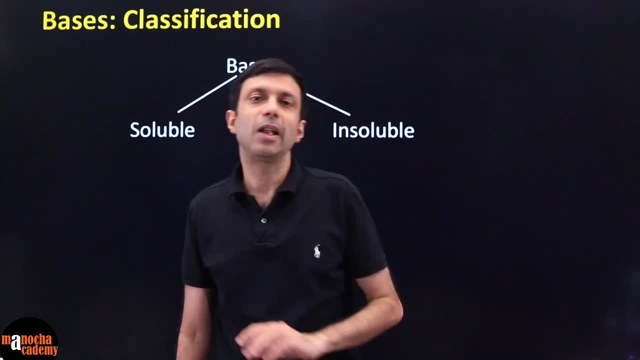 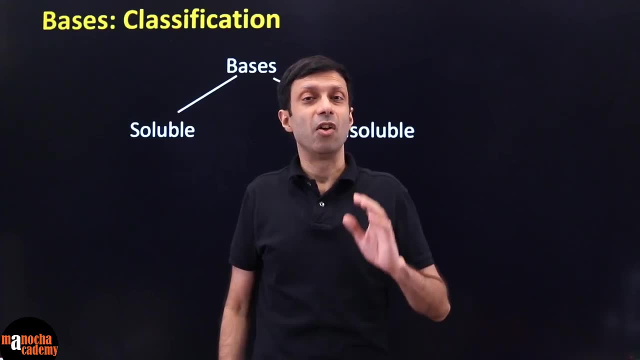 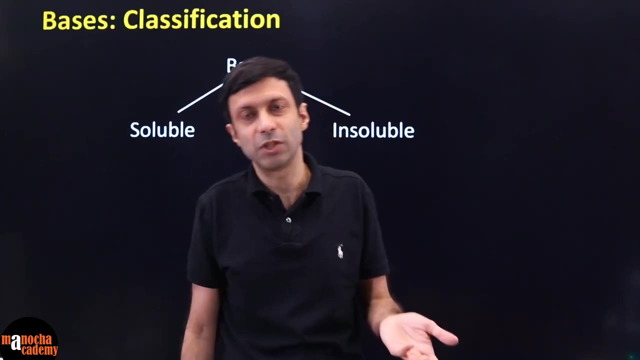 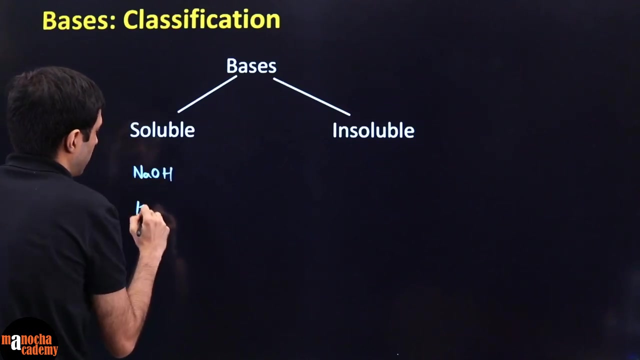 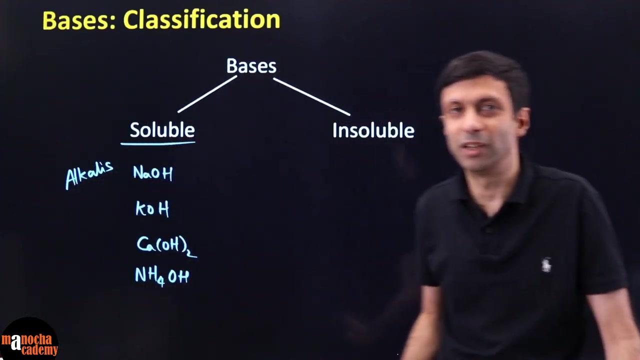 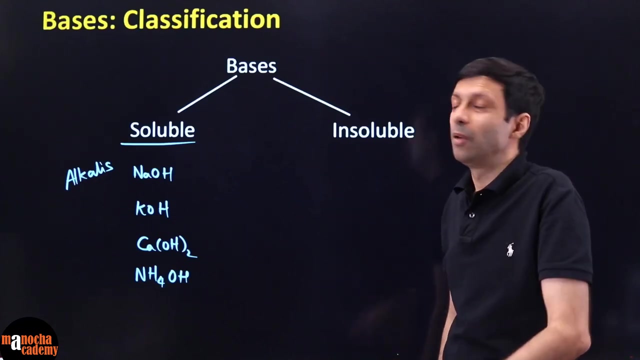 plus ions okay one important thing to remember all acids are pretty much all the acids are soluble in water so any acid you can easily dissolve in water but bases the very few bases did you know very few bases actually dissolve in water or they are soluble in water what are those bases which are soluble in water it's a very small list it is basically sodium hydroxide potassium hydroxide calcium hydroxide and ammonium hydroxide these guys are soluble in water these are soluble bases and they are known as the alkalis so bases which are soluble in water are called alkalis that's why you might have heard of the term alkalis alkaline solution when you dissolve a base in water if it's soluble it is called an alkali the solution is called alkaline in nature but most of the bases 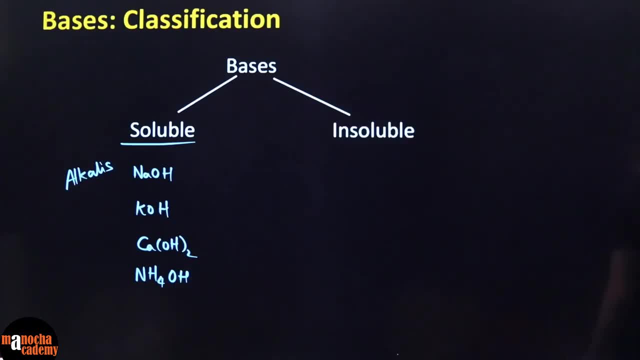 are not soluble in water for example so most of the bases that you have they are 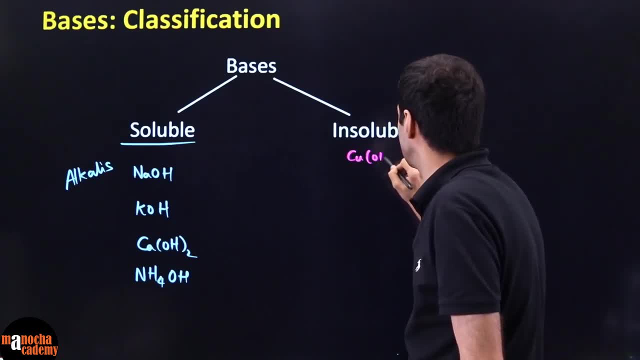 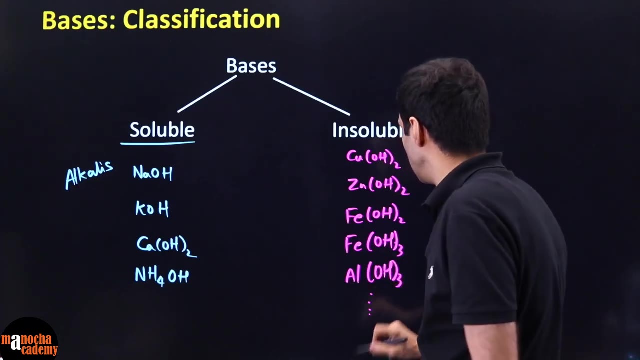 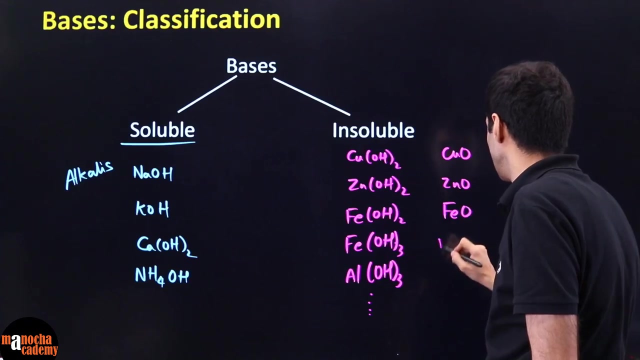 insoluble in water like if you take copper hydroxide zinc hydroxide ferrous hydroxide ferric hydroxide all these guys all insoluble in water aluminium all these metal hydroxides and their corresponding oxides also copper oxide will not dissolve zinc oxide will not dissolve iron oxide will not dissolve Fe 2 O 3 will not dissolve aluminium oxide does not dissolve okay these are all 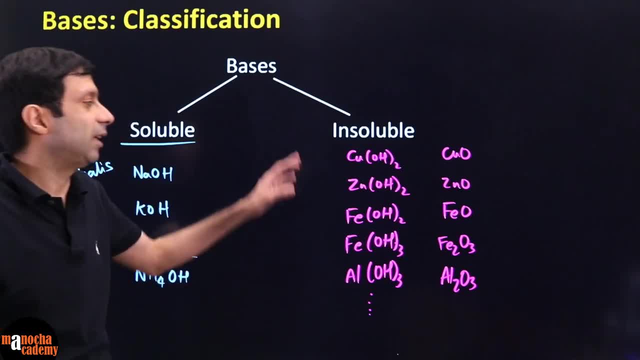 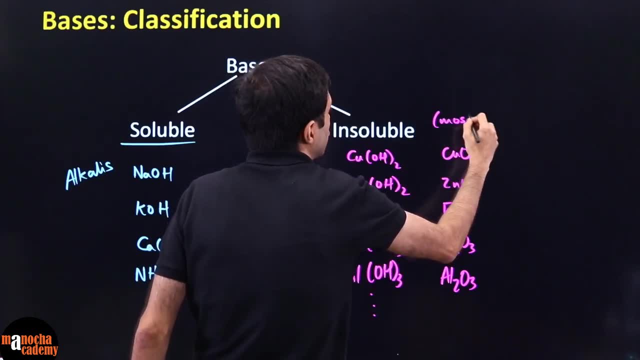 insoluble so most of the bases are actually falling into this category most of the things so we should write that here most bases are actually insoluble how are these soluble ones? How are these soluble ones? 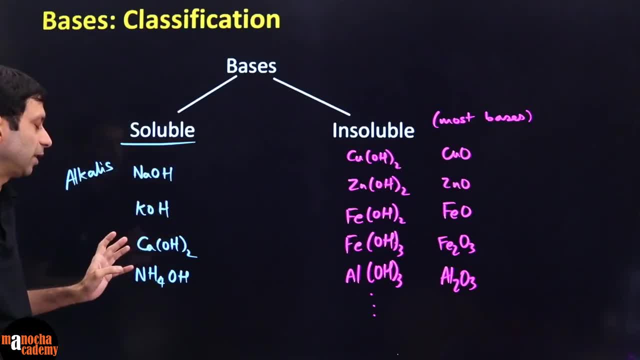 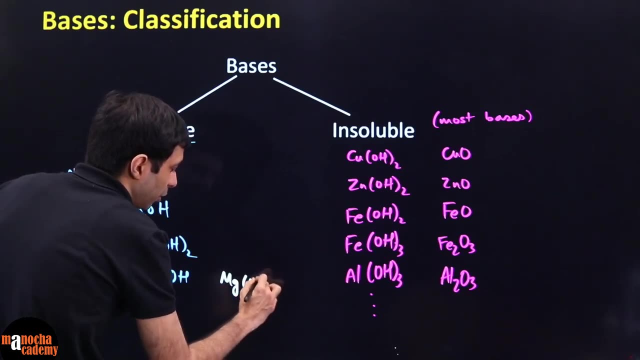 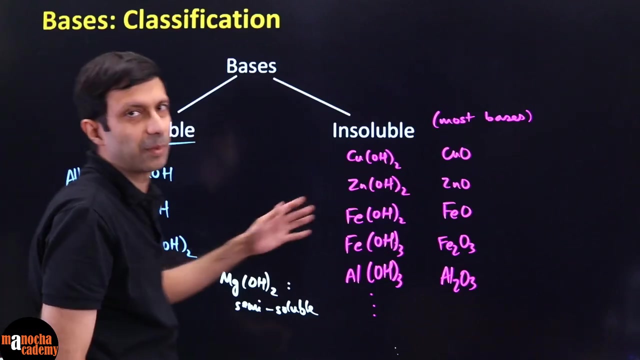 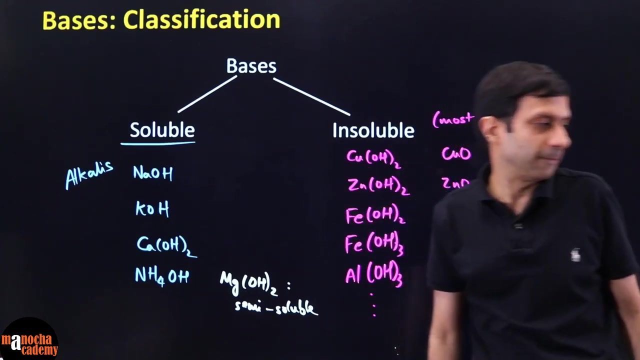 by dissolving sodium oxide and water potassium oxide and water calcium oxide and water and this is a separate one ammonia and water there is one exception here which you should know sometimes magnesium hydroxide so magnesium hydroxides are actually in the middle why do I say is in the middle because he is basically semi soluble this base is semi soluble so sometimes you will see him with the alkali list sometimes with the insoluble so you can learn what is given in your book but typically these are your alkalines but one thing 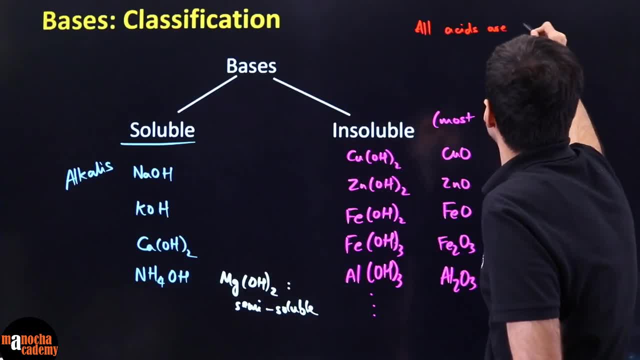 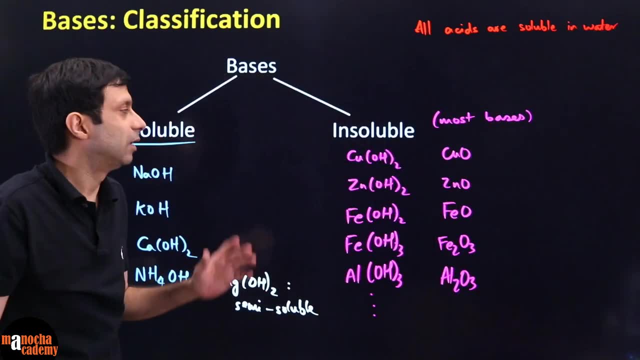 remember all acids are soluble in water so all acids are soluble in water so this is the technique how to identify the acid or base using the formula we 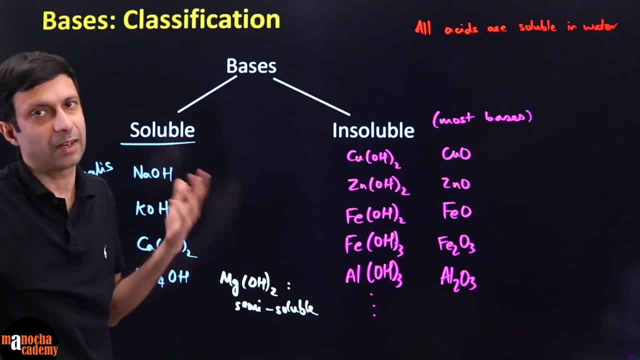 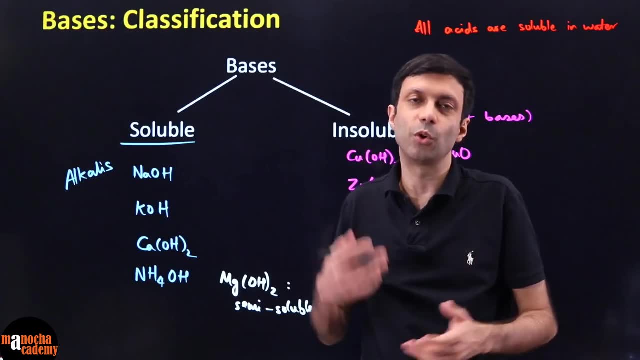 know that metal oxides metal hydroxides and ammonium hydroxide are our bases right so that is one way acid you will usually see it with the example hydro HCL h2 is a four so as you see the formulas you will learn and you will see why it is because you don't know that what is a 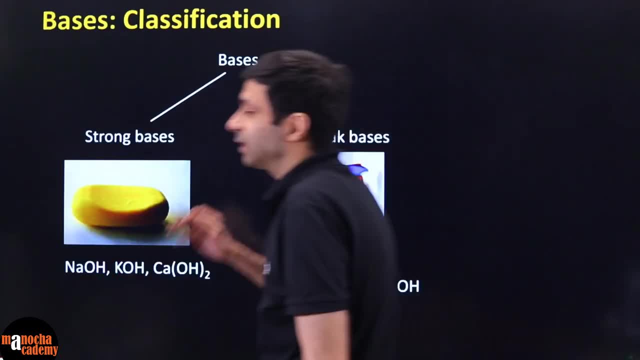 you will know that hey these guys are the assets okay now bases also just like acids can be classified strong weak bases also we can say strong weak 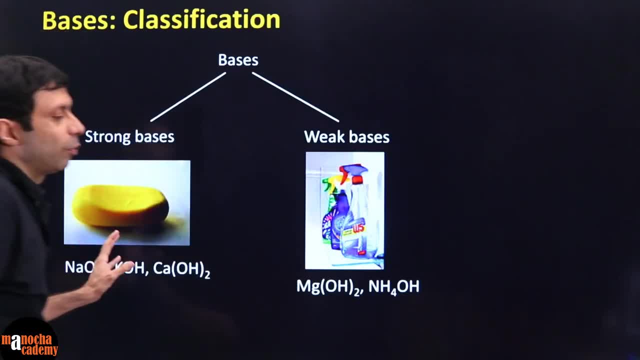 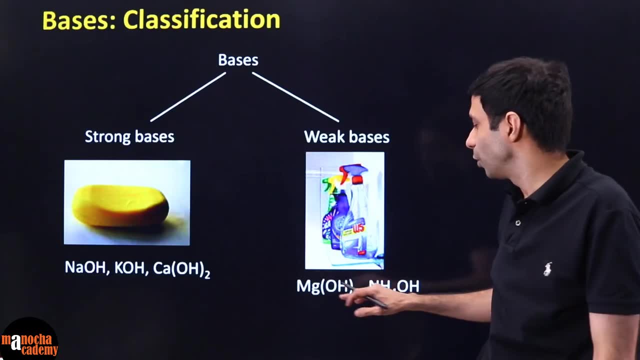 classification so typically again usually in your books you will see the bases that they are involved in involved with are usually the hydroxides right and see again I've taken the example of magnesium hydroxide because it is 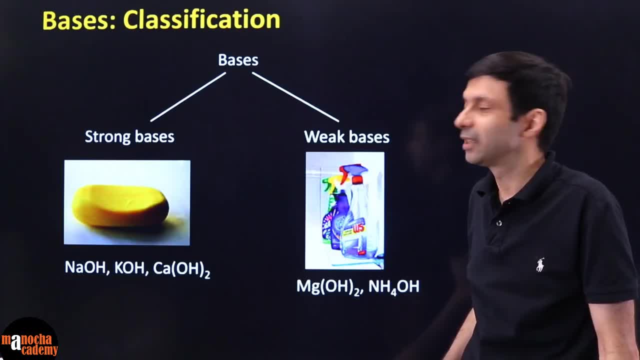 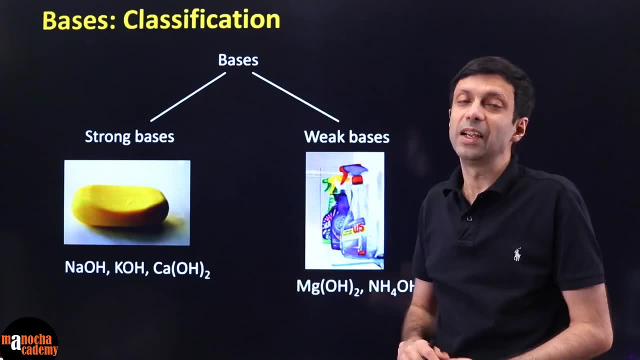 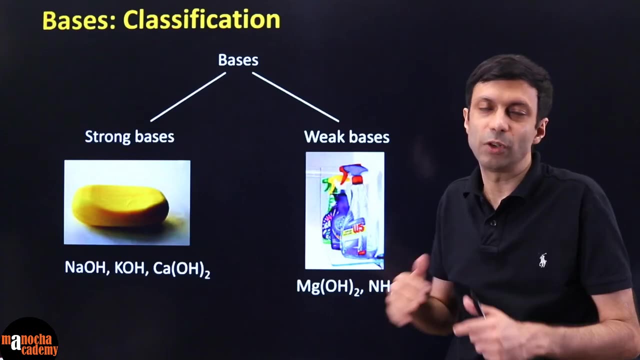 semi-soluble so you guys should know that who are the strong bases strong bases are sodium hydroxide potassium calcium hydroxide and these are again if you take concentrated solution of these these are highly corrosive in nature right so in soap they are found in very mild form or mixed with an acid which 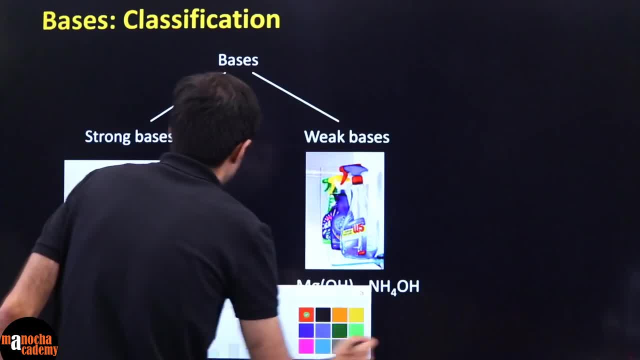 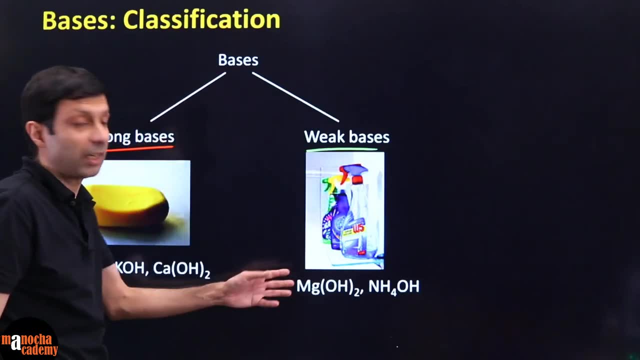 will neutralize it so these are the very strong bases they are highly corrosive and dangerous and these are the weak or the mild bases magnesium hydroxide ammonium hydroxide magnesium hydroxide you might have no known that when you have acidity you know this magnesium hydroxide is the milk of magnesia that you drink to neutralize the acid in your stomach well that is in milk of magnesium 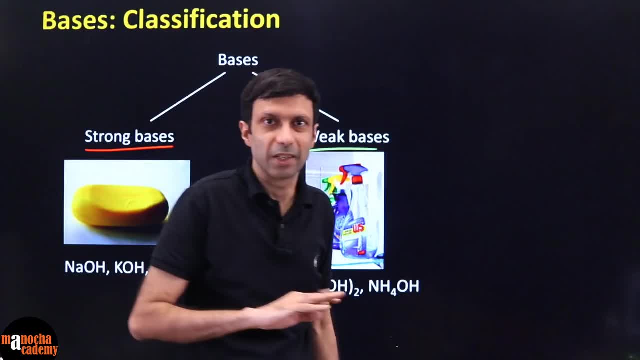 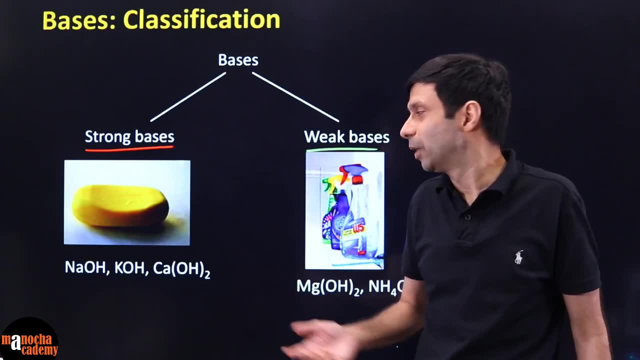 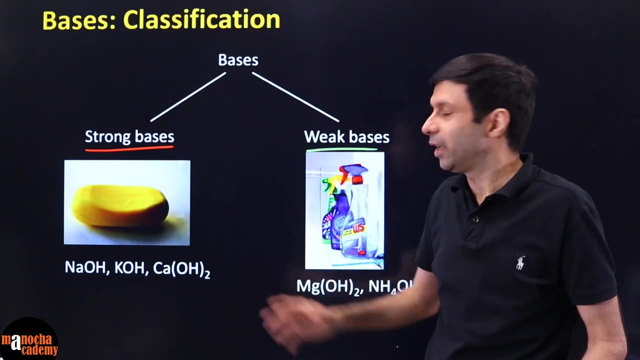 ammonium hydroxide you might know it is used in window cleaning it's a window cleaning agent and the sodium hydroxide it is used in manufactured soap potassium hydroxide in manufactured liquid soap calcium hydroxide you know it is used slate lime is used for whitewashing rent of the walls so there 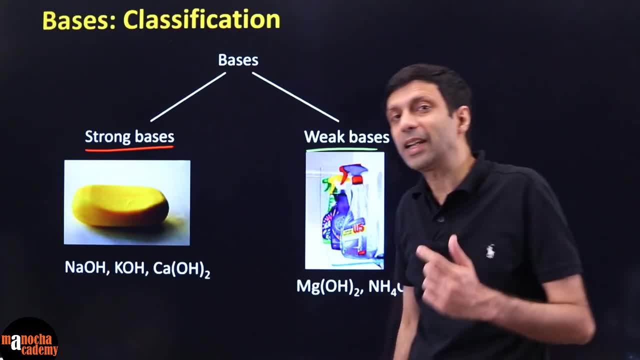 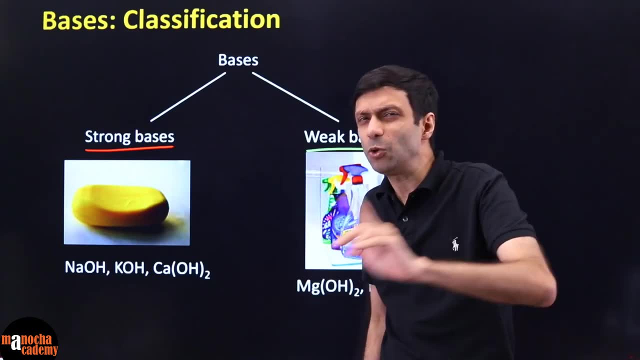 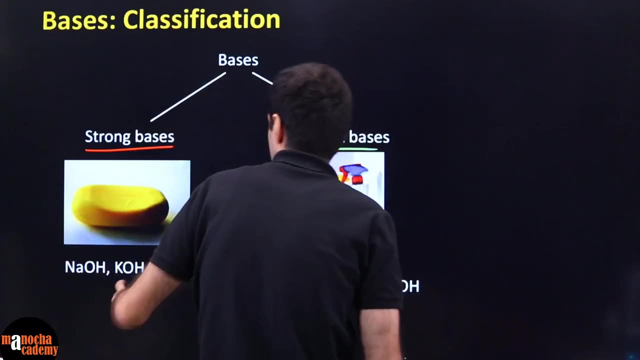 are various uses of these strong bases now again can you tell me again basis means we are looking at the alkali's here can you tell me what makes the base strong or weak can you guess it on the answer based on mineralWell well 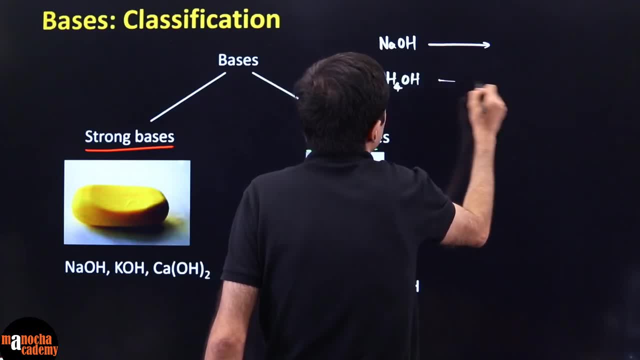 well this is the most important so the two aren't the only ones that process this said help you know when we're talking about the solution that one contains 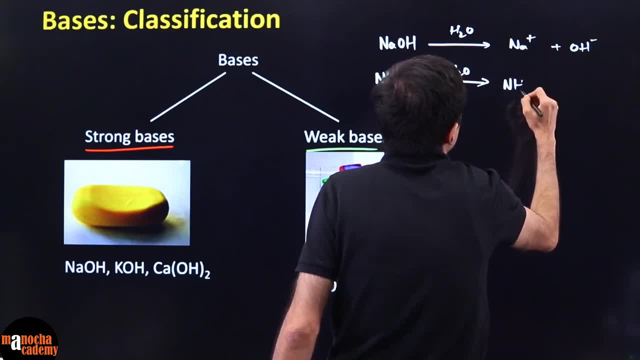 heard and said and that these pants are neutralizing it so we ch punkt here a second 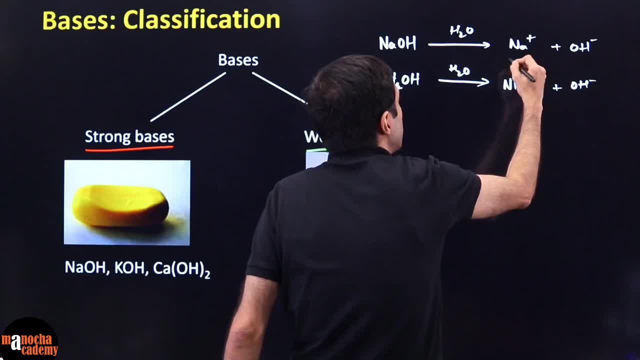 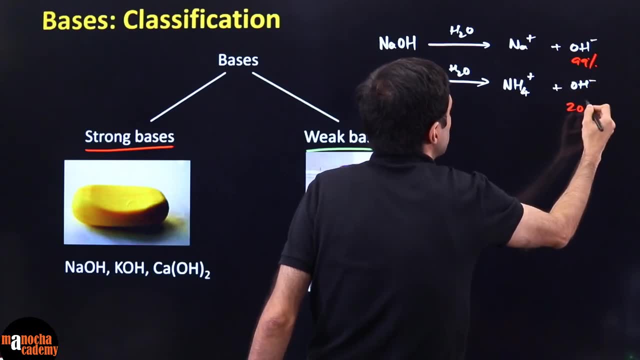 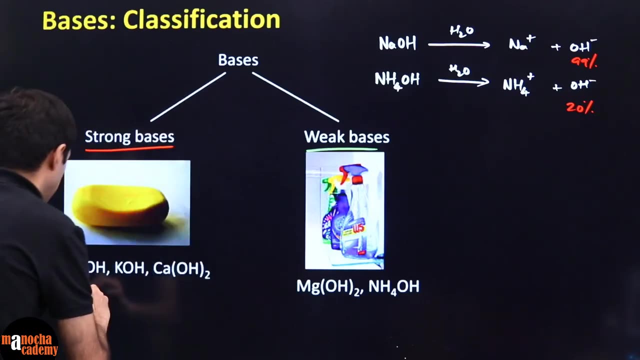 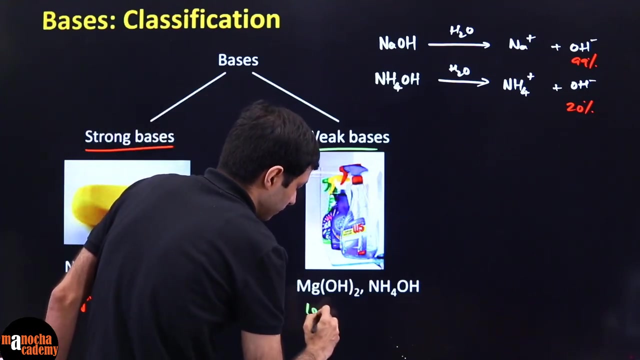 because it will almost again 100% or 99% breakdown so you will get a 99% OH minus here maybe you get only 20% so it is again the degree of dissociation so the important thing here is this will produce a high concentration high concentration of OH minus ions what is the name of OH minus ions guys they are called hydroxyl ions and this will produce a low concentration of OH minus ions so remember again usually we'll be studying about the alkalis alkalis means 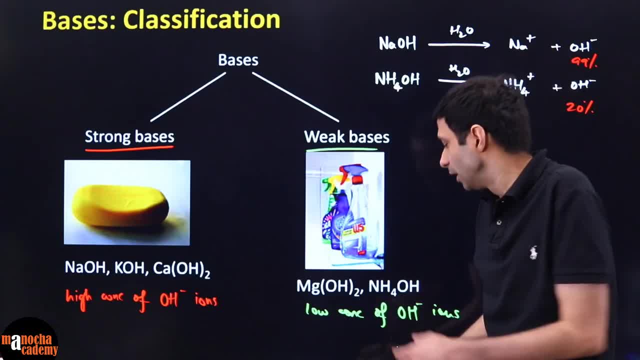 hydroxyl ions are produced by these bases which have been dissolved in water here low concentration for the weak bases here high concentration for the 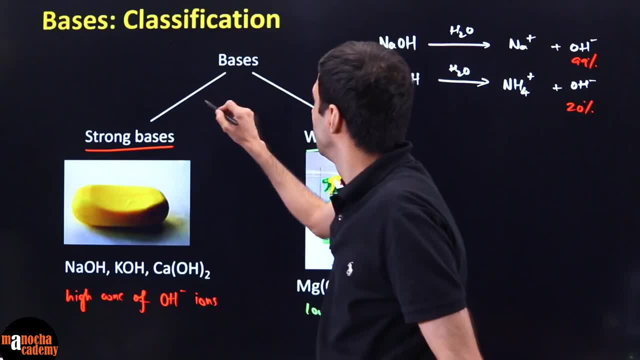 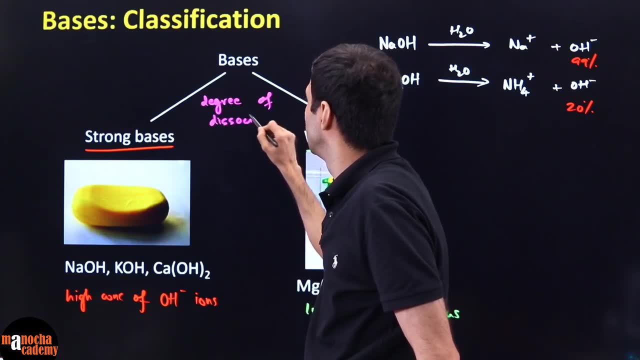 strong bases and it is all related to again it is based on degree of dissociation just like acids it is based on the degree of dissociation how much does it matter 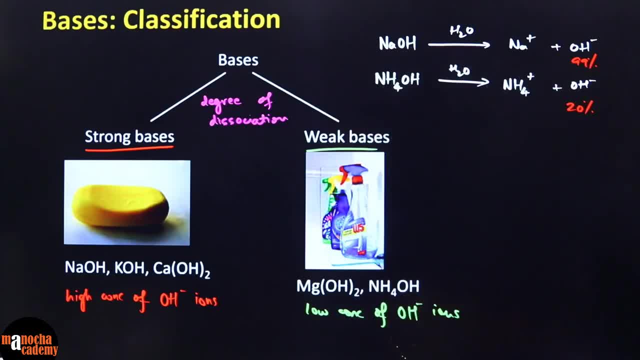 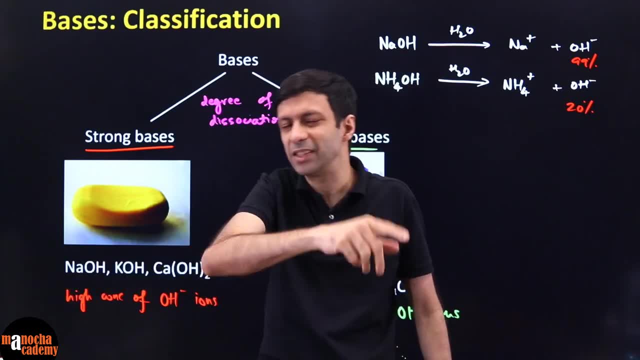 it break down to produce ions very important concept so anytime they ask you this is one trick in the exam anytime they ask you why is this guy strong why is this guy weak whether it's acid or base it basically the answer is 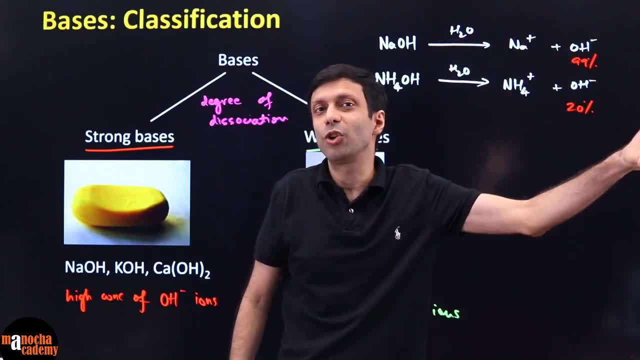 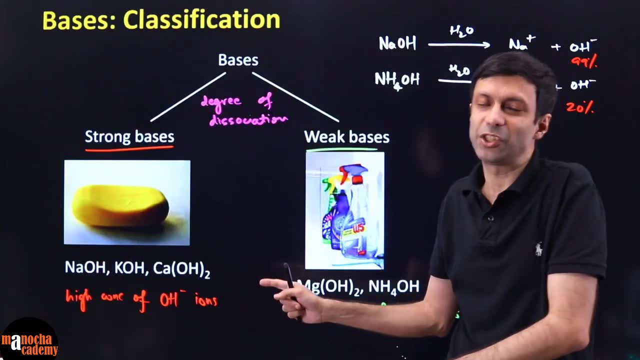 degree of dissociation for acids what will you write high concentration of hydronium or low concentration of hydronium for alkalis what will you write high concentration of hydroxyl or low concentration of hydroxyl ion OH minus 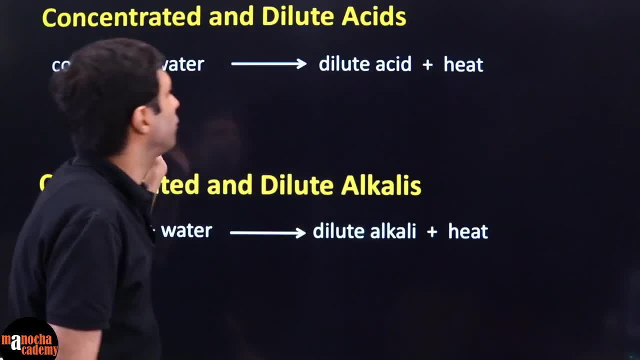 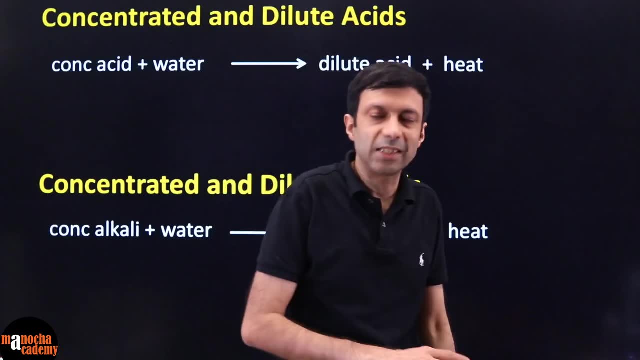 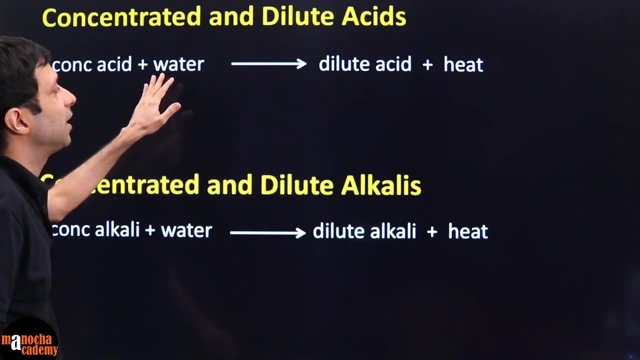 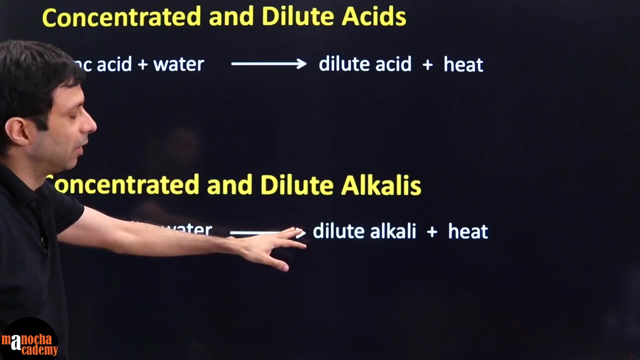 ions now something very simple you might have heard of this concentrated and dilute acid right what is the meaning of concentrated and dilute dilute means there is less acid more water concentrated is the opposite more acid less water right so if you take concentrated acid and you add water you are obviously diluting it similarly if you take concentrated alkalis you add water you are diluting it clear one interesting thing is when you do this 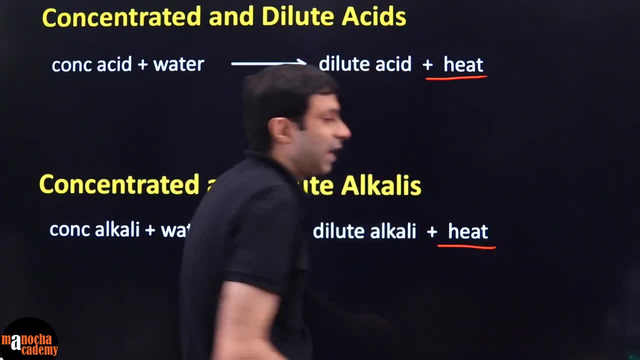 reaction heat is produced a reaction which is produces heat what is it known as can you guys 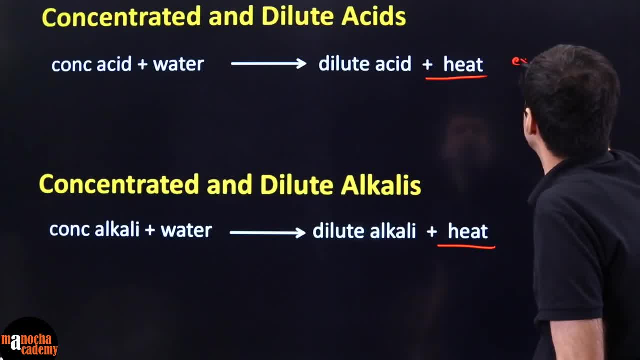 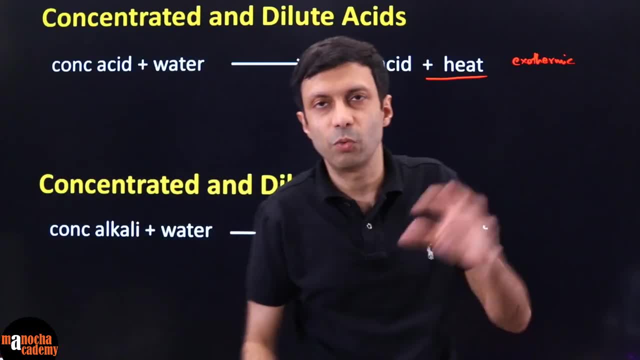 tell me these reactions which produce heat they are called exothermic now why is this so important because this famous question comes when you want to dilute it dilute means when you want to add 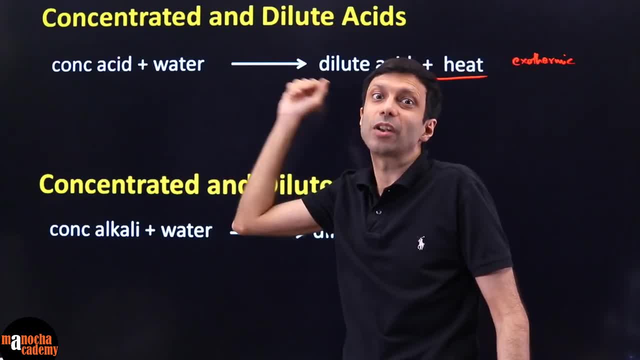 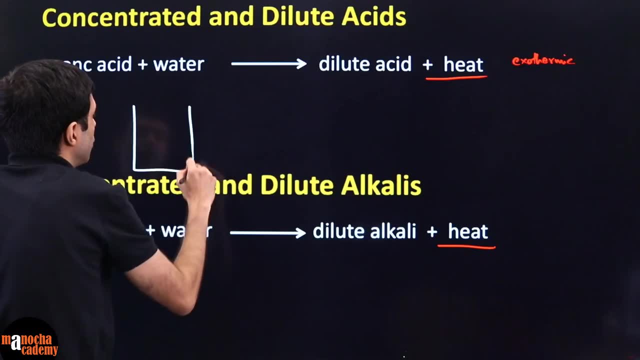 water should you add water to the acid or acid to water this is a very important point when you dilute the acid what should you do so if you have got a container of acid and you say i want to 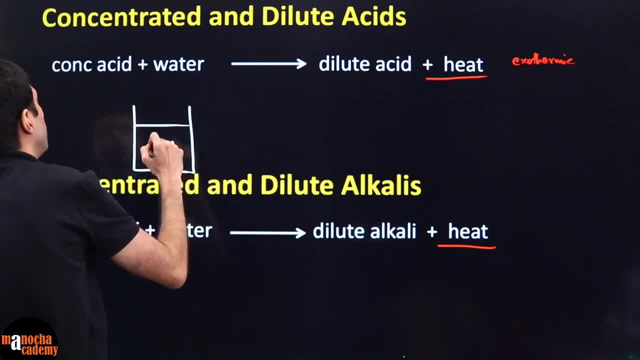 dilute it should you add acid to water or water uh water to the acid what should you do the answer is you should not add water to acid water should be here and you should be pouring in the acid 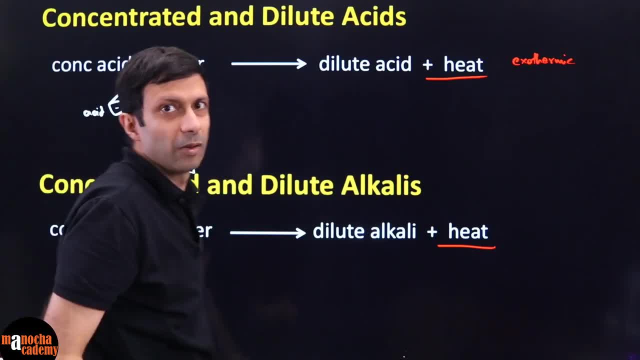 why why this is the case because of this exothermic when you add acid to water it produces a lot of 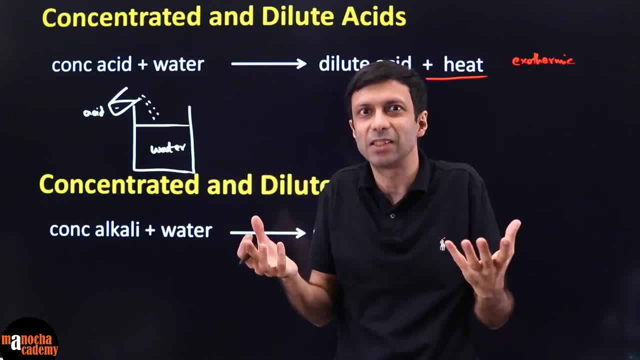 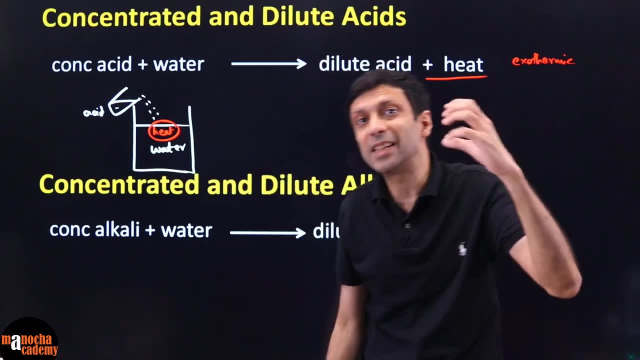 heat right it it sort of makes that sound lot of heat is released so when lot of heat is produced here why you want water to be there because water has high heat capacity it acts as a coolant right 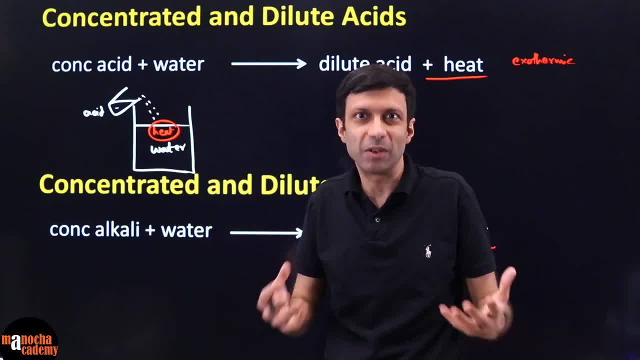 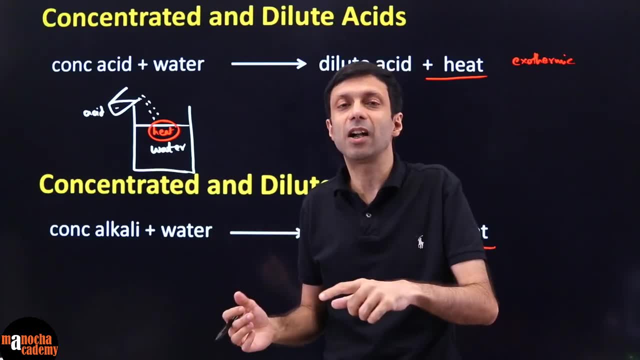 we throw water to make things cool it feels cool in summer it absorbs heat so water has this height capacity it can absorb heat and it can take away the heat but acid can't do that and if you add start adding water to acid what will happen it will heat up and it may spurt on your face right 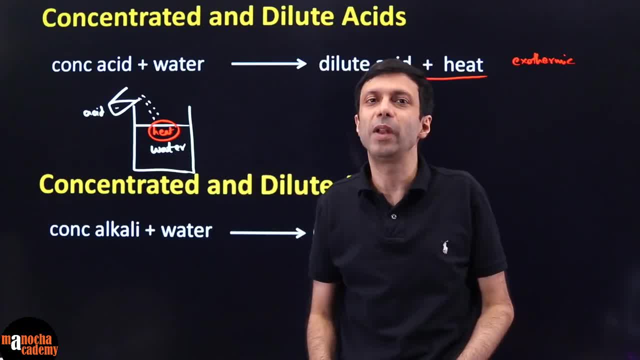 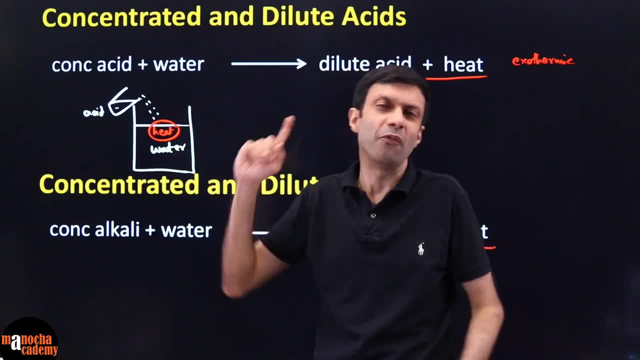 it is highly dangerous so this is where science knowledge comes into play if you are diluting it you will not add water to the acid you will add acid to water very famous question 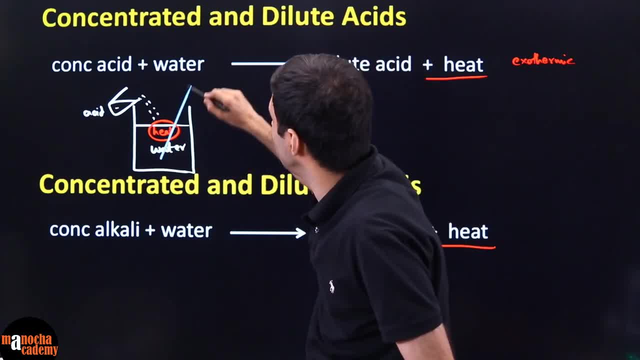 another important point is we should constantly be stirring this why because you are spreading out the heat right you don't want it to be concentrated otherwise 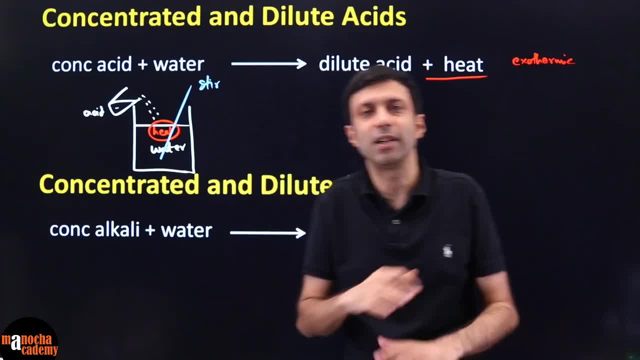 that can also spurt out so you have to mix it and stir constantly to dissipate distribute the heat 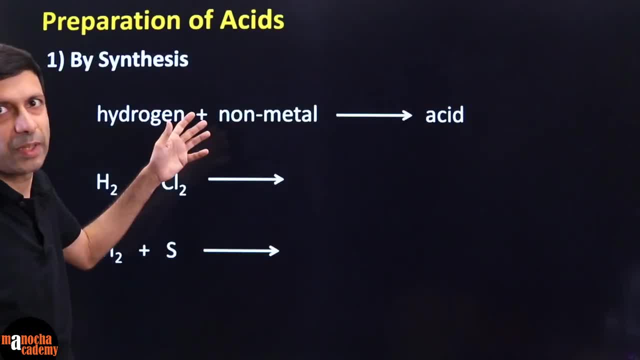 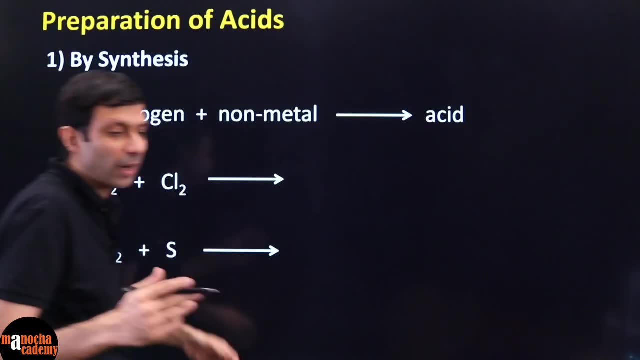 in order to get rid of that name so there's a lot of hydrochloric acid right so the time is very important for your body to be able to absorb that heat and so these are the ten way to go 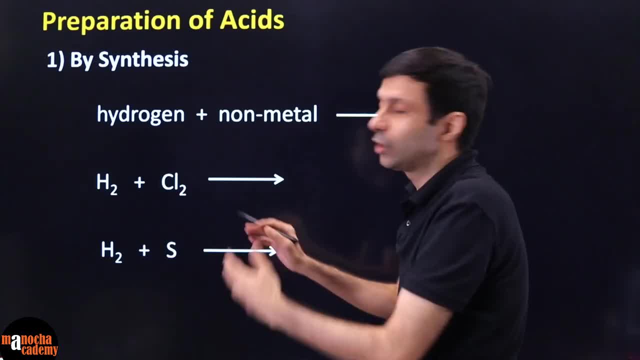 too so we have to add water to the acid right because we want to make the temperature high right and for example if we add a lot of hydrogen to the acid also we can reduce the temperature 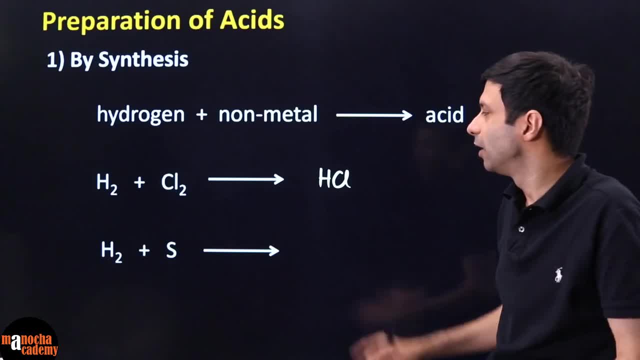 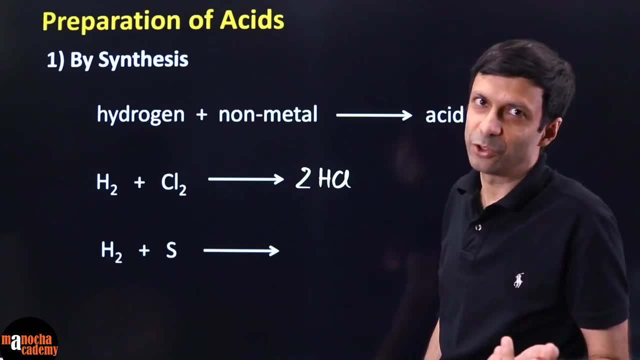 so so let me tell you why we need to add it will bring it back in form or it will produce high levels of hydrogen and it will produce both hydrogen and chlorine in this case if we take these two elements in gaseous form it is called hydrogen chloride hydrogen and sulfur when they 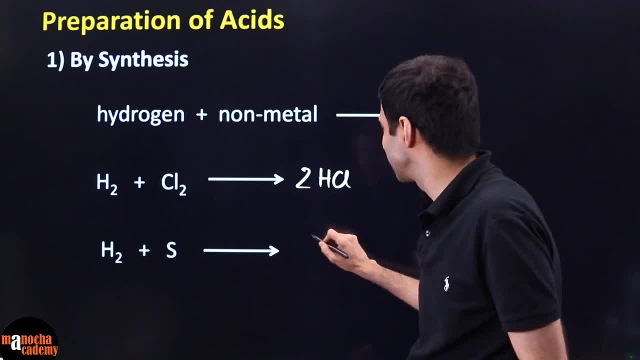 combine what do they form is rotten smelling gas hydrogen sulfide see so 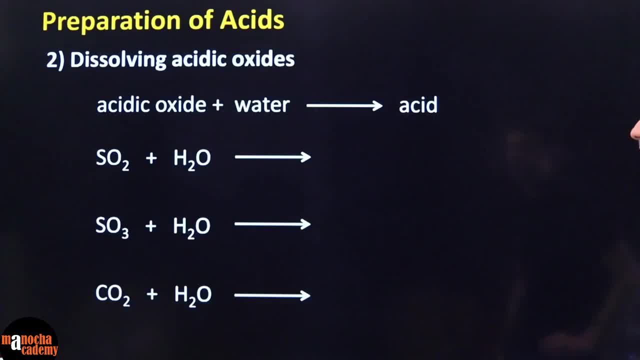 acids can be formed simply by combination reactions you can also form acids by dissolving the acidic oxide in water like if you take sulfur dioxide 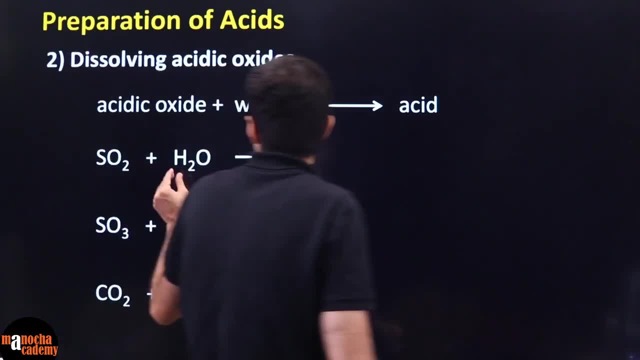 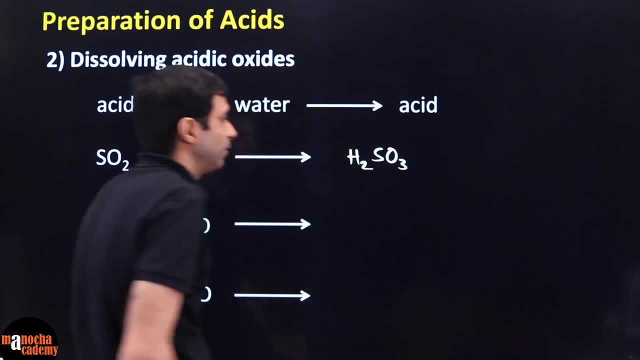 and water what will you get you can predict it just combine it so let me copy this H2 there will be sulfur how many oxygens 2 plus 1 3 H2SO3 do you 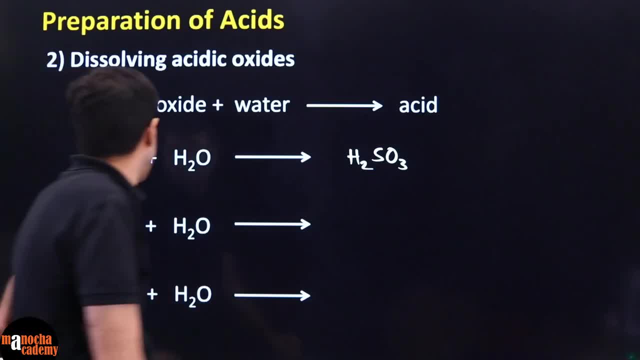 guys know the name of this acid let's finish this equations and you guys tell me the name if you take sulfur trioxide and water again play Lego just combine 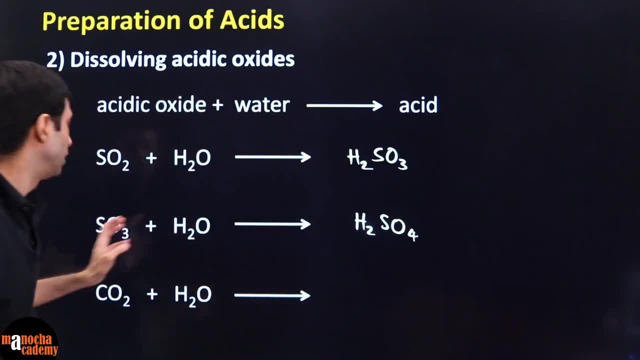 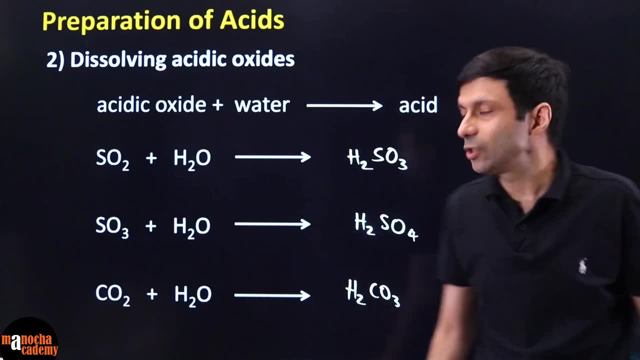 it H2SO4 see just join the atoms 3 plus 1 4 oxygen carbon dioxide plus water again just join it H2CO3 do you guys know the name of these acids this one 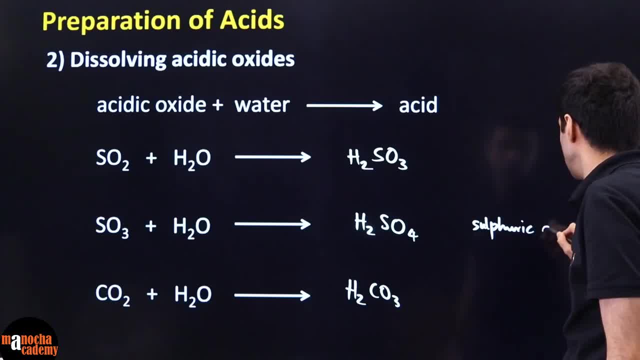 you know I think H2SO4 is called sulfuric acid this one we just talked about H2CO3 which is found in your aerated drinks sodas this is called carbonic acid right what about the first one H2SO3 what is 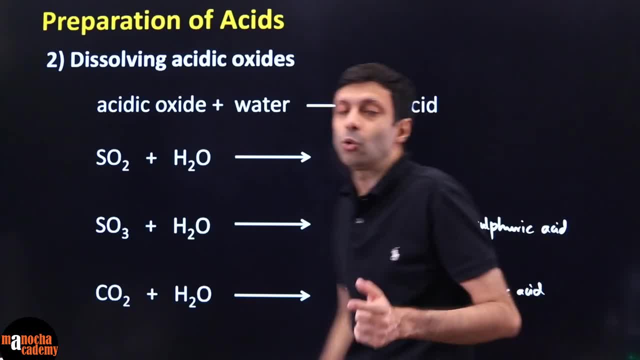 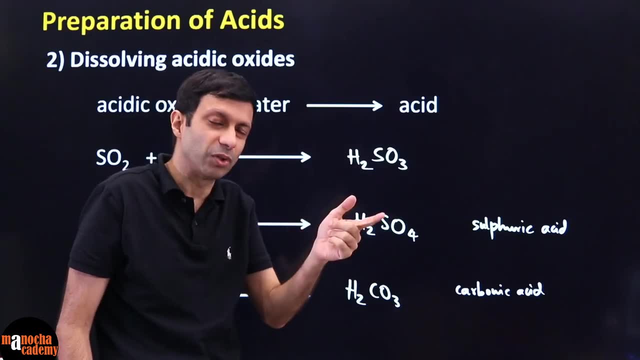 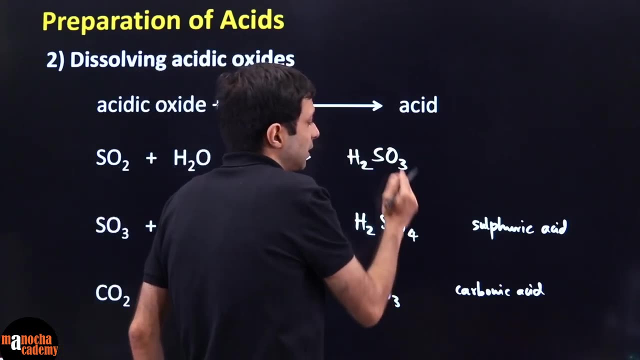 the name of this who can tell me the name of the first one so in chemistry the rule is ick means more oxygen us means less like phosphoric phosphorus we saw that H3PO4 H3PO3 us is less oxygen ick is higher just like valency ferrous ferric right so less oxygen atoms because this has four this has 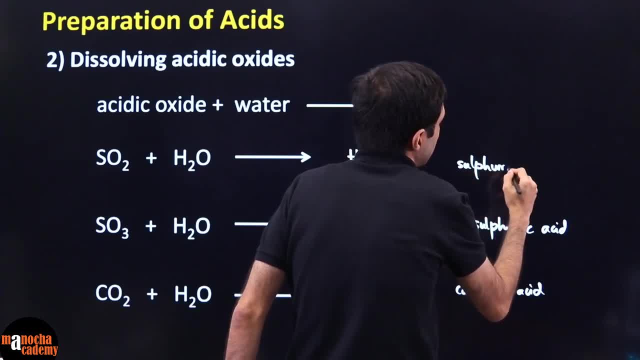 three this will be called sulfurous acid so remember all these interesting tricks right that will help 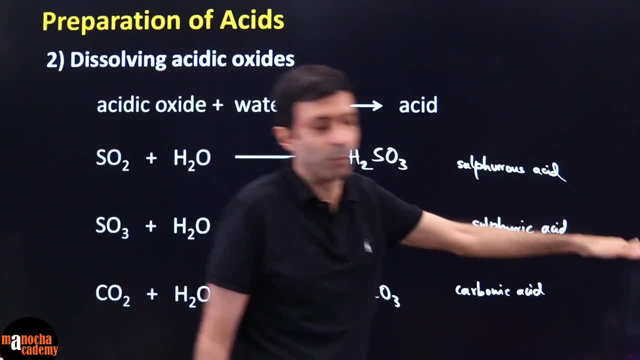 you remember it you're not memorizing us means less ick means more similarly can you guys try this one P2O5 plus water what will I get phosphorus pentoxide 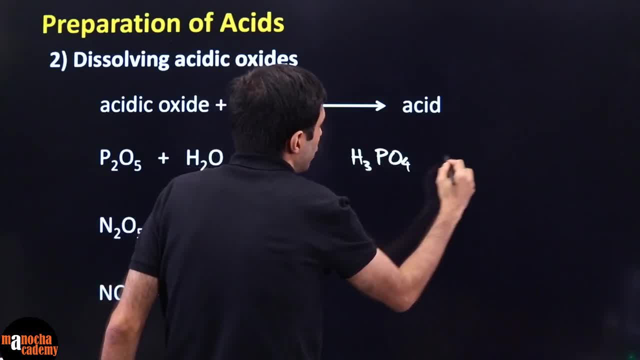 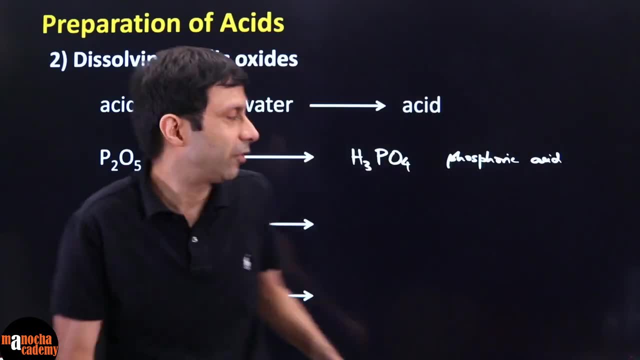 plus water I will get H3PO4 phosphoric acid can you guys balance this equation for me so how can you quickly balance again do the heat and trial 2 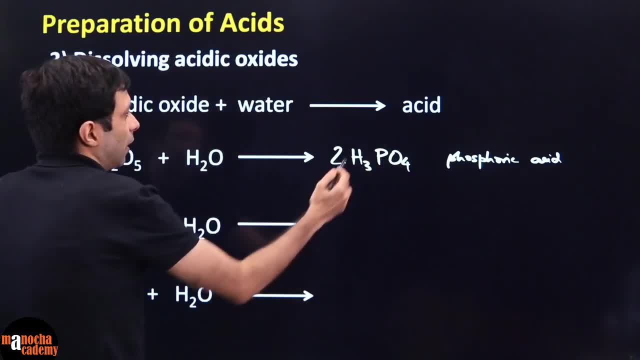 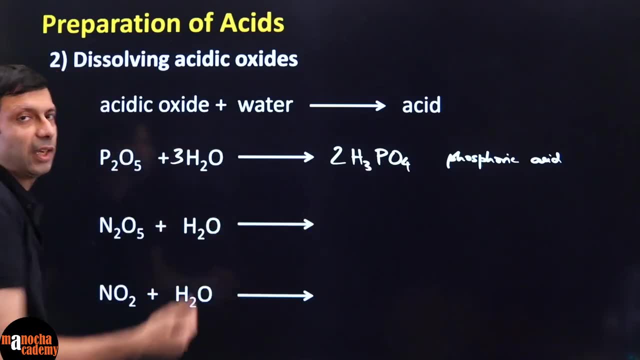 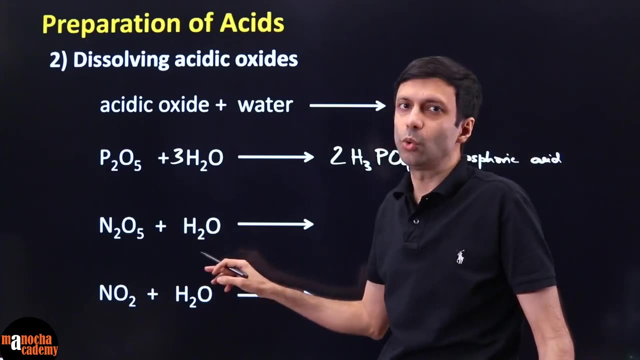 phosphorus 1 phosphorus let's multiply by 2 phosphorus is done hydrogen 3 times 2 6 I'll multiply by 3 yeah hydrogen done oxygen how much 4 times 2 8 5 plus 3 8 done so always try to balance the easy elements first next one in n2o5 plus H2O 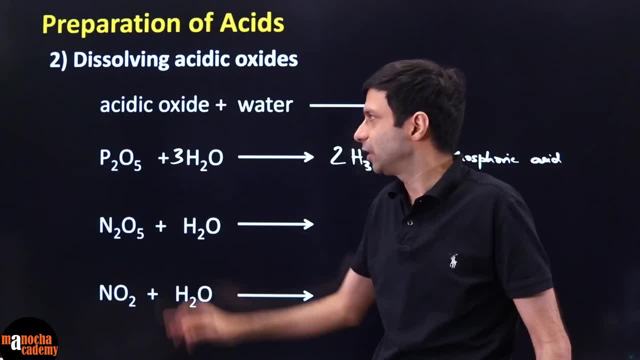 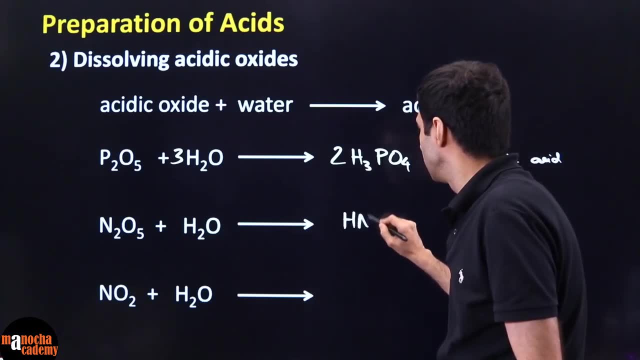 n2o5 is what nitrogen pentoxide just like phosphorus pentoxide do you guys know what will be the answer here so this one will form your nitric acid HNO3 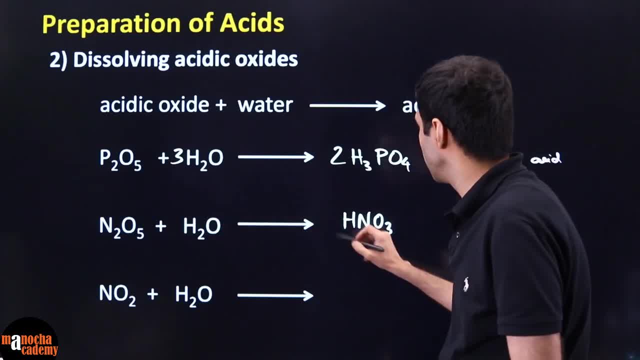 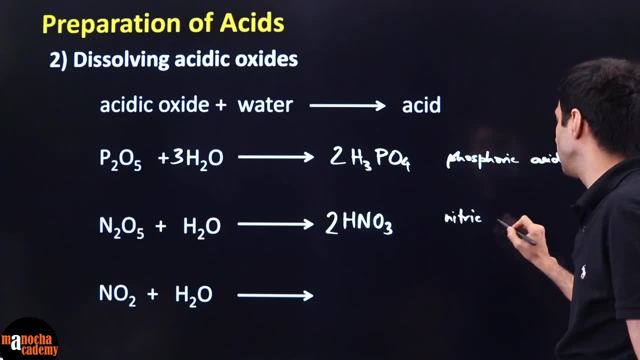 again balance it so you can see 2 nitrogen there's 1 nitrogen here if you multiply by two i think that should balance it out no3 is nothing but hno3 is nitric acid 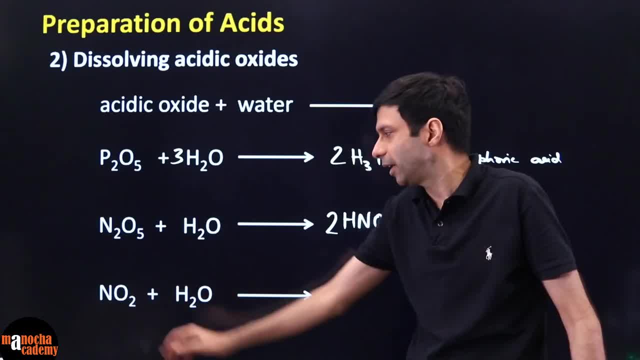 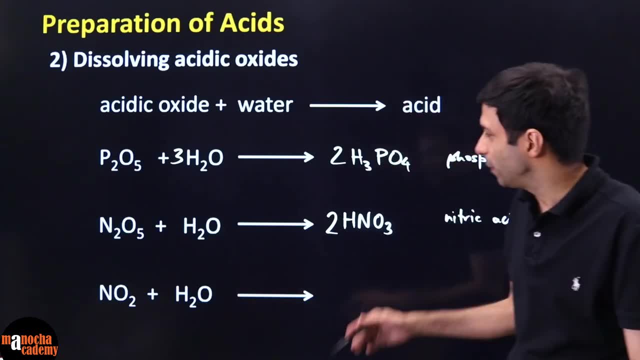 the last one is very interesting no2 just like co2 carbon dioxide no2 is called nitrogen dioxide this is a reddish brown gas when you dissolve it in water what does it form you might be thinking 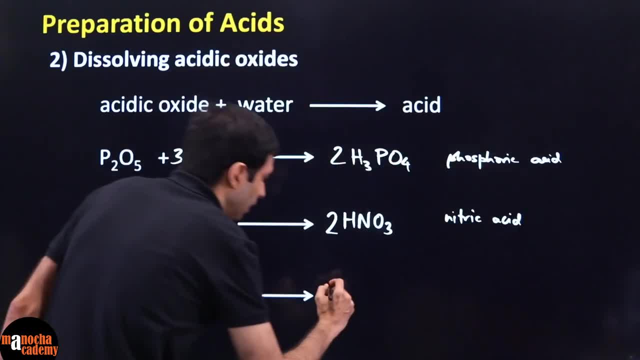 okay again the same nitric acid right you might be thinking hey it's going to form hno3 again 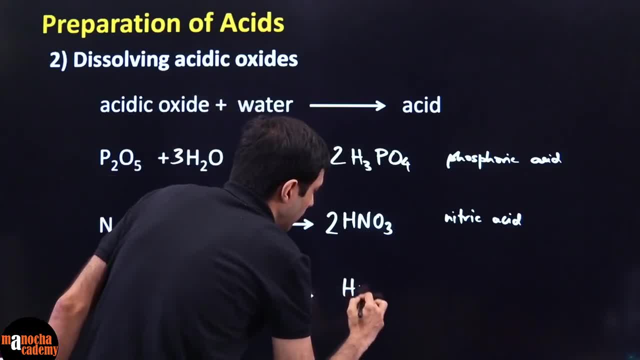 but this is very interesting it actually forms two acids hno3 and hno2 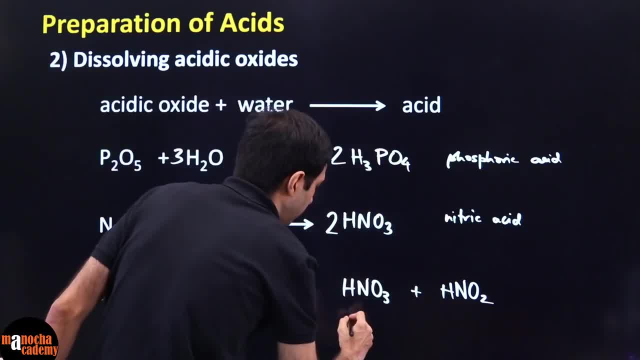 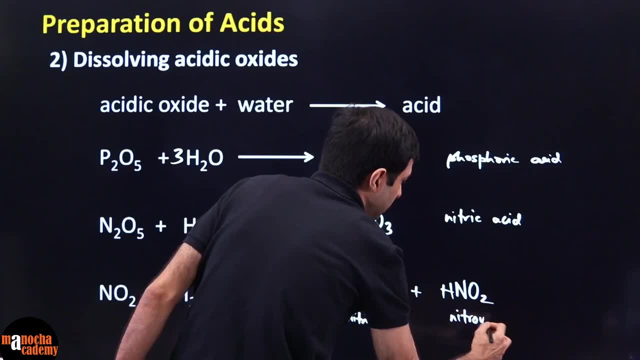 can you guys give me the name of these acids this one we just said this is nitric acid this one now you can guess the name one oxygen i took away so it should be called nitrous acid less 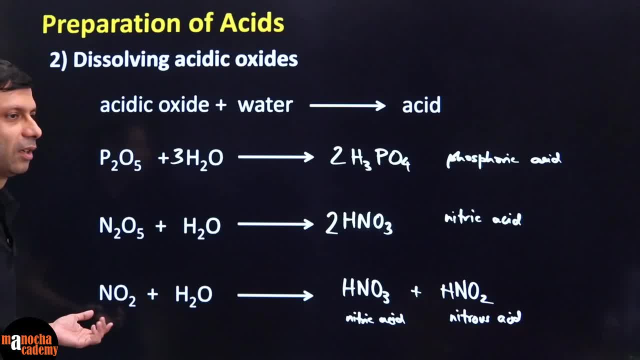 oxygen that is why this is called it is called a mixed anhydride there is another term here these guys on the left 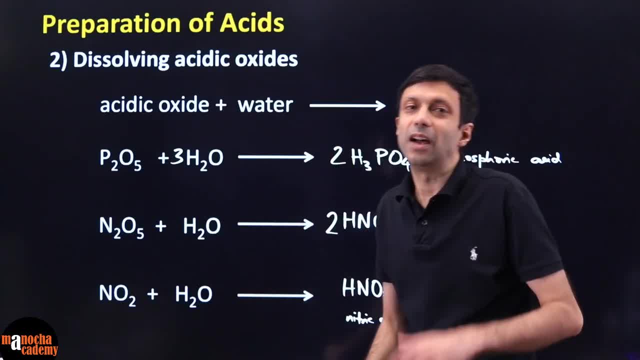 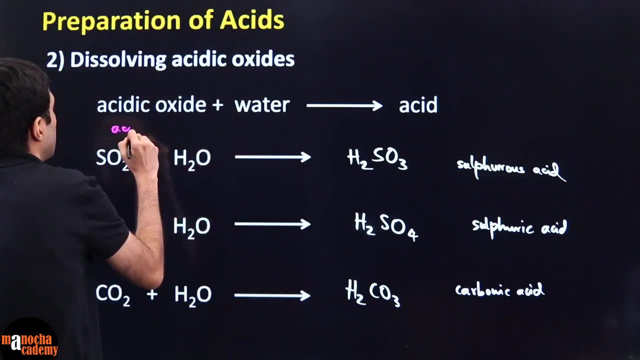 these guys are called acid anhydrides the acidic oxides that you dissolve in water these are called there is a term here these are called acid anhydride why because when you add water you get the acid or you say you remove water you get the anhydride anhydride 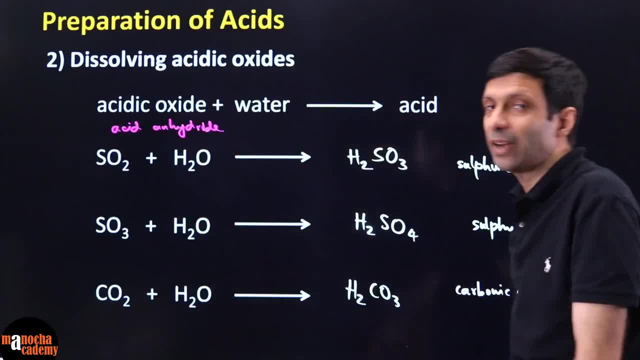 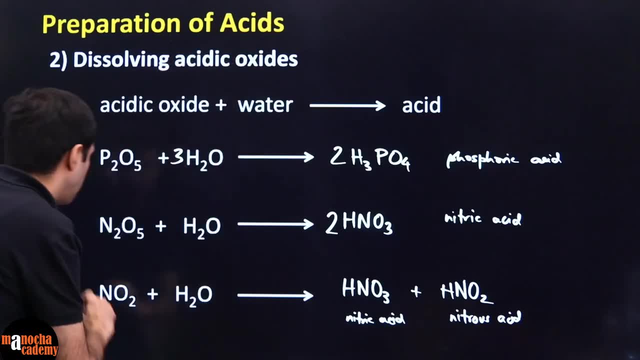 you have taken away the water so these are all called acid anhydrides they are used when you dissolve it in water it produces the acid this guy is special he is called a mixed anhydride and you can guess now why why is nitrogen dioxide a mixed anhydride because it 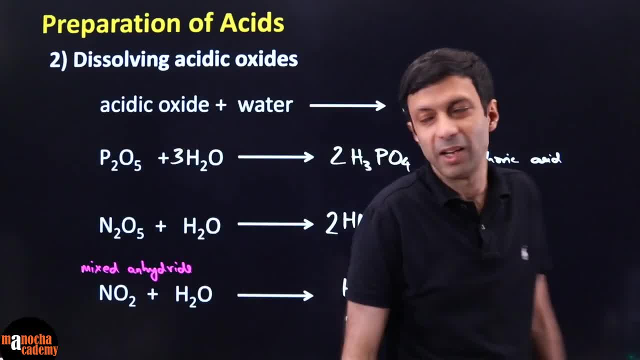 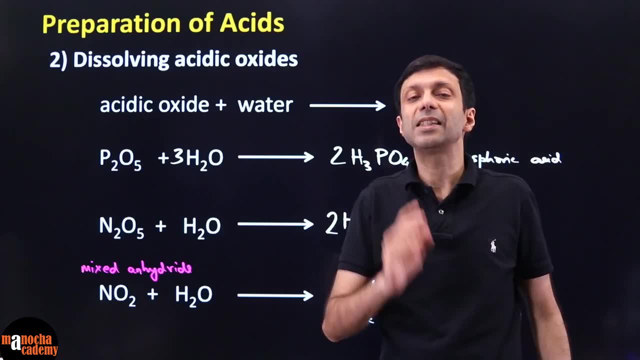 produces a mixture of two acids not one acid it produces two acids so similarly a question can come to you can be asked this question who is the acid anhydride of nitric acid can you guys tell me 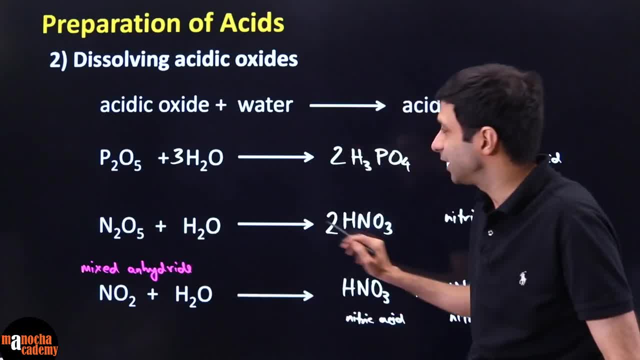 based on this slide so the acid anhydride of nitric acid is n205 not no2 not no2 guys because see 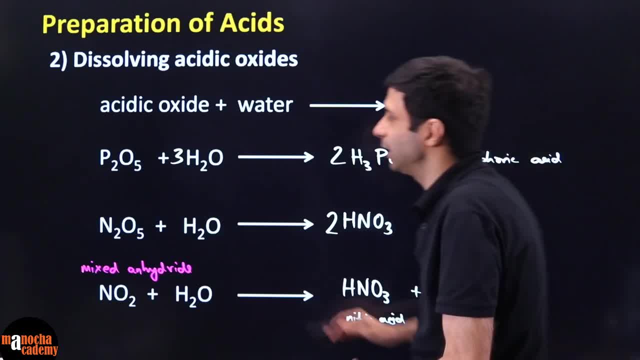 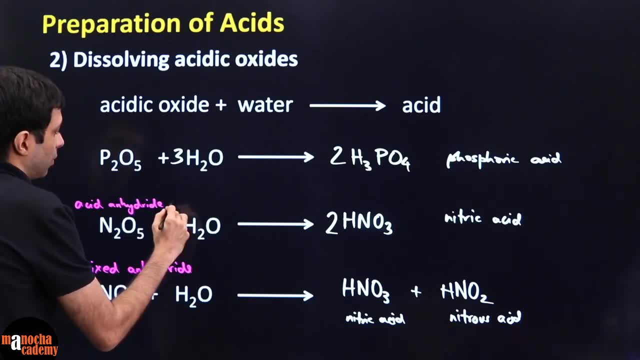 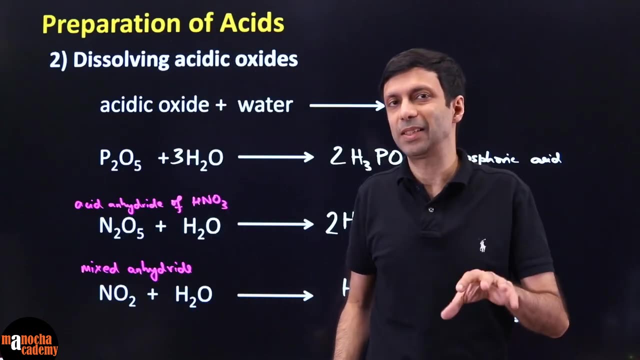 it gives a mixture of two acids so this is the acid anhydride so n205 is the acid anhydride of hno3 so this is another important concept you have learned acid anhydride means when you mix 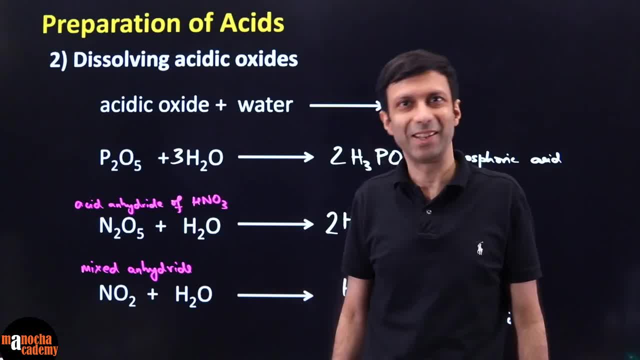 that substance with water it will produce the acid for you clear now another way you can prepare 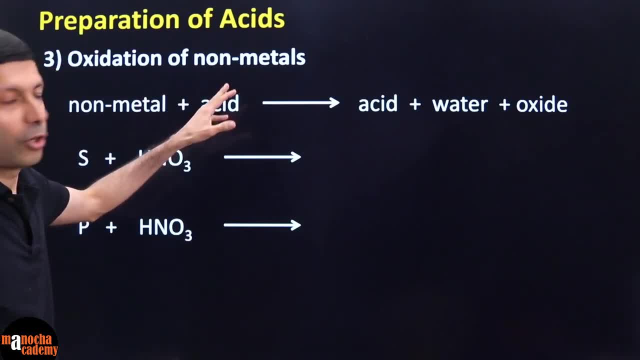 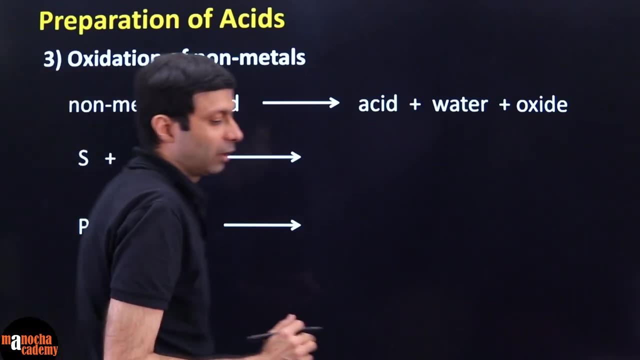 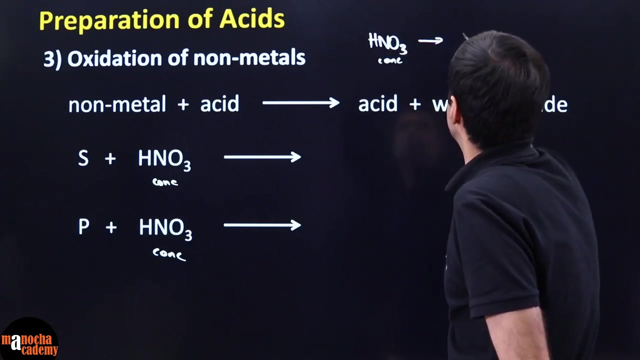 acids is by oxidation of the non-metals how do you do that by using a acid which is a strong oxidizing agent like nitric acid so let's say you take sulfur and concentrated nitric acid or phosphorus and concentrated nitric acid so here what is the trick over here that nitric acid actually if you take concentrated nitric acid it breaks down to give you h2o no2 and nascent oxygen 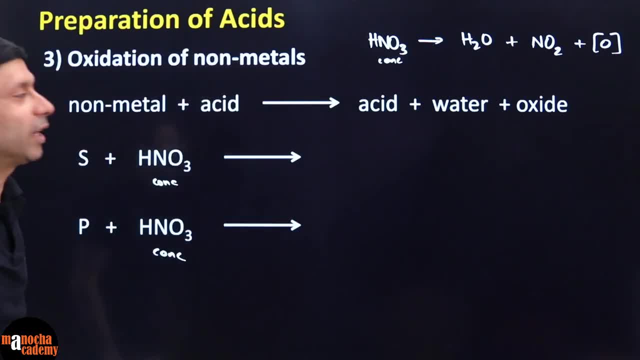 okay that's what concentrated nitric acid does if you take dilute nitric acid that also gives you h2o and nascent oxygen okay so what happens here if you take self sulfur and concentrated nitric acid 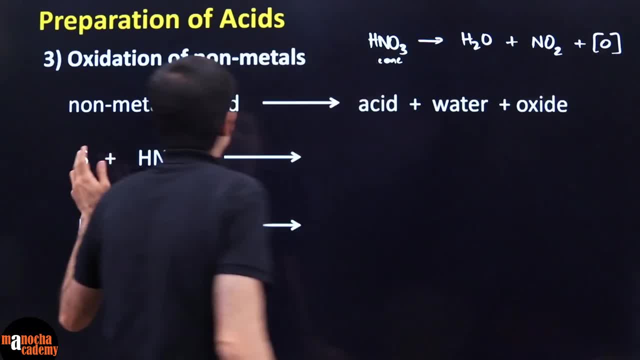 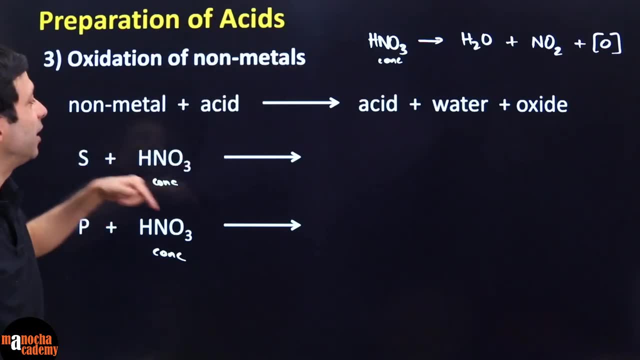 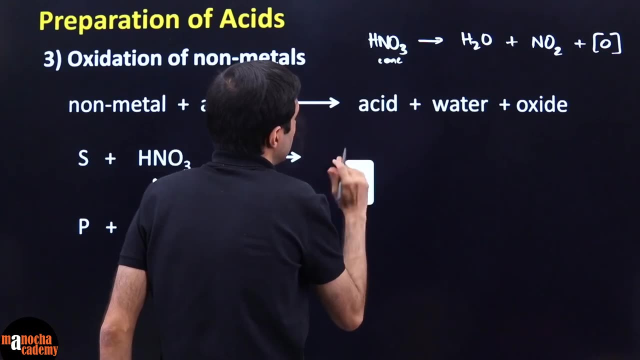 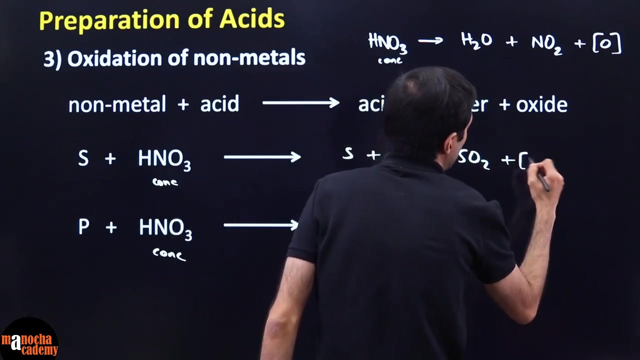 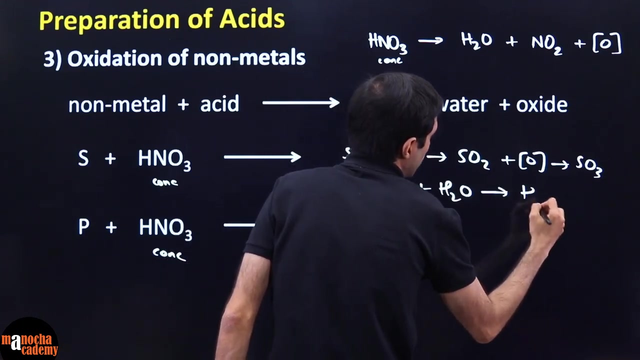 it's going to this nascent oxygen is going to attack sulfur and make it sulfur dioxide then sulfur dioxide will again be attacked by nascent oxygen it will become sulfur trioxide then it will dissolve in the water right and become sulfuric acid so finally what you'll be getting over here so basically the steps will be sulfur plus nascent oxygen will give you sulfur dioxide then you add nascent oxygen to that you'll get sulfur trioxide and then sulfur trioxide plus water will give you sulfuric acid h2so4 so this is what's going to happen okay so finally the 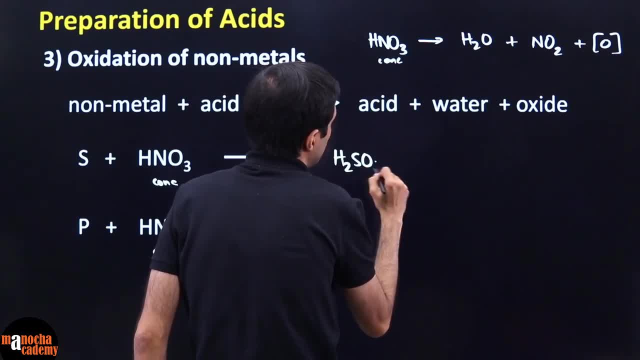 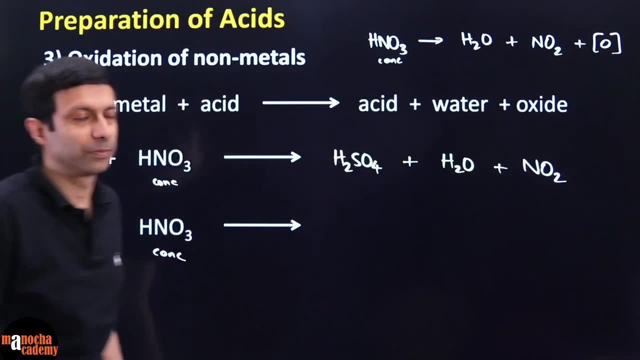 acid that we are going to be left with here is sulfuric acid h2so4 plus water plus nitrogen dioxide no2 okay so this is what sulfur nitric concentrated nitric acid does you get 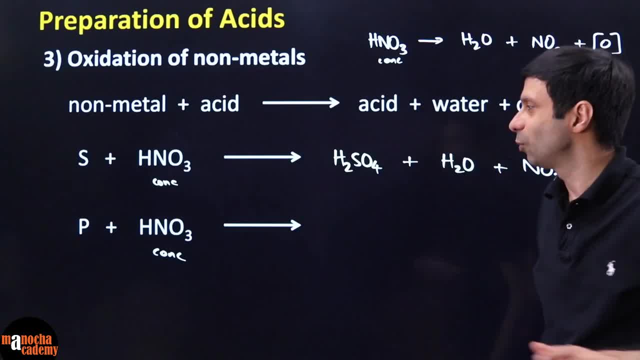 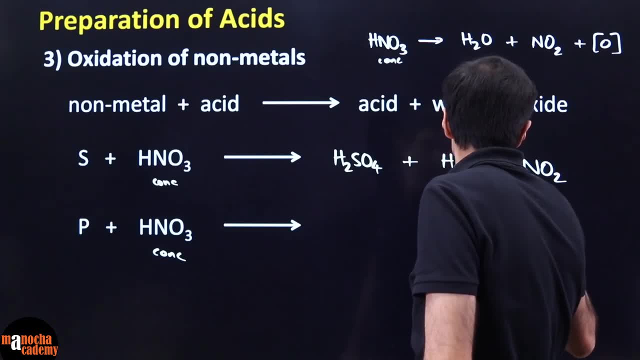 how do you when you react with phosphorus and concentrated nitric acid what do you think we're going to get we are going to get again water and no2 and the acid formed here any gases 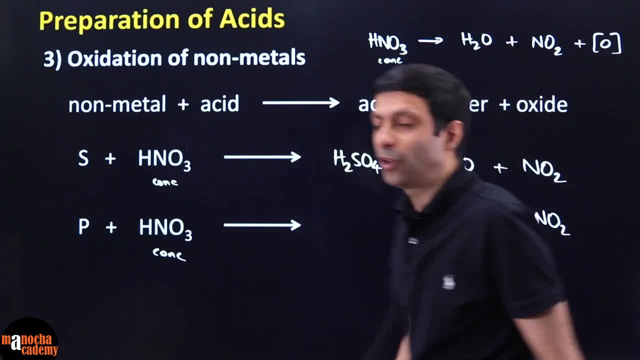 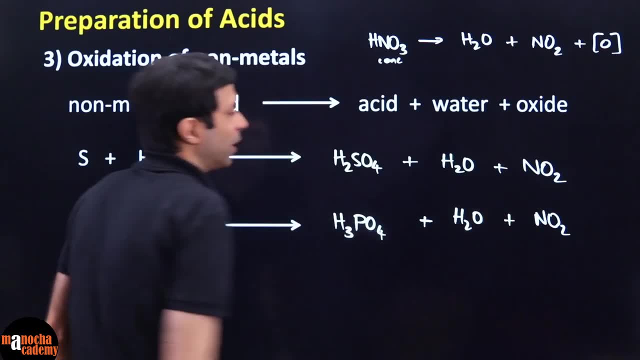 what is the acid going to be formed here it's going to be phosphoric acid h3po4 so what you're going to end up over here is h3po4 phosphoric acid plus water plus no2 again i'm not balancing 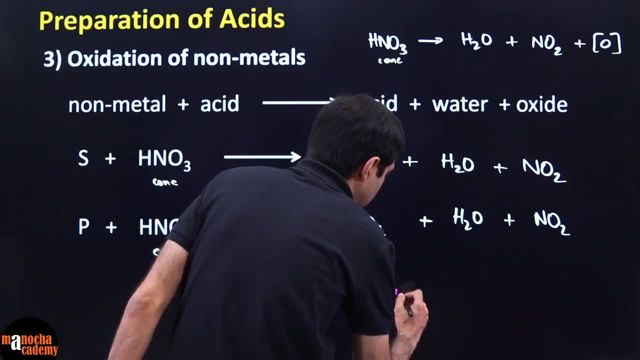 these equations i'm leaving them unbalanced you guys can practice the balancing of it 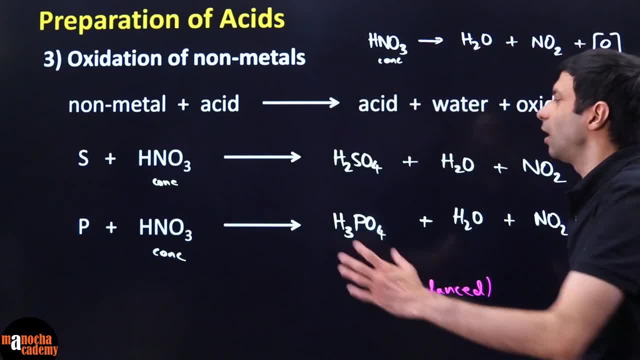 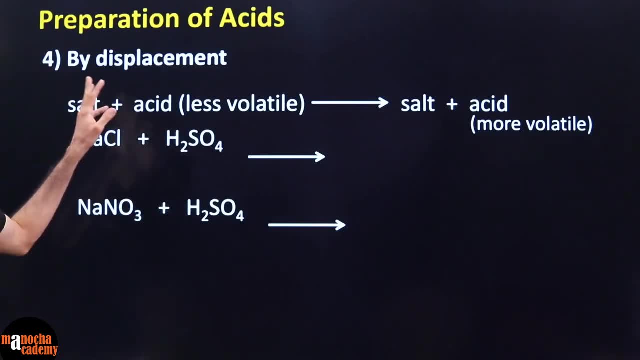 because our goal right now is to predict and learn how how we can write these reactions another way to prepare acid is by displacement of the salts okay so by doing the you take a 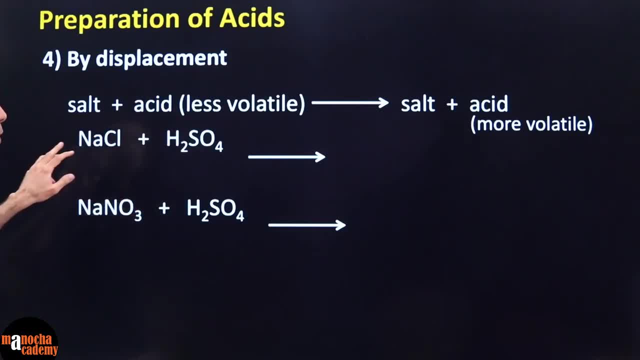 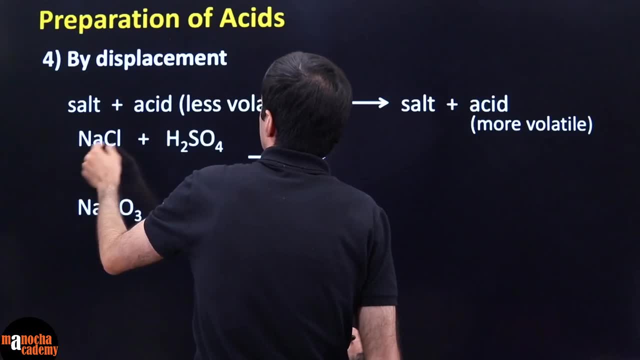 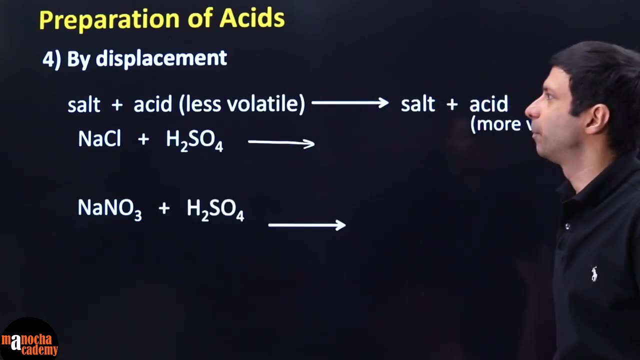 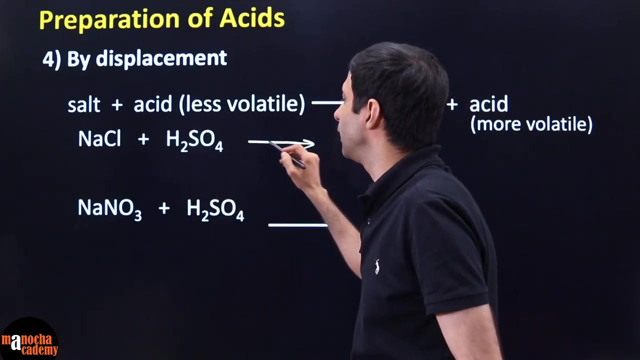 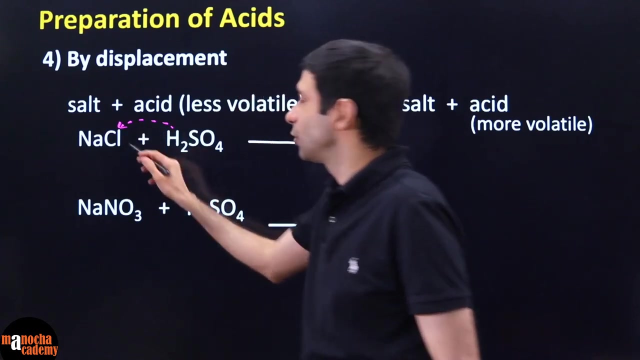 salt and you take a acid which is less volatile like for example if you take sodium chloride and sulfuric acid okay what will it give you so what's going to happen over here the hydrogen is going to be displaced from this by the way this arrow is very low this is another way to prepare let's say you want to prepare hydrochloric acid so what do you do you take sodium chloride and sulfuric acid and then you heat it so what's going to happen in this the displacement will be one of the hydrogen is going to go to chlorine and that is going to 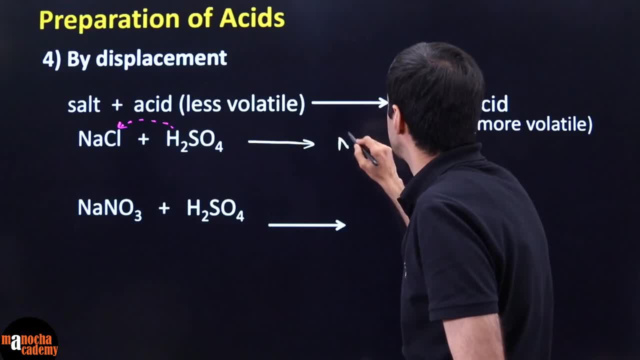 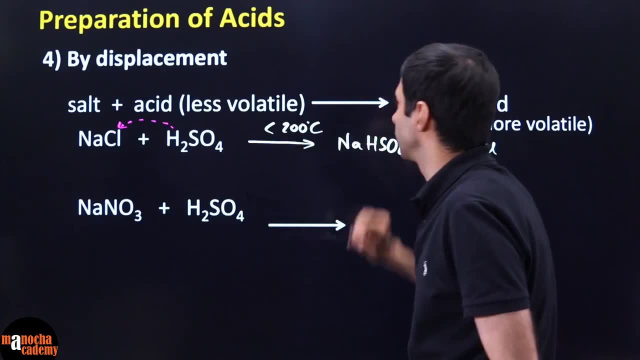 give you hcl and the remaining you're going to be left with is sodium bisulfate plus hc this is if you do the reaction at less than 200 degrees celsius if you do the reaction at more than 200 degrees Celsius, then all the hydrogen will go away, you will get sodium sulfate plus HCl. 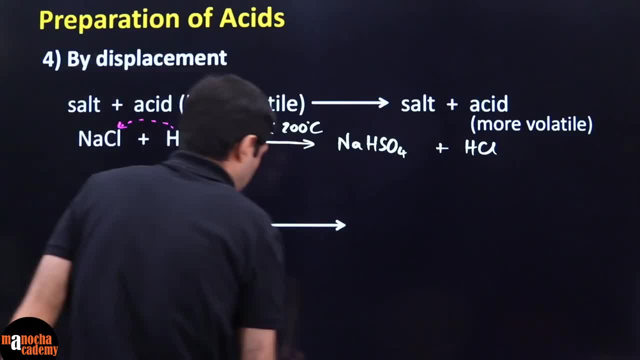 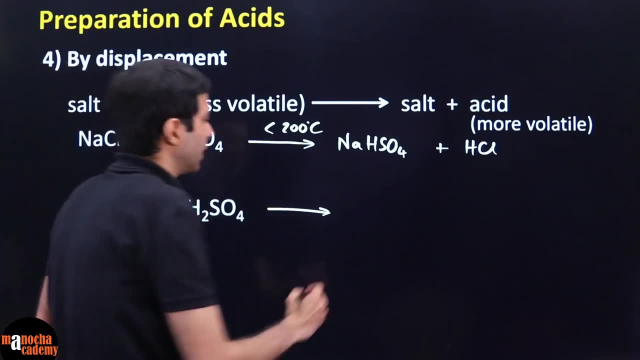 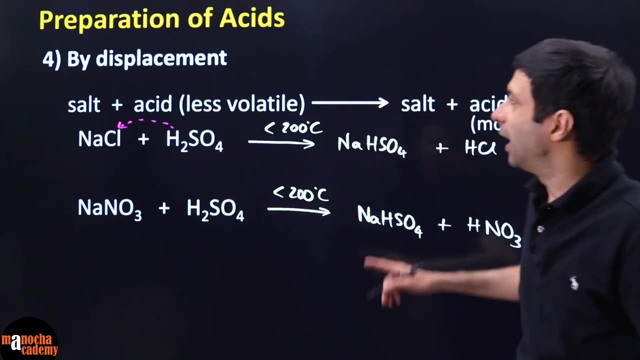 Similarly, over here, sodium nitrate and H2SO4. So, this is going to end up giving you again sodium bisulfate plus nitric acid. Clear? Clear? So, this is the displacement going on where one hydrogen is getting used up, is getting, you know, shifted from sulfuric acid to nitric 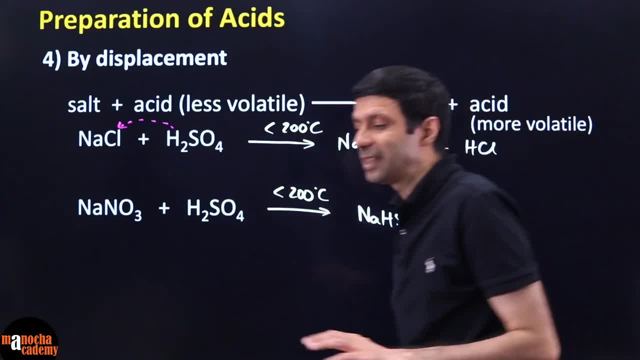 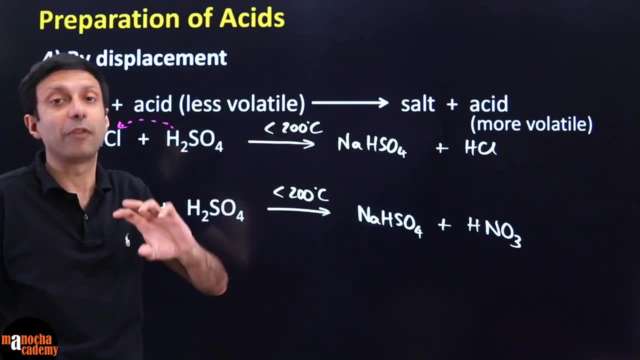 acid. And here we say typically we use sulfuric acid because it is less volatile. What is the meaning of the word less volatile? It does not change easily from liquid to gaseous state, right? Like perfumes are very volatile. They'll easily, if you open the perfume bottle, it will easily change from liquid to gas or petrol, very volatile. But usually when we are preparing a less volatile acid, a more volatile acid, we use a less volatile acid because otherwise if you heat it and if all the sulfuric acid escapes as a gas, then there is no use. 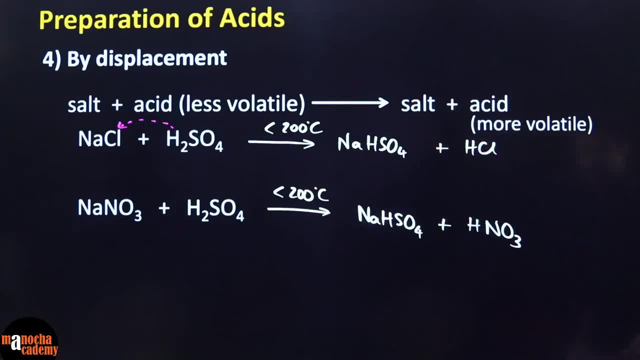 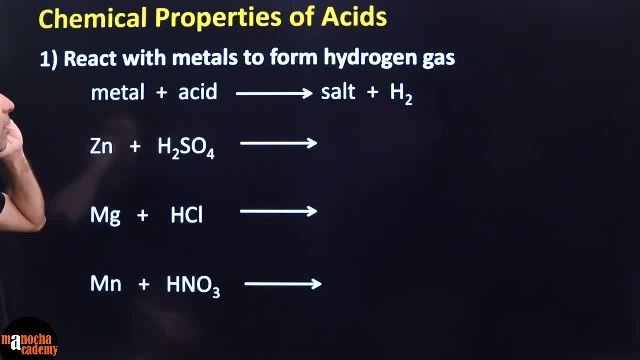 The reaction will not occur. Okay? So, this is another way to prepare acids. The other very important way to prepare acid is by using a metal plus an acid, right? Oh, 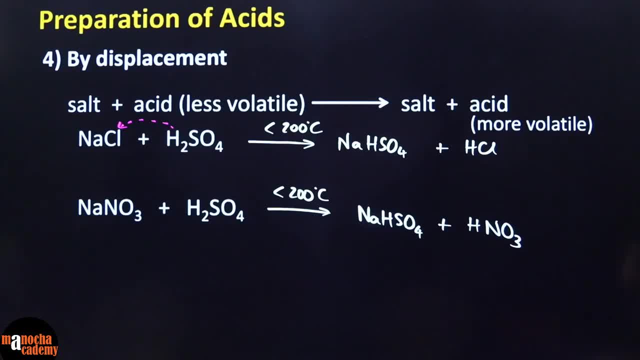 so here we have done. So, this was till the preparation of acids. Now, we are going to go to the reactions, right? Do we need to memorize the word equation? The word equation helps you 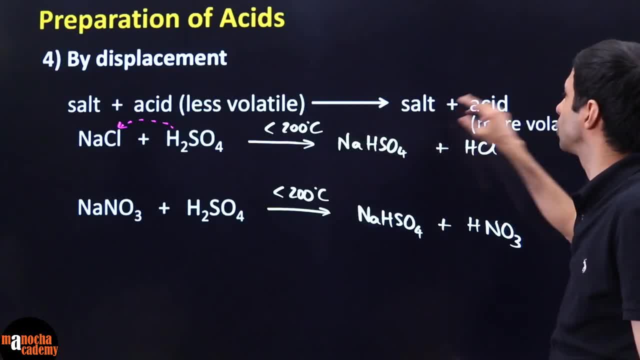 see the pattern. Salt plus less volatile acid will give you the salt plus the more volatile. You do not have to memorize this. It helps you actually to remember. 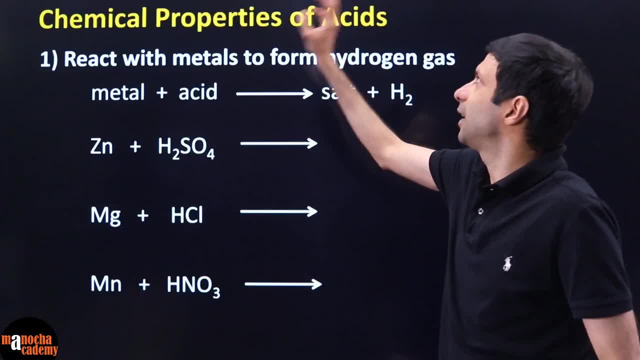 What is the reaction given? Now, next, let's proceed to the chemical properties of the acids. 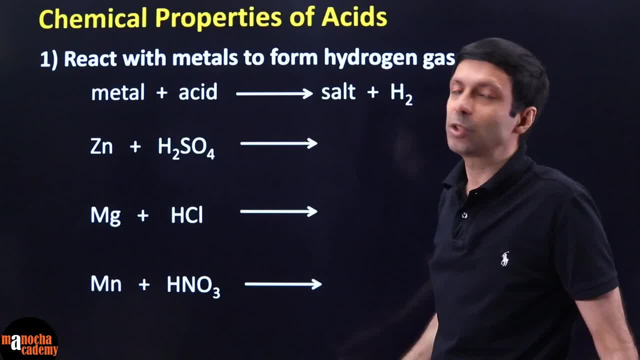 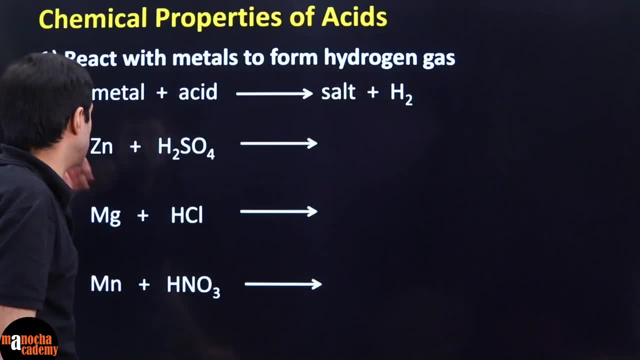 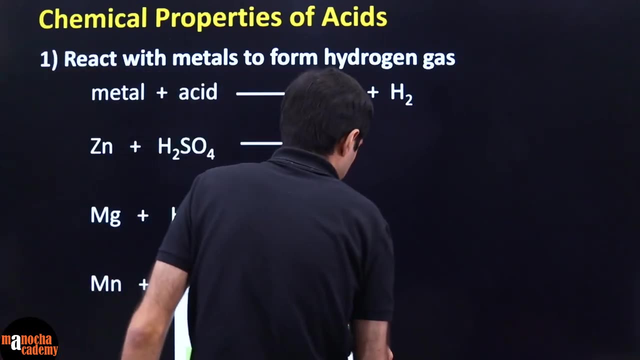 Chemical properties basically means chemical reactions. So, the first and very famous one that we are going to look at is reaction of metals with the acid. So, if you take a metal like, let's say, zinc, magnesium, manganese, right? What will be the reaction with the acid? So, let's say you take zinc and sulfuric acid. What is that going to do? Zinc is more reactive than 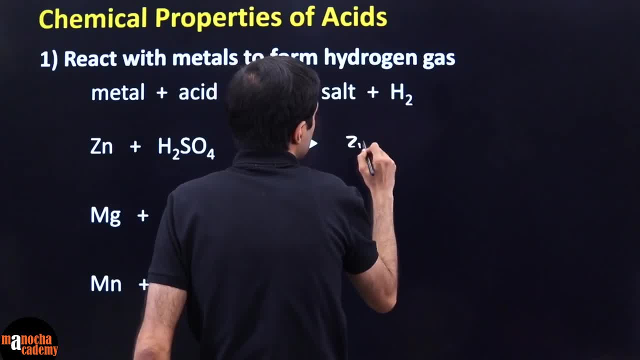 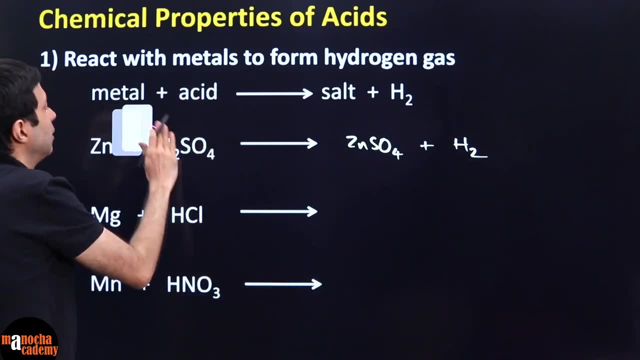 hydrogen. So, it's going to displace it. So, what salt will we get? Zinc sulfate plus hydrogen. Simple. All of you can see what is happening. Zinc is kicking out the hydrogen over here. So, what type of reaction is this? These are all basically displacement 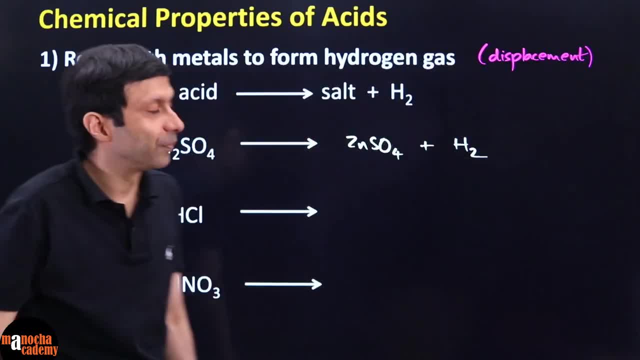 reaction or single displacement. Do you guys agree? So, this is the reaction. The next one, 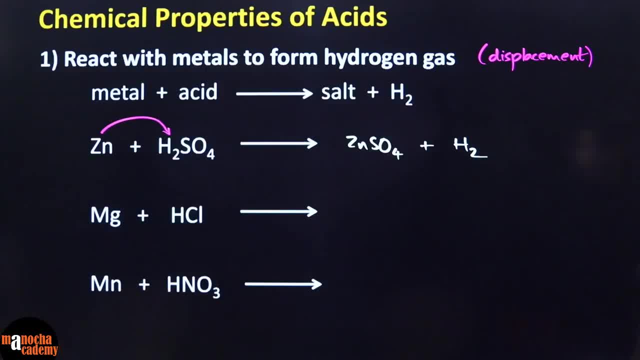 can you tell me? Magnesium plus HCl. Can you guys predict this for me? Magnesium plus HCl. 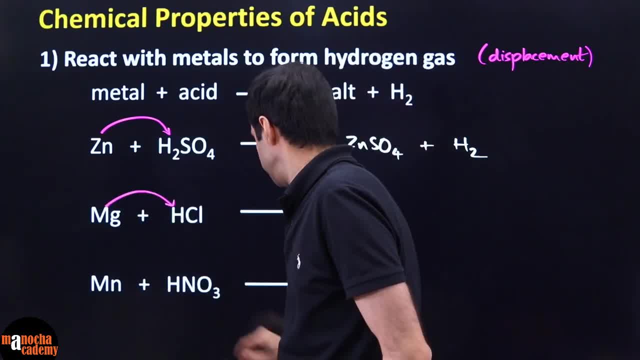 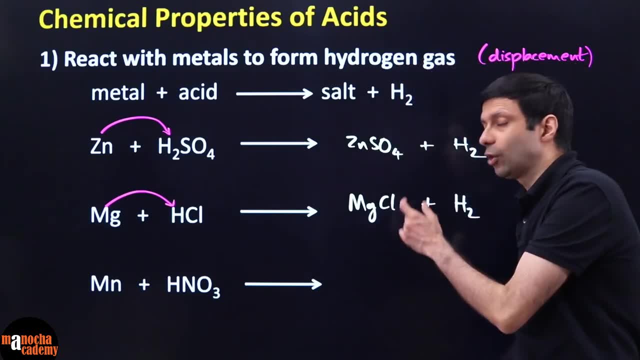 Again, the same thing. Magnesium is going to kick out hydrogen here. And will it give me this? Is this the reaction? MgCl plus H2? No. Whenever you are writing formulas, you have to use the 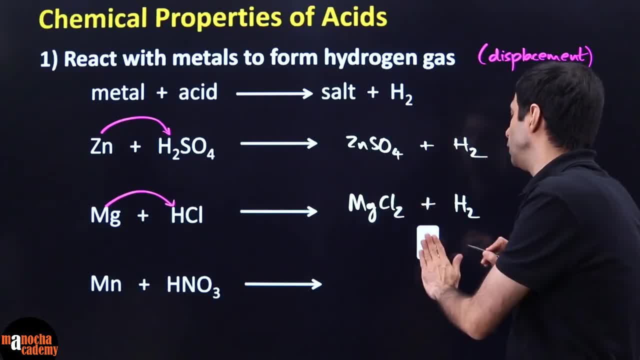 valency. Magnesium has valency 2. So, it will be MgCl2 plus H2. And again, you should balance 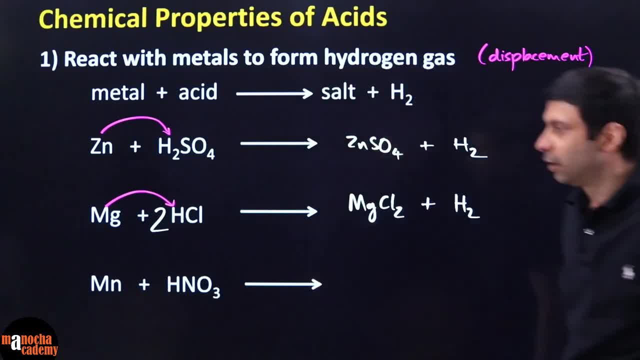 your equation. So, this one is simple to balance. 2HCl. Next one, manganese plus nitric acid. So, 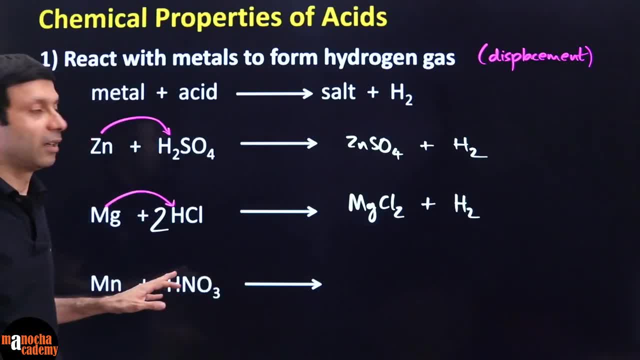 nitric acid is a strong oxidizing agent. So, usually it does not end up giving hydrogen. 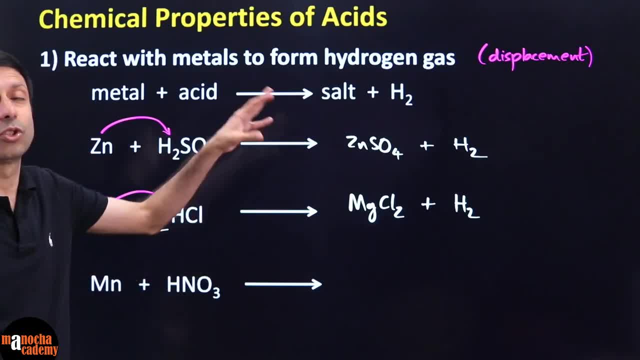 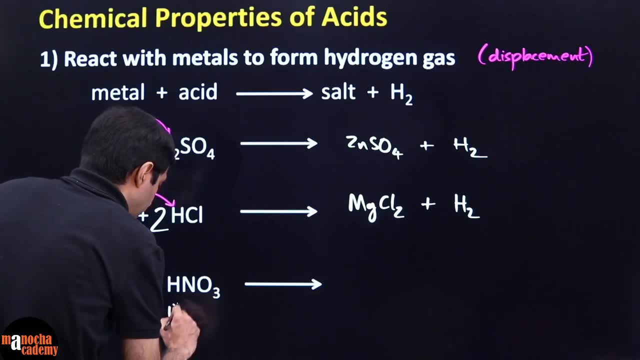 It usually ends up giving, you know, magnesium, nitrate, water and those nitrogen oxides like we mentioned. So, with magnesium and manganese, if you take 1%, very dilute, dilute and cold nitric 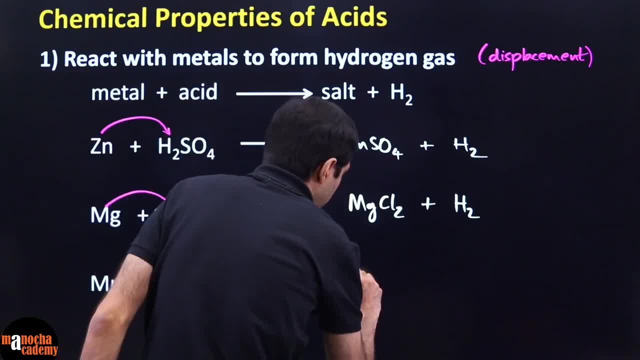 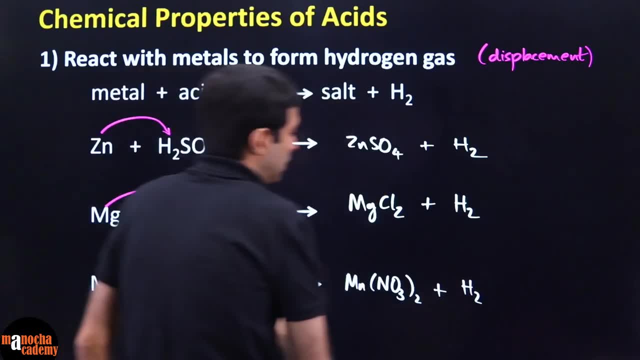 acid, then you get this similar behavior of salt, which is going to be manganese, nitrate plus hydrogen gas. So, you are going to get this simple reaction. If you take manganese or 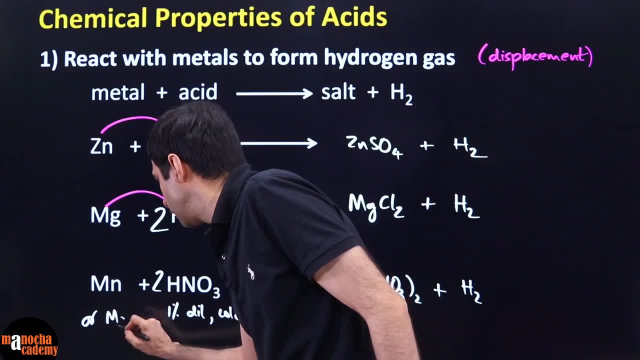 magnesium. So, this is important. Only two metals can react with 1% dilute cold nitric acid to give you salt and hydrogen. So, this is the reaction. So, this is the reaction. So, this is the reaction. 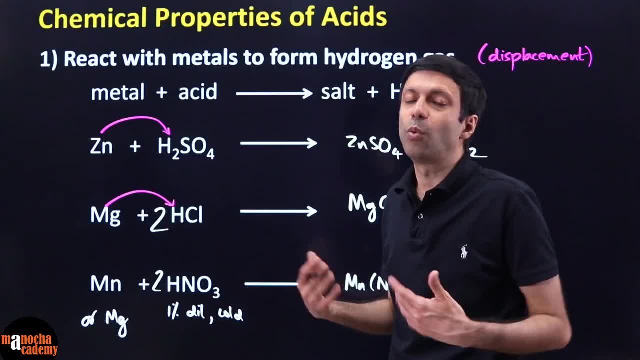 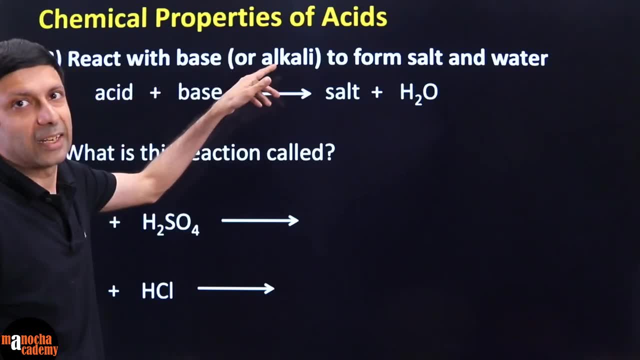 The remaining metals will end up producing salt, water and the nitrogen oxides. Another reaction of acids is that they react with bases or alkalis. What is the meaning of alkali? Bases, which are 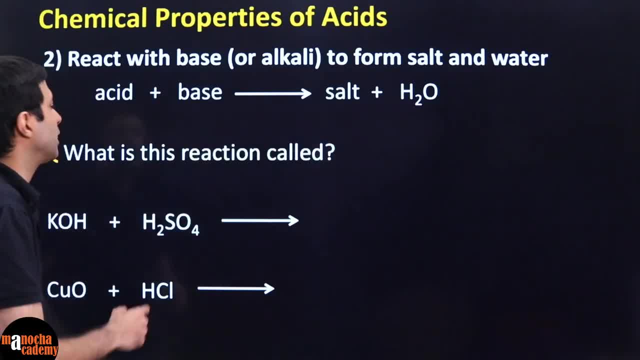 soluble in water to form salt and water. This is the very famous reaction you have heard of. Acid plus base gives salt plus water. Can you guys tell me what is this reaction, famous reaction known 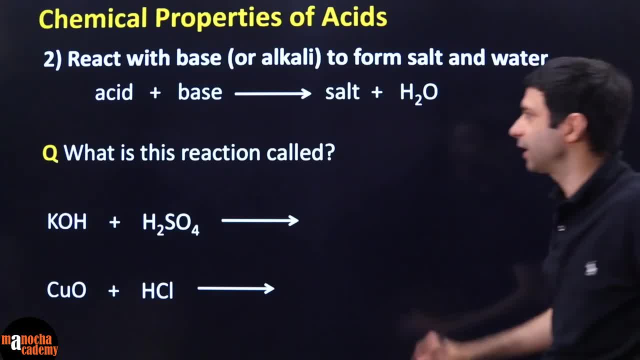 as? Can you tell me what is the name? Very good. The correct answer is neutralization reaction. 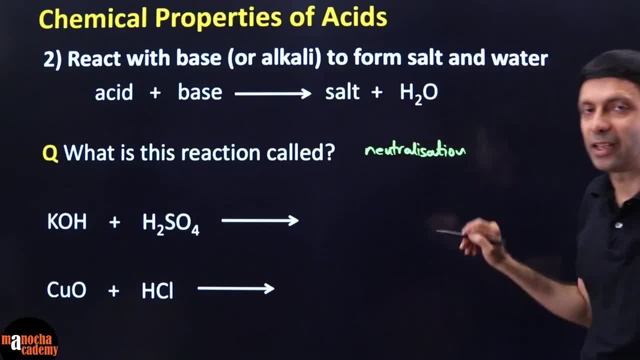 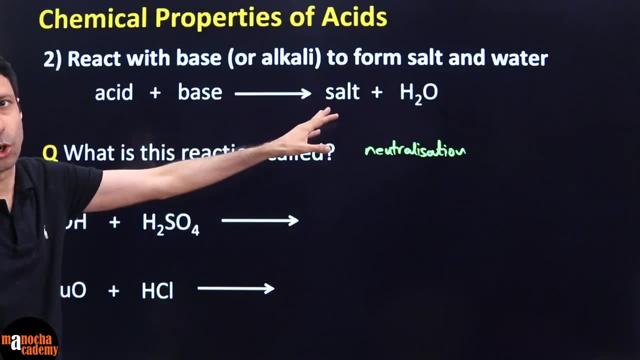 I think English and Indian and British spelling is with an S. American spelling, they use a Z. So, please use whatever your book is using. This is basically your neutralization reaction. Acid plus base gives salt and water or alkali plus acid gives salt and water. So, now can you guys easily 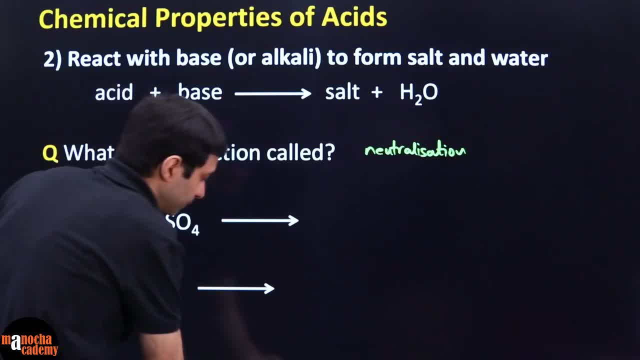 predict this? When you look at this, oh, KOH, this is an alkali. Copper oxide, it doesn't dissolve in water. So, it's a base. And here we have these acids. So, obviously, we can see that this is an acid plus base reaction. So, it's a neutralization. 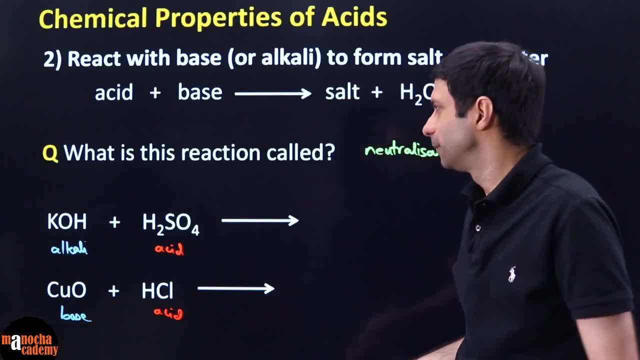 It is going to give us salt plus water. So, can you guys predict the answer for me? Very simple. These are all, you know, like the double displacement reactions because if you break 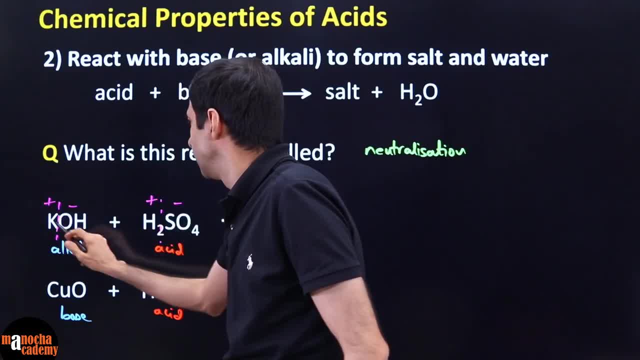 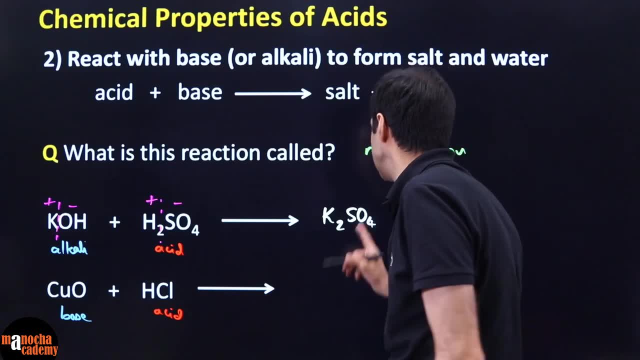 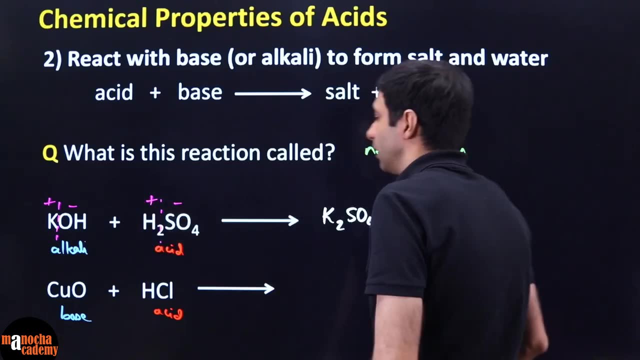 it down, plus, minus, plus, minus, you guys can see the potassium is going to go to sulfate to form potassium sulfate. And please combine it according to valency. Valency of sulfate is 2, potassium is 1. So, it is K2SO4. H and OH combine to form water. So, plus H2O. Similarly, for this 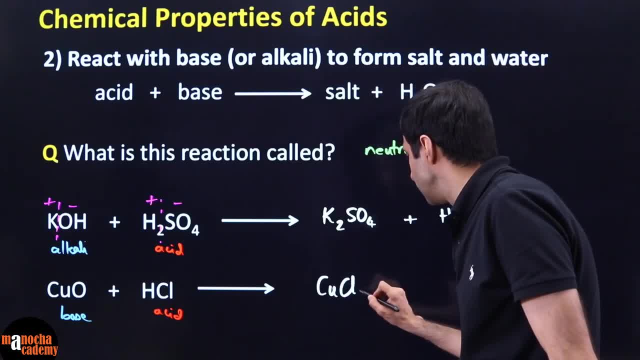 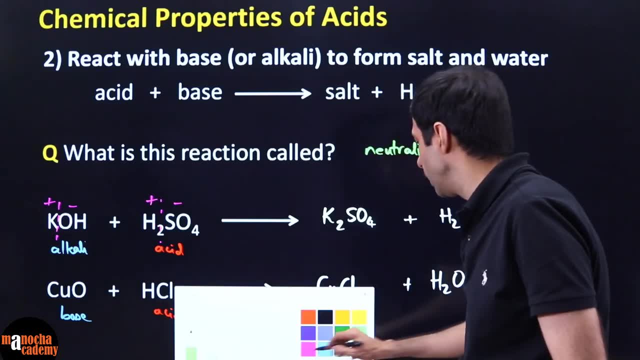 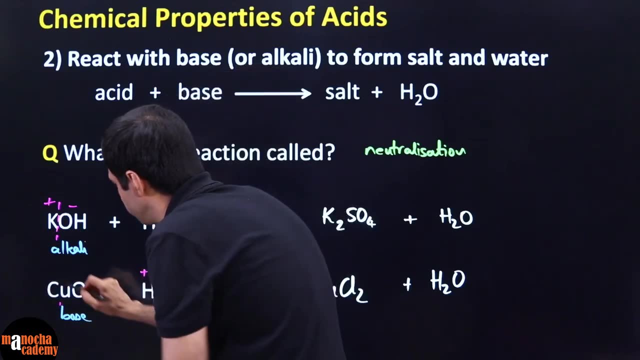 acid, again, they combine according to their valencies. The salt we are going to get is CuCl2. Copper usually carries its valency of 2 plus H2O. Again, you can easily do this by breaking this down into plus, minus, right? So, copper and oxygen here. So, copper and chlorine, hydrogen and oxygen. Clear? How we predicted this reaction? Similarly, you can predict other 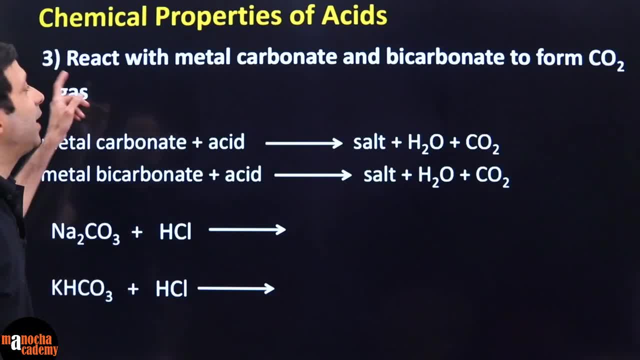 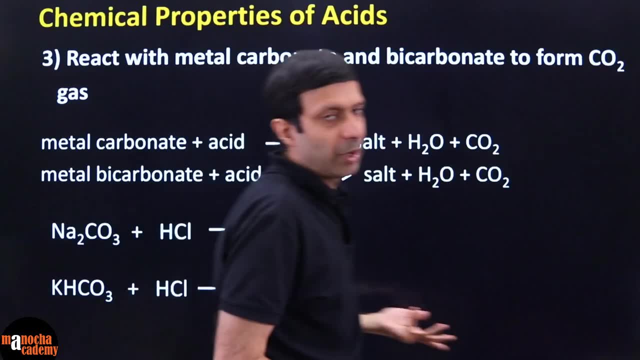 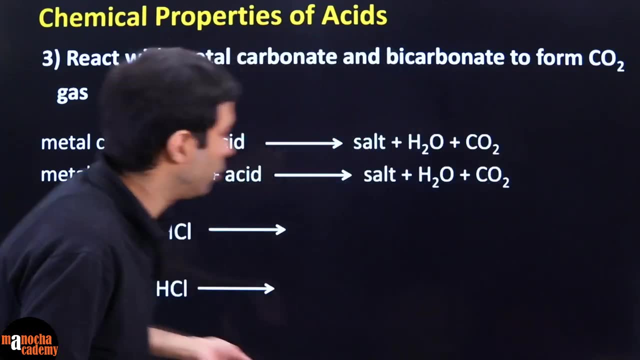 neutralizations. What are the chemical properties of acids? They react with metal carbonate and bicarbonate to form carbon dioxide. So, they react with metal carbonate and bicarbonate to form carbon dioxide gas. So, what is the meaning of bicarbonate? Bicarbonate basically means hydrogen carbonate. So, let's see how we can easily predict this. Again, let me show you a very simple technique. So, let's say you take sodium carbonate and an acid. Again, it is a double displacement. 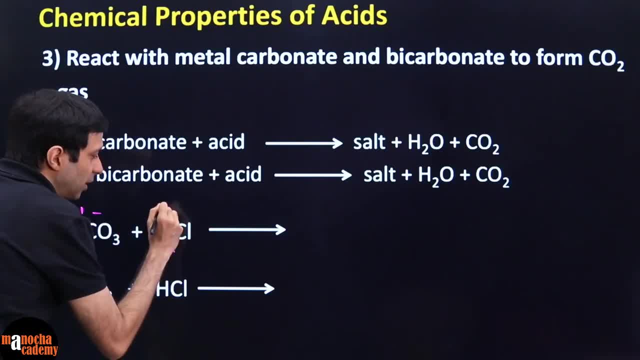 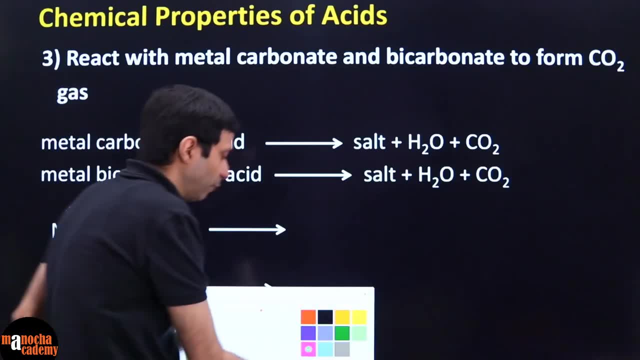 Please break it down like this. Plus, minus. Do all this in rough work. Please don't show all these secret tricks. Okay? Do it in rough work and or erase it out. Do it in pencil. So, again, 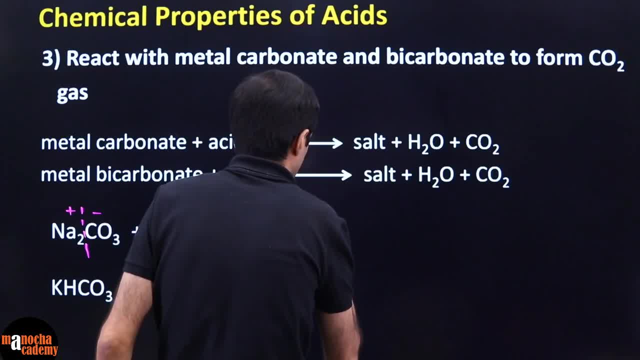 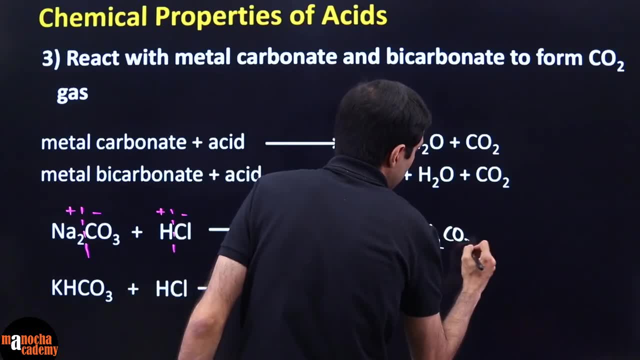 what do you need to do? Combine the sodium and the chlorine. So, that will give you, positive, negative will combine sodium chloride. Then combine the hydrogen and carbonate. So, that will give us, what is this called? Can you guys tell me? 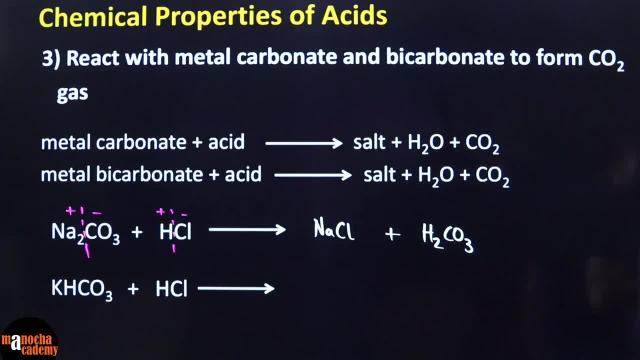 So, we have got salt and H2CO3. What is it known as? Very good. This is carbonic acid. H2CO3 is 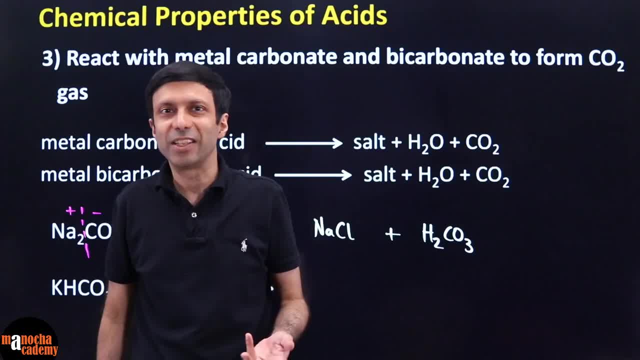 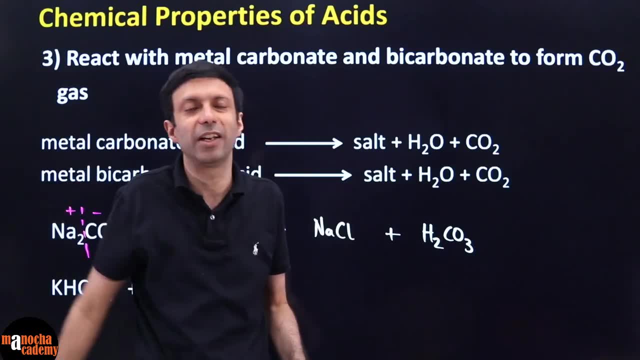 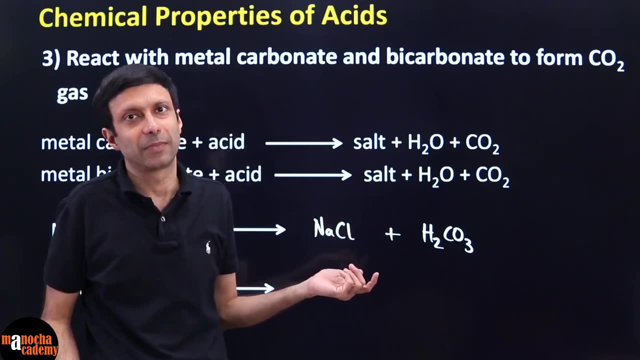 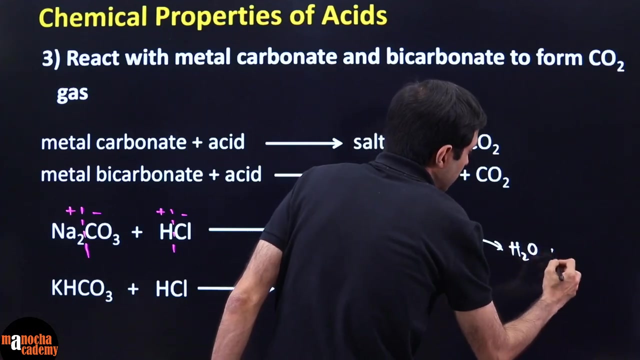 carbonic acid. Where have we seen carbonic acid? In our aerated drinks. The Coca-Cola, Pepsi you have, that basically contains carbonic acid. Why? Because they have compressed carbon dioxide into it. They have dissolved a lot of carbon dioxide into the aerated drink. So, carbon dioxide and water. Carbonic acid is unstable. Right? So, it doesn't usually like to remain at carbonic acid. It quickly breaks down into water and carbon dioxide. That is why 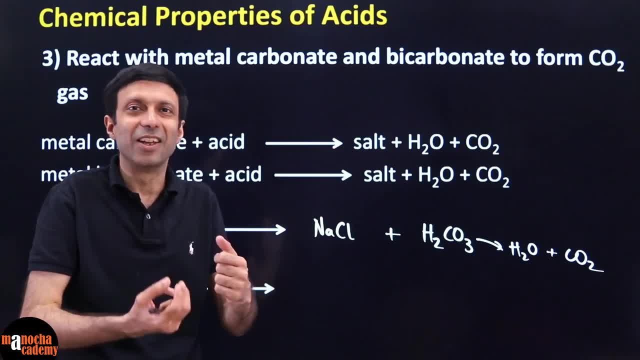 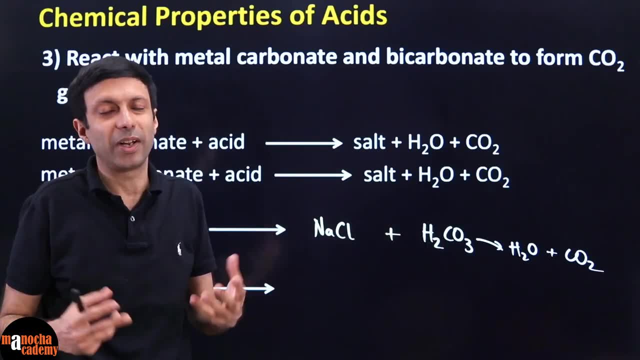 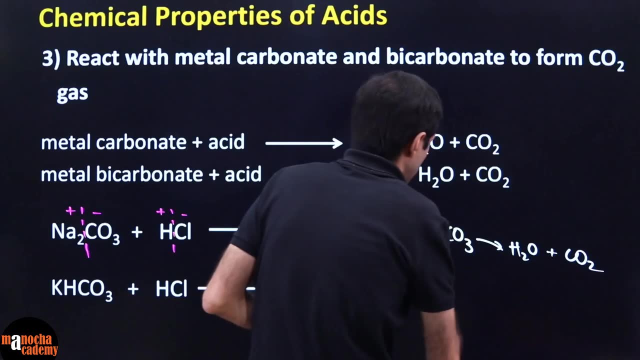 you know that when you open that Coca-Cola or Pepsi can, you get that sound, right? Is the carbon dioxide coming out? Okay? Because carbonic acid is breaking down, right? They are pushing a lot of carbon dioxide into the can or into the bottle, right? And so, when it breaks down, so that is why we do carbon dioxide. 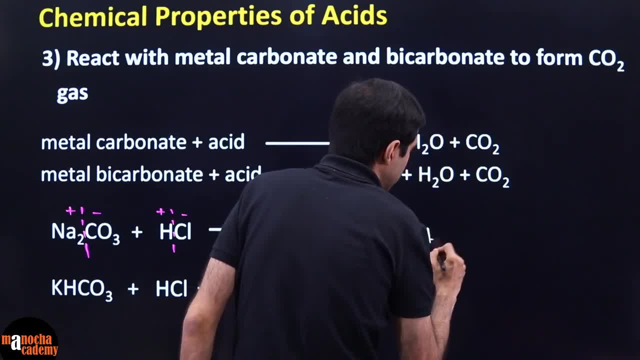 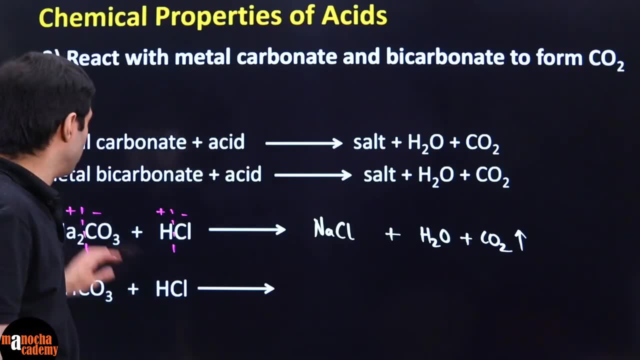 We don't write H2CO3. We break it down and write it as H2O plus CO2. And that is how you can see that it releases carbon dioxide gas. So, any carbonate you react with acid, it produces a salt, 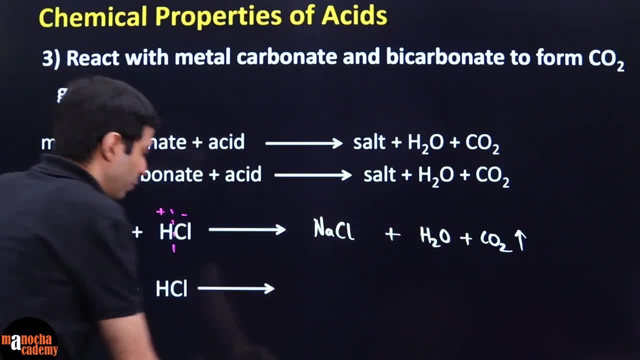 water and carbon dioxide gas. Similarly, for the bicarbonate and again, please balance these equations. Just to save time, I am not balancing it. So, here positive, negative. Similarly, 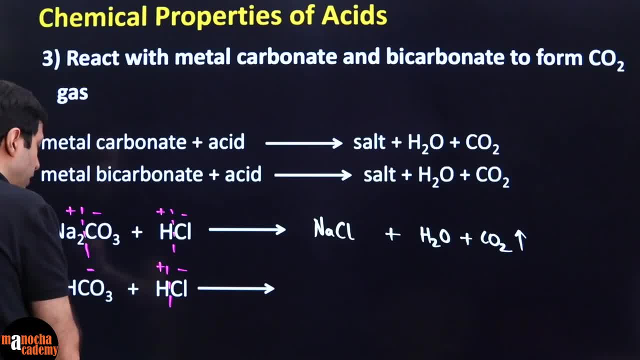 potassium bicarbonate. Potassium is the positive, carbonate is the negative. So, when you guys combine this, what will you get? Potassium and 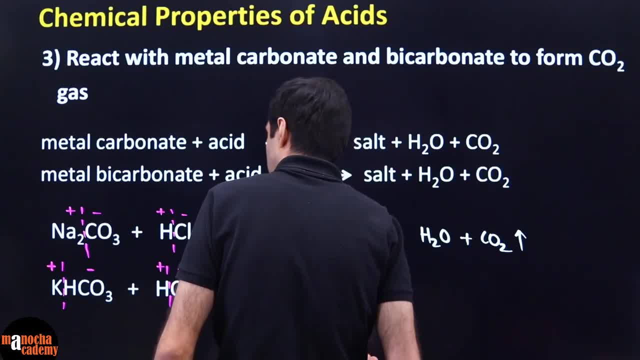 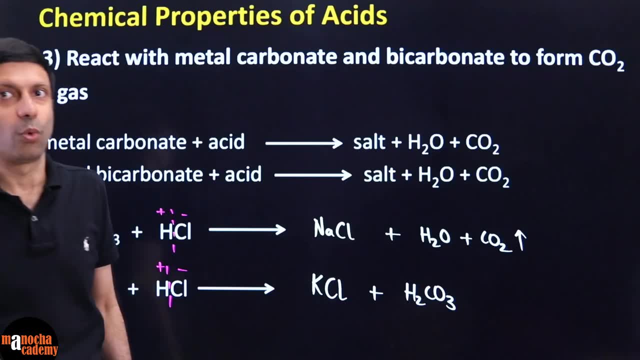 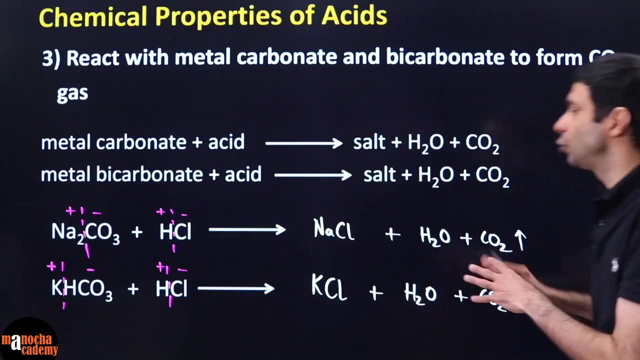 chlorine will combine to form potassium chloride. Okay? H and HCO3 will again form carbonic acid, H2CO3. But that quickly breaks down into water and carbon dioxide. So, what we are going to end up with is H2O plus CO2. So, very good question. We should not write H2CO3. So, that is the secret. 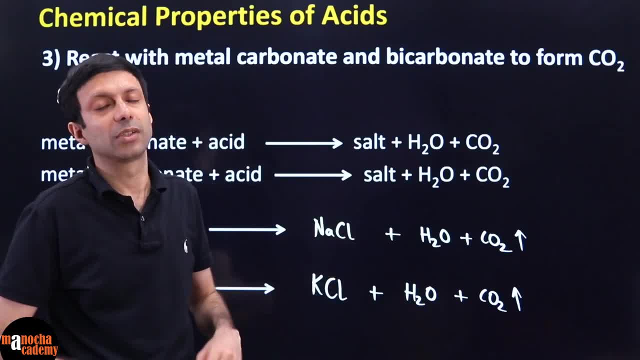 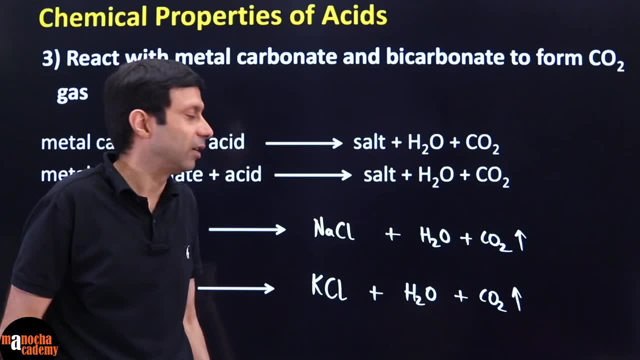 It is finally giving us H2CO3. But we should not write it because 90, 95 percent, it breaks, and it releases carbon dioxide gas which goes out into the atmosphere. So, you can do that in 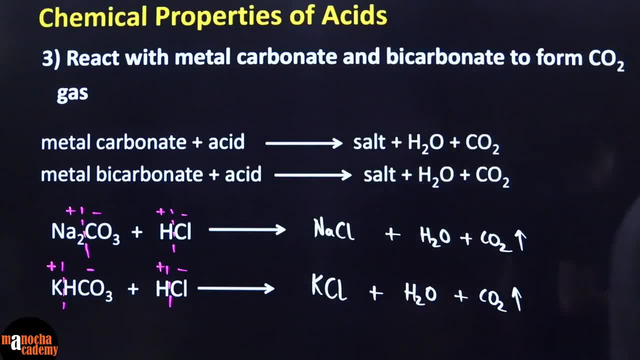 rough work, but you should end it like this. Okay? Do not write H2CO3. Clear? So, this is how we predict the reaction, right? If you remember this technique, so, I will tell you in my school days, 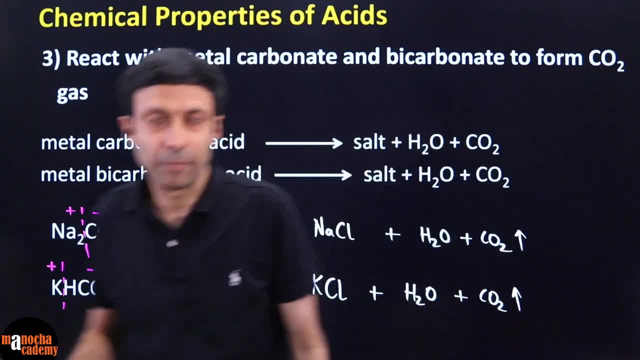 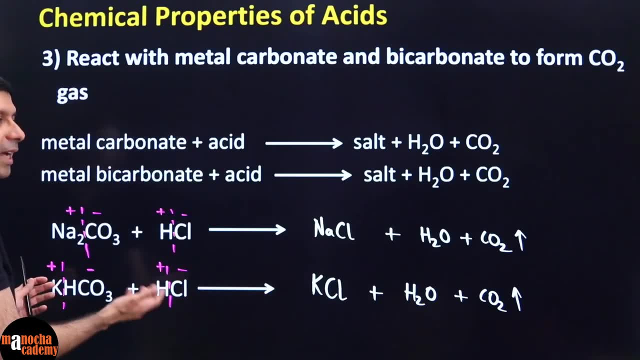 I never memorized this. I would easily predict it based on this logic. Plus, minus, oh, sodium chloride, H2CO3, that breaks down. Potassium bicarbonate, HCl. So, you give me any acid, any bicarbonate, carbonate, we can do it. So, this is how we predict the reaction. So, 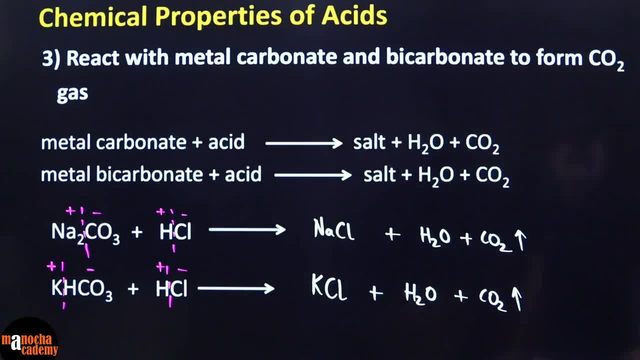 we can easily predict this. We do not have to memorize these reactions. Similarly, see, for the sulfites also, we can do that. Even if you do not read the rule, let us try this. 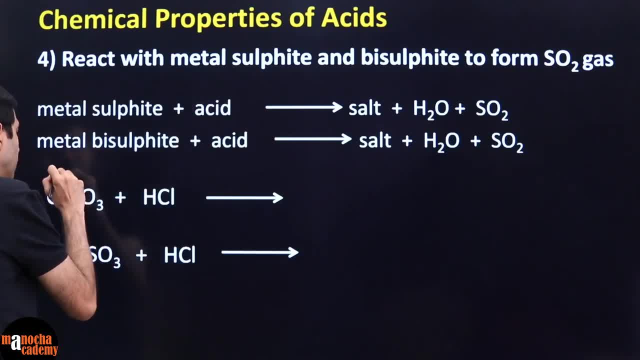 You have got calcium sulfide, HCl. Everybody, pick up your pen and paper. Do this plus, 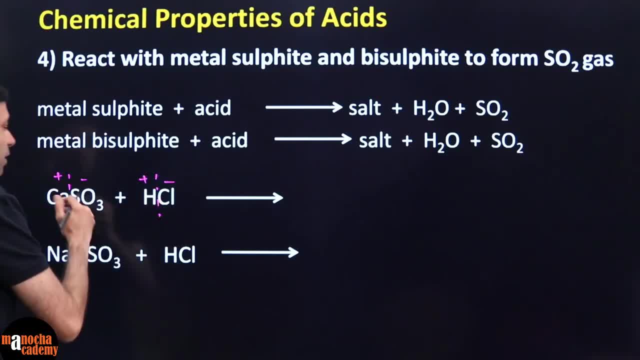 minus. Break it down. Positive gets attracted to negative. Positive to negative again. So, 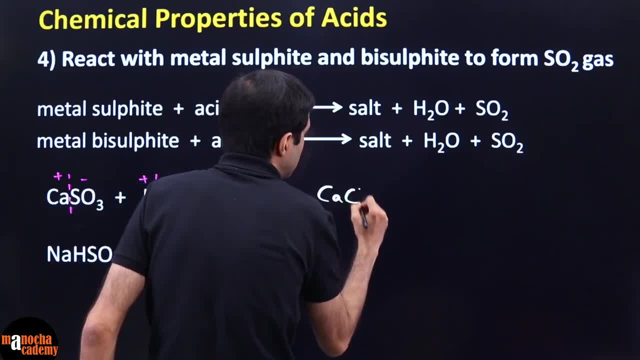 what will we get here? Calcium and chlorine. But please do not write CACL. Use the valency. 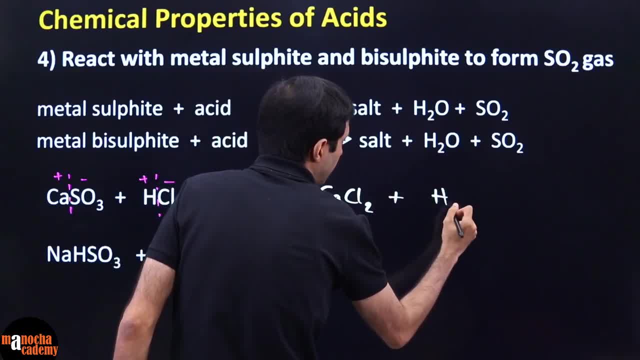 Calcium chloride, CACL2. Sulfite has valency 2. So, it will give me H2SO3. 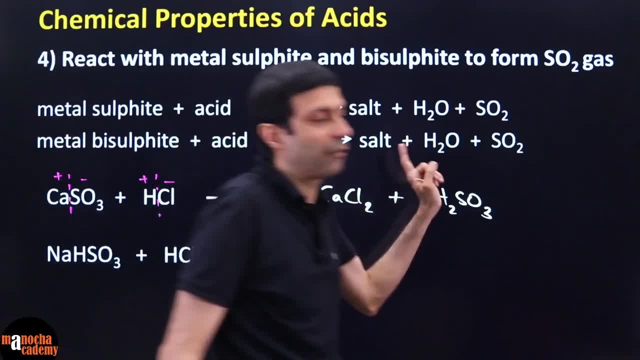 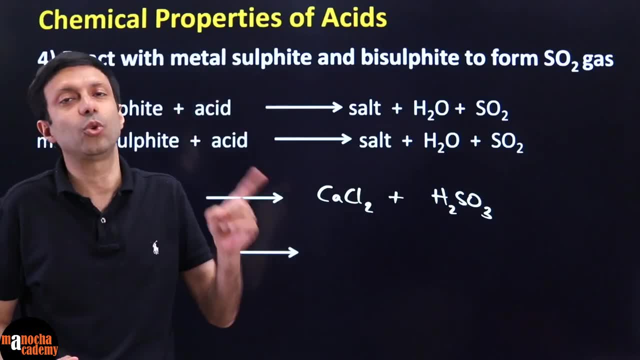 What is the name of this guy? Can anybody name this guy for me? Who is H2SO3? Guys, this is not sulfuric acid. This is sulfurous. Sulfuric is H2SO4. Everybody knows. But one 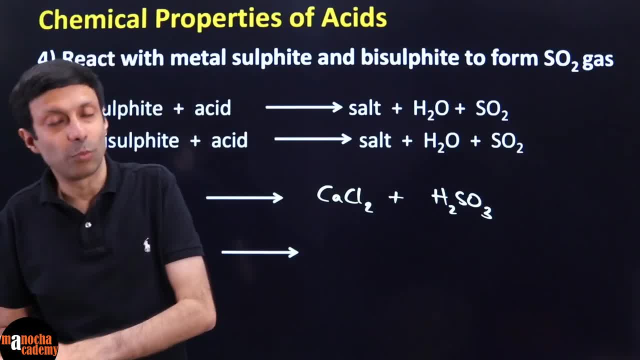 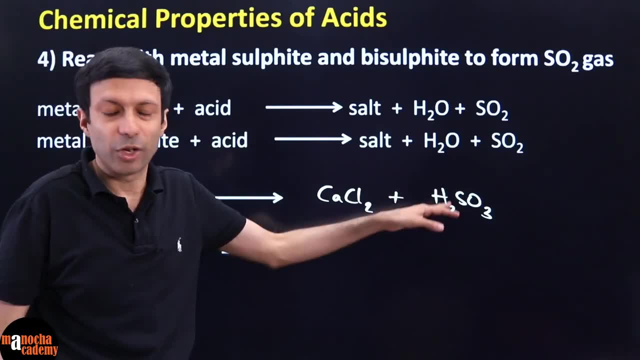 oxygen less. Remember, I told you, us means less oxygen. Ik means more oxygen. This is sulfurous acid. Again, how to predict this reaction? Sulfurous acid is just like carbonic acid. Carbonic acid is H2CO3. H2SO3 quickly breaks down to give you H2O plus SO2. Remember, 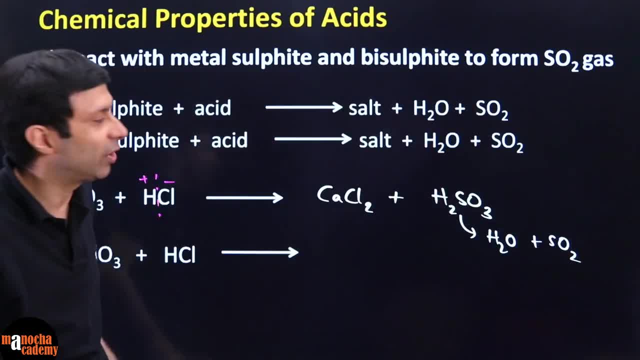 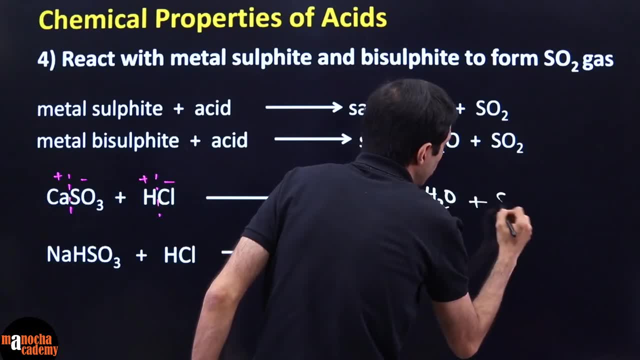 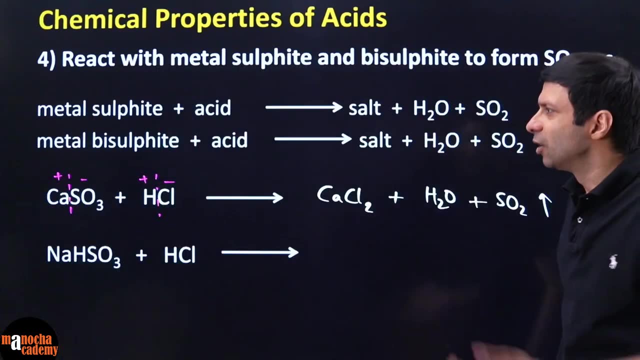 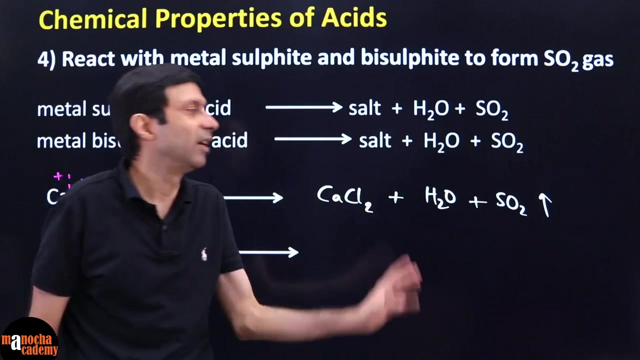 this was the acid anhydride of it. If you dissolved it in water, you got H2SO3. So, it is breaking down into water and it's acid anhydride. And that is why the answer will be H2O plus SO2. And this is your gas sulfur dioxide. So, guys, you can predict these equations. You don't have to memorize them. You just follow this plus minus technique. Only thing you have to remember, I should not end my answer with H2CO3 or H2SO3. It will break down further. That's it. Similarly, for the bisulfite. 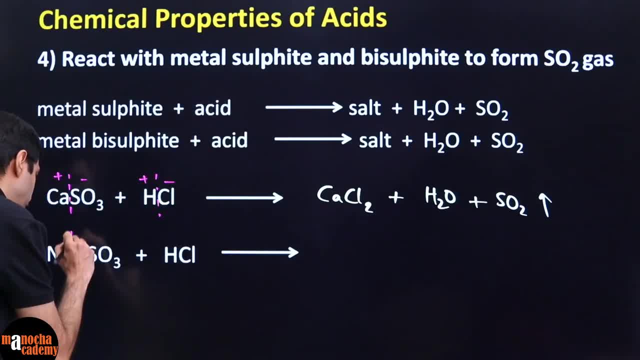 Bisulfite. Look here. Again, come on. Pick up your pen and paper. Do this. This is a really 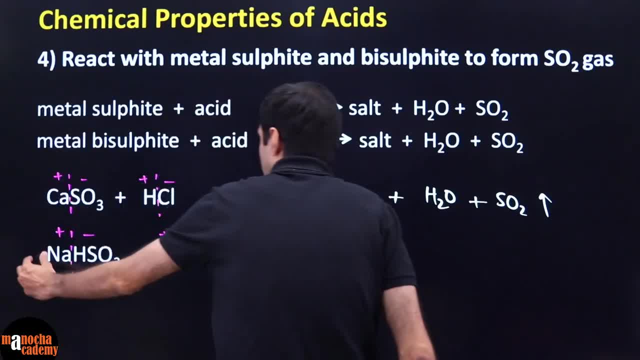 important trick to understand what is happening here. Now, combine sodium and chlorine, NaCl. 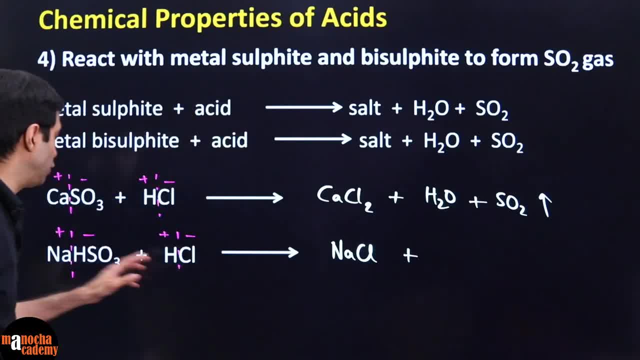 Valency is 1. So, obviously, I will not write NaCl2. H and HSO3. It will give me H2SO3. 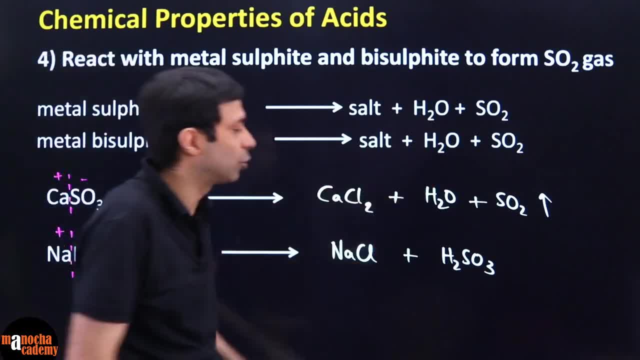 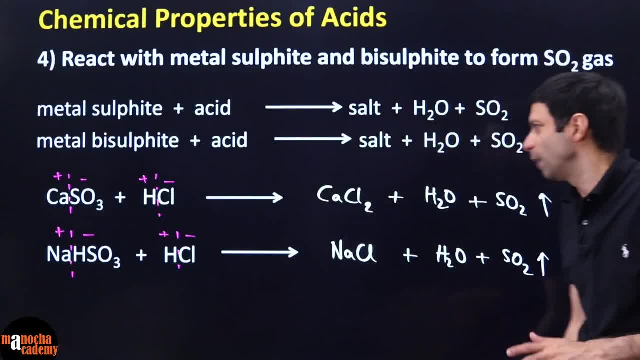 So, before balancing these equations, you know, you guys can balance. These are quite easy to balance. Like if you look at the first one, there is Cl2, there is H2. I think if I put a 2 here, it's going to get balanced. Anhydride means those compounds like carbon dioxide is the 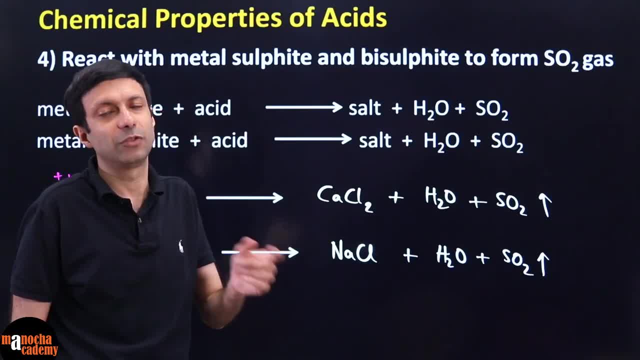 acid anhydride of H2SO3. You take carbon dioxide plus water, it gives you H2CO3. 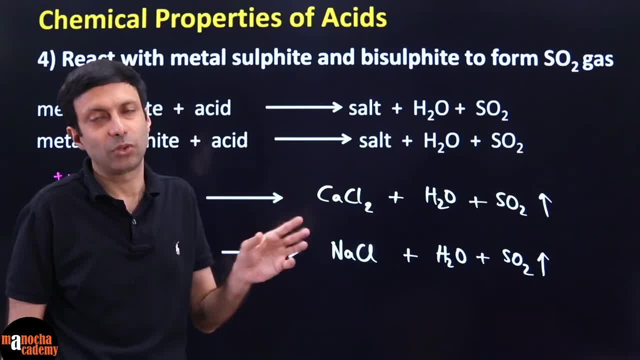 SO3 is the acid anhydride of H2SO4. SO3 plus water, H2SO4, right? So, the compound that you dissolve in water, when it gives the acid, that compound is called it. 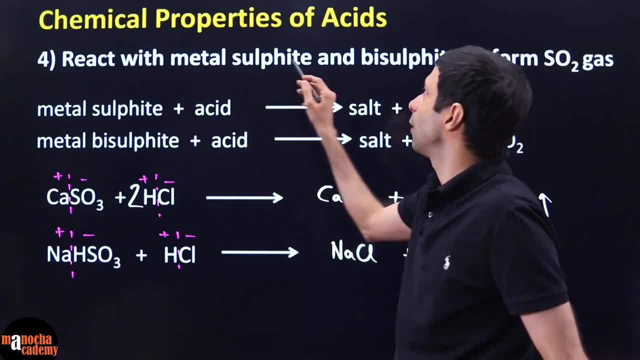 Acid anhydride. So, you guys can see that with metal sulfites, again, sulfite is not sulfate. 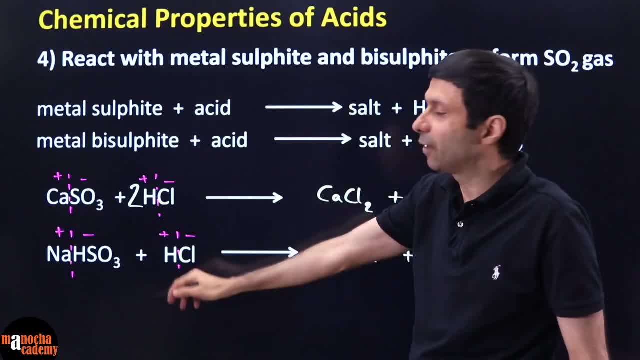 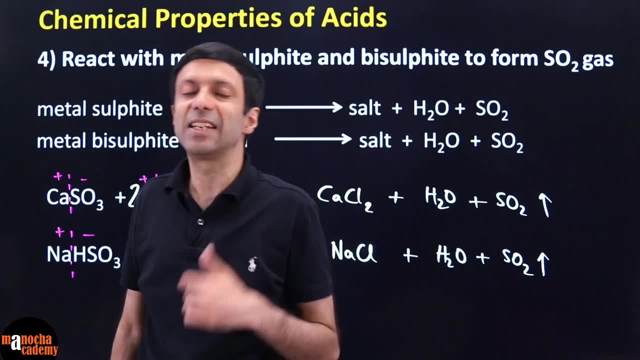 Sulfite is SO3s and the bisulfites or the hydrogen sulfites, you get sulfur dioxide gas. Clear? What is the observation of sulfur dioxide gas? It is a pungent smelling gas. It has the smell of burnt 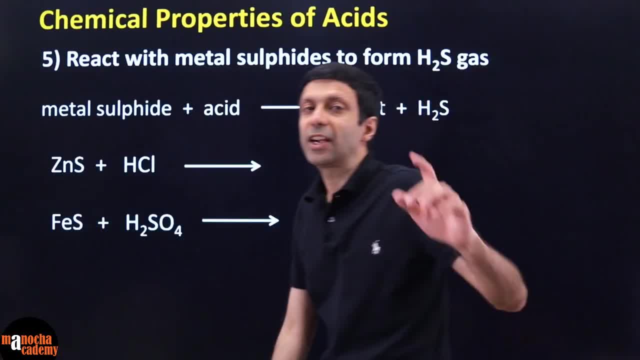 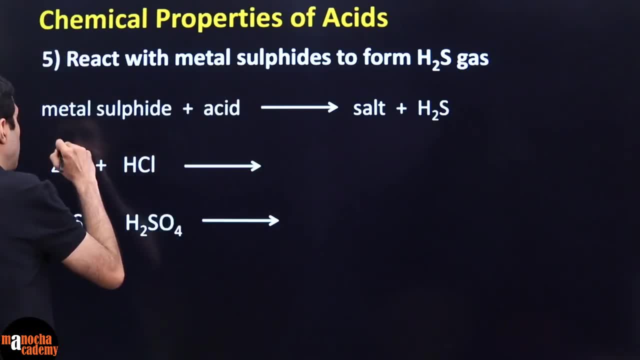 sulfur. So, all these things you have to remember. Next, it reacts with the metal sulfites to form hydrogen sulfite. Again, I will show you how to predict this. Very easy. Don't learn these. Plus, 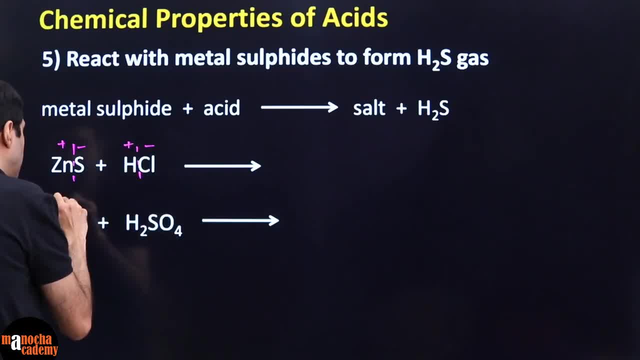 minus, plus. Minus. All of you try. Same way here. Plus, minus, plus, minus. You can easily predict this. Zinc and 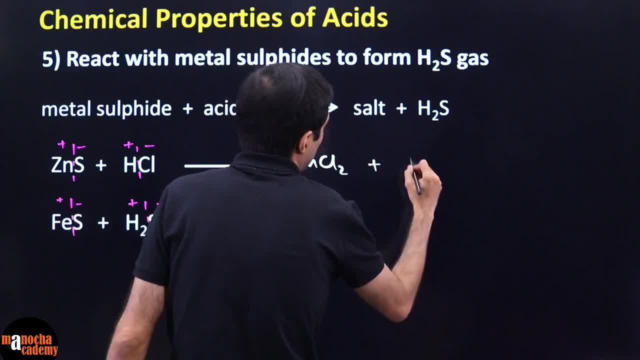 chlorine, ZnCl2. Hydrogen and sulfur, H2S. There you go. You want to balance it, put a 2 here, I think. Done. FeS plus H2SO4. What will be the answer? Ferrous sulfate. Hydrogen and sulfur, H2S. 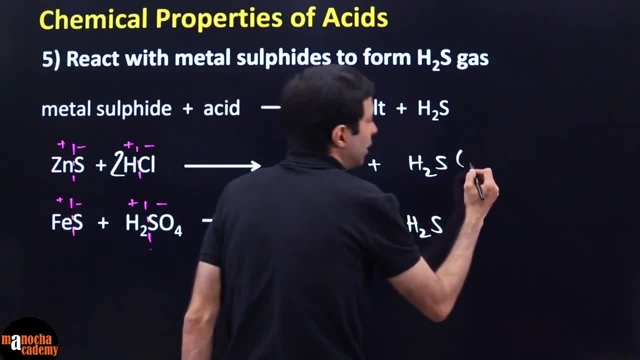 What is the property of this H2S? H2S is a gas, right? You can write G or you can put the up arrow. Observation is what? 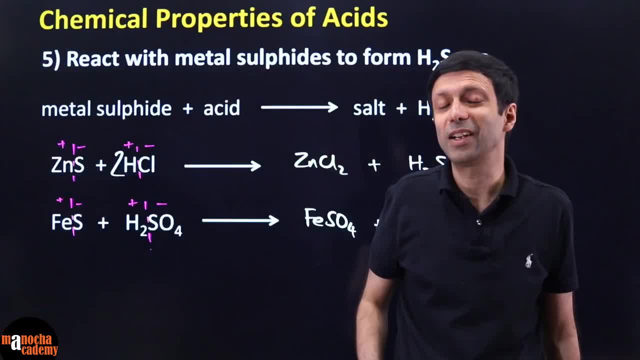 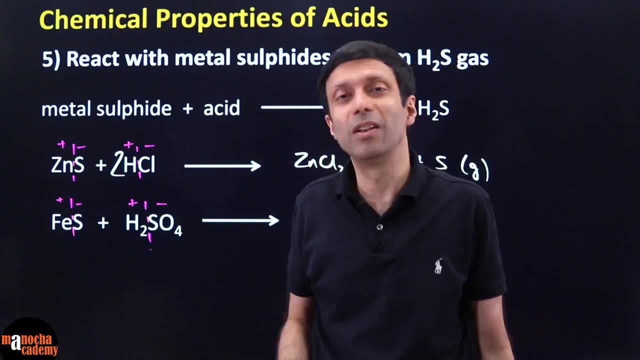 Pun. It has the smell of rotten eggs, right? Rotten egg smelling gas. I remember when we used to do in our school days, this chemistry lab experiments with H2S gas. It was horrible 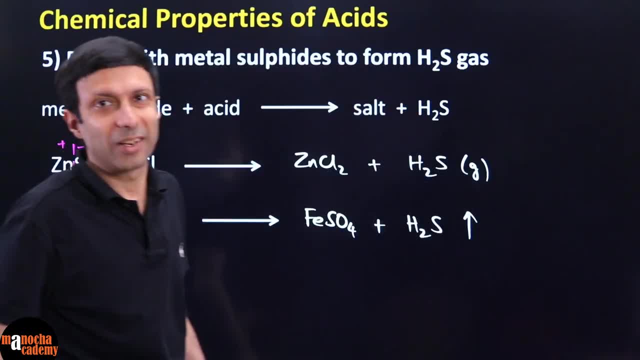 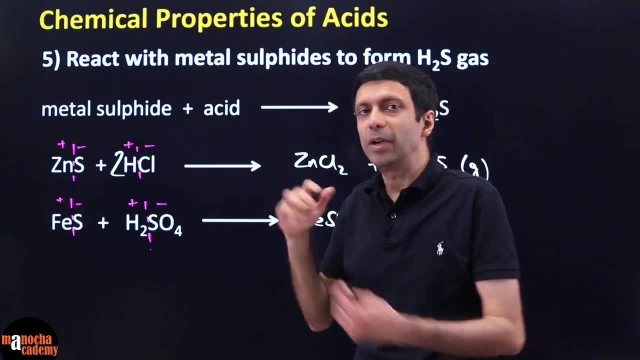 smell, right? Because it releases a rotten egg smelling gas. So, you guys confident how we can predict this? If they give you any sulfite. So, you can see these are all working out to be double 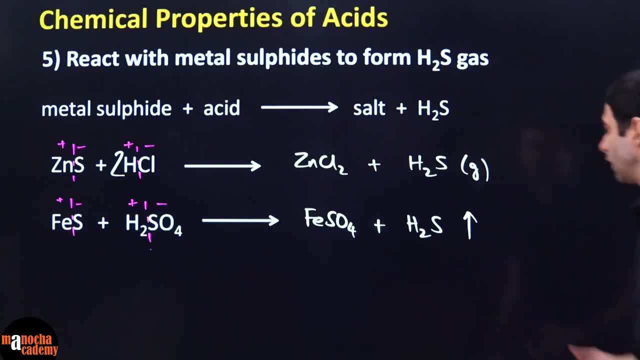 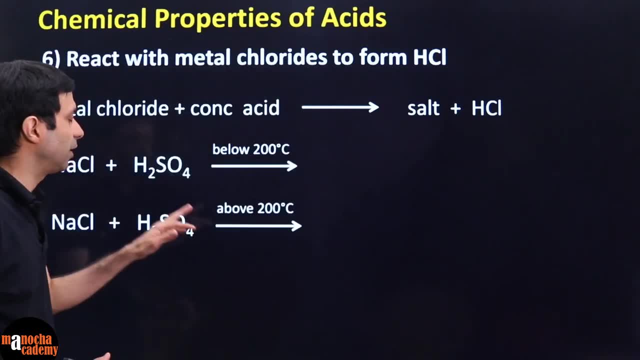 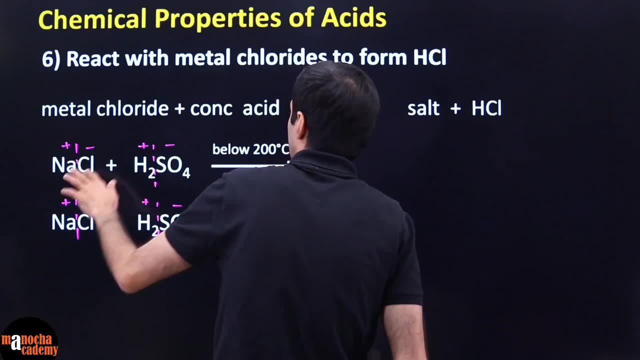 displacements. Plus, minus, plus, minus. Exchange the ions and you are done. Next, reaction with the metal chlorides. So, metal chloride, I told you temperatures. Important, like we had discussed, if you do below 200 degree Celsius, again here, these are all double displacements. The only difference being if you do the reaction at a lower temperature, 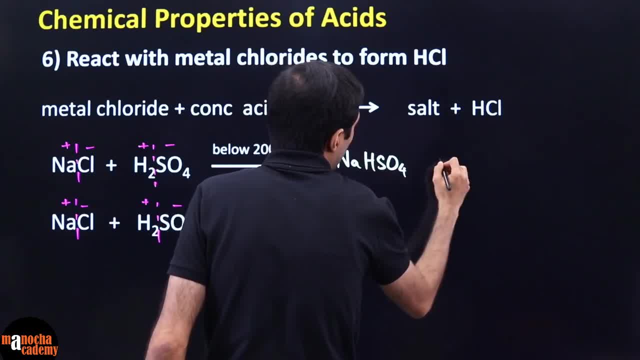 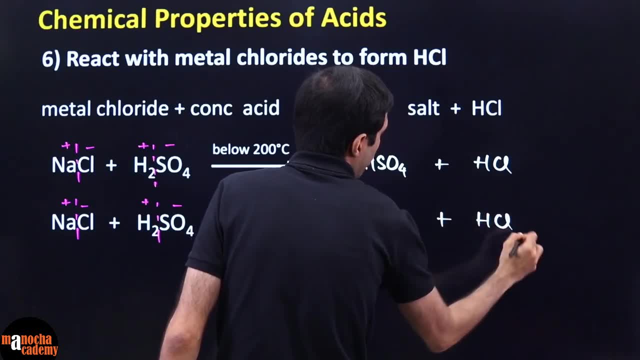 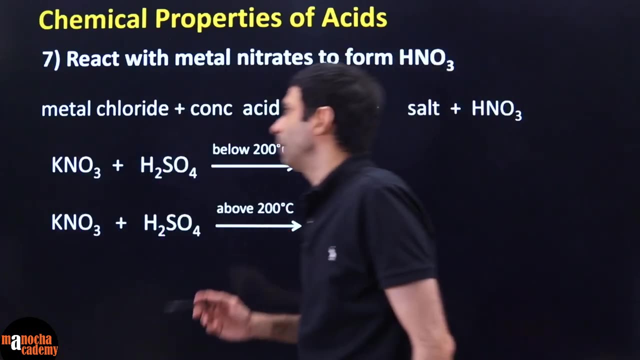 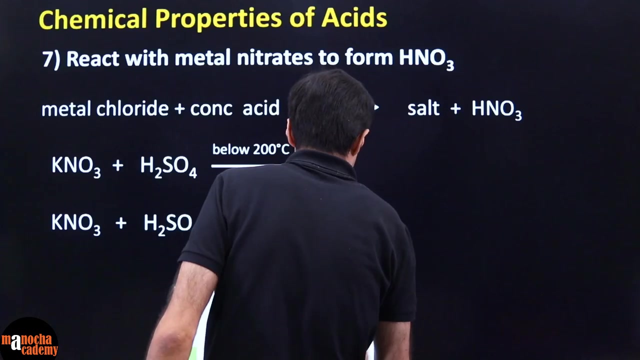 it will give you sodium bisulfate. Only one hydrogen will go and HCl gas. But if you do at a higher temperature, it will give you sodium sulfate and HCl gas. Both the hydrogens will go away. This is the reaction below 200 and above 200 degrees. Same thing happens here. Metal chloride, below 200 with the nitrates also, same story. Again, you can do the plus minus here. So, that's my goal to teach you how to predict these reactions, guys. So, if you do this reaction, what 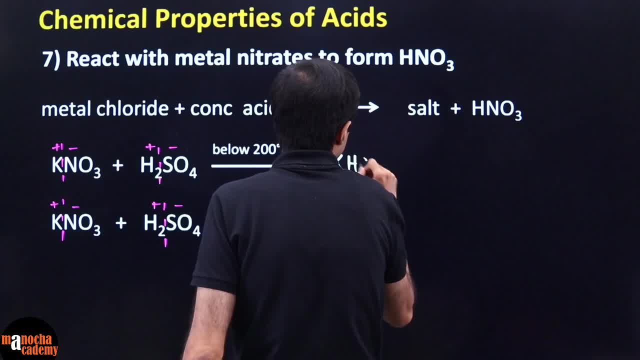 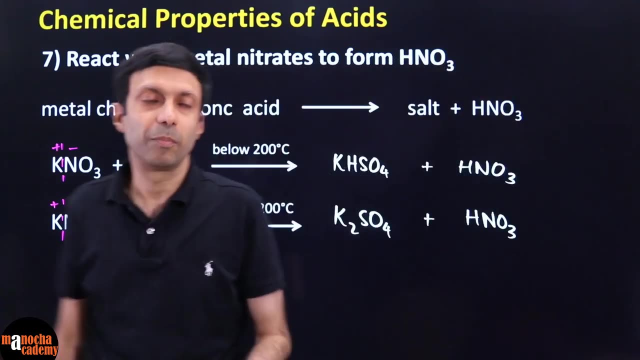 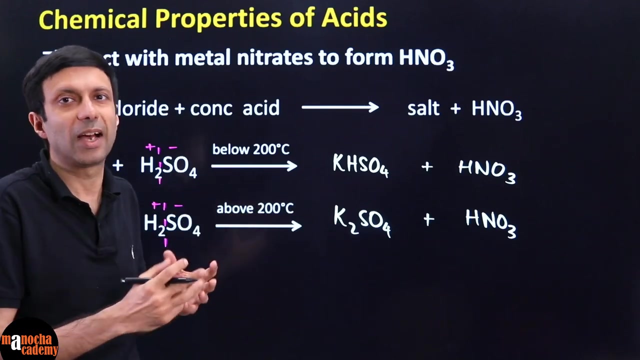 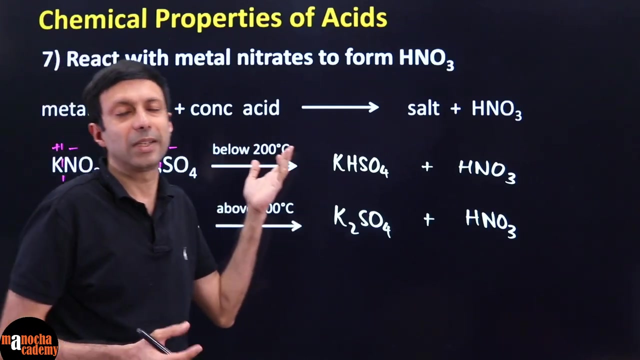 will happen? This will give you potassium bisulfate plus HNO3, just like last time you got HCl. And here, you will get above 200, you will get all the hydrogen replaced, potassium sulfate and HNO3. And this is given in the ICICI textbooks that the reaction is preferred below 200 because what's the problem here? One, you are not going to get the same reaction. So, you are going to get the same reaction. So, you are wasting fuel also. And the potassium sulfate, which is formed above 200, it sticks to the glass. It spoils the apparatus, right? And the reaction speed slows down. So, always the preferred is temperature below 200, where it will form the bisulfates. 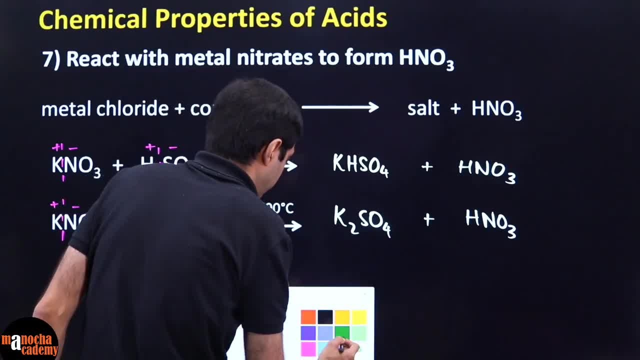 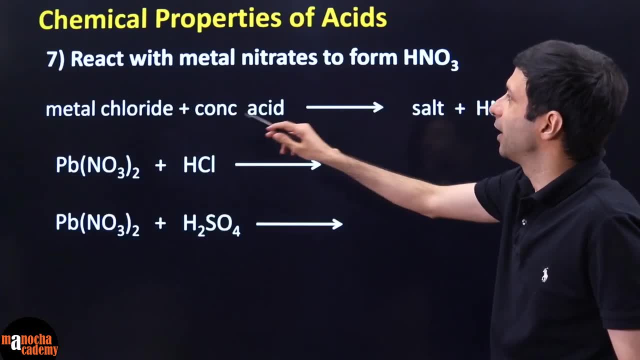 Sorry, guys, by mistake, we have written metal chloride here. It should be metal nitrate. So, thank you for pointing that out. This one should be metal nitrate. So, reaction with, again, metal nitrate. It should not be chloride, metal nitrate. 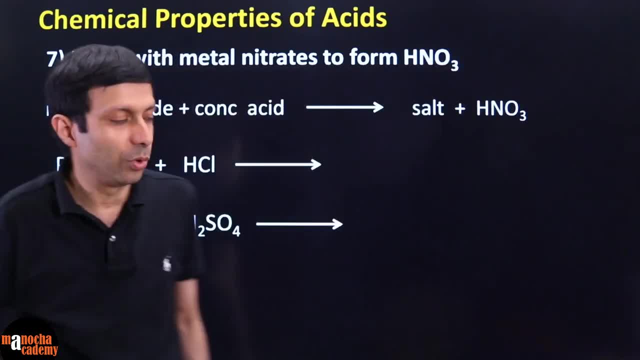 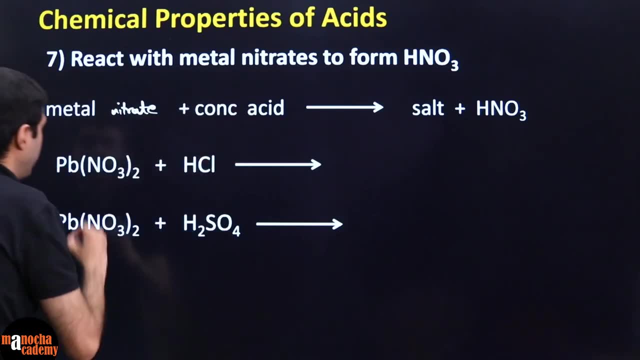 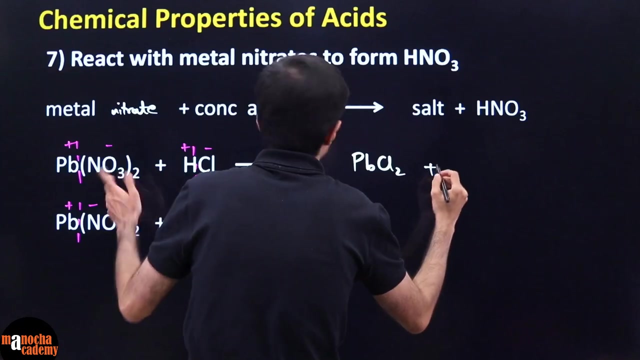 So, if you take these metal nitrates, like lead nitrate, again, you just do the positive negative, plus minus here, same thing here, plus minus, plus minus. So, as expected, double displacement will happen. So, you will be getting PbCl2 plus HNO3. Similarly, here, you will be getting PbSO4 plus HNO3. So, you will be getting PbCl2 plus HNO3. So, you will be getting PbSO4 plus HNO3. 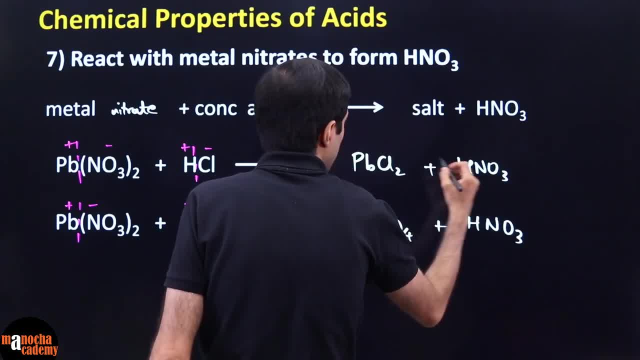 So, you will be getting PbSO4 plus HNO3. And I think you guys can balance. It will be, I think, 2 here, 2, 2. So, we have discussed all the chemical, how to prepare the acids and the 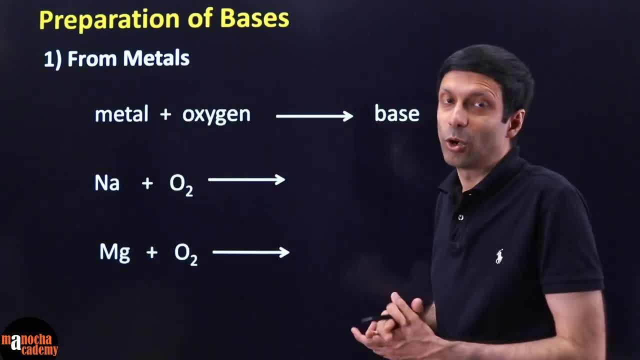 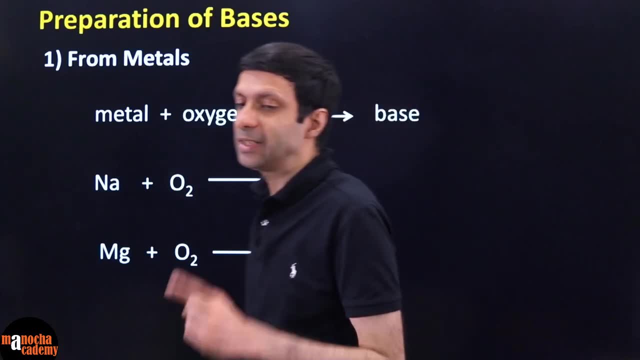 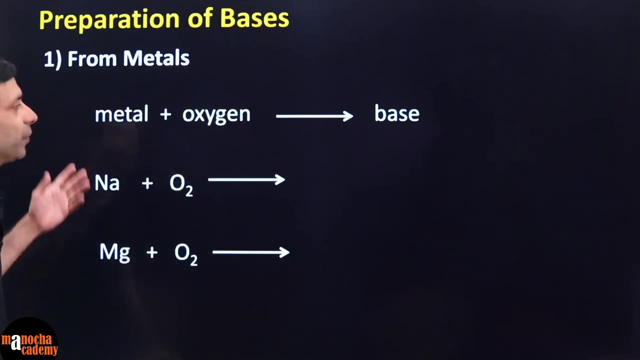 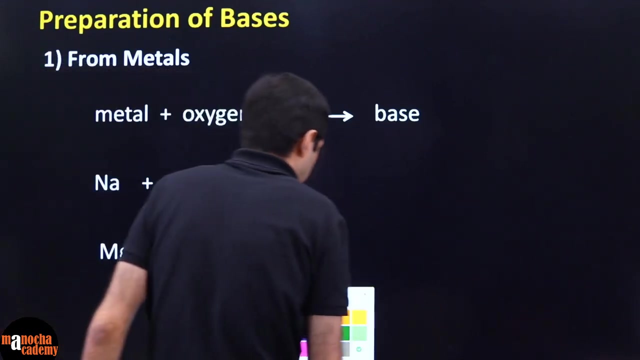 chemical properties of acids. Now, let's talk about the bases. First of all, how we can prepare the bases and then their reactions. So, how do you can prepare the bases? Remember, we have discussed what are bases, metal oxides, metal hydroxides, right? And then you also have ammonium hydroxide. So, let's talk about how do you prepare a base. It's a simple metal oxide. So, let's talk about how do you prepare a base. It's a simple metal oxide. So, let's talk about how do you prepare a base. It's a simple metal oxide. So, many metals are highly reactive with oxygen like sodium and magnesium. You just heat them, they will happily react with oxygen. 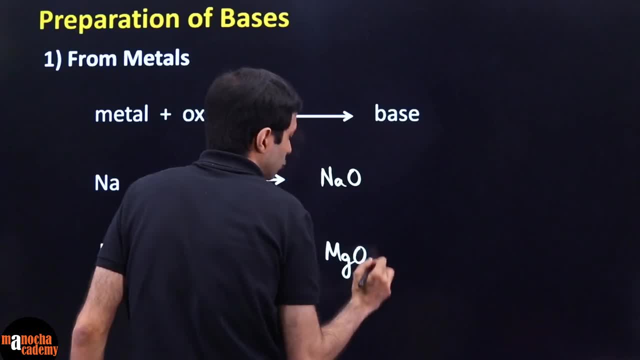 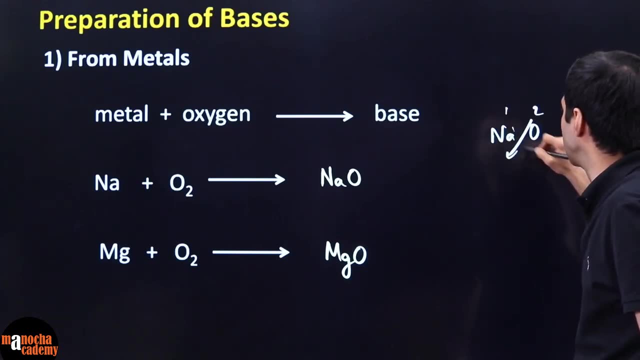 Here, can you tell me, is this the correct formula? Which formula is wrong? Sodium oxide or magnesium oxide? Which one is wrong? Guys, sodium has valency 1, oxygen has valency 2. Don't forget 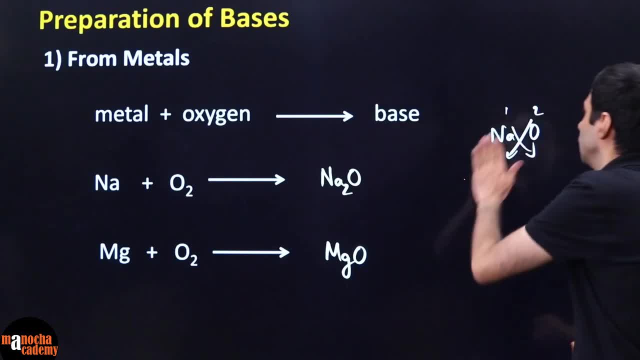 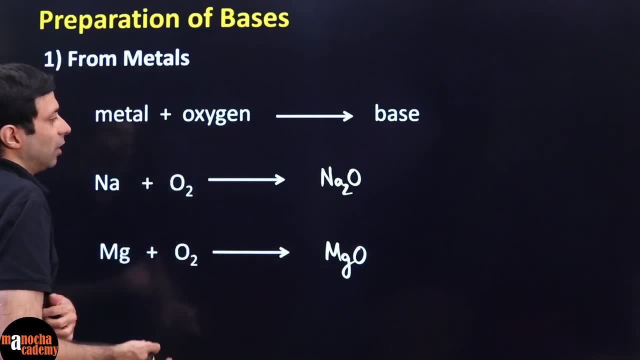 valency, crisscross. This is going to be Na2O, sodium oxide. Magnesium oxide is correct. Both have valency 2, magnesium and oxygen. It will cancel. Now, you can balance your equation. So, you have 2, 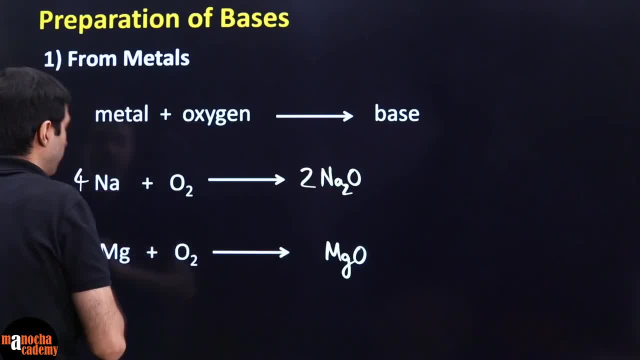 oxygen here only 1. So, we will multiply by 2, we will multiply by 4 here. This one, 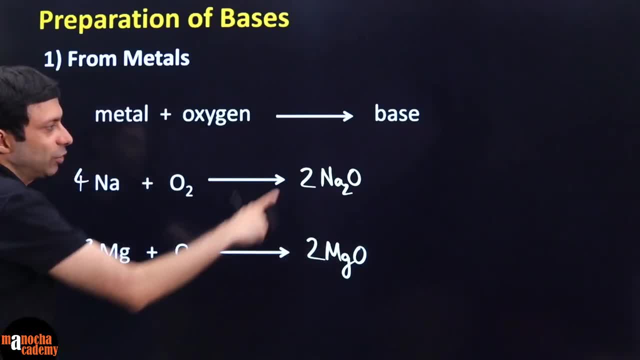 I need to multiply by 2 here and 2 here. So, can you see these are the bases formed? 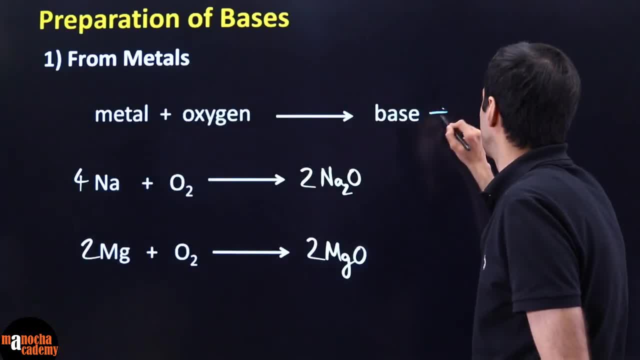 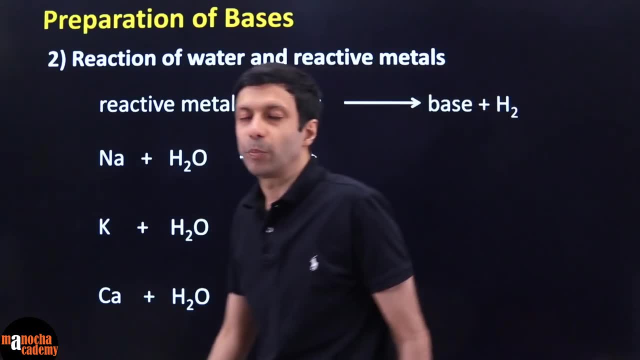 Because bases we discussed, they are basically the bases are your metal oxide, metal hydroxides and ammonium hydroxide. Next, you can also prepare the bases by reaction of water and 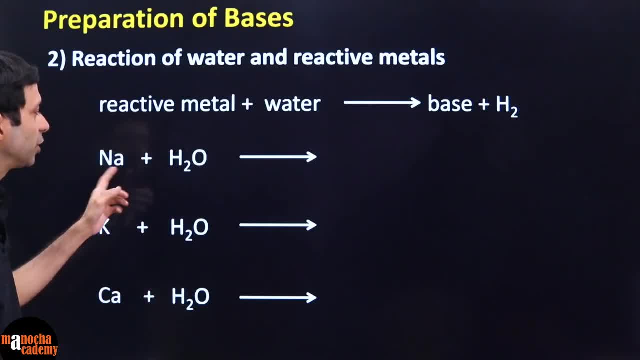 reactive metals. So, can you guys predict here for me? Try the first one, sodium plus water, what will it give? 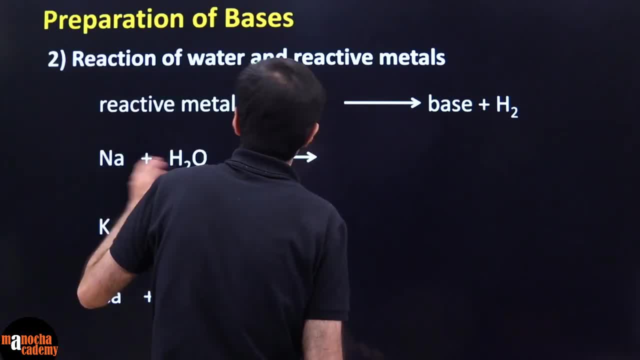 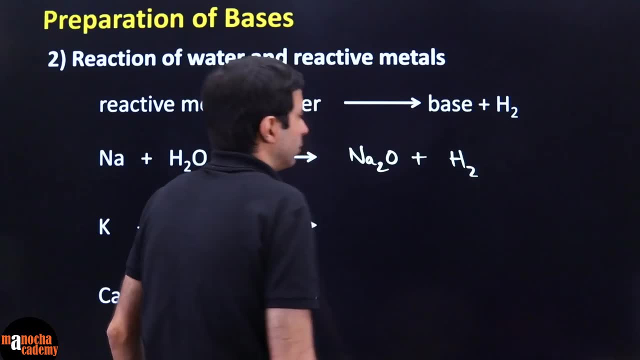 Sodium plus water, what will you get? See, again, sodium is going to kick out hydrogen. So, let's say you predicted sodium oxide plus hydrogen. Sodium is going to kick out the hydrogen. But will that 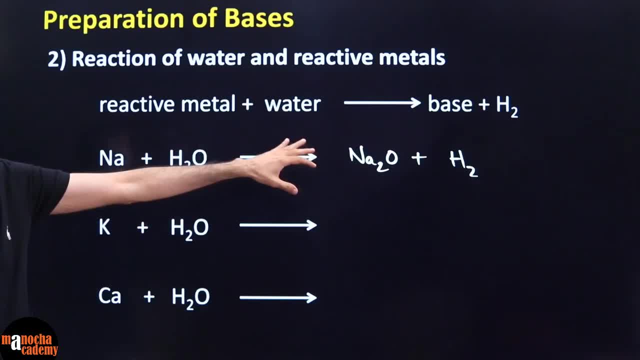 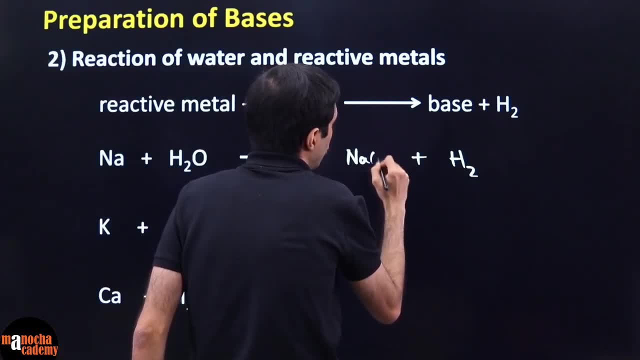 be the right answer? No, because there is still more water left. So, sodium oxide is an alkali, it will easily dissolve in water. So, it will actually produce for us sodium hydroxide plus 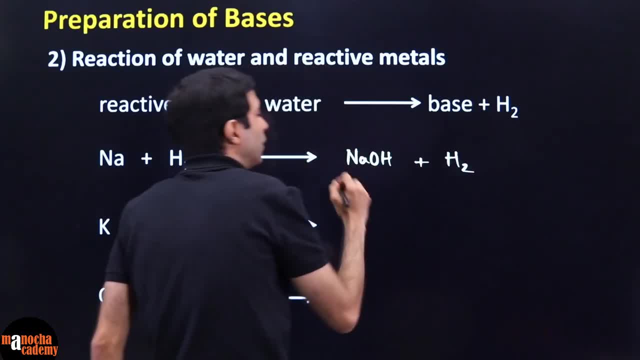 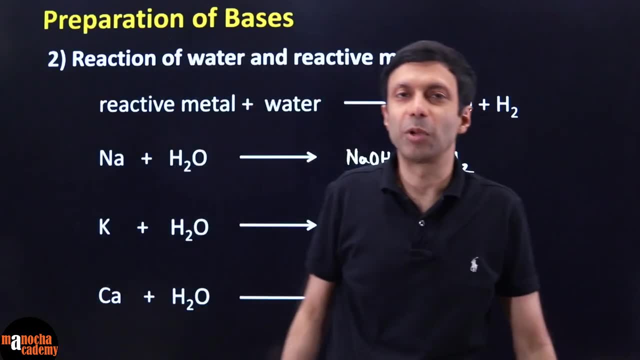 hydrogen. So, please do not think it will dissolve in water. It will dissolve in water. So, it will give oxide. Suppose accidentally you thought oxides, then think, oh, that oxide is going to react with water to give me my alkali. Because sodium hydroxide is a strong alkali, remember? 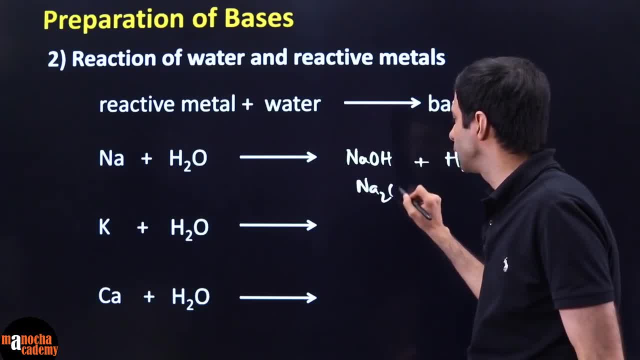 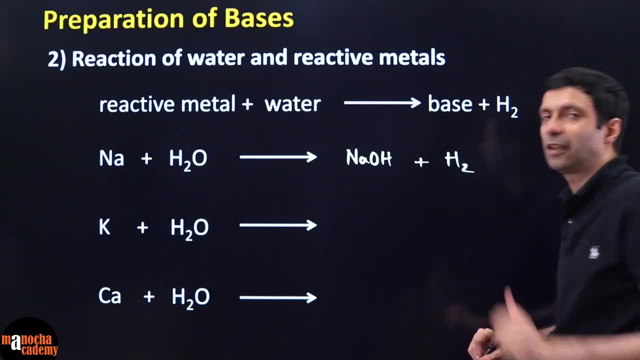 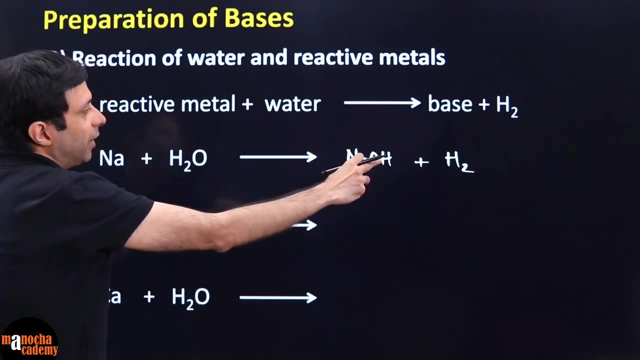 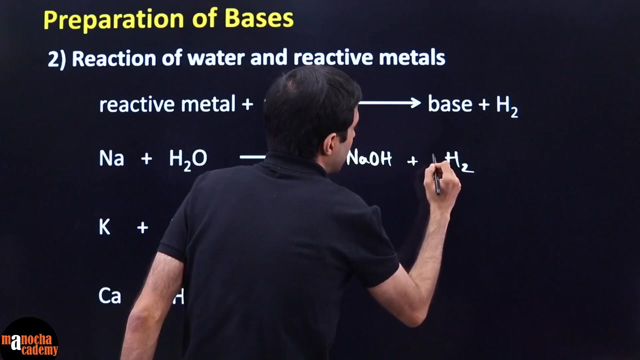 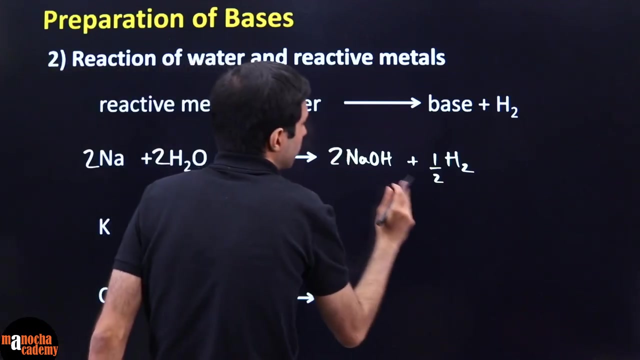 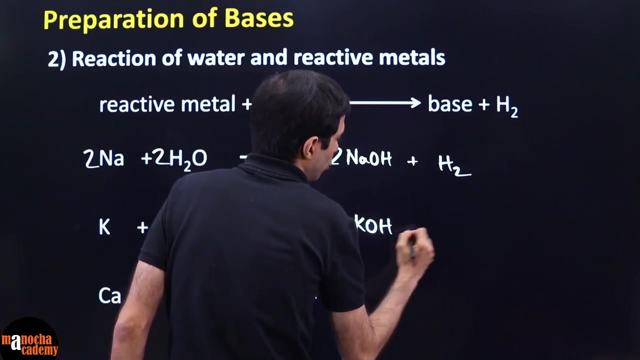 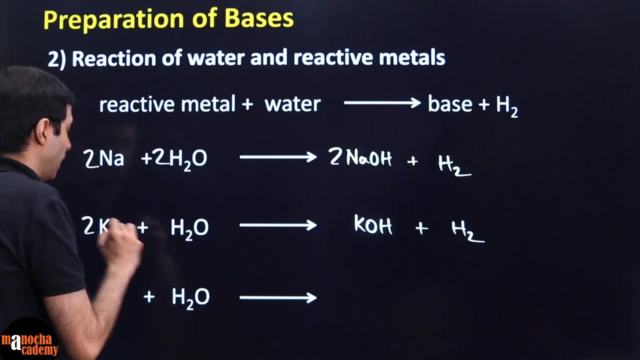 All of you understood why this will not be sodium oxide? Many times this is a common mistake to write sodium oxide because that sodium oxide will again react with water to produce sodium hydroxide. So, there is no chance there will be sodium oxide left. How do you balance the first equation? See, sodium is balanced, oxygen already balanced, only irritation is hydrogen. It is 2 there. It is 1, 3 there. So, when element is alone, we can easily use the fraction technique half. See, now it is balanced. But I want to get rid of the 2. So, I will multiply by 2 throughout. There you go. For potassium, same story. It is going to give you a KOH. Sodium, potassium are like brothers, right? Or sisters. Similar reaction, KOH plus hydrogen. And again, to balance it, it will be the same balancing. They have the same valency. 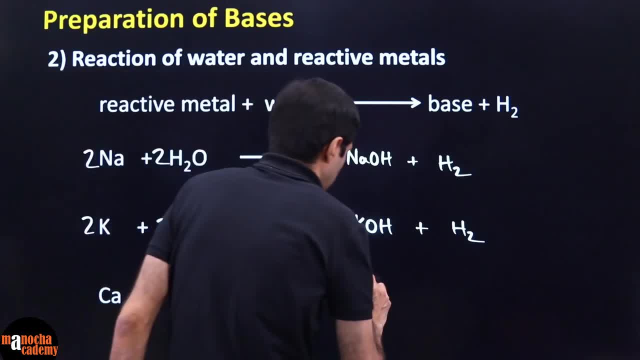 What about the last one? Last one also same story. Calcium will give you calcium oxide. That 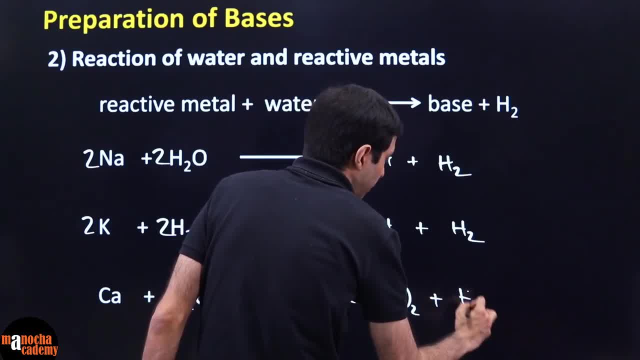 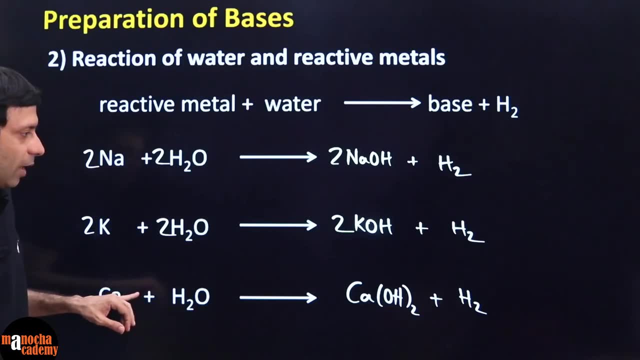 will react with water to give you calcium hydroxide. But be careful here. Calcium valency is 2. So, the reaction will look like this. Now, to balance it, you can see that you have to balance oxygen. I need to multiply by 2 here. There is 4 hydrogen. There is 4 hydrogen. Done. 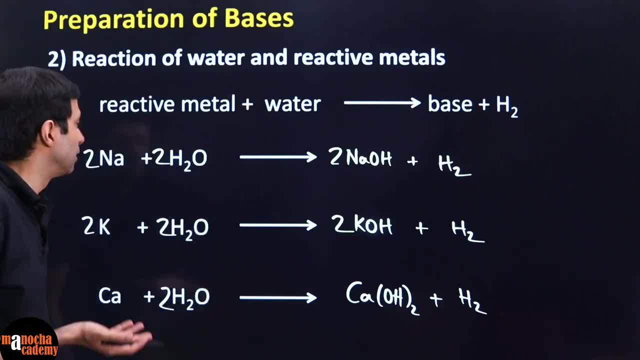 Guys, this is how you predict the reactions in chemistry. You do not have to memorize these. These are just simple displacement. Hydrogen is being kicked out. 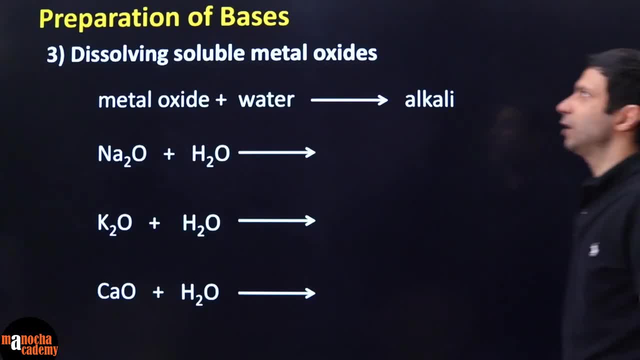 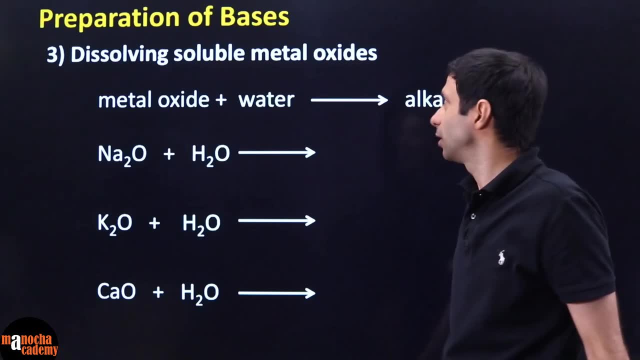 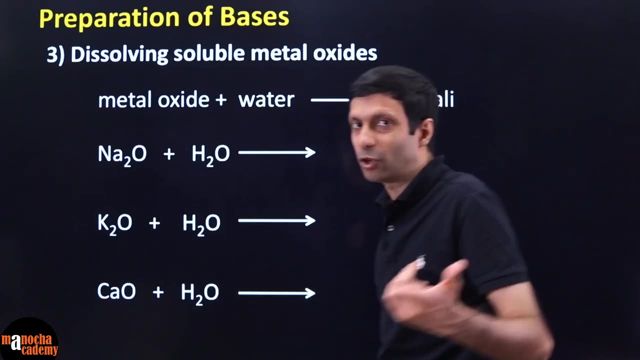 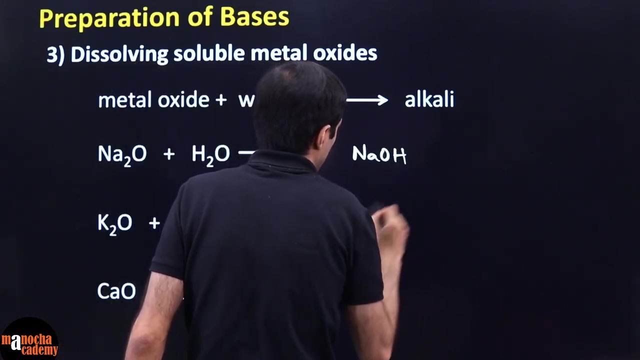 And you are getting your hydroxides here. Next one. How can you prepare the alkalis? Another option is just what we talked about. You dissolve the oxide, metal oxide in water. You will get your alkali. You have 4 famous alkalis. Sodium hydroxide, potassium hydroxide, calcium hydroxide and ammonium hydroxide. So, very simple. Sodium oxide when dissolved in water will give you sodium hydroxide. This will give you potassium hydroxide. This will give you calcium hydroxide. Finished. 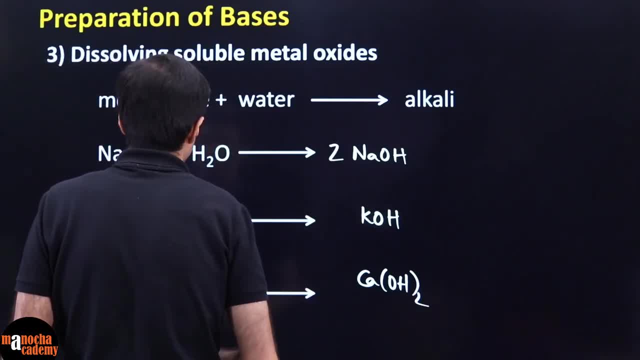 So, you can easily balance this also for me. I think balancing will be like just put a 2 here. That will be done. The last one is I think already balanced. There you go. Again, 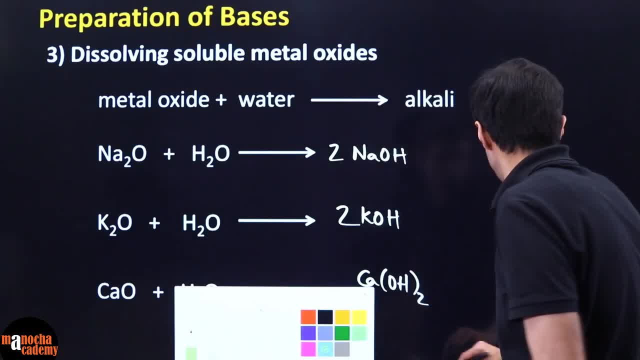 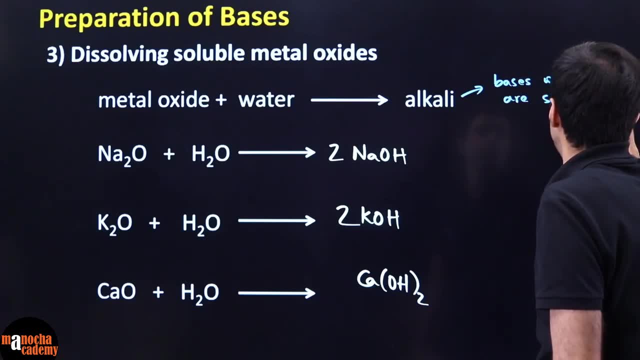 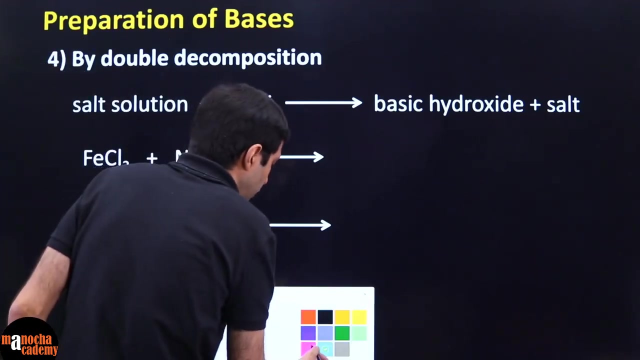 remember what is alkalis? Alkalis are those bases which are soluble in water. Bases which are soluble in water. Because if you do zinc oxide plus water, it is not going to give you zinc hydroxide. Because it does not dissolve in it. So, you can also prepare bases by dissolving it. So, you can also prepare bases by dissolving it. So, you can also get double decomposition. Again, see the beauty of chemistry. How you can easily predict this reaction. FeCl3, sodium hydroxide. This is a salt. This is a base. 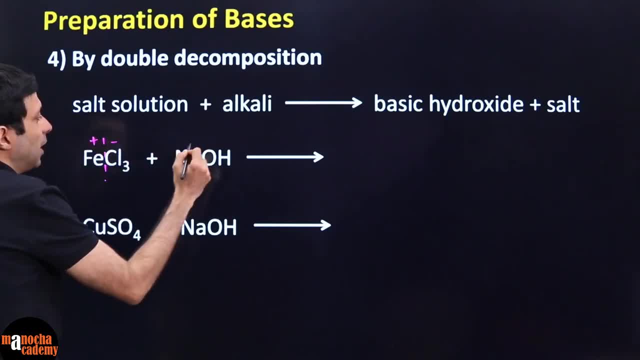 That means I think because it's not like acid base. So, maybe let's try double displacement. 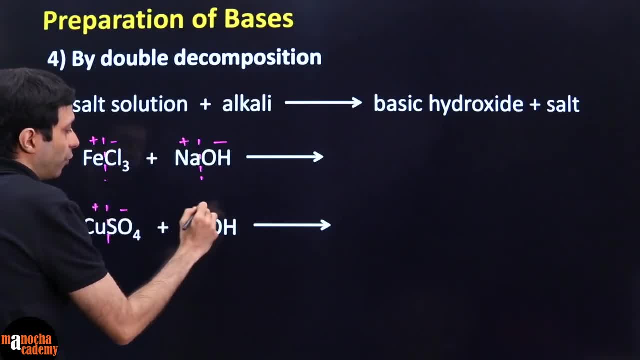 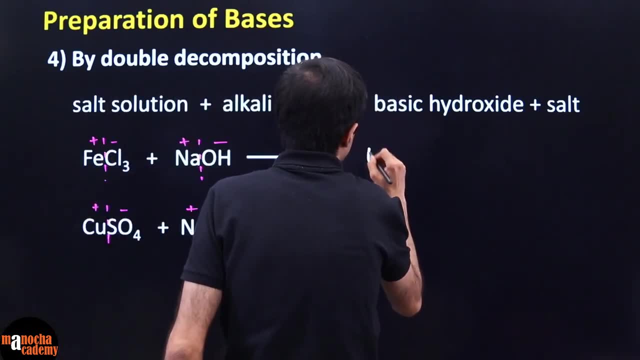 There is no chance of combination here, decomposition. So, for this, just try your double displacement. So, what will it give? Fe and OH will combine. So, it will give me FeOH, NaCl. 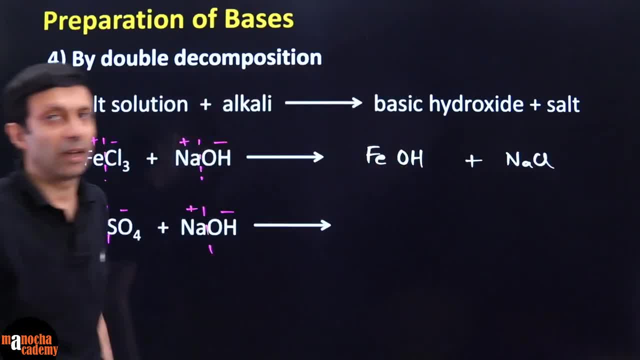 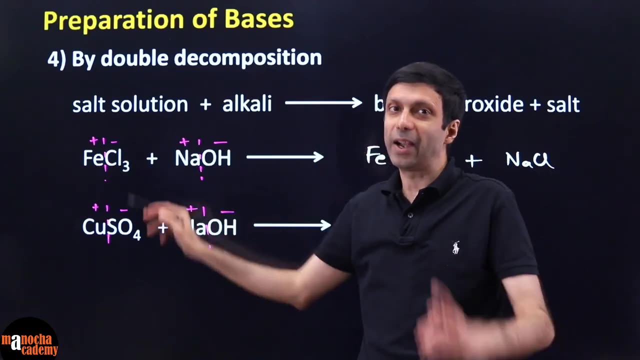 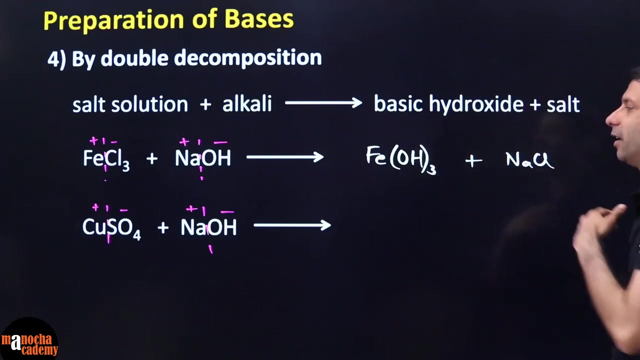 the question is what is the valency of iron what valency of hydroxide is one iron is how much valency usually the valency iron has two valencies ferrous ferric two and three but usually the valency on the left is carried on the right here you can see this is a ferric chloride iron with valency three so it will give me a ferric hydroxide that's it plus NaCl again you can balance out this equation I think you'll put a three here and a three here will balance it out same story for the 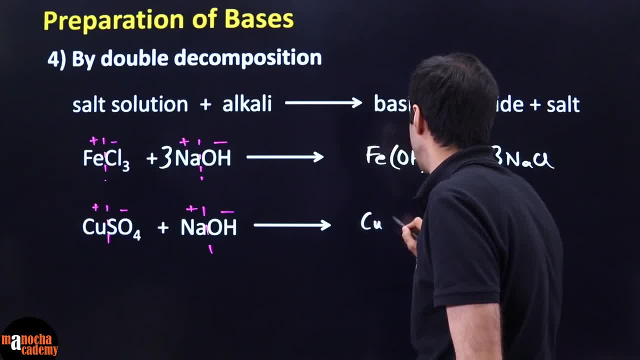 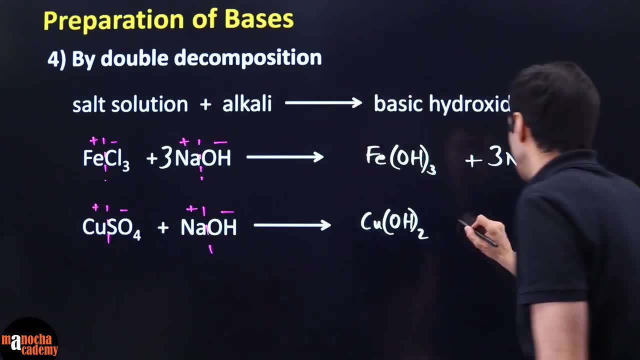 next one copper and OH will combine to give you copper hydroxide copper will carry its same valency of two so CuOH whole two Na and SO4 but please do not write NaSO4 that will make me really sad sulfate has valency two sodium has valency one so Na2SO4 crisscross your valencies clear 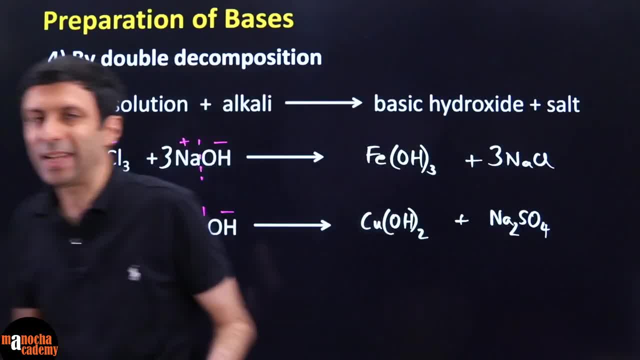 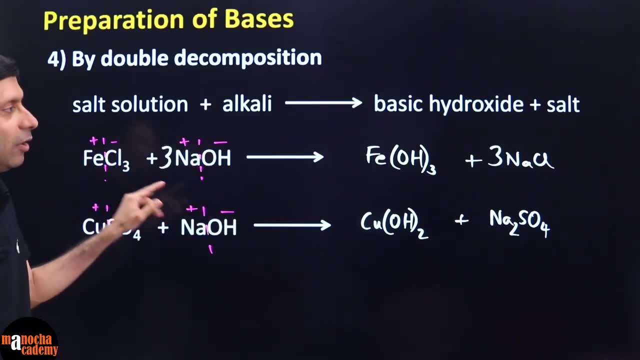 so can you see we are just switching the we are just exchanging the ions here but with the correct valency. It is not just playing lego. You cannot write FeOH plus NaCl3. You have to write according to the correct valency. Is this clear? 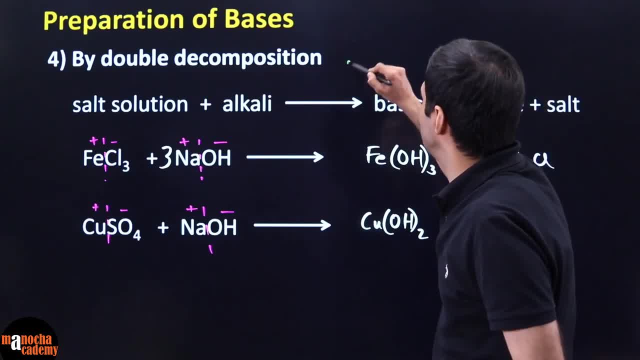 Double decomposition also known as or double displacement and you can see we are getting 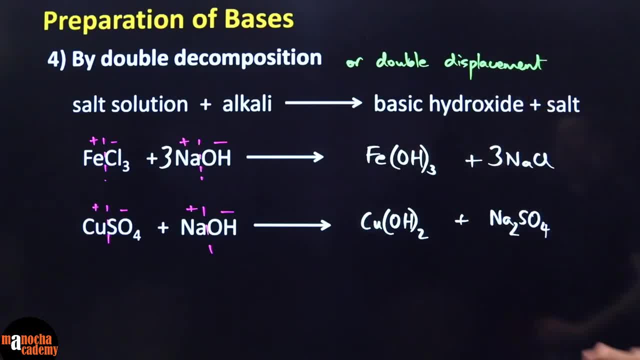 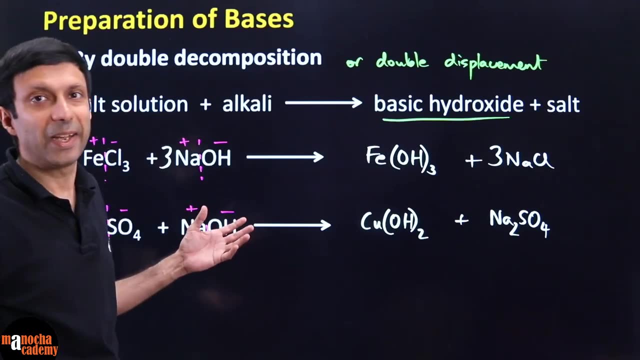 the hydroxides plus the salt. Hydroxide is your base. See these are your bases. So see ferrous hydroxide, copper hydroxide you cannot get by simply dissolving ferric oxide in water or copper oxide in water because it is not an alkali. It will not dissolve. So you prepare it by double 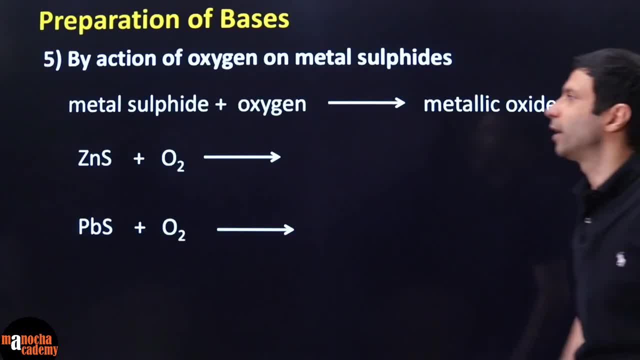 displacement. This is how you prepare these bases. Next one, by action of oxygen on metal sulfide. 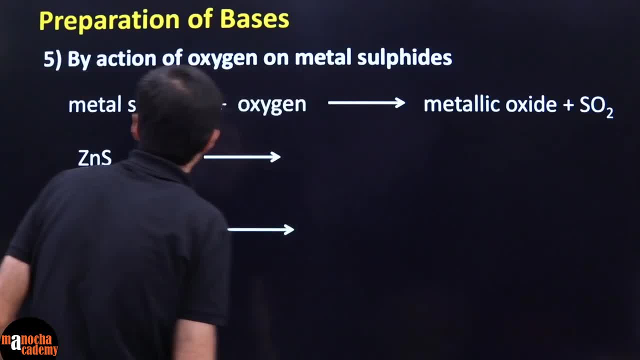 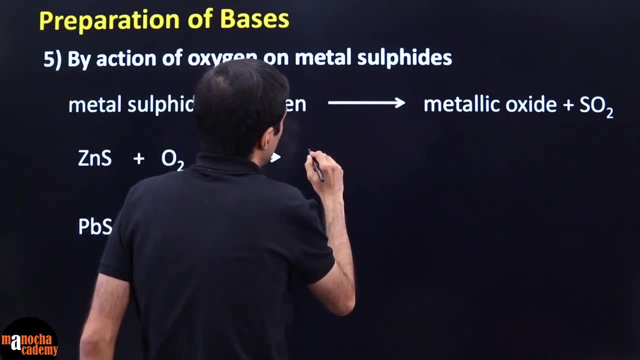 So what will happen here? When oxygen reacts with zinc sulfide, now what will happen? Oxygen is highly reactive with zinc and sulfur. So it is going to give me the zinc oxygen. So it is going to give me the zinc oxygen. So it is going to give me the zinc 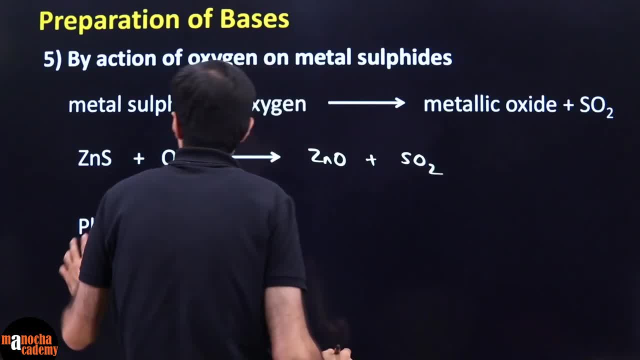 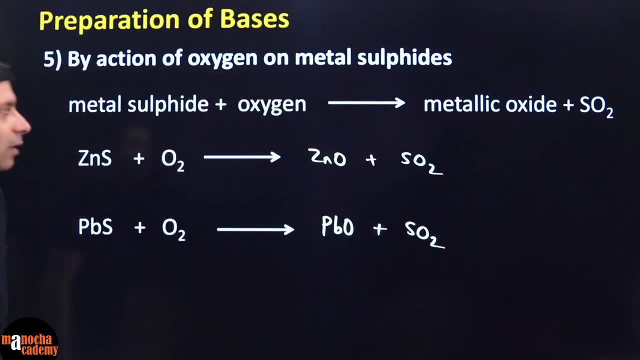 oxide plus sulfur dioxide. Same for PBS and oxygen. It is going to give me PBO plus sulfur dioxide. Okay. Again, make sure you guys balance this. See zinc is already balanced. Sulfur is 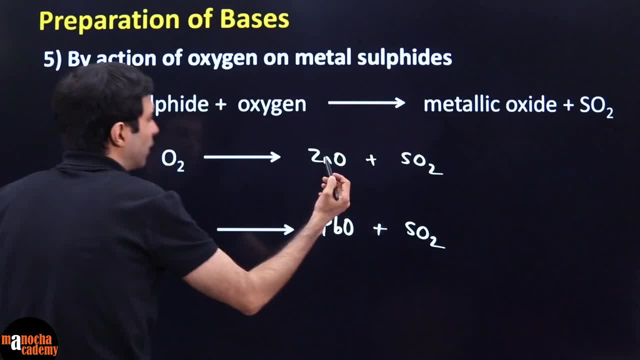 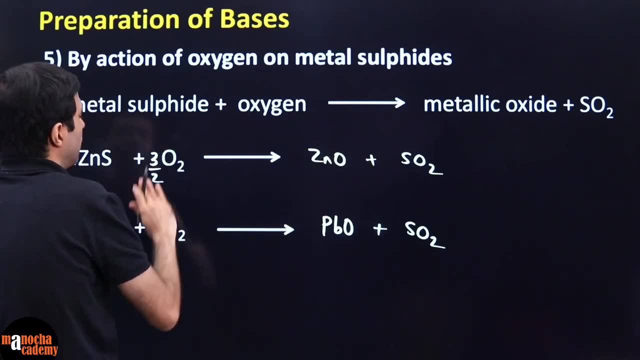 balanced. Only oxygen is not balanced. Oxygen is how many? Two plus one, three atoms here. Only two here. So we will multiply by three by two to balance it. To balance the entire thing, let's multiply the entire equation by two. There you go. Here also you can see, 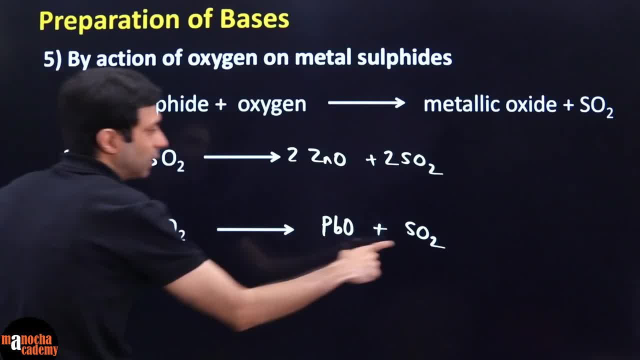 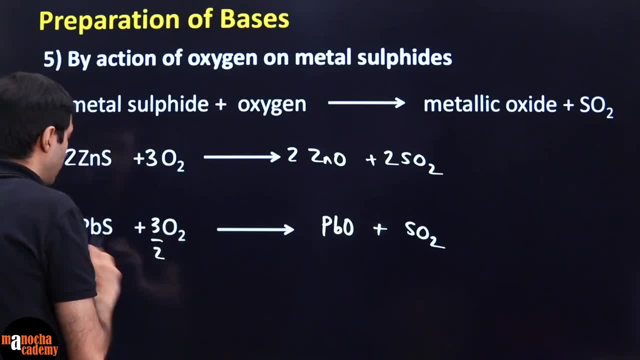 lead and sulfur balanced. Oxygen is not balanced. Two plus one, three atoms over here. So we will multiply by three by two fraction technique. See, three oxygen is balanced. Now get rid of the 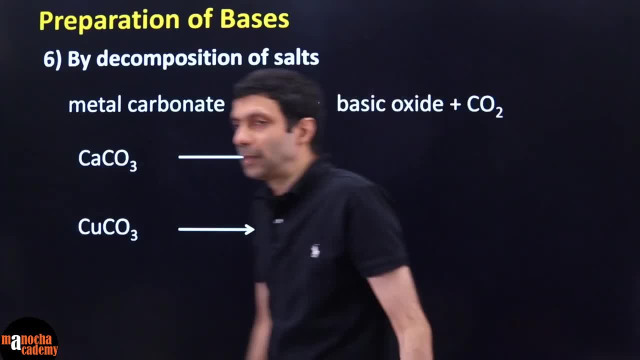 fraction. There you go. Done. You can also prepare bases by decomposition of salts. Decomposition 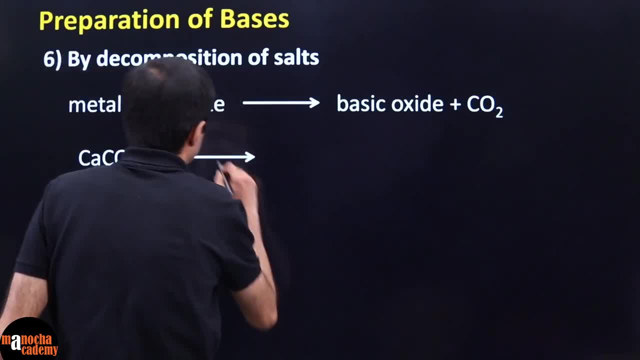 means breaking down. So let's say you heat these carbonates. So when you heat and it decomposes, 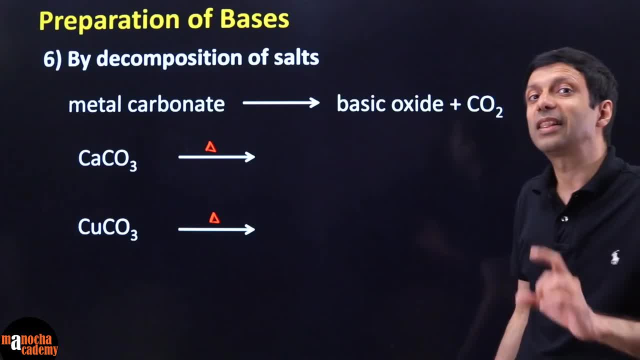 what is it known as? Decomposition under heat. It is called thermal decomposition. 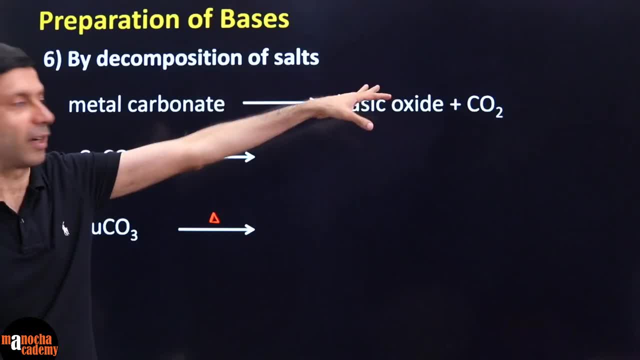 Decomposition, what does it mean? One reactant, many products. Okay. So what is it going to break down? Calcium carbonate, right? Marble chalk. When you heat it, it breaks down into 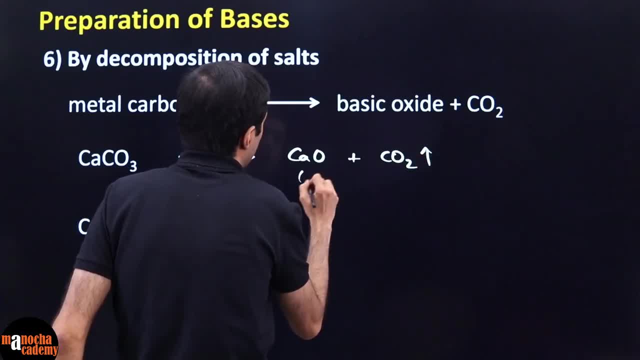 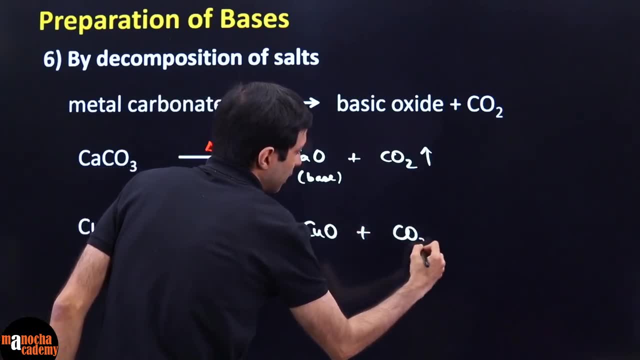 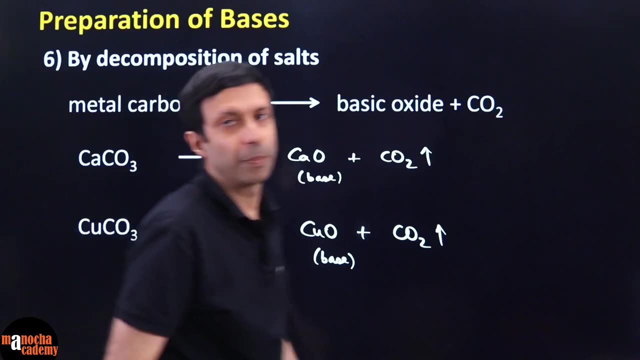 calcium oxide plus carbon dioxide gas. See, this is your base, the metal oxide. Similarly, copper carbonate, it breaks down into copper oxide plus carbon dioxide gas. See, this is your base, copper oxide. Clear? So this is how you can also prepare the metal 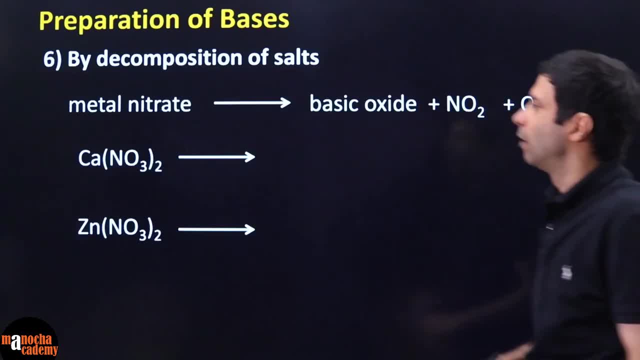 oxides, the bases by heating their carbonates. Metal nitrates. If you heat the metal nitrates, then also you can get a base. Like if you take calcium nitrate or zinc nitrate, 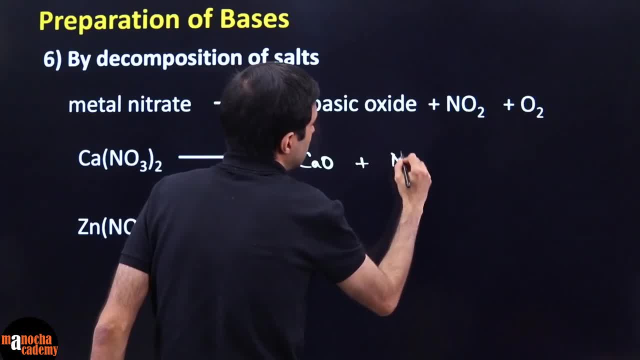 it will give you calcium oxide plus it's going to give you these gases, nitrogen dioxide and oxygen. 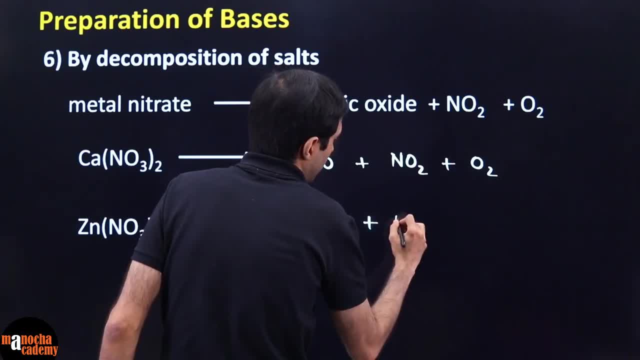 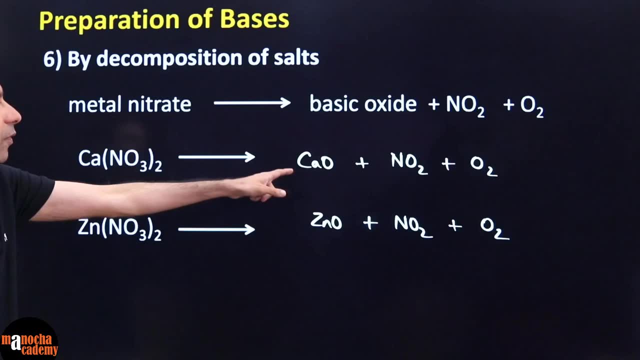 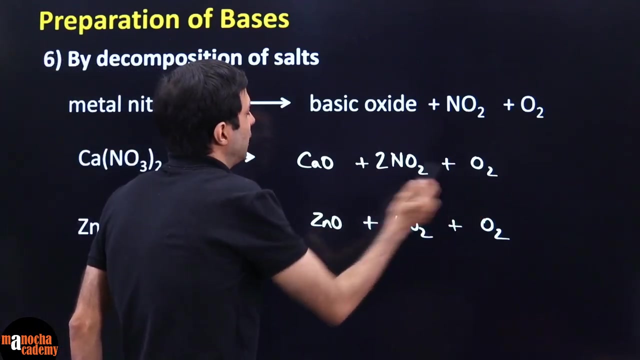 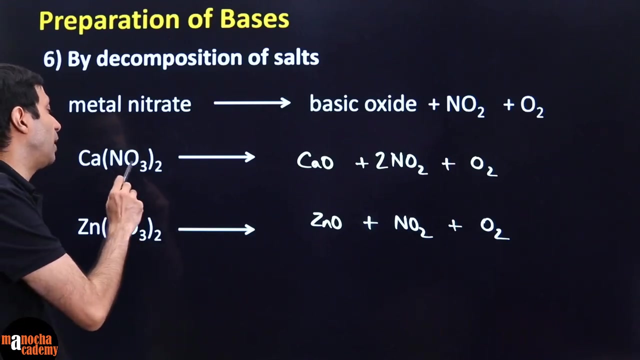 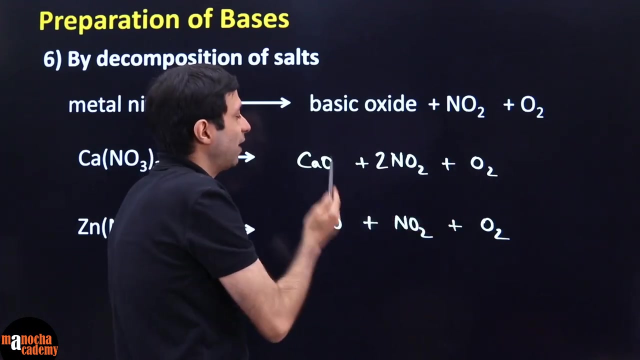 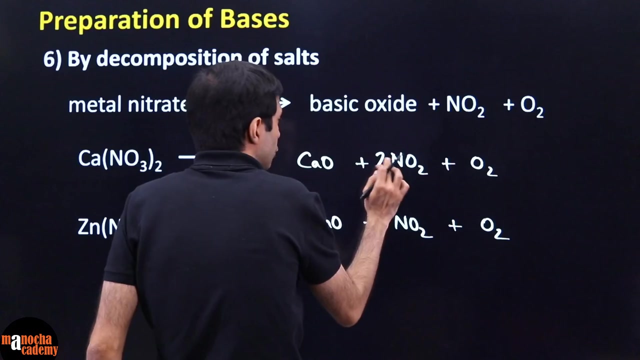 Similarly here, it will give you zinc oxide plus NO2 plus O2. Now make sure your equation is balanced. So again, you can see calcium is one, one balanced. Nitrogen is, two over here, only one there. So let's multiply by two. How many oxygen here? Three times two is six. How many here? Four, five, six, seven. See, this is where fraction will really help you to balance this fast. How? Because you have three times two, six oxygen here. How many you have on the right side? Two times two, four plus two, six, seven. Now you want how many? Six. But you have a lone oxygen there. You can put whatever fraction you want in front of it. So you have two times two, four plus one, five. You need only one more, but you have two. So if I half it, I'll get it, right? 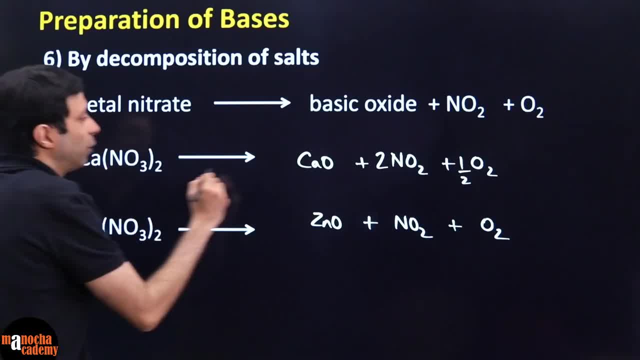 Now you want to get rid of that half. You just multiply the entire equation by two. 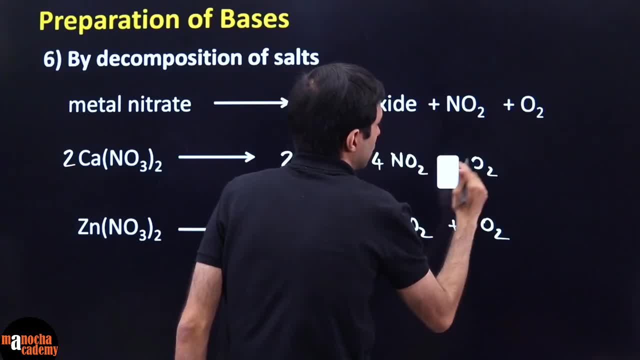 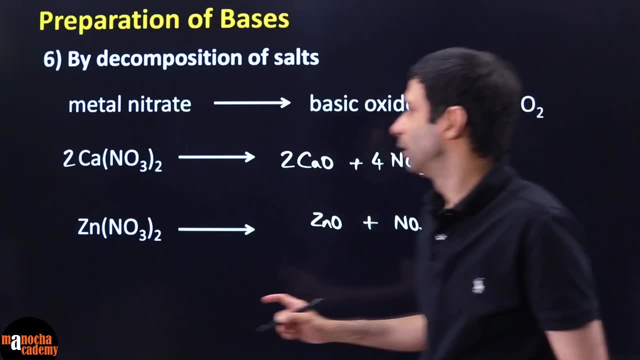 You're done. See how fast it is. So if you learn this fraction technique, it can help you to balance it very fast. Similarly for the next one, the, since the valency of calcium and zinc 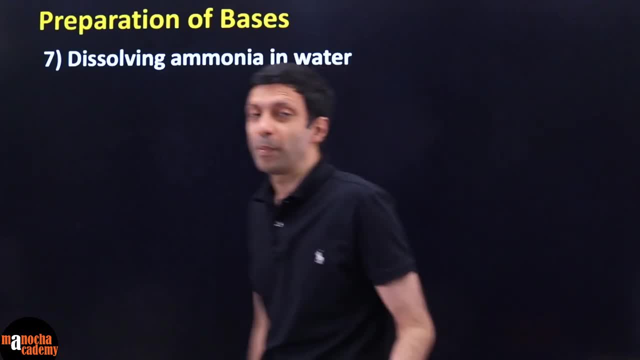 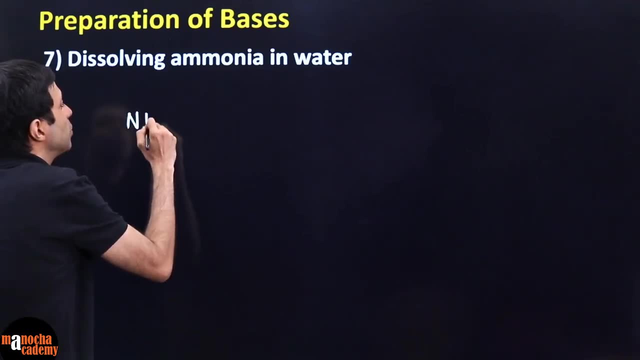 is the same answer here. Clear? You can also prepare bases. You have this base ammonia and water. Can you guys tell me what base will you get here? Ammonia is what? Nitrogen and three hydrogen. Nitrogen has valency three, hydrogen one. So, but we write nitrogen first. So ammonia is NH3 plus water. Can you guys predict what, what base we'll get here? One hydrogen. If you combine here, you get NH4OH. This is ammonia. So, you can also prepare bases. So, you can also prepare 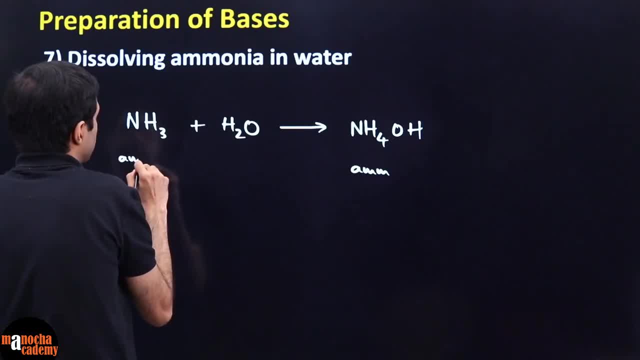 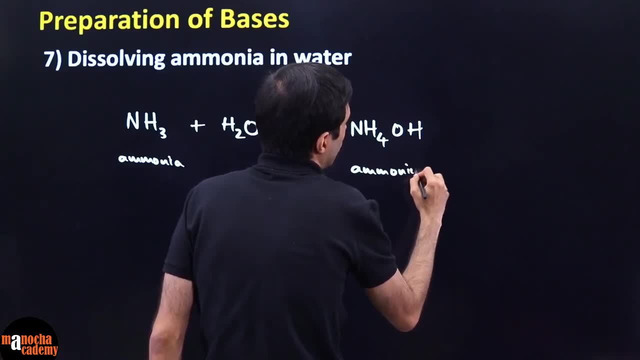 bases. Ammonium hydroxide. This guy is ammonia gas. Ammonia gas is highly soluble in water. On dissolving in water, it gives you ammonium hydroxide. Ammonium hydroxide is also a base. 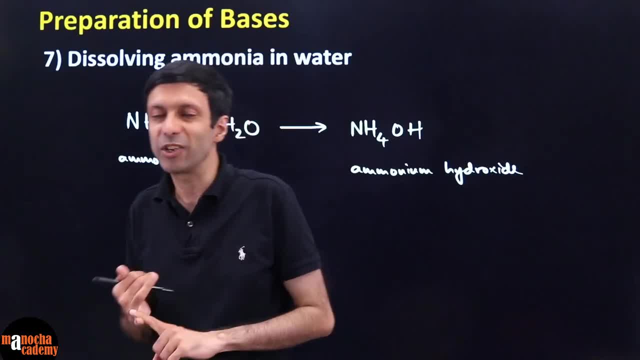 Like I told you, the famous alkalis are sodium hydroxide, potassium hydroxide, calcium hydroxide, ammonium hydroxide, magnesium hydroxide, semi-soluble. Now let's talk about the chemical 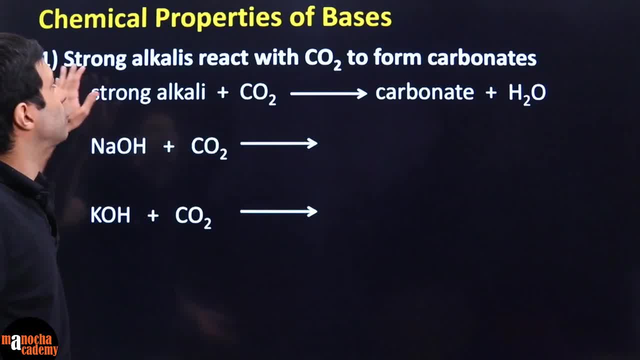 properties of bases. Chemical properties means chemical reactions. So strong alkalis, we know 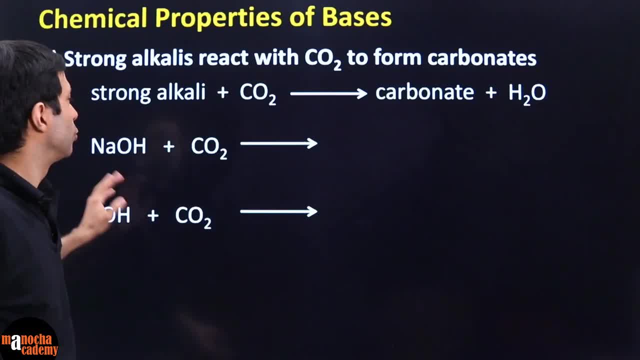 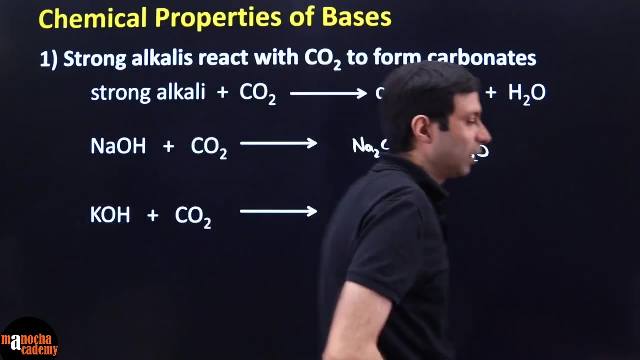 with carbon dioxides to form carbonates. Okay. So, what will happen? Like let's say you take sodium hydroxide and carbon dioxide. What will happen? The sodium oxide and carbon dioxide will combine to form sodium carbonate plus water. Now, what is a good way to learn this? Because you can 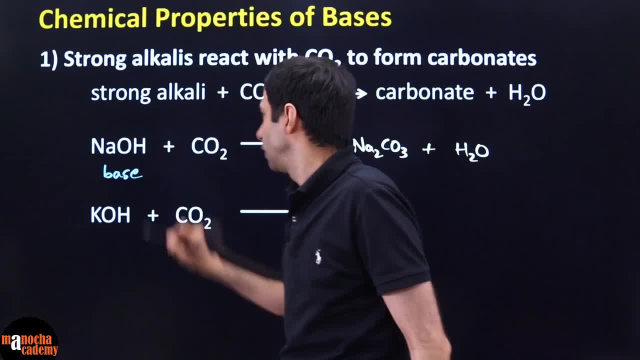 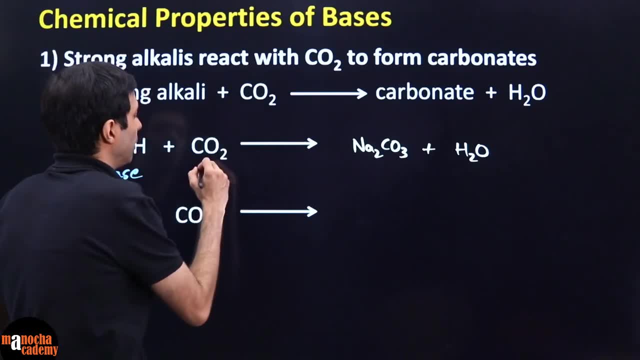 see that sodium hydroxide is a base and carbon dioxide, carbon dioxide is not an acid exactly because acid must contain hydrogen. But we know that carbon dioxide is a base. So, we can see that 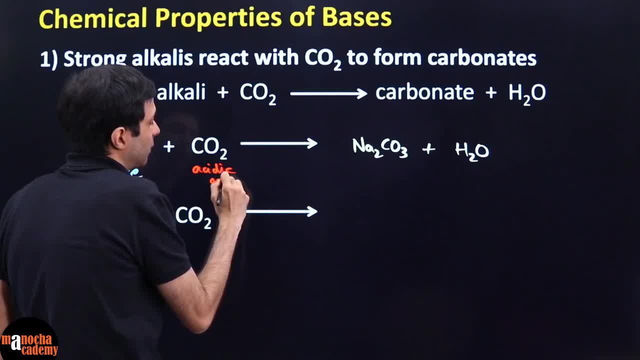 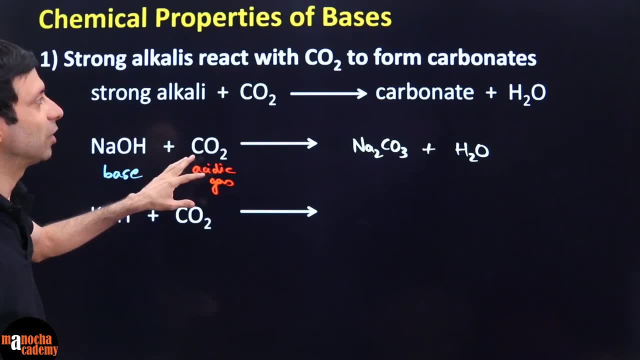 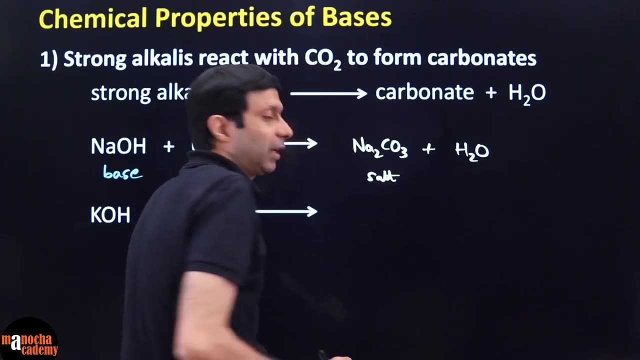 we know it is acidic gas because when you dissolve it in water, it gives carbonic acid. So, you can see finally a base and acidic gas, right? Gas which is acidic in nature is bound to give you salt plus water. So, see it's basically like a neutralization that is happening. Not perfectly a neutralization 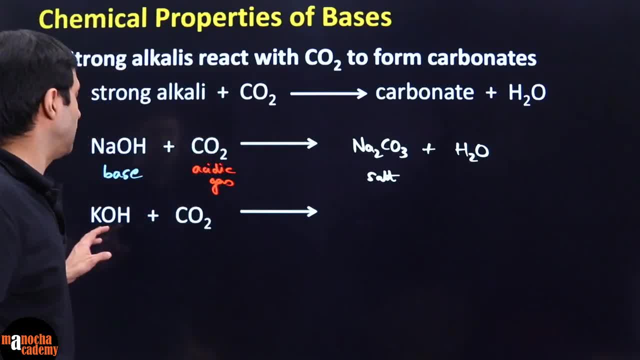 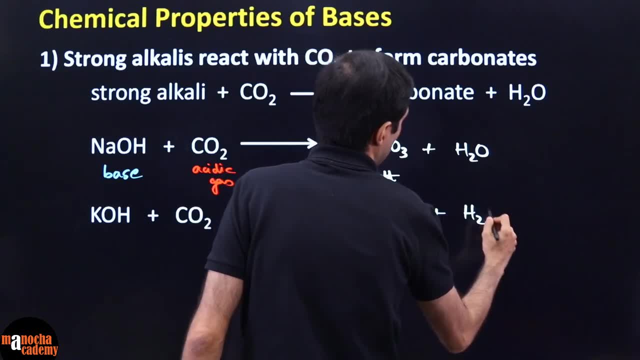 because this is not an acid. It's an acidic gas. Same thing with potassium hydroxide and carbon dioxide. What will you get? You'll be getting K2CO3 plus water. And of course, you should 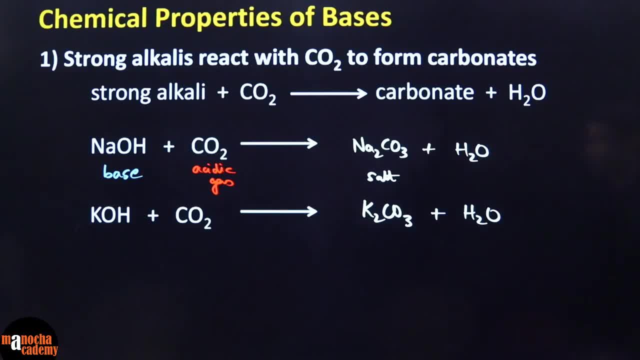 balance these reactions. Clear? Can you guys see how we are getting a base and acidic gas? So, is it making sense that we are getting a salt and water? If you want to write the state of matter here, 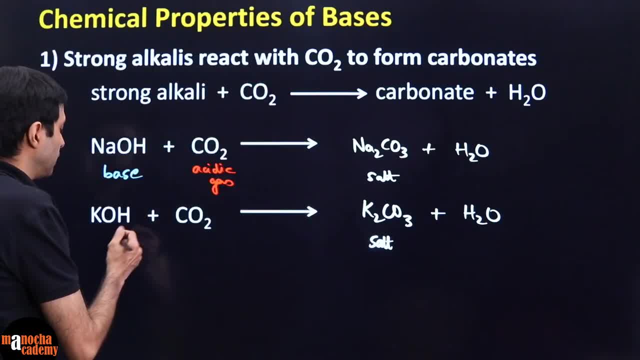 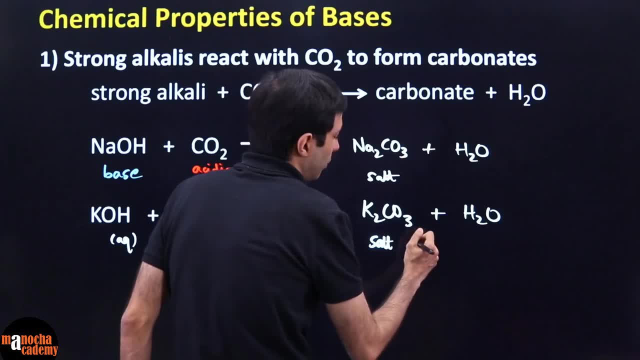 what is the state? Let's try it for this one. Potassium hydroxide is soluble in water. So, we write aqua state. Carbon dioxide is a gas. So, you should write G. Potassium carbonate is soluble 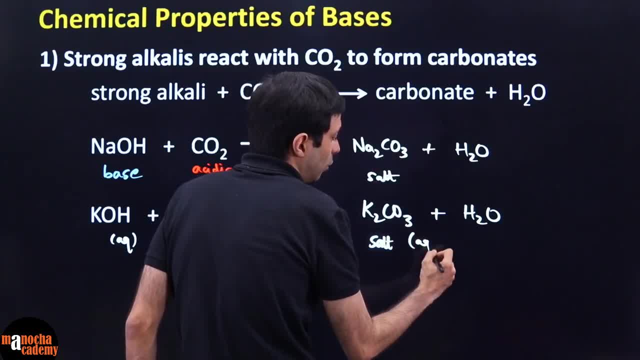 in water because also sodium potassium salts are soluble. So, we write AQ and water itself is a liquid. 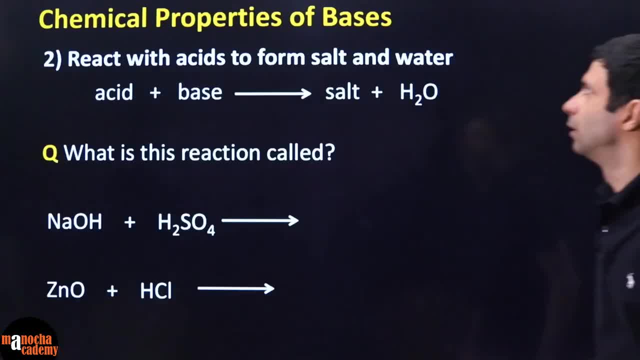 So, there I have written the states of matter also if you want to write them. 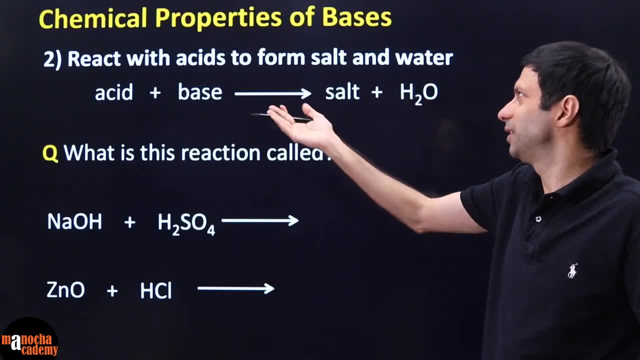 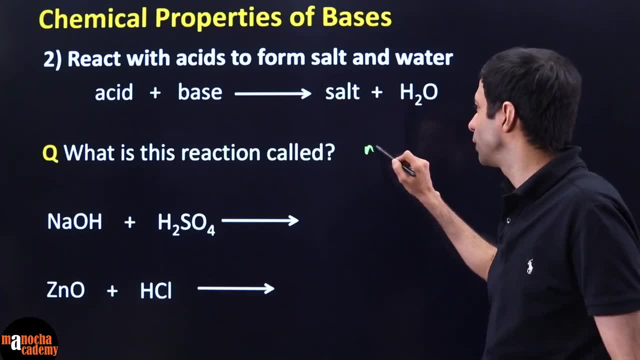 We know that acid reacts with base to form salt and water. Similarly, same thing, right? Bases will react with acids to form salt and water. This is that famous reaction which we have discussed. Always questions come on this reaction. This is the neutralization reaction 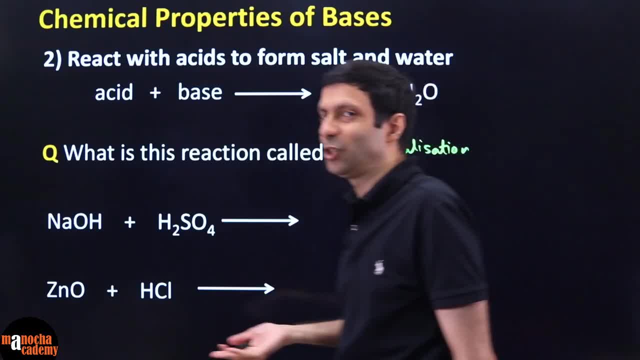 because acid is neutralizing the base or base is neutralizing the acid. So, can you guys work this out for me? Sodium hydroxide plus sulfuric acid. What will this give? 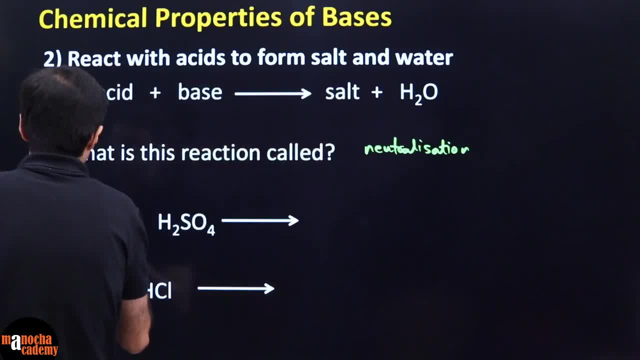 The easiest way again I told you. It is finally like a double displacement. 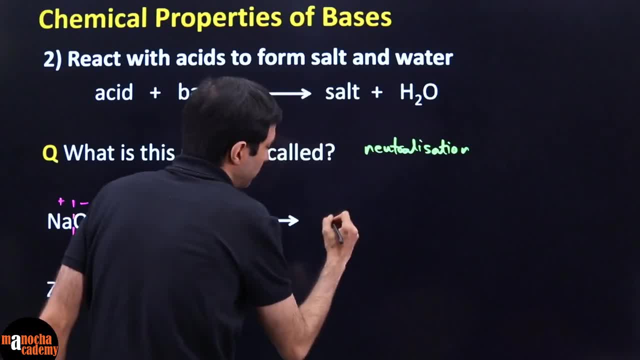 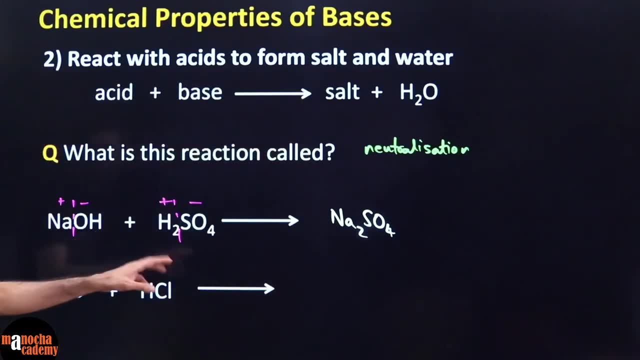 So, sodium and sulfate will form the salt, sodium sulfate, but carefully think of the valency. Sulfate has valency II, sodium one. So, it is going to be Na2SO4. H and OH will r Give you 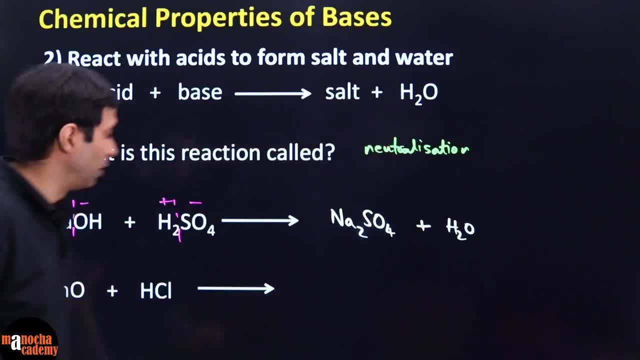 water. Done. There you go. You got your salt and water. What about the next one? Zinc oxide plus 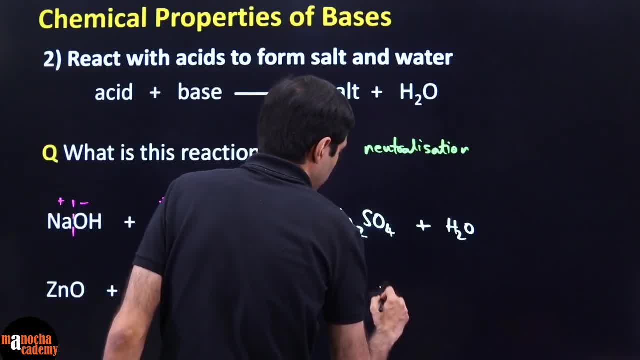 HCl. Again, you will get your salt and water. Z and Cl2 plus H2. Okay. 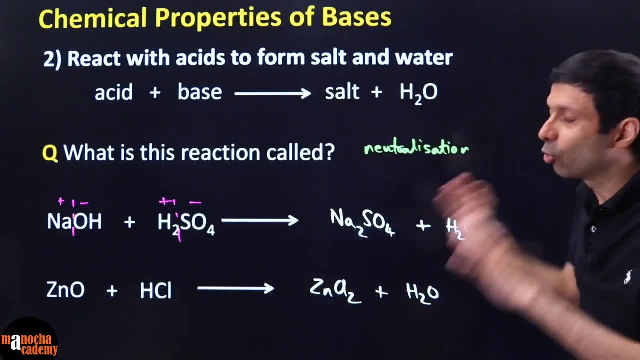 Again, I m leaving this to you. Again, we have found that nitrogen dioxide continue to form the sal- sodium sulfate. them unbalanced for you because my goal today was to teach you how to predict these reactions how 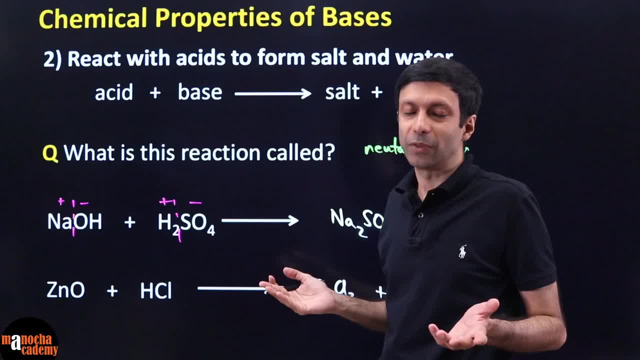 to understand these reactions so that you don't have to memorize so many of them right you can easily predict any of these this one let me write it a little more clearly it's looking like zinc 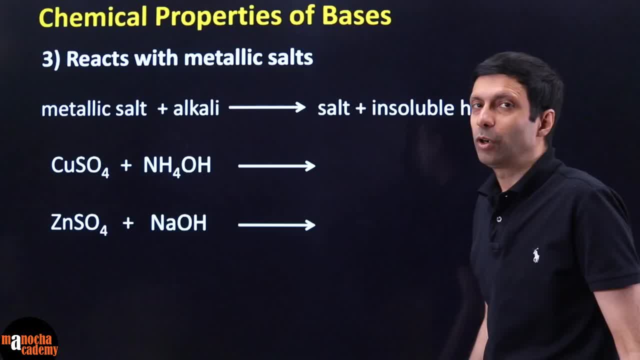 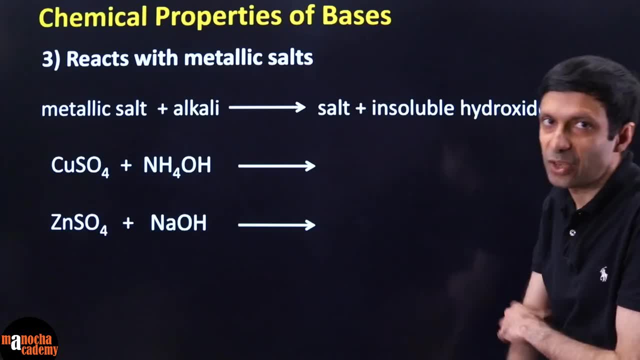 oxide it's zinc chloride cl2 how about this one metallic salts when it reacts with alkali again can you predict it suppose you have never seen this reaction can you predict it 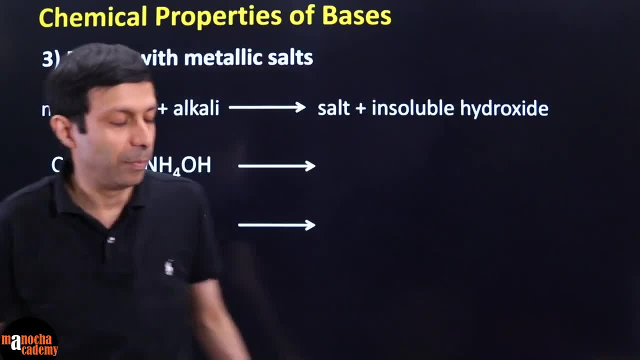 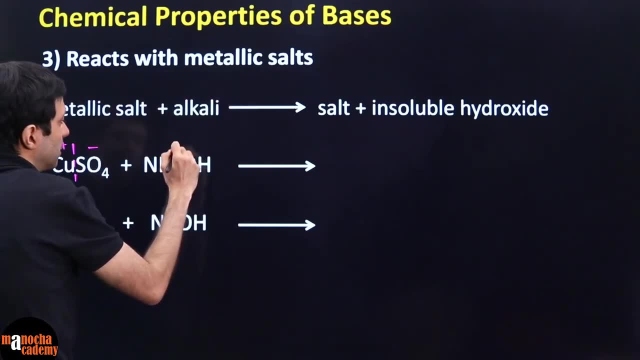 see again you can see the trick there's a salt and a base right ammonium hydroxide or sodium hydroxide you try your double displacement plus minus plus minus so what will this give me copper 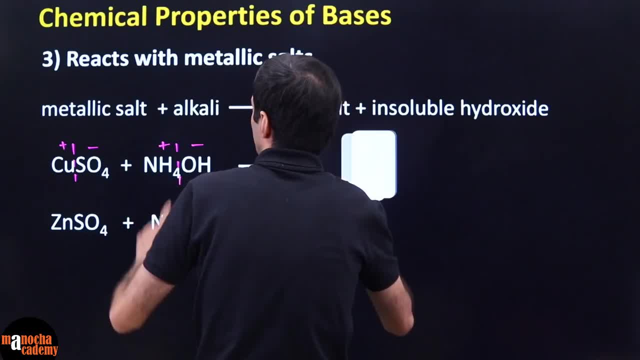 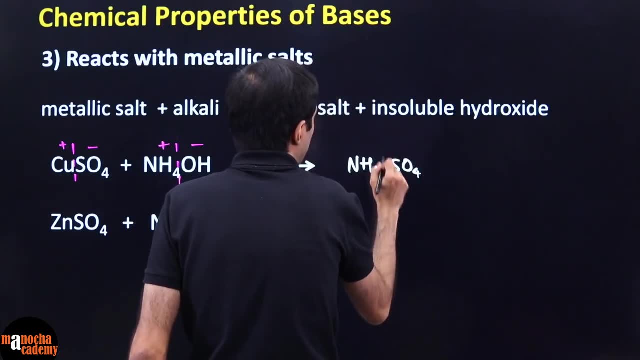 and oh will give me or let's first do ammonium and sulfate that's going to give me ammonium sulfate ammonium has valency 1 sulfate 2 so this whole thing will come under a bracket because nh4 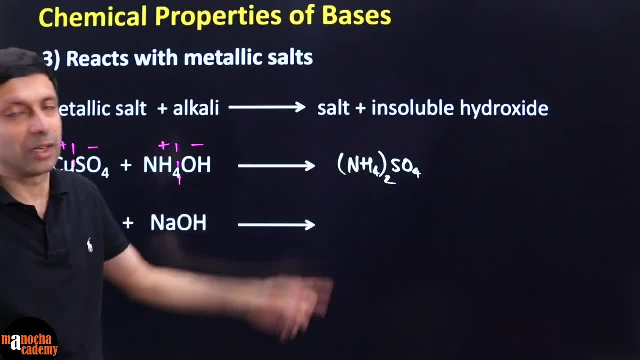 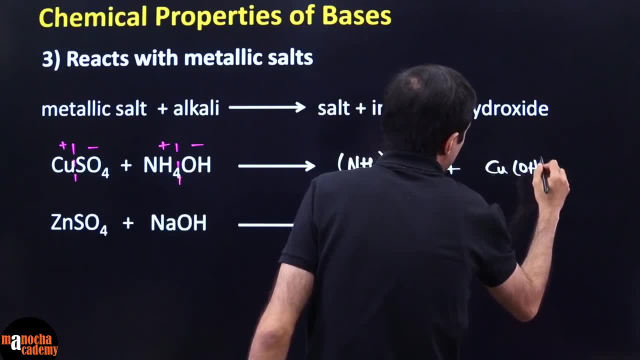 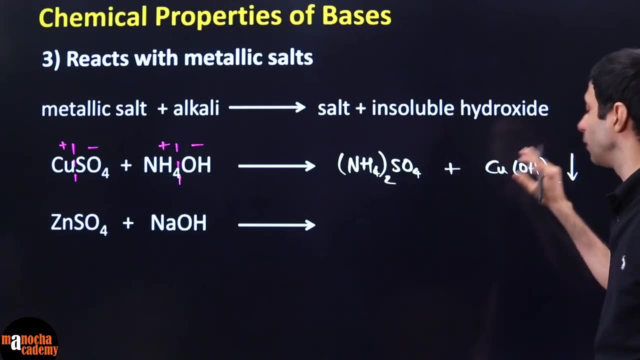 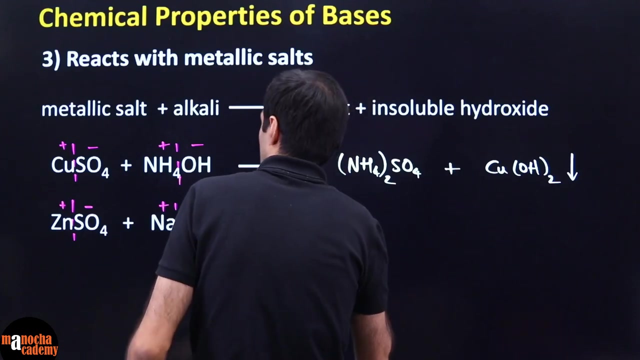 is an ammonium it's a it's an iron right so the whole thing comes under two ammonium sulfate plus what are we left with copper and oh copper will carry its valency too so it is going to be copper hydroxide we know that copper hydroxide doesn't dissolve in water so it will precipitate out in fact it forms a bluish precipitate right so insoluble hydroxide can you guys similarly predict the next one again very simple break it cut these compounds into its positive negative zinc is zn plus this is the positive radical negative radical again sodium and hydroxide positive negative come on guys exchange the ions so sodium and sulfate will give you ne2so4 plus 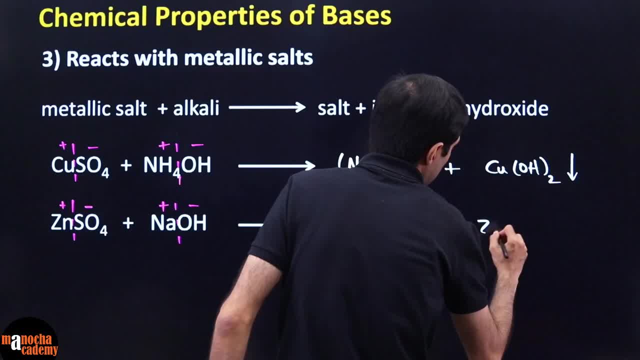 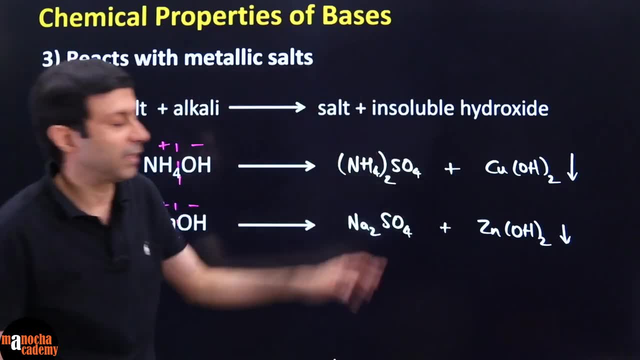 you have zinc and oh will give you zinc hydroxide again zinc hydroxide not soluble in water so it will precipitate out see we are getting salt plus insoluble hydroxide we are getting salts and insoluble hydroxide 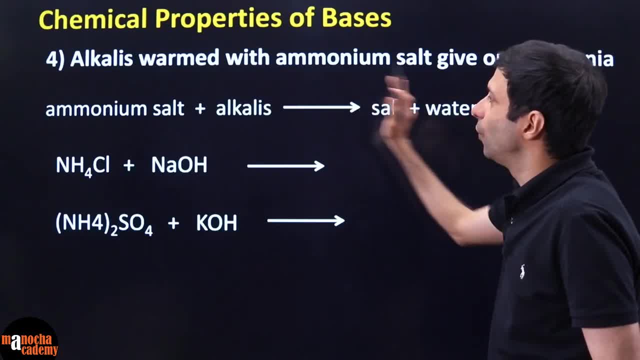 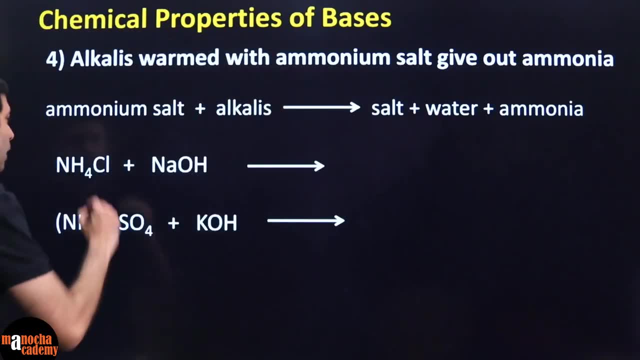 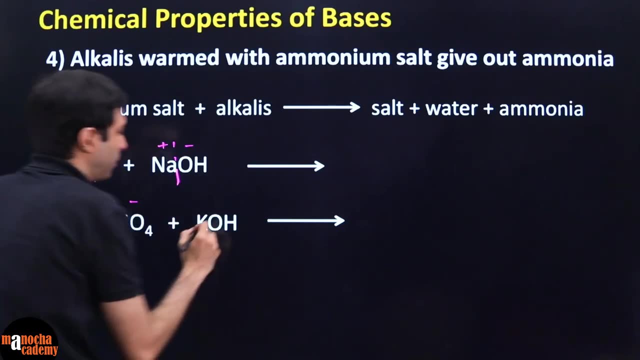 let's try another one alkali is warm with ammonium salt will they end up giving ammonia let's try to predict these ones so what is the prediction here again we will do double so you can see many of them are just working with simple double displacement okay so let's do that plus minus plus minus 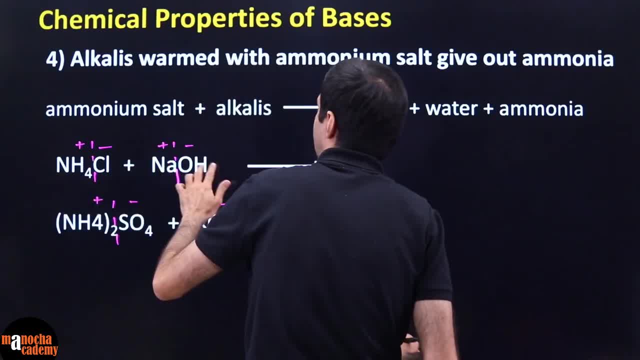 what do we get out of here and and it looks like these 2 as i said so we want to do 3 of these so and 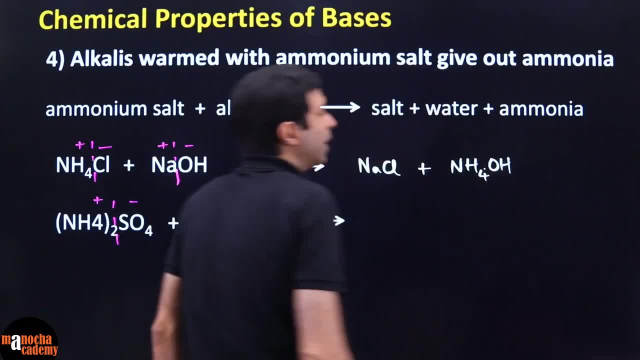 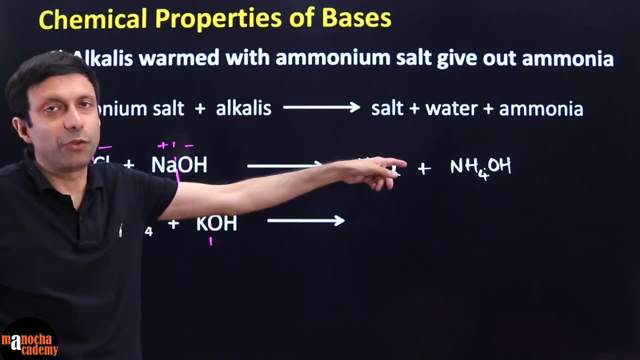 let's get back to the two tweeters for this one so i'm gonna use the distance which i've warts okay of distance of dihnahmen right good solet's stop this question for a second 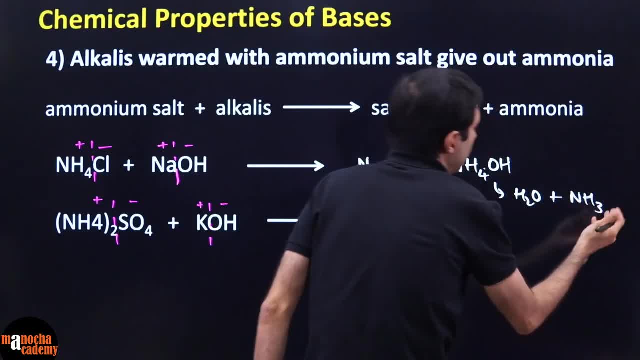 so the distance from point to point is regardless of the satiety of the acid Similarly, it will break down easily. 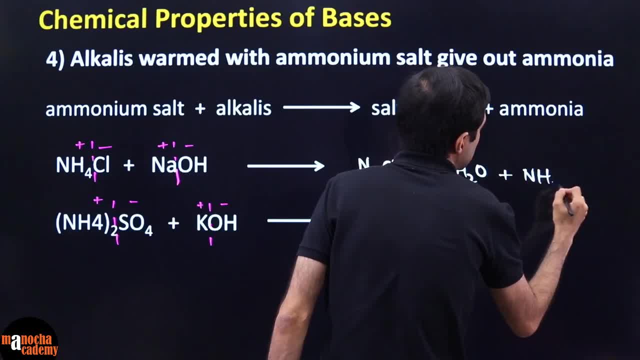 So, the answer is going to be water plus ammonia gas here. Similarly, if you take ammonium sulfate and potassium hydroxide, what will you get? You are going to be getting potassium sulfate, K2SO4. 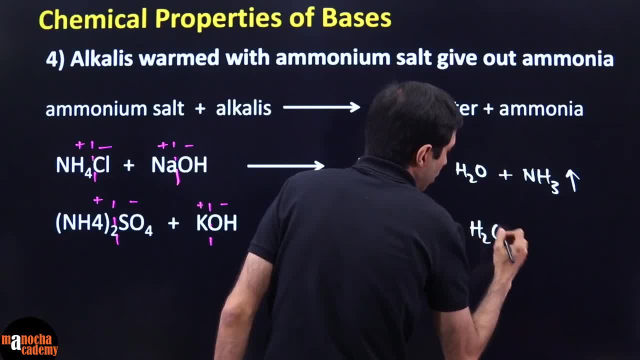 And again, ammonium hydroxide, which is going to break down into water and ammonia. 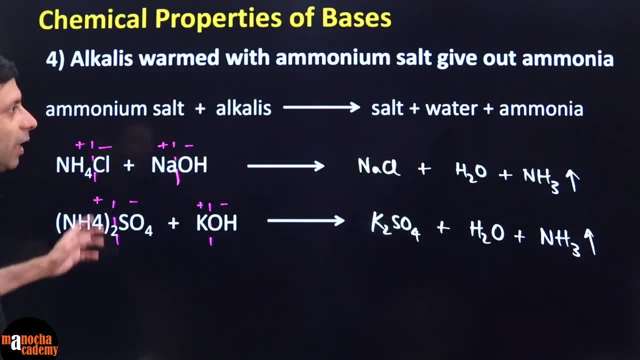 The only final thing you are left to do is to balance it. Like, I think the first equation is already balanced. The next one is a K2SO4. So, I need to multiply by 2 here. And ammonium is 2. So, maybe you need to multiply this by 2 here. You can check how many is the hydrogen balanced. Hydrogen is 4 times 2, 8, 9, 10. And here you can see 6. So, I think we need to multiply by 2 here. There you go. Done. 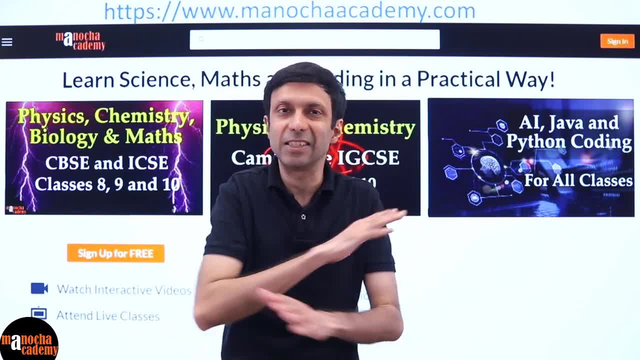 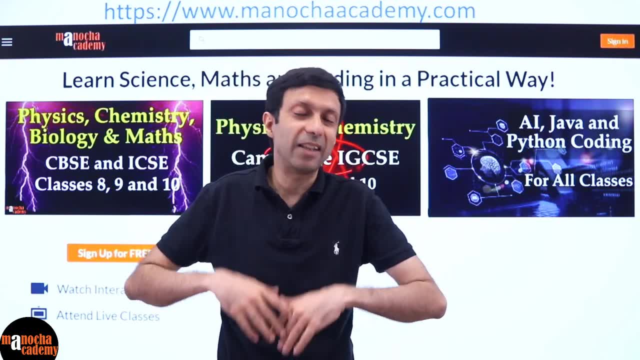 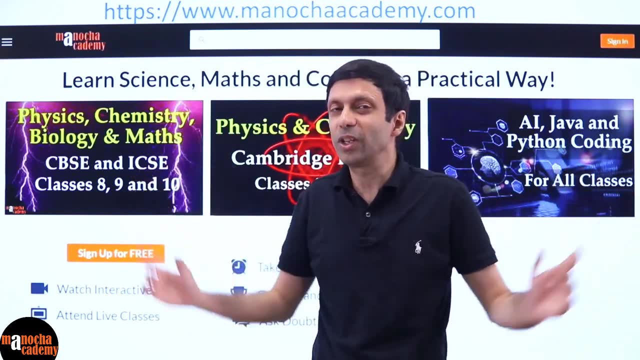 So, hope you guys found this class. Useful where we did the acids and bases in one shot. We compared the properties of acids and bases. We looked how to prepare acids and bases and their chemical properties as well. And I showed you the tips and tricks on how to predict these chemical reactions. So, do check out the other courses on our website. 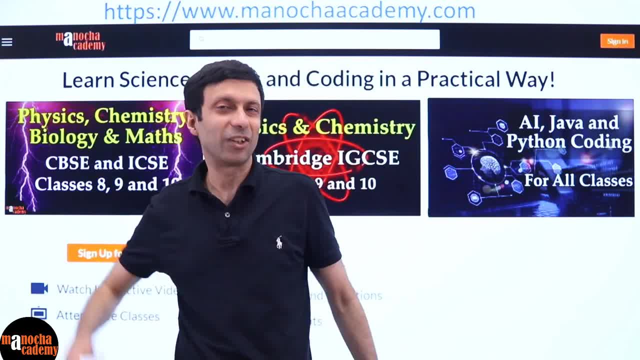 Make sure you have subscribed to our YouTube channel. You can follow us on Facebook and Instagram. So, stay connected with Manocha Academy and keep learning. 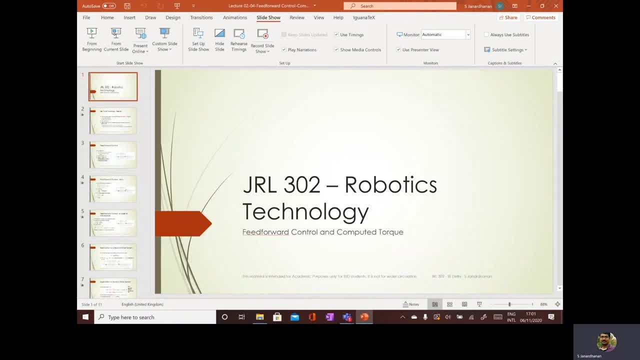 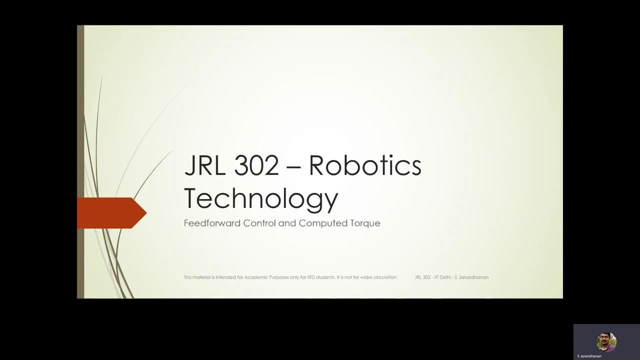 Okay, so in the last class, we had talked about PID control and how it can be used for set point tracking. That is the case when you have a constant reference signal and a constant disturbance. But this entire exercise, the consideration that the reference is constant and also the set point, the disturbance is constant is something that is not very realistic. 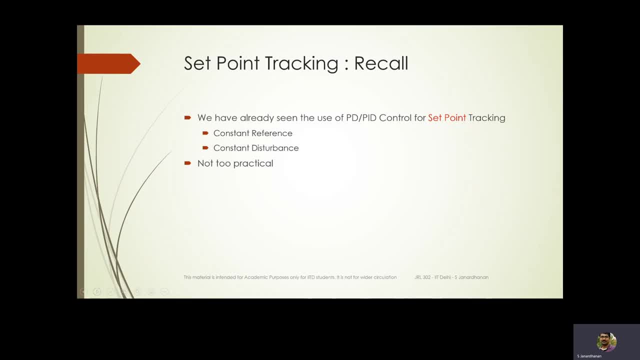 If you are talking about manipulator control, your manipulator set point, the way the target of your manipulator is set, the way the target of your manipulator is set, the way the target is actually a trajectory. And that trajectory is seldom constant. You may, in certain special cases, you may have a case where specific points are given. However, it is more often than that, you would have a trajectory as a reference signal. Okay, so I have QDT or theta DT